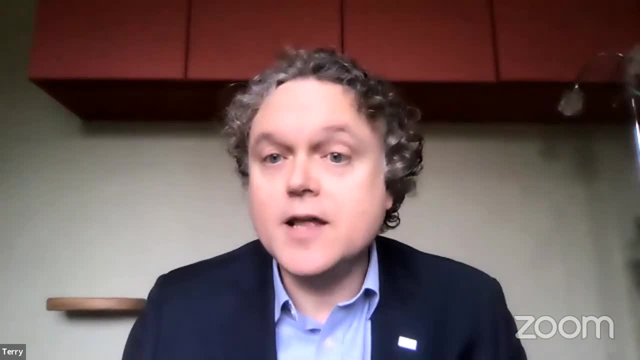 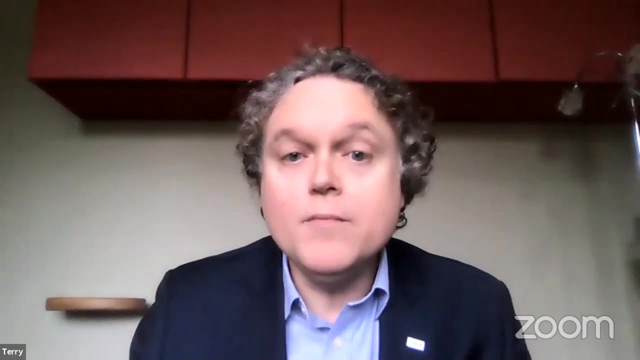 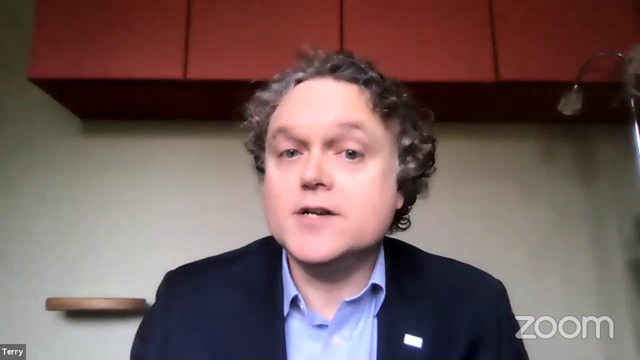 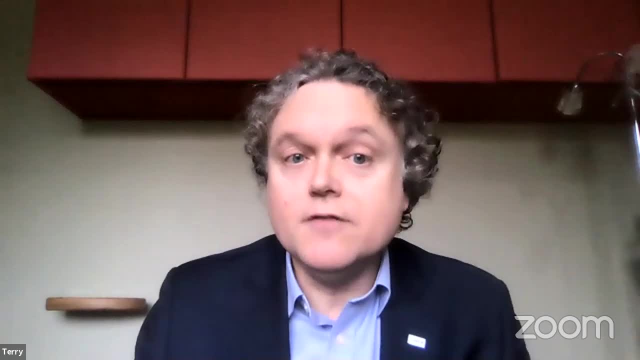 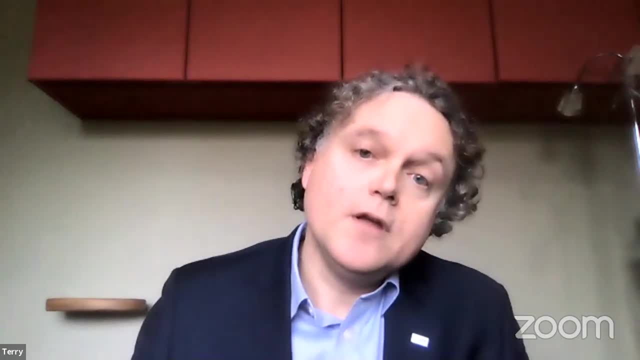 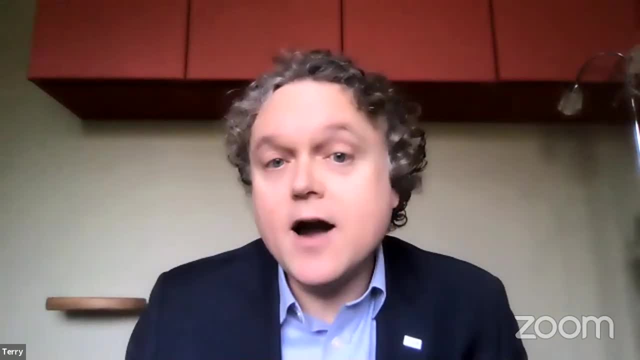 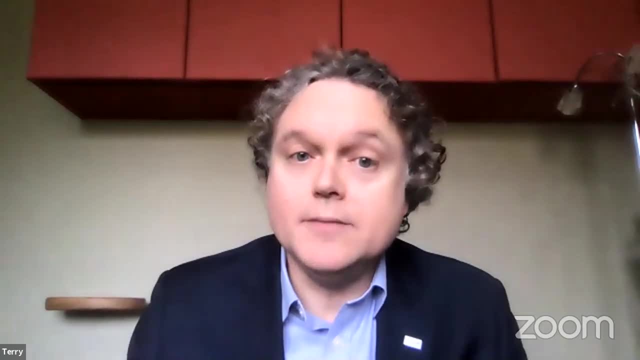 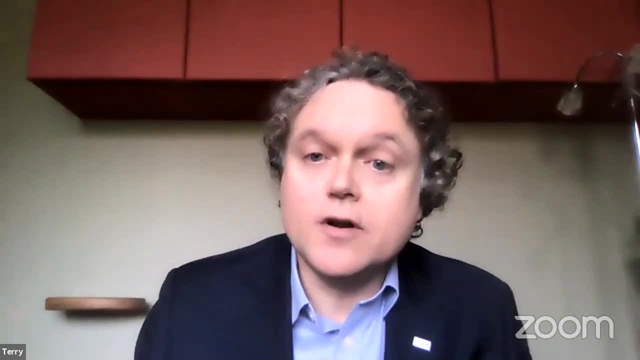 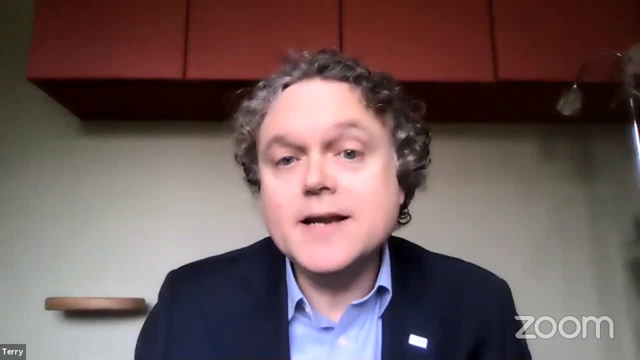 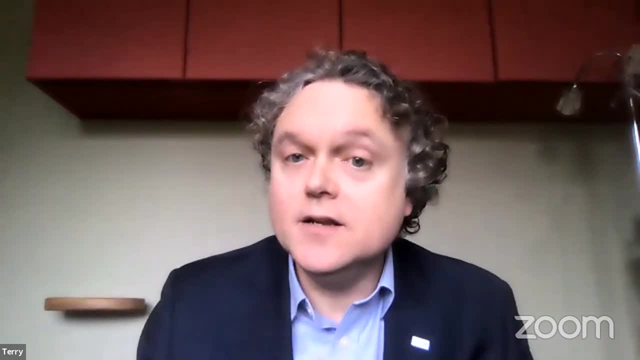 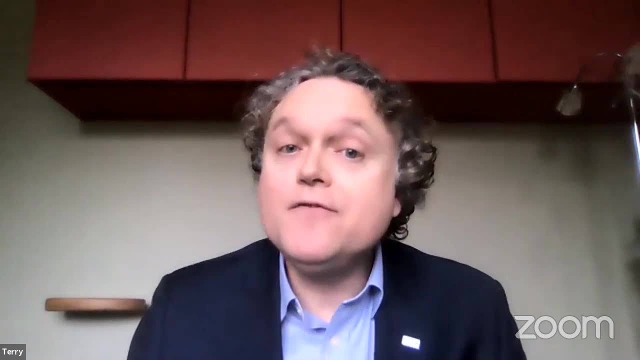 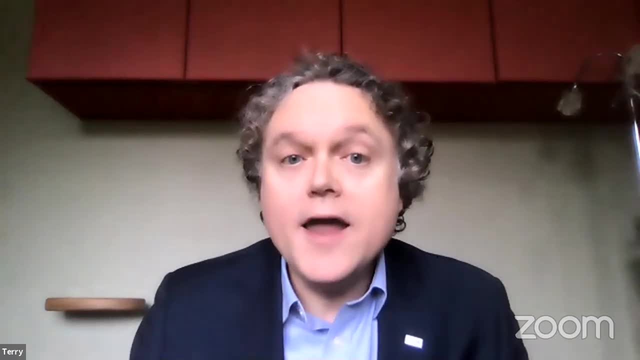 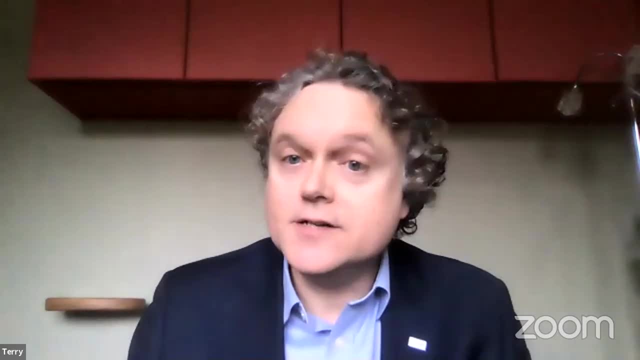 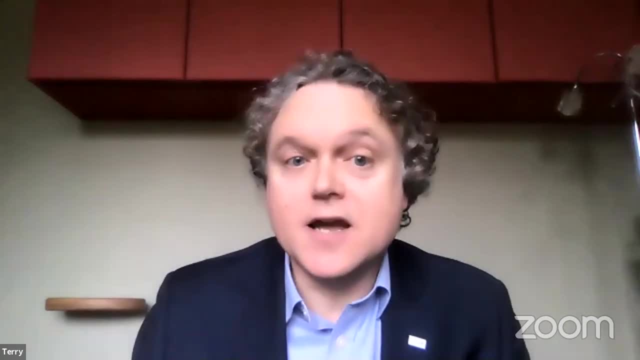 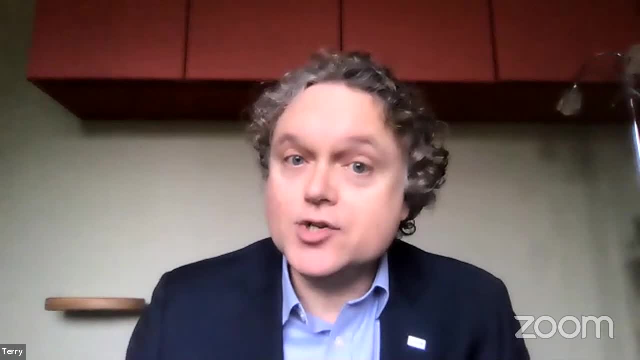 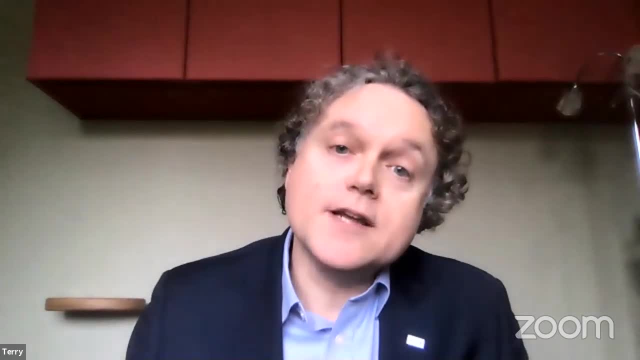 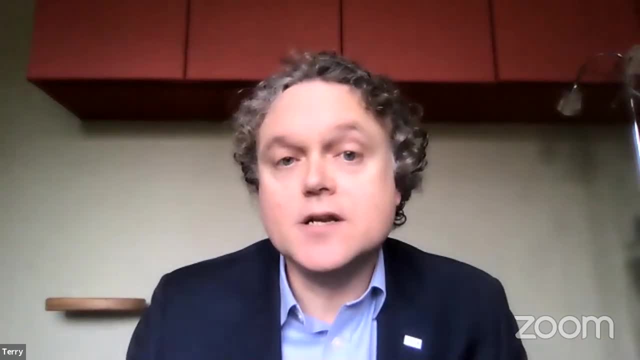 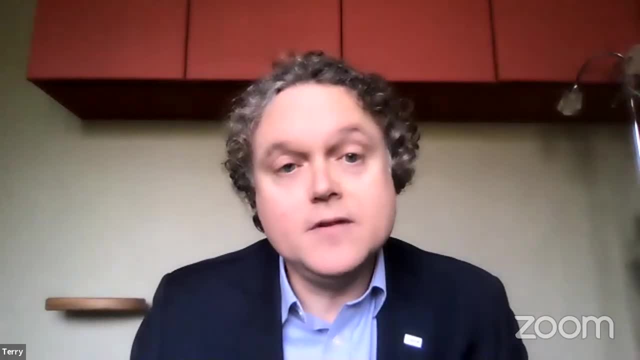 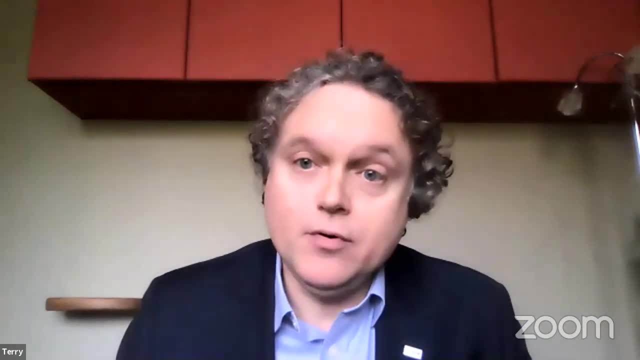 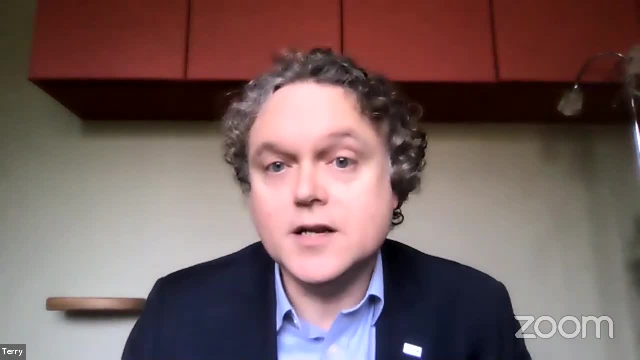 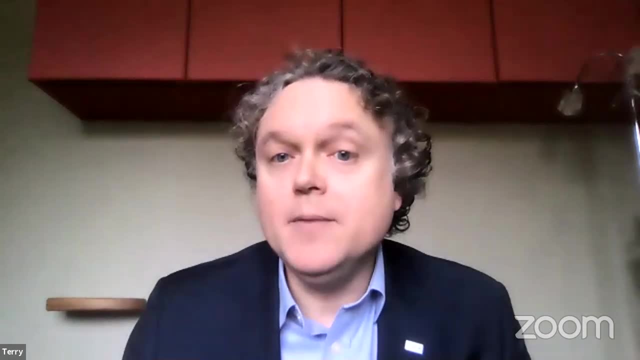 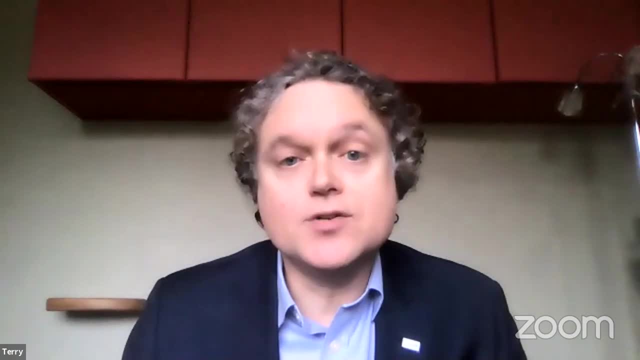 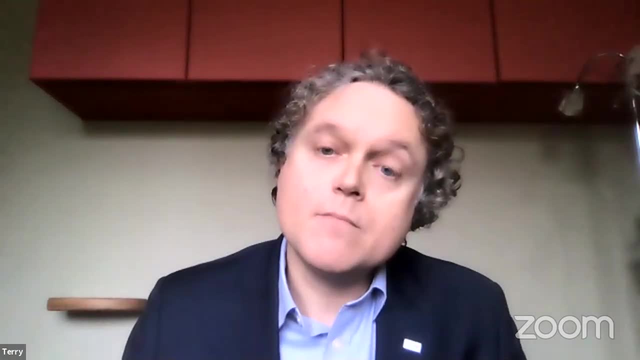 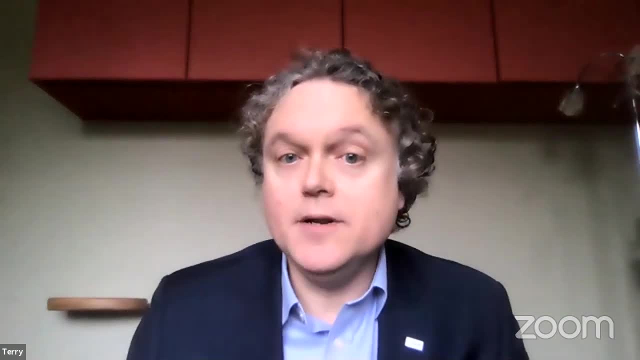 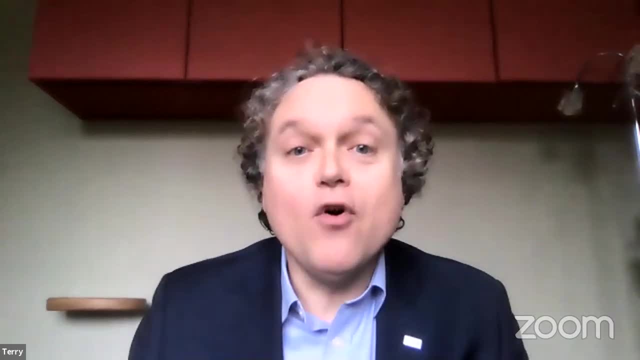 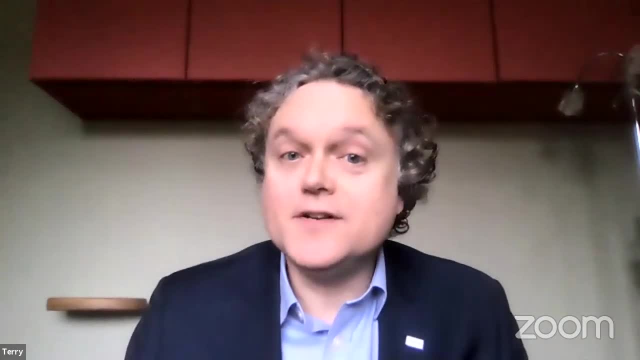 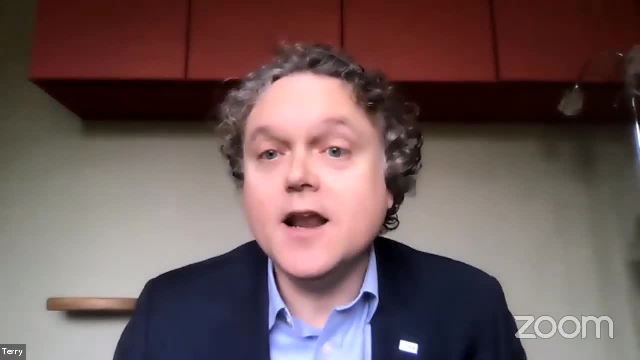 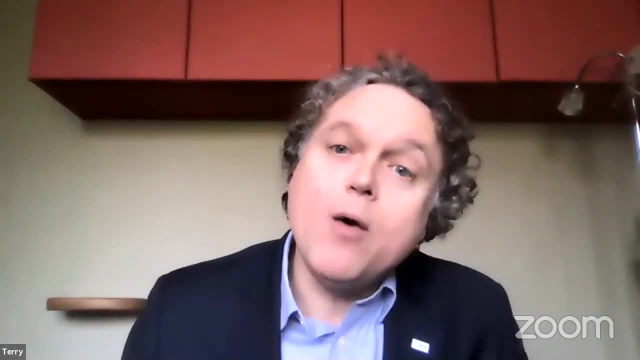 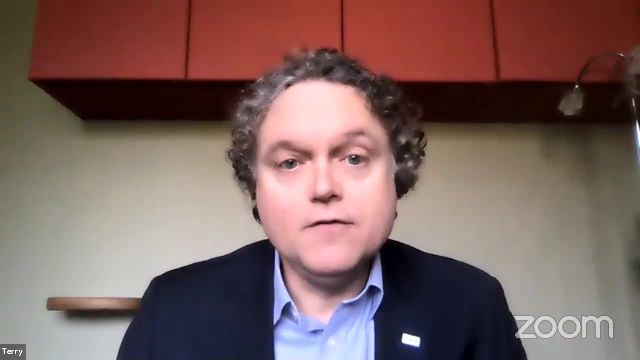 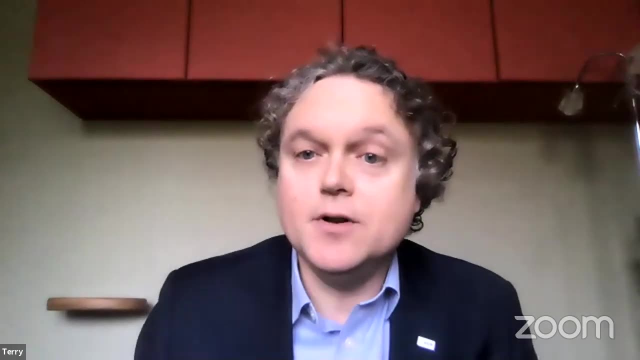 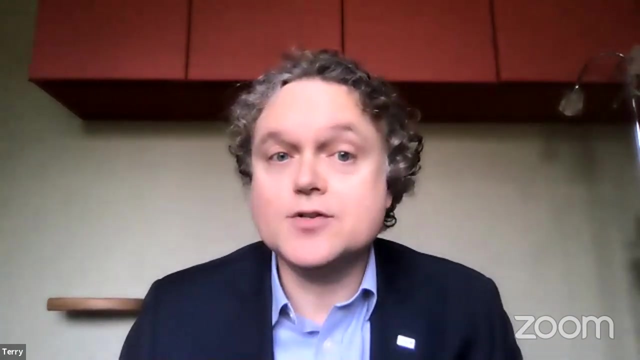 which will inform the UK government's third climate change risk assessment- so important. Following on from, Stephen Chris Stark, Chief Executive of the Climate Change Committee, is joining us to give his assessment on progress for preparing for climate change. We'll then be joined by Mike Keel from the Consumer Council for Water, to talk about why. 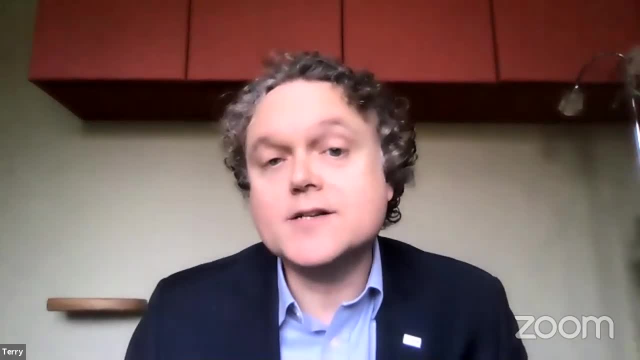 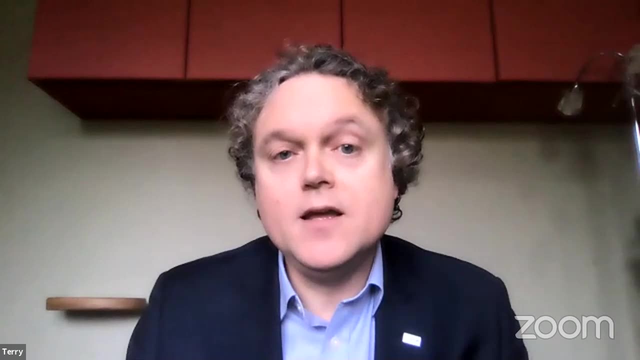 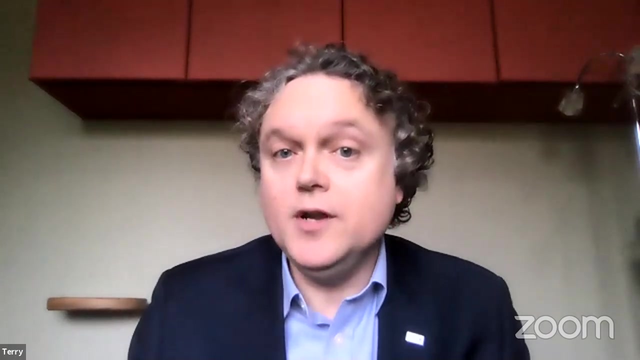 adaptation matters to consumers and how organisations can reassure their customers that they are preparing for the challenges of climate change. And to complete the first session, Francis Pimenta from DEFRA will join us to talk about how DEFRA will use the ARP submissions to progress adaptation and their ambitions for the next decade. 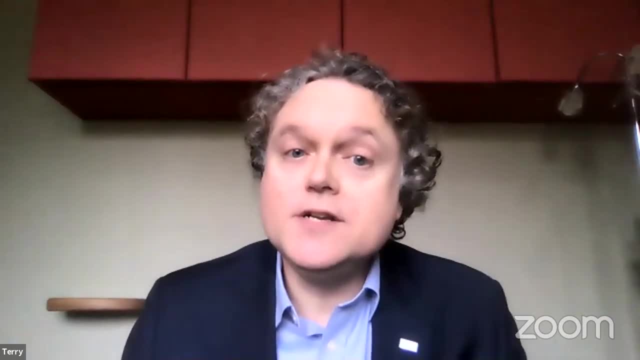 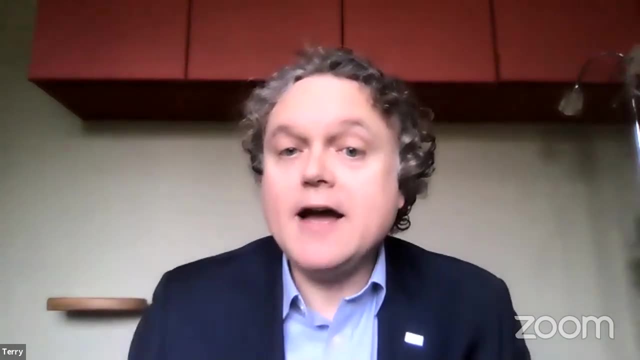 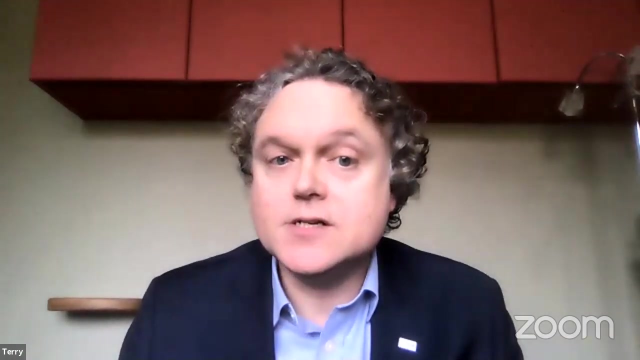 Now, after our first four speakers, we'll have an opportunity for you to ask some of them questions. After a short break, we'll then have six experienced reporters from a range of sectors giving their view on best practice for ARP submissions and how they use the process to mobilise change within their organisations. 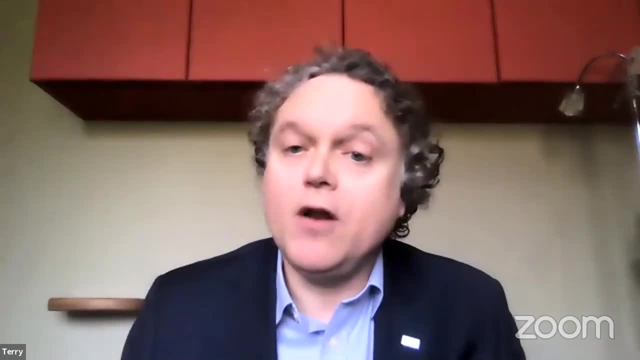 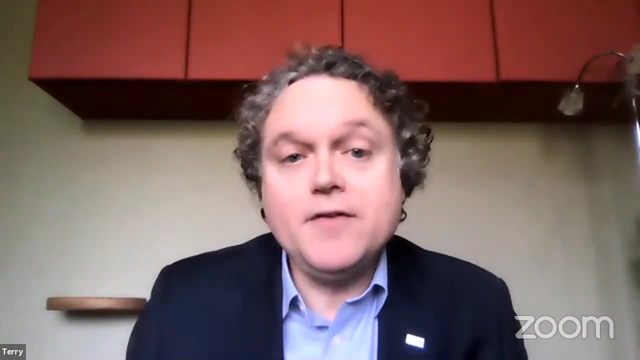 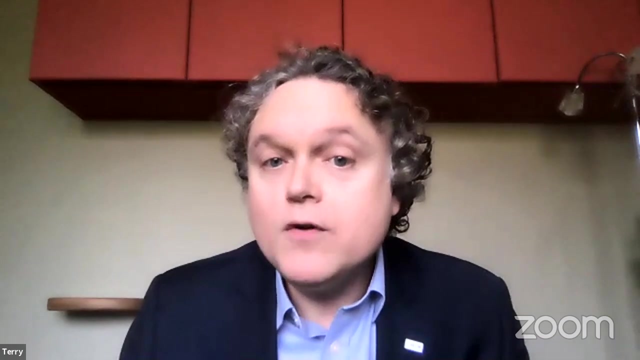 and progress adaptation, And this will be followed by a panel Q&A session. Now, before we launch into our talks this morning, a quick bit of housekeeping. We'll be splitting this two-hour session into two sessions. We'll hear from all of the 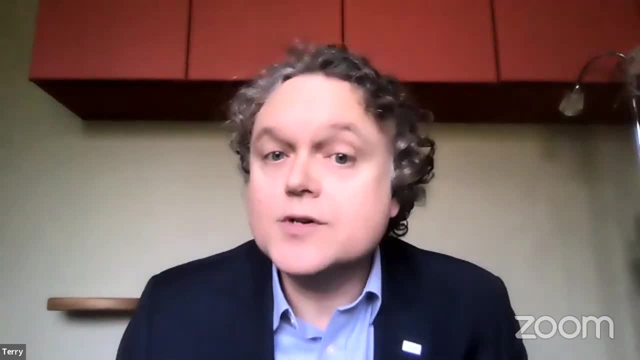 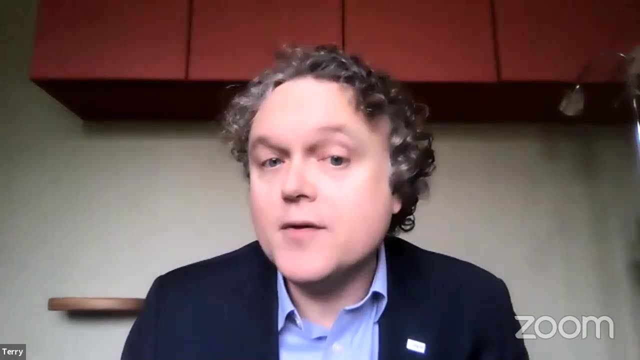 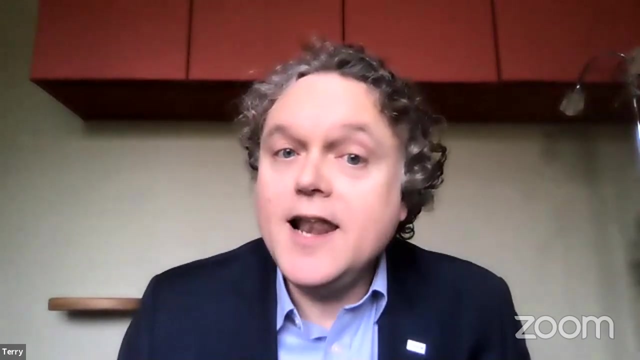 speakers in each session and at the end of each session, we'll take your questions. We want you to pose the questions to our speakers, as well as to see and comment on what other people are asking. Now, the best place for you to do this will be using the Slido You will notice on the left-hand. 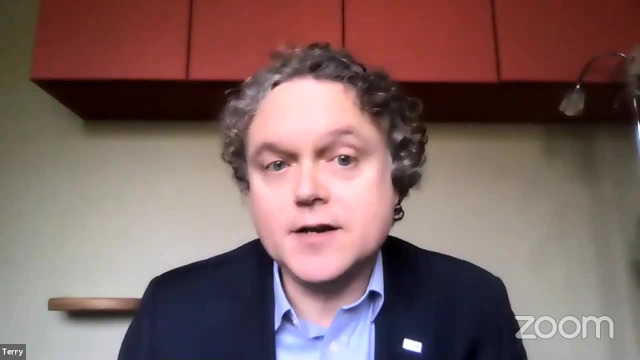 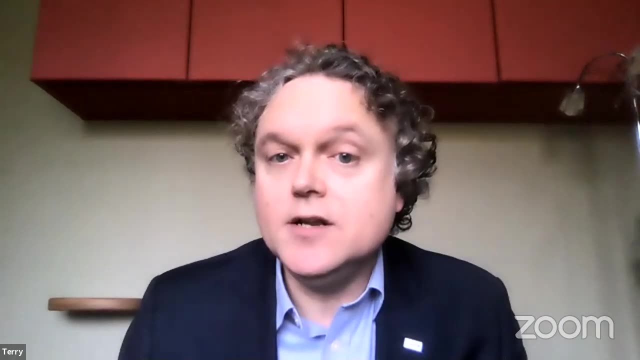 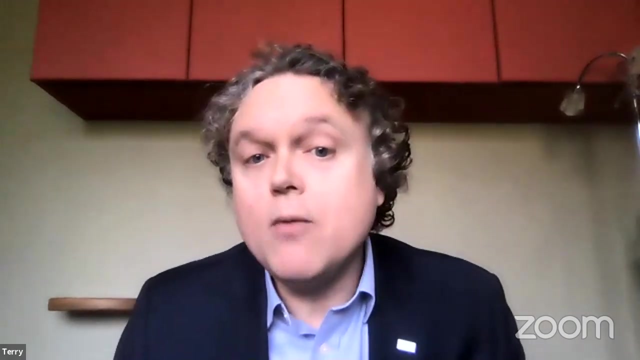 side of your screen, next to the chat, there is a tab for Slido. You can submit your question within the Q&A session at any time during the presentation and hit the thumbs up to get the questions submitted by others. You can also interact with each other and comment on any 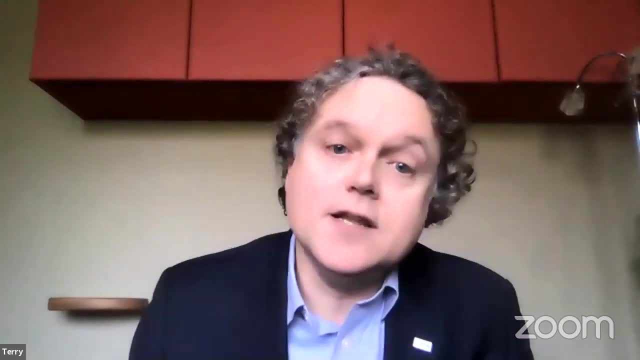 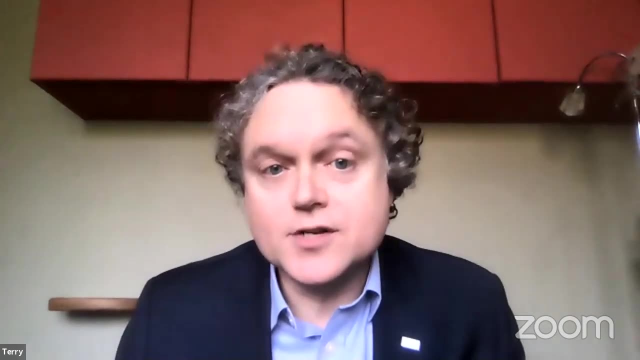 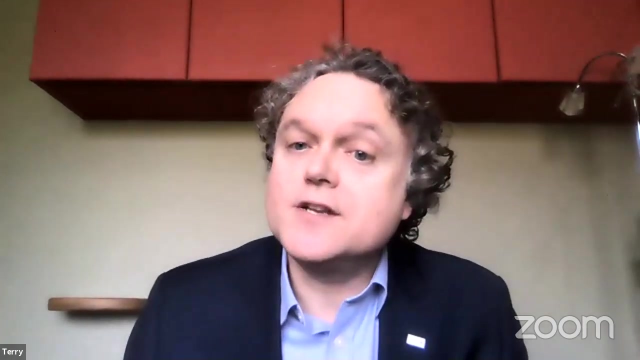 active questions in Slido by hitting reply underneath the question. Now we also have a short poll which is running on Slido too. A few questions which we hope you'll take a couple of minutes to answer. The poll will stay live during the event, but also for the rest of the day, if you. 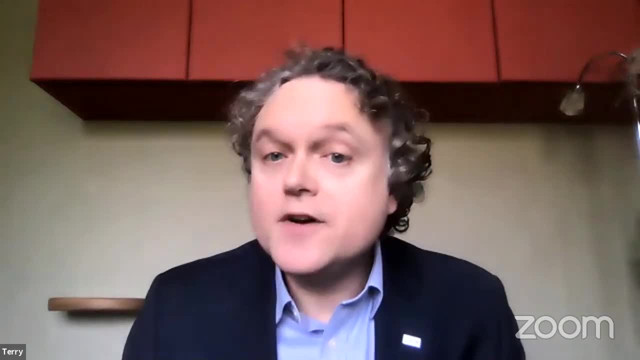 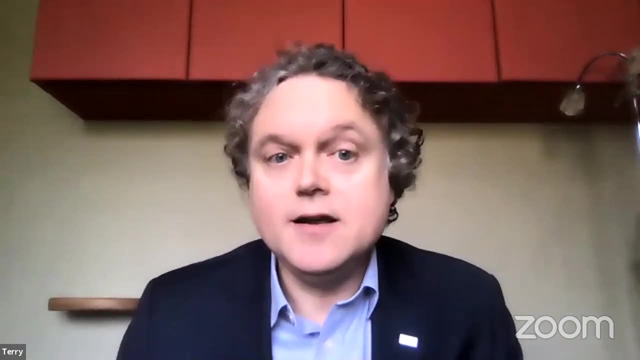 want to go in later. Now, after the first speakers are finished, at around half past 10,, we'll have a five-minute comfort break and return for the second session, and we'll wrap up at 11.30 sharp. After we conclude the webinar, we will invite you to visit our exhibitor. 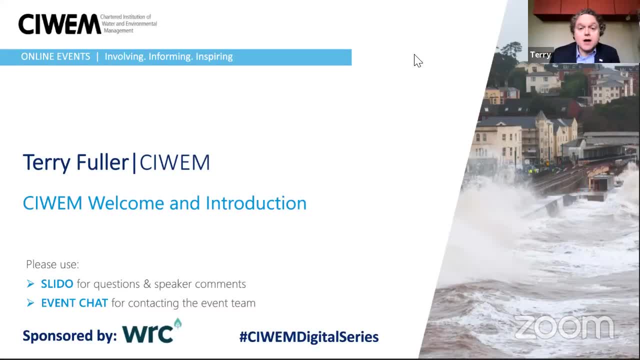 booths. CCW, WRC and our CyWEM membership and learning and development teams will also be ready and waiting to speak to you. There will also be a speed networking session open up so you can meet other attendees Without further ado. it's time to introduce you to our first speaker, Professor Stephen Belcher, As the 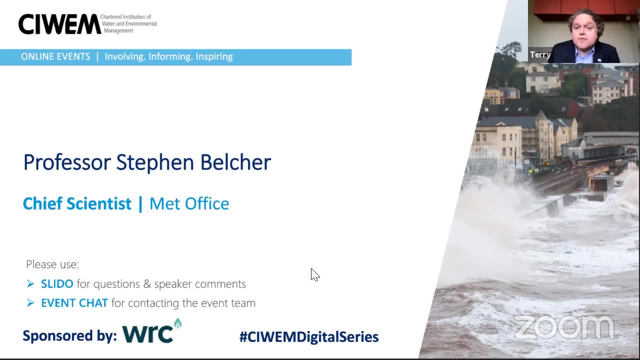 Met Office Chief Scientist and Technology Officer. Stephen provides leadership at Met Office Science and Technology, leading on the implementation of the research and innovation strategy. Stephen led the evolution of the Met Office Hadley Centre to focus on climate science and services. He was a 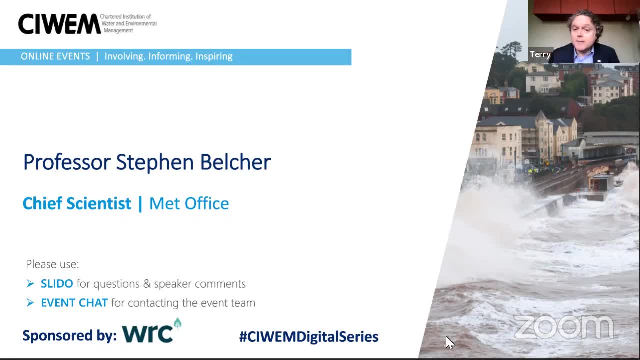 driving force behind the initiation of Newton Fund's Climate Science and Technology Centre. He was also the founder and founder of the Science for Service Partnership China, in which scientists from both China and the UK are now working together to develop fundamental climate science and climate services. Stephen, over to you. 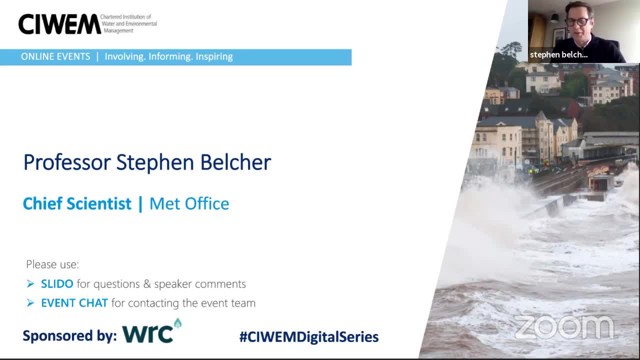 Well, brilliant. Thank you very much, Terry, for that wonderful introduction And it's a great pleasure to be able to speak to everyone this morning. As Terry described, what we've got in front of us is a real massive challenge here in adapting. 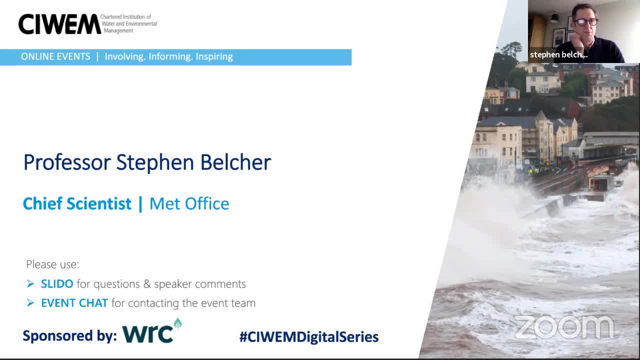 to climate change, And so the element of that puzzle that I'd like to present on this morning is really the hazard. so whatwhat will the weather throw at us in this changing climate? And clearly that'sthat's where the Met Office has some expertise to offer this complicated arena. So I can move my slides on. 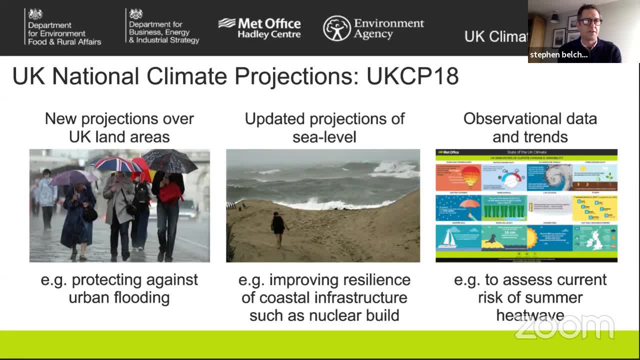 So I'd like to start just with a few slides to describe what we describe as what we call UKCP, so the UKCP, UKC, UKCP, UKC, UKC, UKCP, what we call UKCP, so the UK National Climate Projections, and the latest iteration of these. 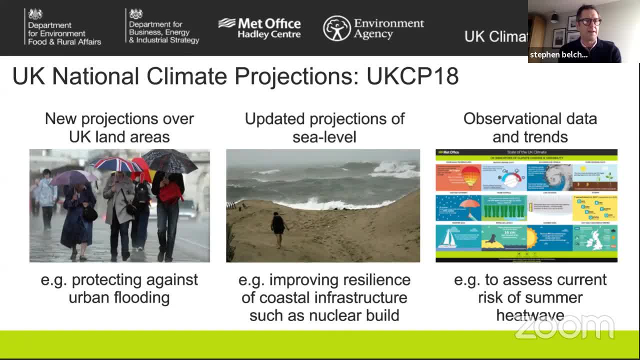 was launched in 2018.. It's a joint endeavour by DEFRA, BASE, Met Office and Environment Agency, and we had enormous user community engagement in designing this product, and what UKCP18 provides is a set of projections for over the UK for sea level and, of course, it includes observations of 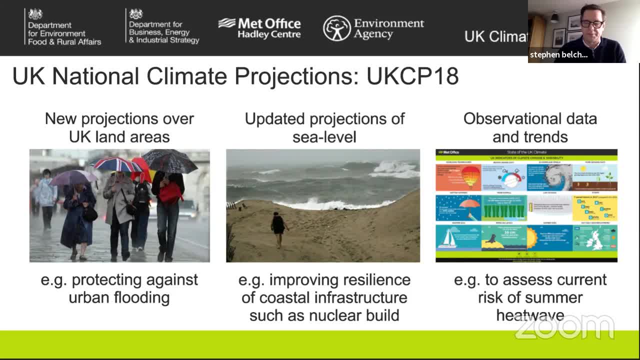 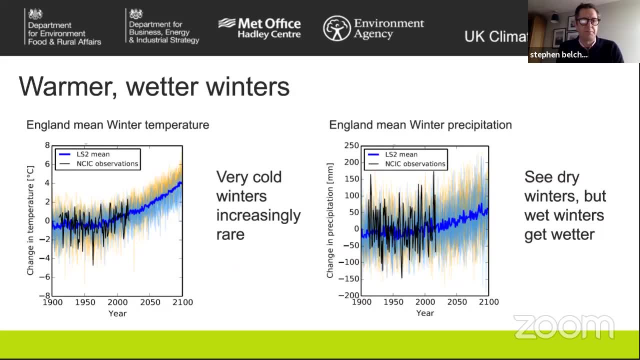 past and present climate to complement the future projections. The main messages from these projections remain unchanged from previous iterations, namely winters will become warmer and wetter. You've probably heard that message before, but really the innovation in UKCP18 remains unchanged from previous iterations, namely winters will become warmer and wetter. 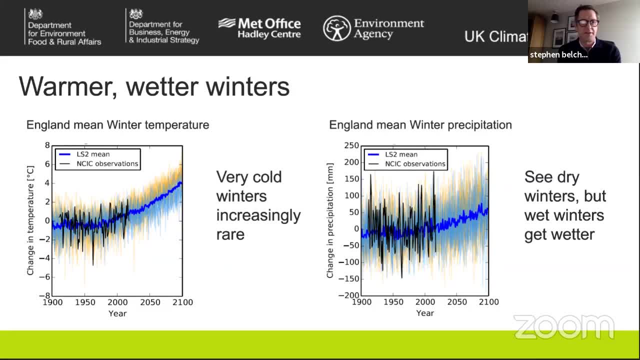 is that we're able to describe the weather conditions that sit under that broad changing climate. So we've got two charts here. on the left hand side is temperature in the winter over England and on the right hand side is rainfall or precipitation in England during winters and the. 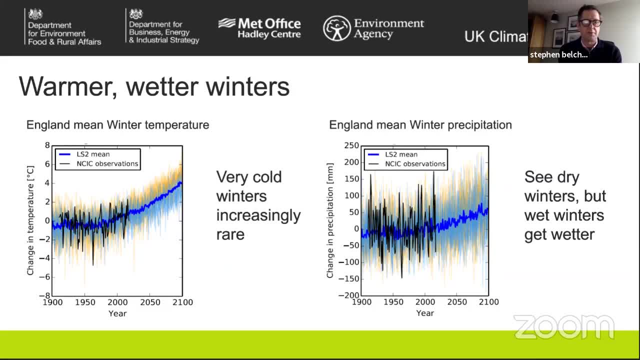 vertical axes. on each of these are the change in either temperature or precipitation, and then along the x-axis, horizontally, we've got the year from 1900 through to present day and then out into 2100.. In each case, the black lines show observations of what has actually happened, and then the blue line 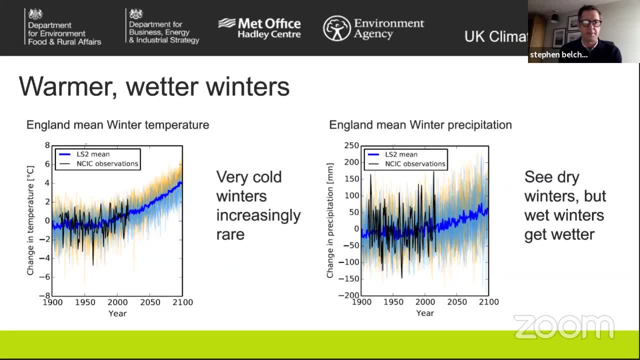 is the average of the change under our changing climate for temperature and rainfall and, as I said, the blue line here is really average, is it? and that's what we used to talk about in climate change? but I think you can see on those charts some faint blue lines and faint orange lines. so 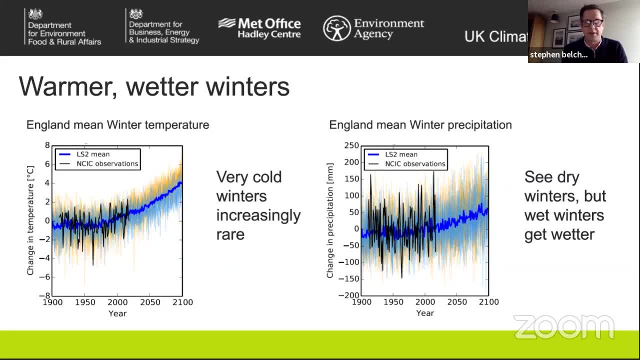 those are the actual conditions in year of the weather conditions provided by UKCP. so we're not forecasting when these weather conditions we're having. we're saying what's the character of the weather conditions that we'll see in these future climate. and the contrast I wanted to draw between these two charts is: on the left hand side you can see temperature. 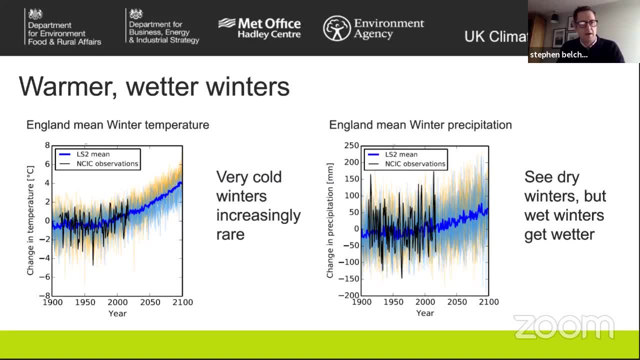 and temperature is increasing as a band, showing these warmer, warmer winters. but you can see the range of temperatures is broadly constant through that that period, so staying about the same as the range of temperatures we experience In present day climate. if we contrast that to the right hand side, I think what you can see is that 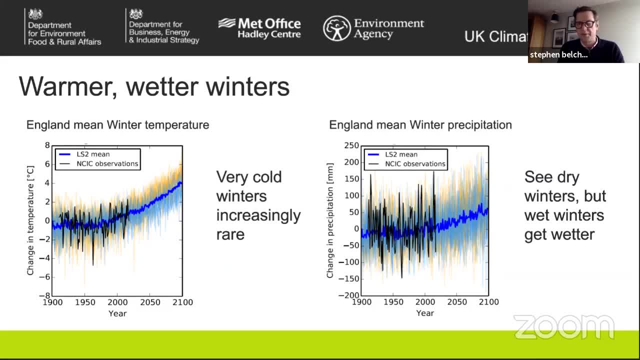 we're still living with the dry winters, so the lower values of the rainfall that we're seeing in the future. so, whilst the average is increasing, the dry winters remain dry. but you can see from the upper fan of those pale blue and pink lines that the wet winters get wetter. so we're seeing 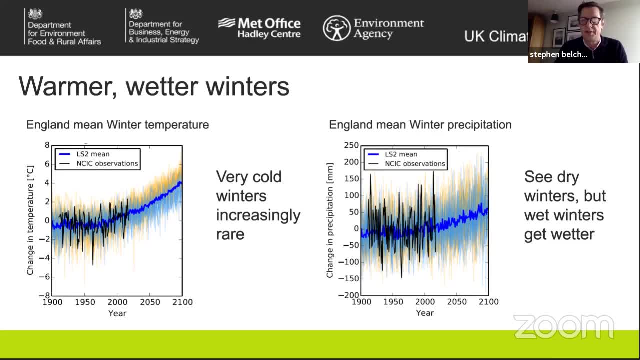 an expansion in the range of conditions that we'll need to adapt to. So so that's one of my key messages: yes, we need to adapt to warmer, wetter winters, but in some of the variables- rainfall in this example- we need to adapt to a wider range of conditions. 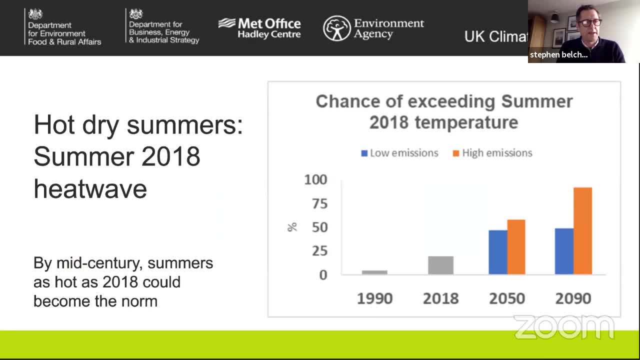 If we turn very briefly to summer now, you'll have heard again the message: hot, dry summers under a changing climate. here's the example of the summer 2018 heat wave, which happened immediately prior actually to us launching UKCP18, and the chart here gives a gives a kind. 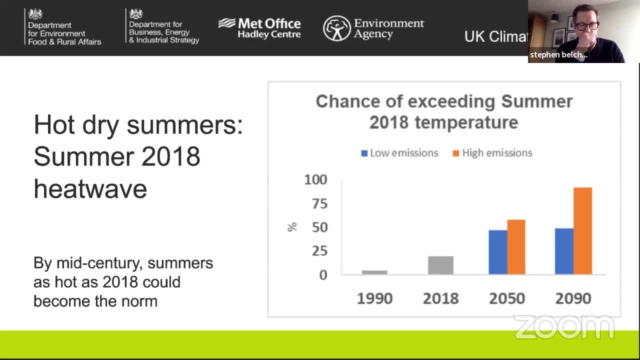 of indication of how those conditions have changed over time. So if we go back to 1990, this was really quite a rare event. 2018 it's more like a one in five event and by 2050 this is looking like a normal summer. so a 50: 50 chance of those events and then 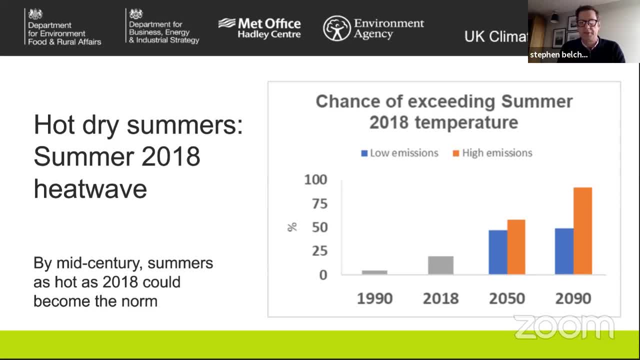 by 2090 we begin to see a much more differentiated occurrence, depending on what we do to mitigate climate. so what do we do to emissions, And I think Chris Stark may pick up on this in his presentation later. under low emissions it will remain a 50: 50 event, but under high emissions you can see it's almost becoming. every summer looks like that. 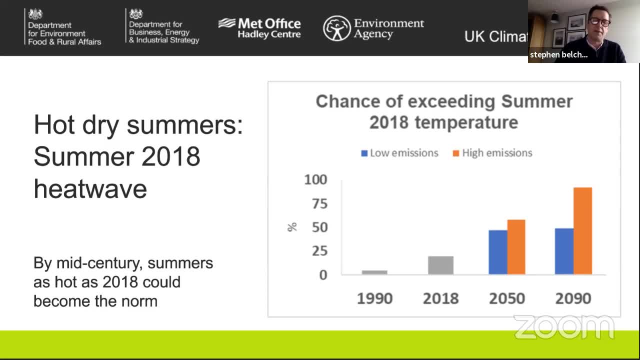 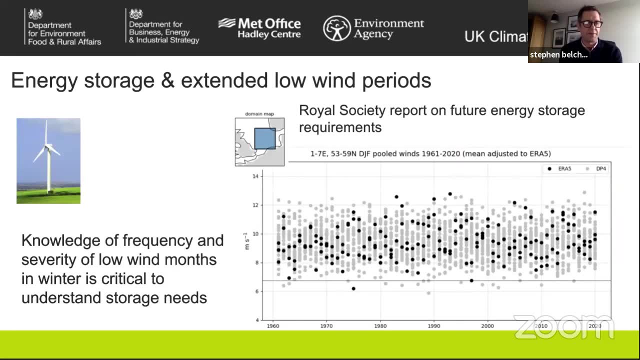 So we're beginning to see the effects of what we do now on the conditions we may have to adapt to towards the end of century. Very briefly, just to end this brief introduction to the weather conditions under a changing climate. I wanted to just give sightings. 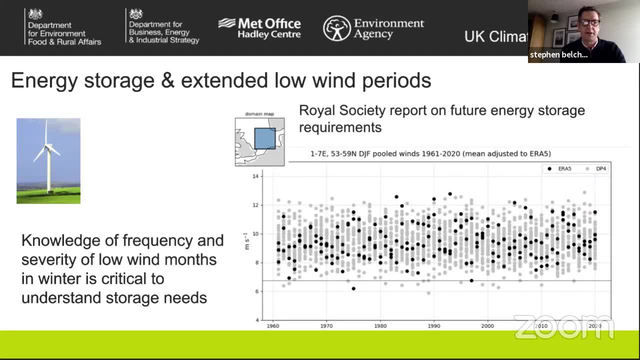 of a new product that we're able to offer at the Met Office, which is looking at present day conditions. so we know climate has changed, And so the question is: what could present conditions, present climate, throw at us and, in particular, could it throw us? throw at us, what's the chances of present climate throwing us conditions that we've never seen before? 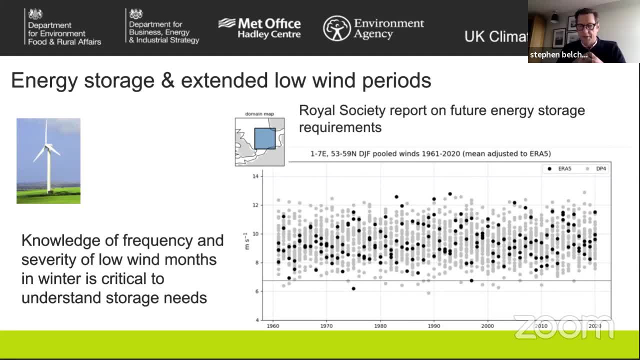 In order to help us with that. we've got observations of past climate, but that's relatively short, particularly because the climate has changed. We've got observations of past climate, but that's relatively short, particularly because the climate has changed. We've got observations of past climate, but that's relatively short, particularly because the climate is changing, of course. So what we do is we complement. 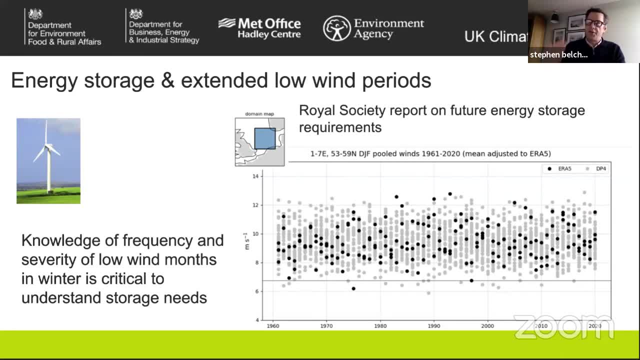 The observations of recent climate with synthetic present-day climate from our model simulations. what you're seeing here is some work we submitted to a Rorsa society report on future of energy storage, And what we're looking at is wind generation of energy over the North Sea. so the little instead there. 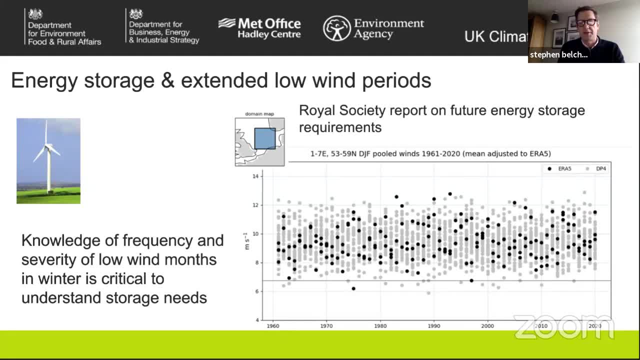 shows you the box we're looking at in the North Sea And we're looking at a um December, January, February wind conditions over that area and you can see on the chart. we're looking at conditions from about 1960 to uh present day and we're asking the question: what's? 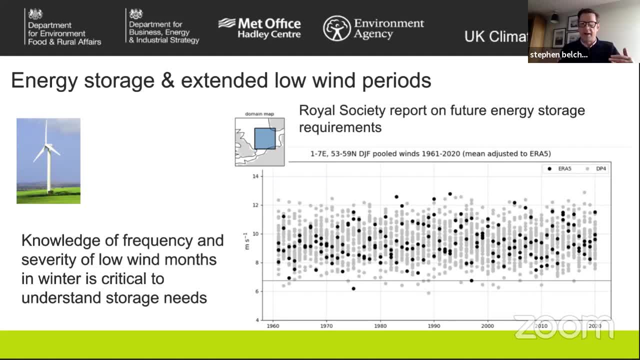 the chance of getting very low wind conditions in that winter period under present climate. you can see there's a dark black dot, which I hope my pointer is able is illustrating here, which is the lowest on record. and using this combination of observations plus model, we're able to say: 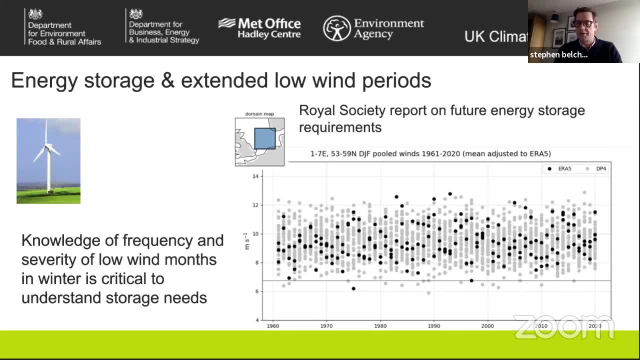 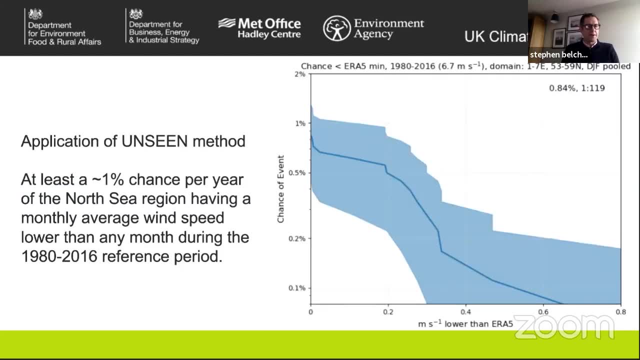 what's the chance in the future of seeing a very low wind condition, which of course would limit the renewable supply that we might be able to provide? putting all of that together, we're seeing that there's a one percent chance in every year that the North Sea region might have a monthly 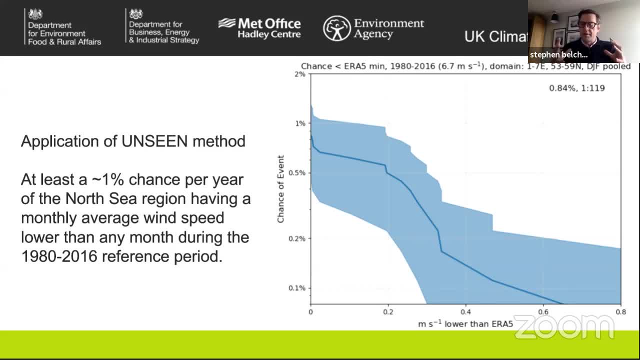 average wind speed that's lower than anything we've seen. so really, what we're trying to get out of here is that we're seeing a very low wind speed, and we're seeing a very low wind speed here is under present day climate. there are risks that we need to adapt to that we may not have seen. 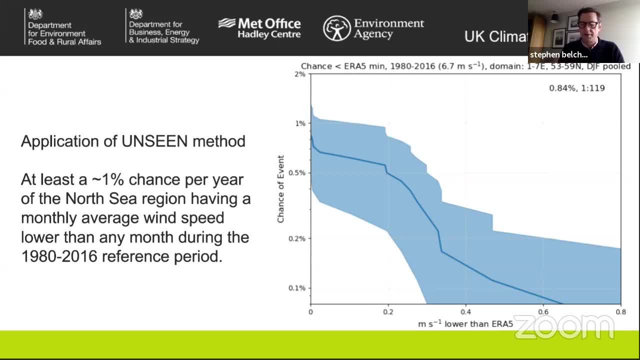 before. I've given the example of low wind speed. we can do a similar analysis. we call it the unseen method. there's a glorified acronym that sits underneath that, but it's unseen conditions. we can apply it to rainfall, uh, temperature, and you're seeing it here for wind, so I can see. 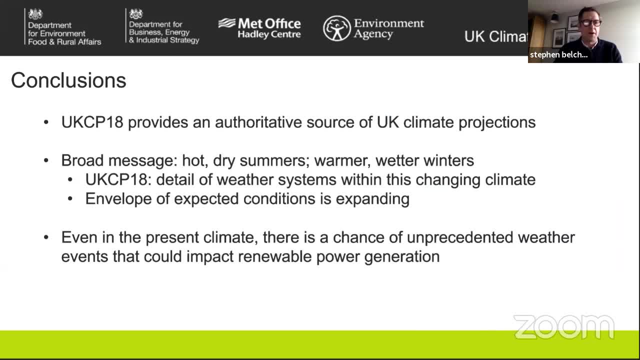 Terry back on screen. so that's my prompt just to wrap up. so my final slide- um, perhaps I can leave you with- is that the UKCP provides a consistent source of um information on weather conditions under the future climate. that might help folk provide adaptation planning. the broad 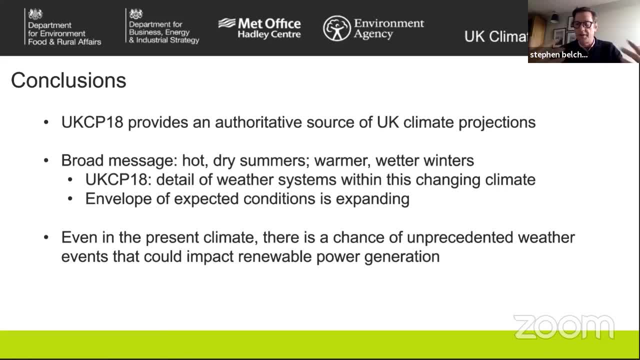 message is a hot, dry summer, warmer, wetter winters, but what UKCP provides is a lot more detail under that, and the envelope of conditions we will need to adapt to, we think, is expanding. and then, finally, even under present climate, there are things out there that nature hasn't yet thrown us, which we think it could well do, so we need to. 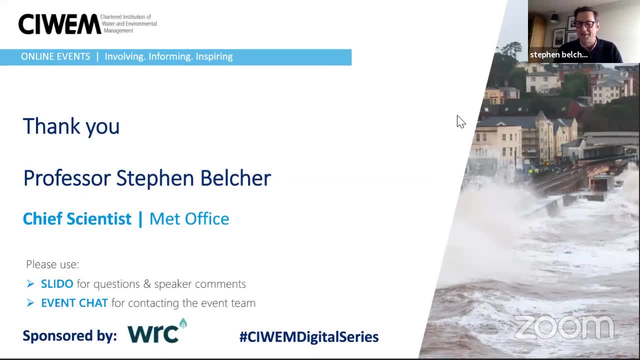 just be prepared for those as well. with that, I'll say thank you to Terry and the team for organizing this and thank you for your attention. Stephen, thank you very much. that. that was tremendous and really has set the scene very nicely in the imperatives that we face. thank, 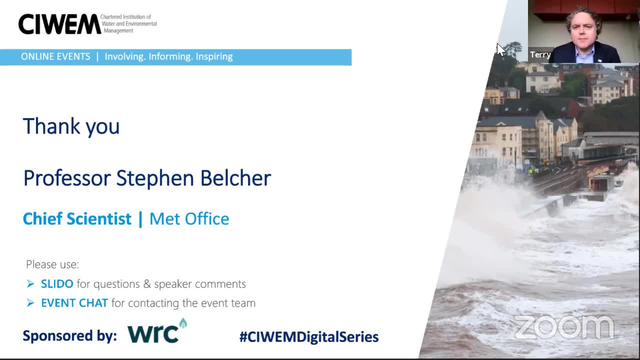 thank you. um, I can see that some questions are starting to come through, but please do use the slido to submit your questions and also to promote up and down those that uh that you would really like to be asked. okay, it's now time to move on to our next uh speaker, uh, Chris Stark, who is chief executive. 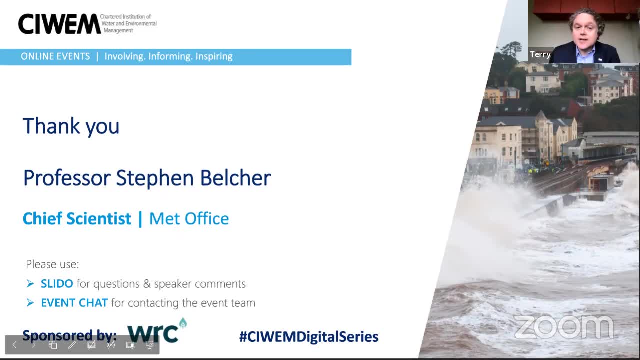 of the climate change committee, which is the UK's statutory advisor on tackling climate change. Chris led the committee's work in 2019 to recommend a new net zero target for the UK, which is now brought into law. he speaks regularly on the transition to a net zero economy. Chris, over to you. 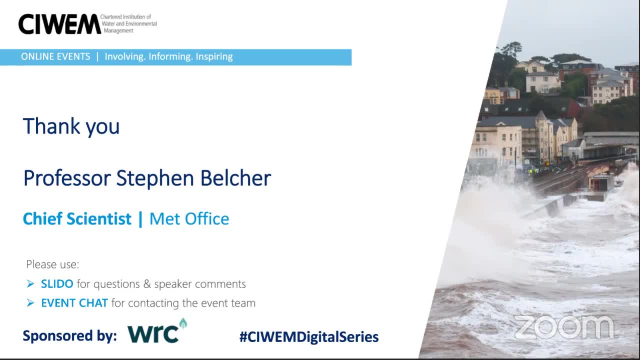 hi, Terry, and the first gremlin is that I can actually show my video, so I'm going to try and work out how to do that, Terry, while I, while I filibuster for a second. so, um, I don't know if the tech support can help me with that, but the, the uh, the uh, the option to do. 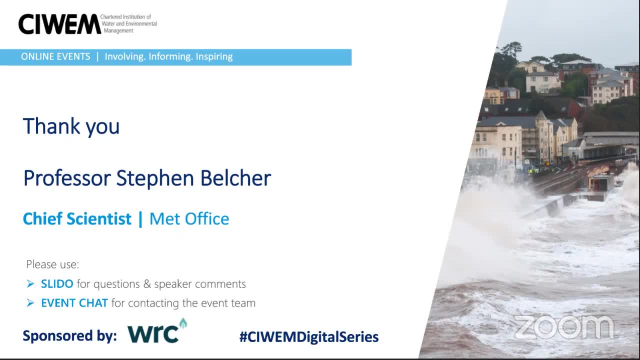 it has disappeared from my screen. why don't I do it without video? and then you can hear me as a ghostly voice, because I can certainly- um, I can certainly do so. so as long as you can hear me, I think that's fine. but there's a question that's coming in from the audience. 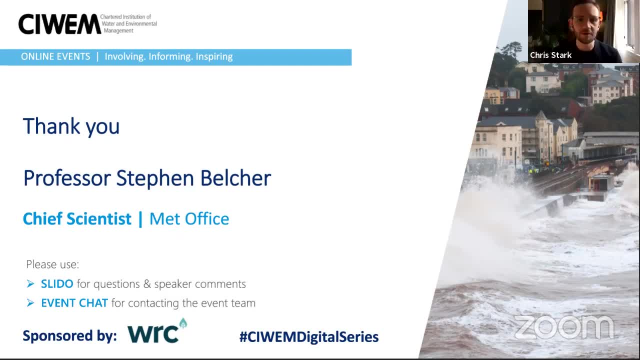 fine, um, uh, well, here we are. i've been offered the chance to start my video. that's wonderful, great. can you see me, terry? uh, yes, see you and hear you as well. lovely, great. well, look, i only have eight minutes, so i'm gonna. i'm gonna keep this uh nice and and punchy, if i can, and um, uh, 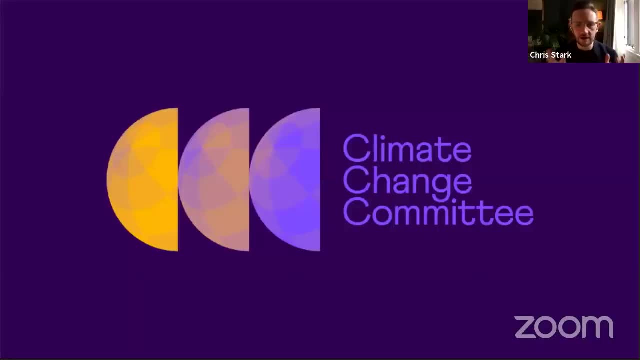 let me just start by saying that, uh, we're talking about adaptation reporting this morning, and it is absolutely a key component of the uk's armory when it comes to tackling climate change, but it is, frankly, an area, uh, where we could do better. so that's what i'm going to talk about in the next. 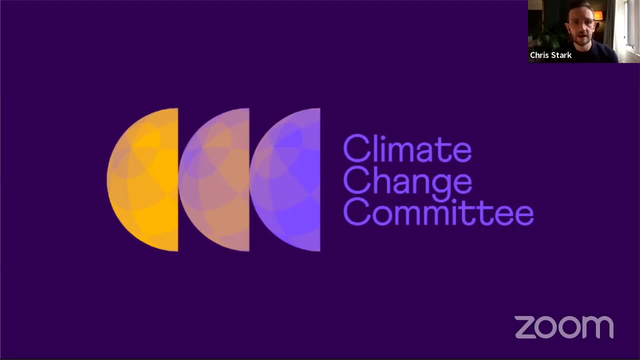 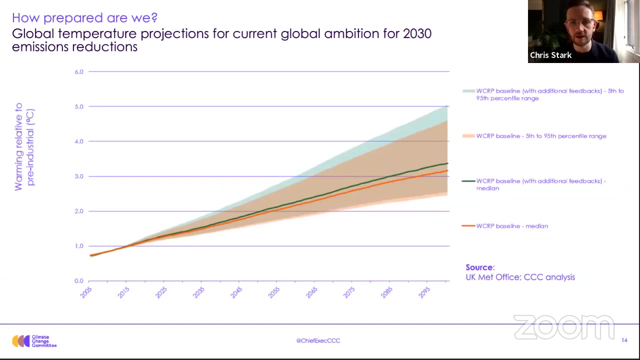 seven minutes or so, and i'm going to pick up where stephen belcher left off with some of the advice that we presented in december in our sixth carbon budget: advice about the global commitments to cut emissions and their implications, and, um, this is a chart that we that we published. uh, just a few. 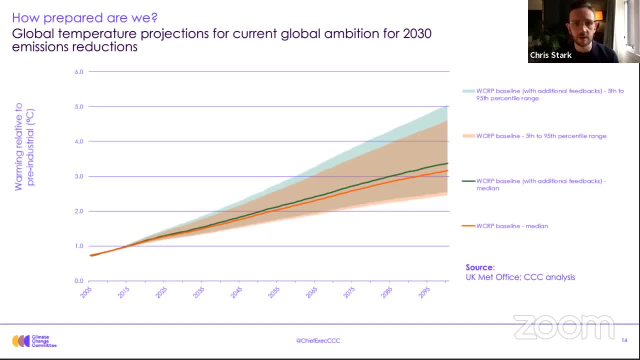 minutes ago. so this this is looking at the implication of the current uh emissions targets for 2030. so we look at the ndcs, as they're known, the national commitments for cutting greenhouse gas emissions. this is the projection for temperature. uh, that is the that is implied by. 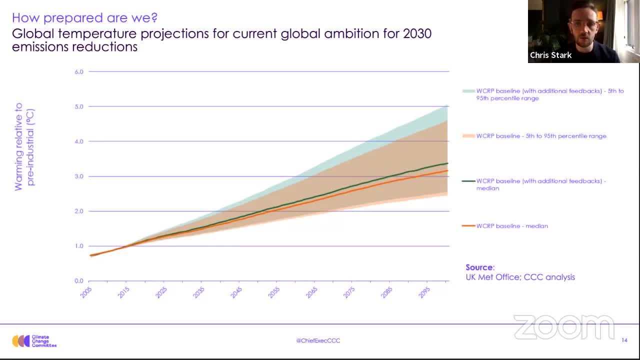 those commitments. now it is. it is taking us to uh warming by the end of the century of between three and four degrees centigrade, and uh, that is pretty disturbing uh, now it's worth saying that that has come down over recent years, because that's testament to what's been happening with 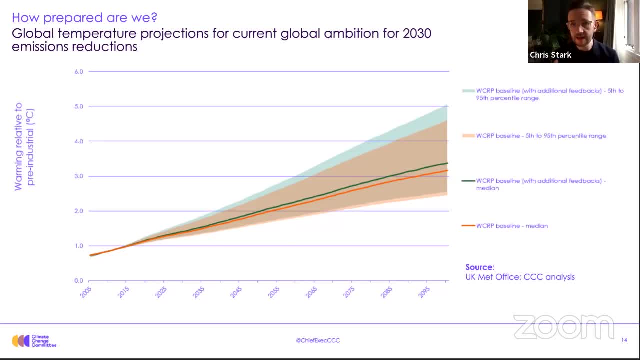 climate commitments and climate policy. but the mistake here is in thinking that we're going to wish all this away by focusing on net zero. now we're going to hear a lot about net zero this year in the run-up to the cop, but this is the implication of where we are at present from. 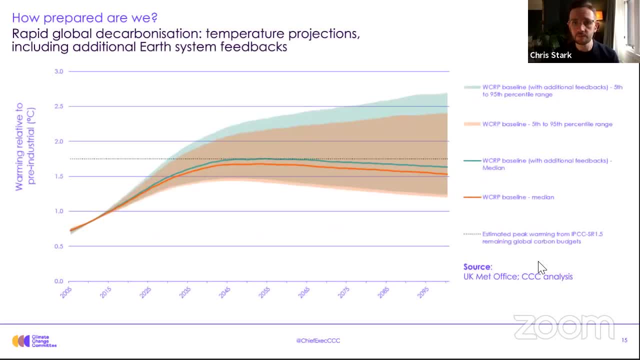 those ndcs. and if i just roll on to the next chart, this is a nice chart that shows you what we will get if the world shifts- as i desperately hope it will- to that rapid decarbonization scenario that's going to be changed by the paris agreement. this is the implication of net zero by mid-century, for 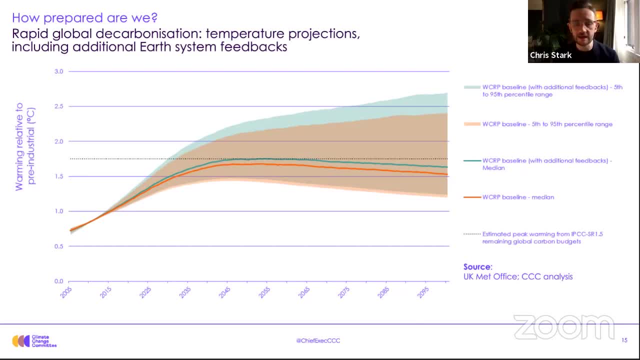 the developed economies, 2070 for the world as a whole, and you can see that that is a quite a significant change from the chart i just showed you. it takes us to much lower levels of warming. so, uh, you know, less than two is the goal that we're looking for here, but, crucially, we are still going. 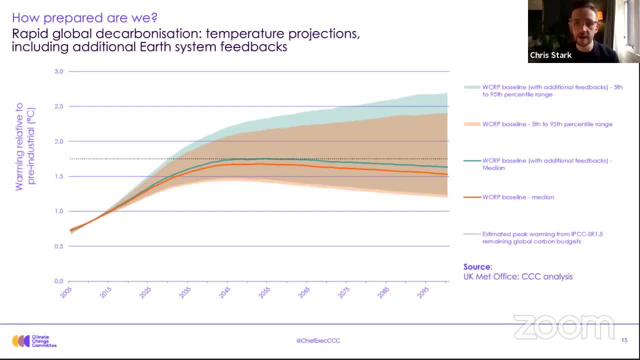 to need to adapt to temperature change and the climate changes that come with that. and there are still, even in this uh on this rapid decarbonization scenario, there are still high warming scenarios that will bring big challenges. so the big message to start with is that net zero is not the free. 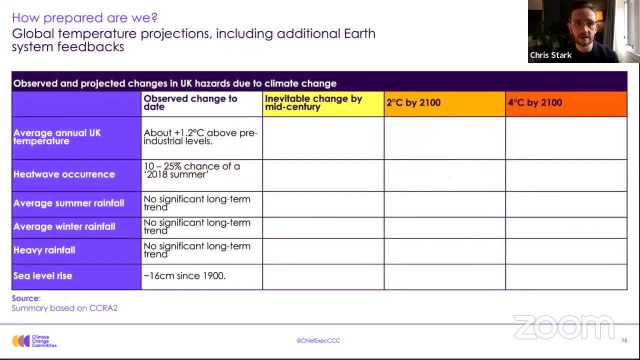 pass that sometimes i think it is presented at. so if we just move on then to to just to pick up actually many of the things that stephen talked about, this is another take on the evidence of the possible impacts for the uk across different mitigation pathways. um that we have. this is 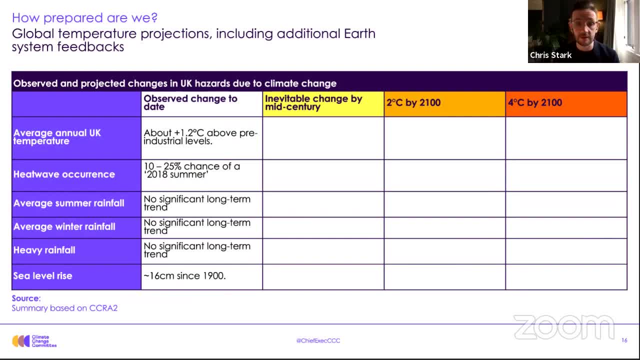 based on the work that we did for the second climate change risk assessment. we're updating this for the third climate change risk assessment, which we'll be publishing in july, so let's just take a moment to reflect on this. the first column here is the climate change risk assessment, which is: 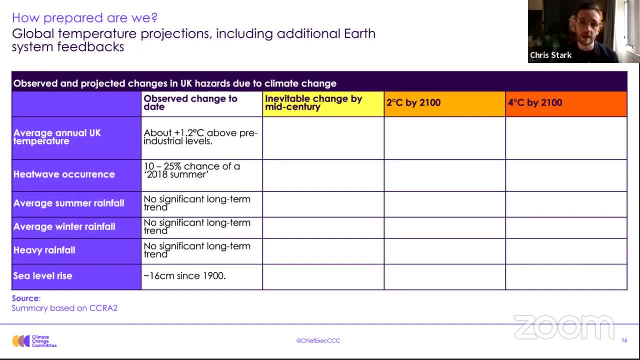 based on the work that we've done for global climate change risk assessment, where the heat wave every year, 10 less rainfall in the summer, 10 increase in heavy rainfall, higher seas- this is the inevitable change that is definitely coming, so already we can start to ponder whether 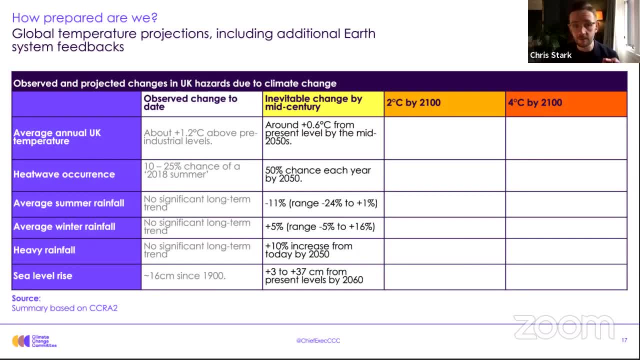 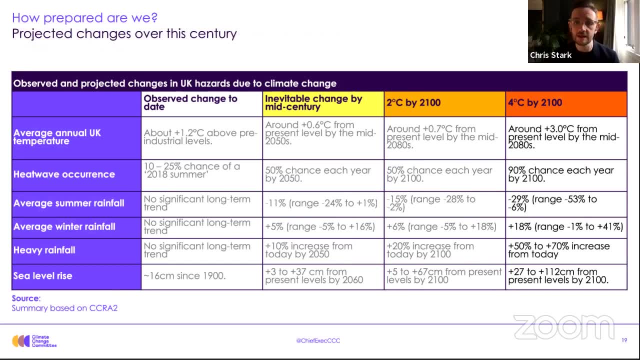 we're really ready for that kind of change by 2050, but we should also be prudent, so we've got to look beyond that. so, looking at a two degree world: um, two degree world is not one we want to be in. we're going to have more warming, even less water availability in the summer: 20 increase in. 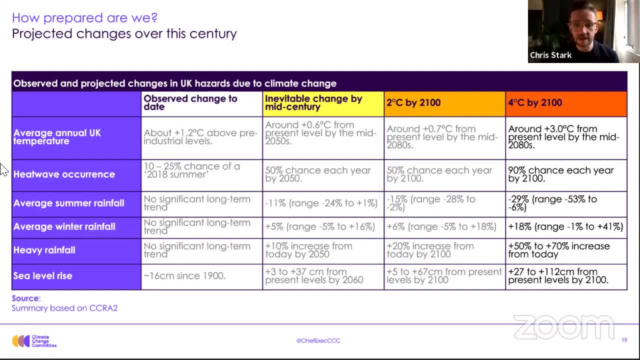 heavy rainfall, strikingly higher seas, and then four degrees is, i'm afraid, a world that we also have to consider. just look at the four degree impacts that i've got on this table here for you. so three degrees centigrade of warming from where we are today. 2018 heat waves almost every year. 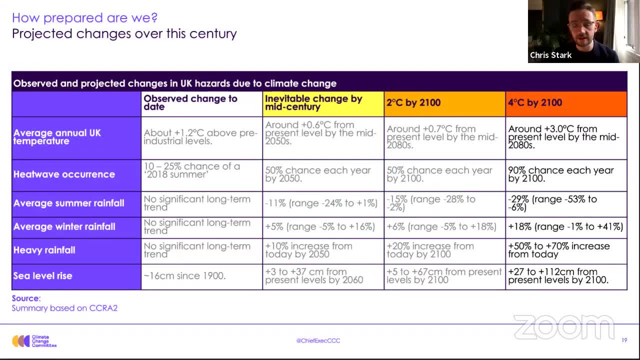 shocking fall in summer rainfall, similarly shocking increase in damaging heavy rainstorms and over a meter of sea level rise potentially. now this is a very plausible outcome, and that's not, of course, what we wish to see, but it's the kind of outcome in infrastructure terms that 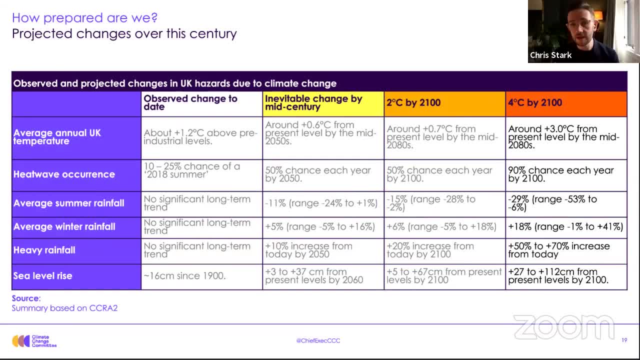 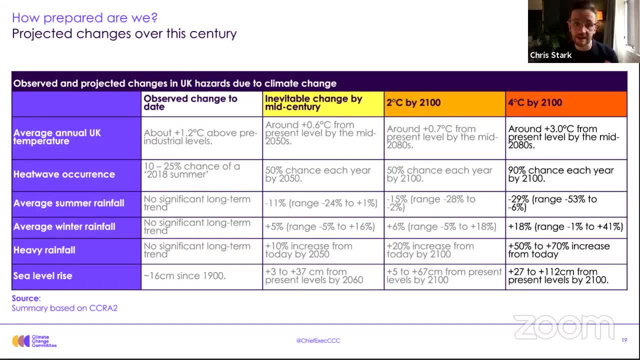 centigrade, the kind of planning assumption that is mostly considered when this is actually at the optimistic end of the spectrum. surely, given the year that we've just had, it's time to get real about what lies ahead. so let's talk about that now and move on to the uh, the governance. 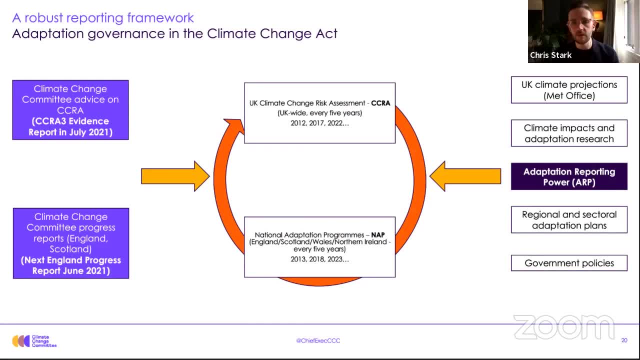 framework for adaptation. now a few words for me on this. when the climate change act was conceived, there was a great deal of good foresight in the way that it was drafted, particularly about the institutional arrangements and the reporting framework for emissions reduction and also for adaptation. but- and i don't say this lightly- it is simply not delivering the same kind of outcomes. 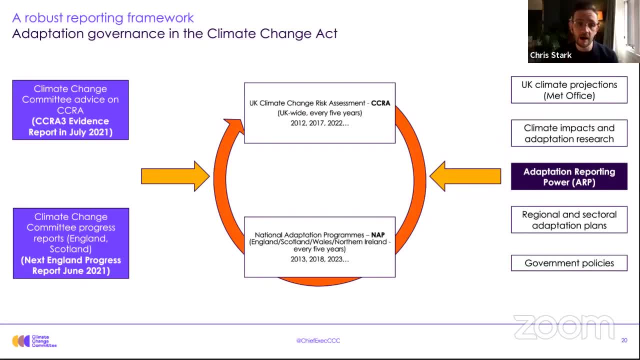 on adaptation as it as it is on mitigation. i think there are genuine weaknesses in the way that the governance works in the uk, and it largely revolves around the same sort of topics: the lack of mandatory requirements to act, the looser arrangements that there are for independent 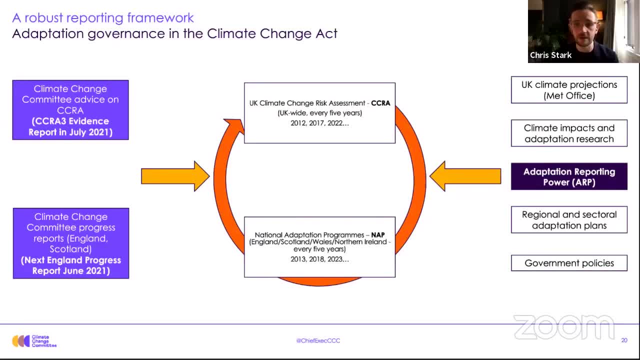 scrutiny for adaptation versus mitigation. also, of course, the unattractive politics of acting on adaptation. we are into our third cycle now of uh, of climate change risk assessments, uh and the sixth cycle of the uk climate change projections. that that is. that is a great process. it's not yet. 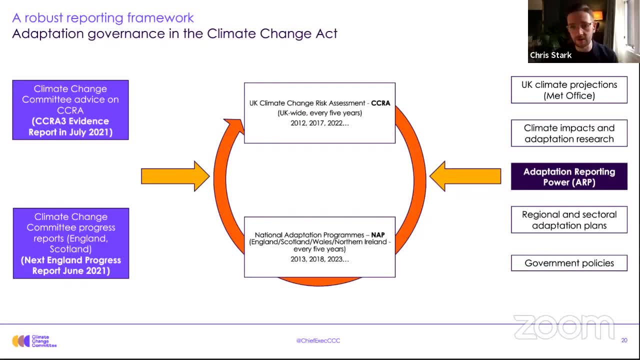 delivering the kind of outcomes that we need to see. crucially, the uk is not prepared for that two degree world, let alone the four degree world. so when we've looked at that, we've seen lots of sectors that have good adaptation plans in place but no sector at all yet showing good progress. 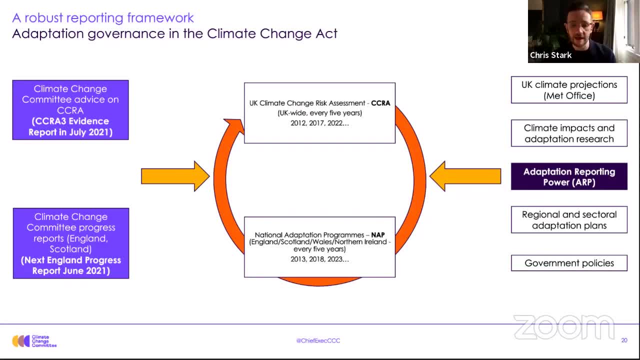 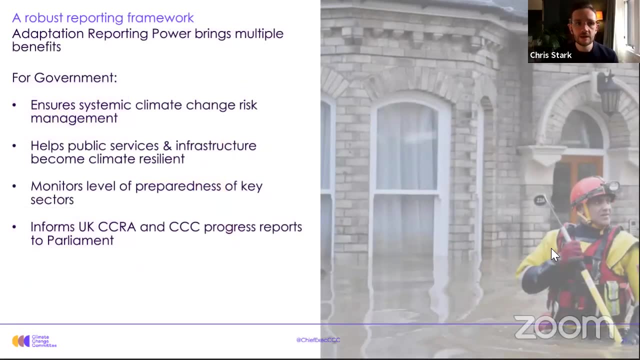 in actually reducing those risks. so this is the year to change all of that and i think the adaptation reported power is absolutely central to improving that overall outcome. so just in this final section, uh, just a few takes on that before we go into the next section and, um, yeah, just a few things to say more on on the adaptation reporting and why i think it is. 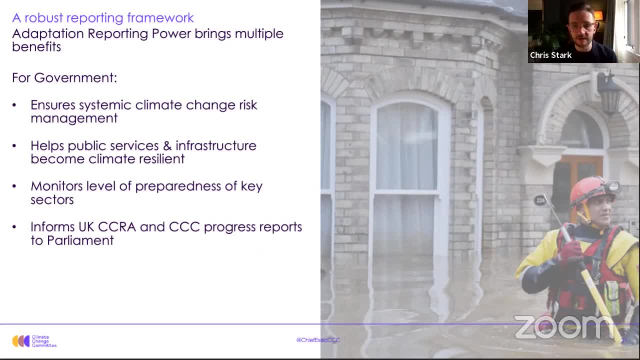 important. well, it's very obviously a huge benefit to the government because of the and, by extension, citizens in this country, because we're helping to build and ensure much more systematic climate change risk management, building better assurance that public services, uh, and our infrastructure in this country is. 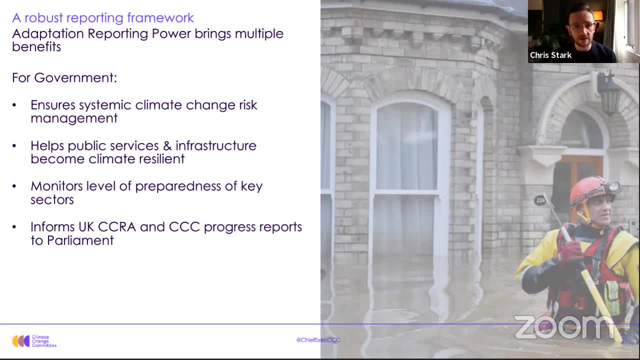 genuinely resilient to climate change and we're going to have better information on the level of preparedness in the key sectors, not the hot spots that we have now. and, of course, we're helping to make adaptation assessment and that governance under the climate change act better. we, we and 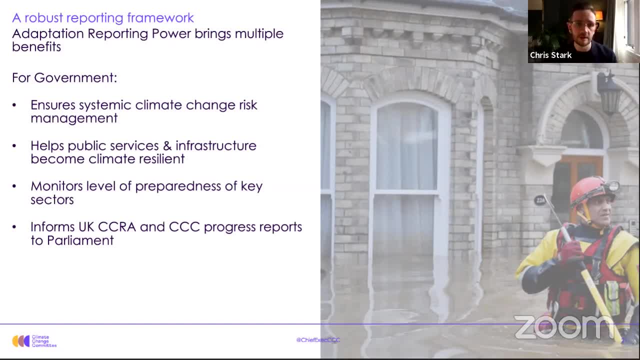 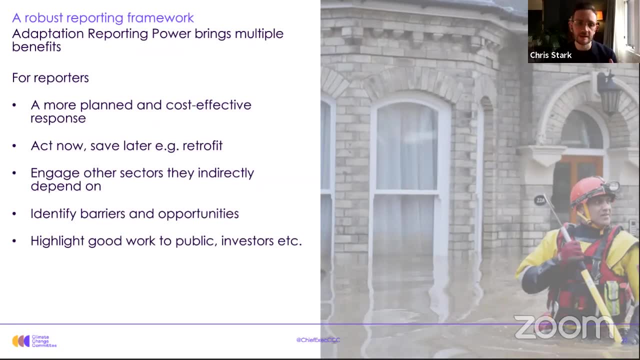 the ccc are going to be able to do better scrutiny, with better information from the reporting. that we'll get from this- and for reporters themselves, probably more important- is, of course, a way to demonstrate climate leadership. so if you are a reporting organization, this is a great way to do it, but, more important than that, it's going to help to systematize the 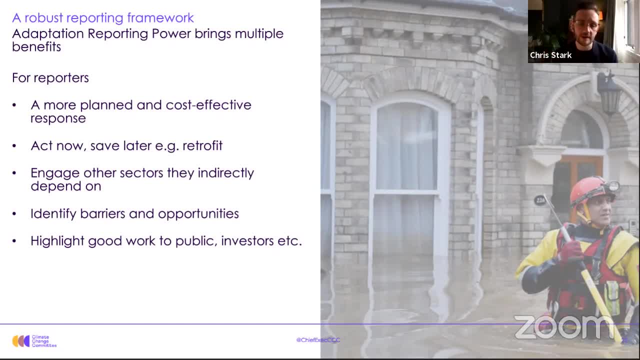 the identification of the climate risks and a proper assessment of how they're being managed. now, we don't see that at the moment. it's going to reduce our organization's vulnerability to climate change. that's an obvious thing to say. but with it there will be cost reduction, so we're 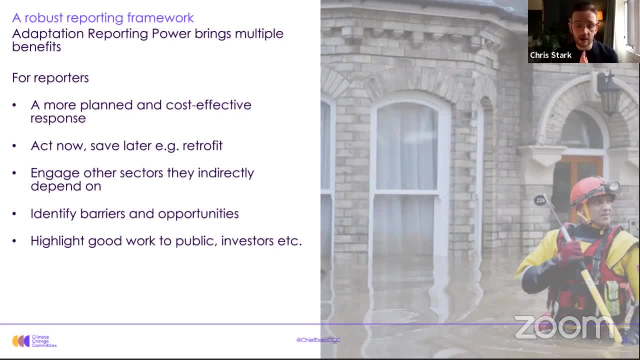 reducing the cost of inaction. later we're going to encourage by doing this a broader engagement with other sectors and that's going to help identify where there are those interdependencies that often are the biggest riskier overall- the cascading risks as i sometimes refer to- and it presents clear as day where the big barriers lie. 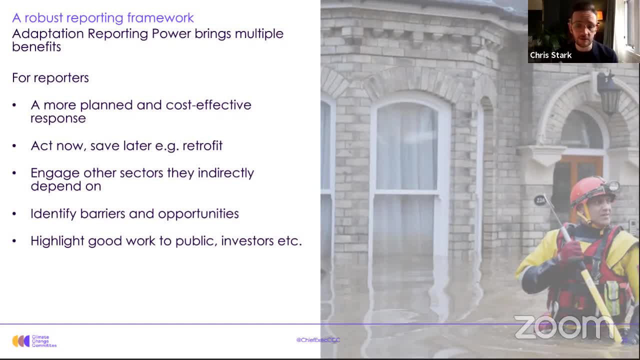 in responding to climate change also some of the opportunities that come from climate change. it's okay to talk about that and, of course, it provides a much more transparent platform for others to learn from. so that's the kind of key point when it comes to reporting organizations. 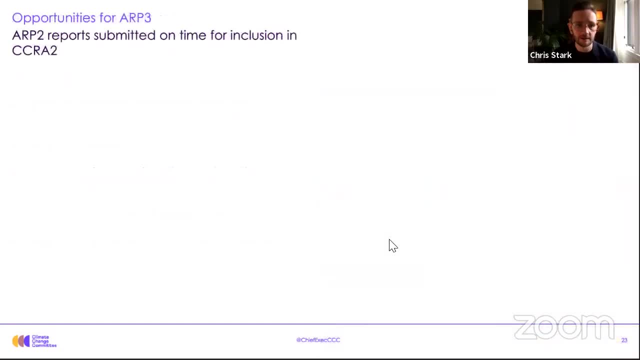 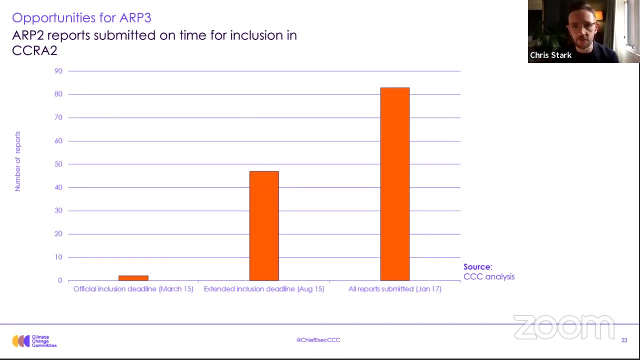 and just a final point from me, terry, before i hand back to you. um, this is a nice chart that just shows you, uh, where we got to with the 84 reports that were submitted in the last round of adaptation reporting, and this is broadly what we found. firstly, look at the poor. 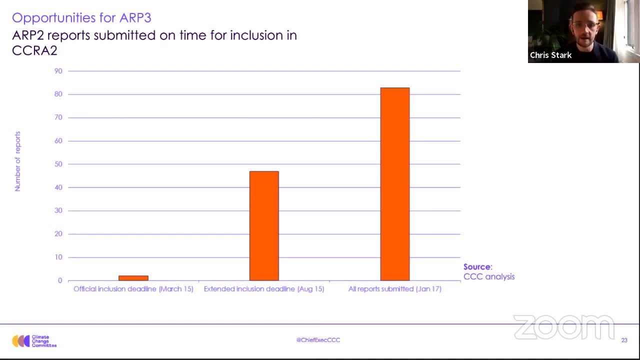 response rate by the, by the, by the first deadline and secondly, most reports that we got described the nature of risks. that was good, some usefully, quite, quite quite usefully quantified, ranked and aligned um, but we couldn't build an overall picture of the climate change risk and opportunities at the. 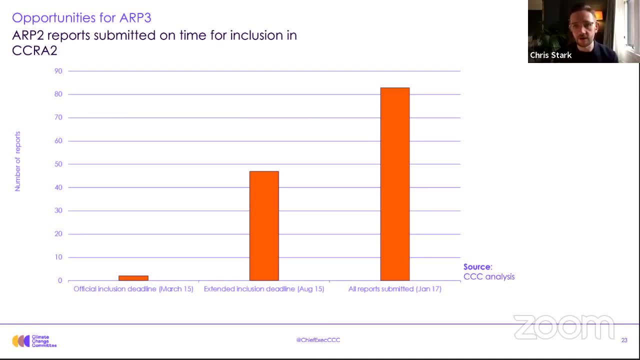 national and the regional level, nor the sector level to feed into our work for the second climate change risk assessment, and that's a problem that was mainly due to the timing of reporting, which doesn't align well with the climate change risk assessment cycle. so for me, that's something that 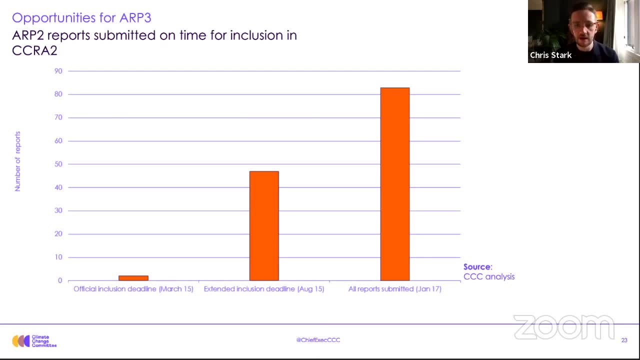 needs to be addressed. it's a huge missed opportunity, just a timing issue. we don't see a lack of good or consistent quantification of the risks and the impact of the adaptation actions and there are big gaps, frankly, in the risk assessment that we see across those uh 80 or so. 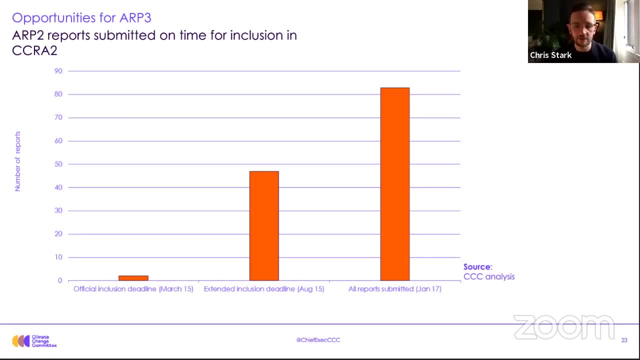 reports, especially on those interdependencies. in general, there was much more that we thought could be done to identify and prioritize the key actions that come in these reports. so that's the thing i'd like to put to this audience we should work on. and the final slide for me, terry, just thinking about 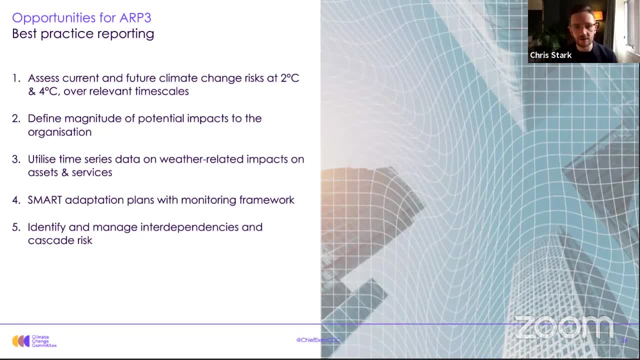 best practice when it comes to reporting. again, adaptation reporting really should be, i think, at the heart of a better adaptation cycle in the uk, mimicking where we get where we're getting to now on the emissions reduction side under the climate change act. uh, here are five broad pieces of advice to develop best practice. hopefully this will set us. 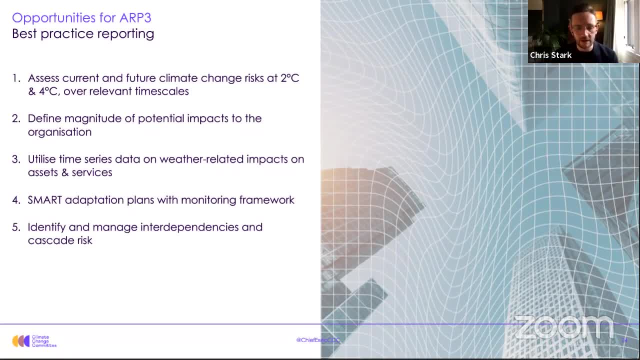 up nicely. the first is the most important. we need to get real about where we're heading with temperature change. so assessing current and future climate change risks at two and four degrees centigrade and, of course, the relevant time scales need to be attached to those temperature outcomes. 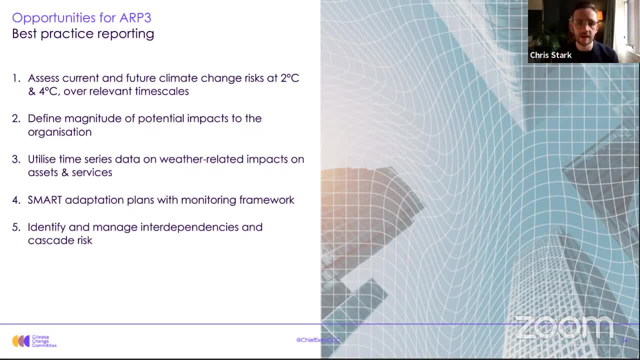 secondly, let's define the magnitude of potential impacts to the reporting organization. for many of you, the financial reporting requirements of tcfd are going to lead to this kind of more quantified outcome in any case, so there's going to be a lot of work that needs to be done to address that. so 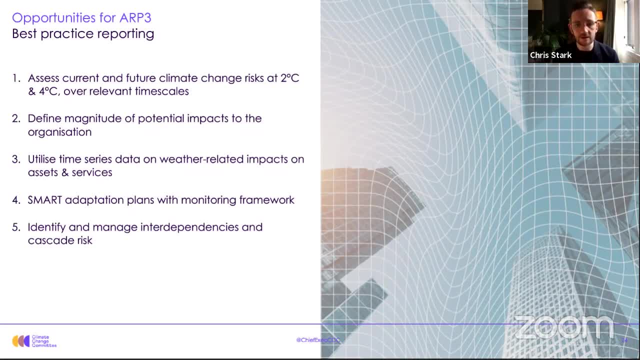 this is just going to be good practice. thirdly, please use time series data on weather related impacts- we've just heard stephen brilliantly cover some of this, but the impacts on the assets and the services that are supplied by your organization. fourthly, make those plans for 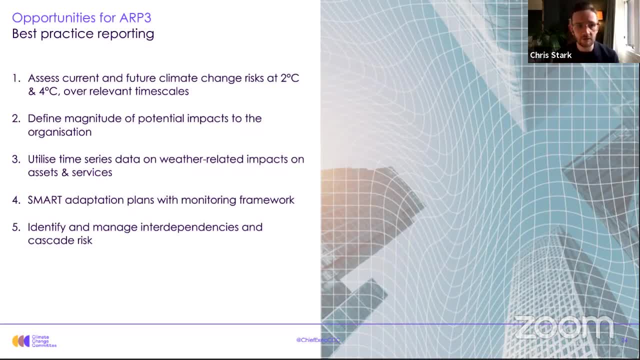 adaptation, as smart as they can be. we need a monitoring framework alongside that. and lastly, number five, let's identify and manage those interdependencies between the risks. that's that's the really important thing that is often missed: the very real cascade risk between those, those risks that we've seen out, notably in in texas just recently, and i'll just 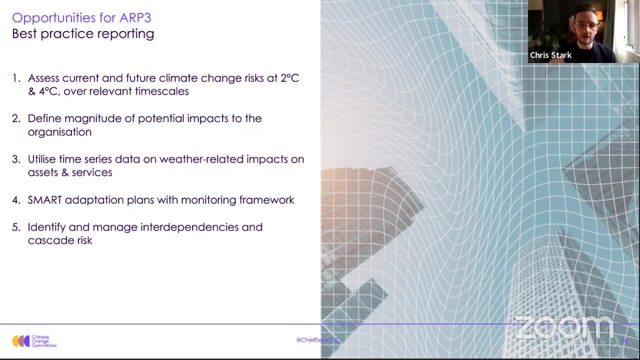 add just a handful, a couple of thoughts before i finish. we're going to need to move, i think, to mandatory reporting, something that i've said before and our organization have said before. we can do that in a way that that is not a burden. we can target that strategically so it doesn't 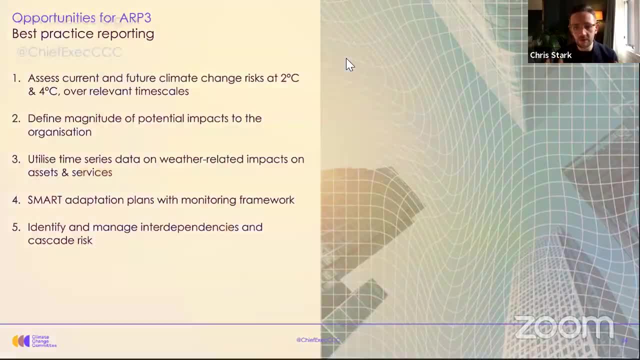 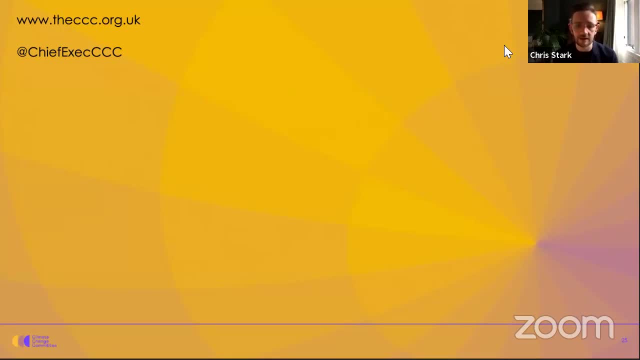 become the burden that i think minister's concerned it will be. it will reveal a host of benefits to the reporting organization as well. i've said it already, but a quick one is also to align the reporting better with the adaptation, assessment and planning cycle and let's very finally have have best practice that becomes business as usual. 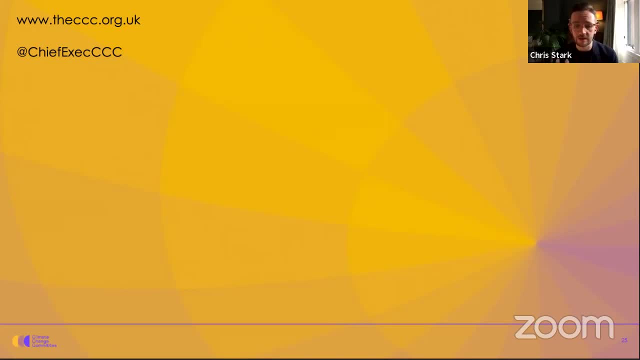 we should have an approach that is sector focused. if we can reporting to the tailored needs of each sector. it needn't be that burden. it should become the norm, the normal practice, and if it does so, i think there's huge benefits in doing so. terry. back to you, chris, that's excellent. thank you very much. 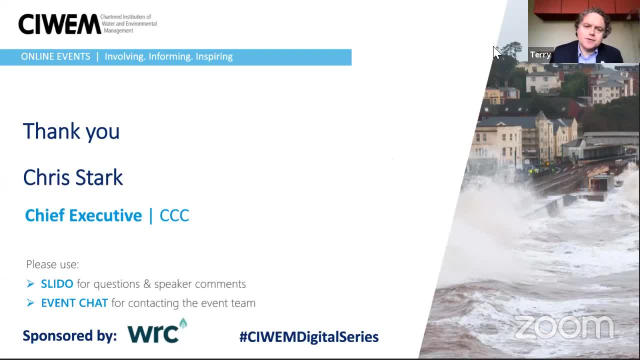 indeed and really strong message to to leave us uh with the takeaway: um, i'm gonna move uh on now to. our next speaker is mike keel. mike will talk to us about why all this matters to consumers. mike is the consumer council for water, head of policy and research. he spent the first decade of 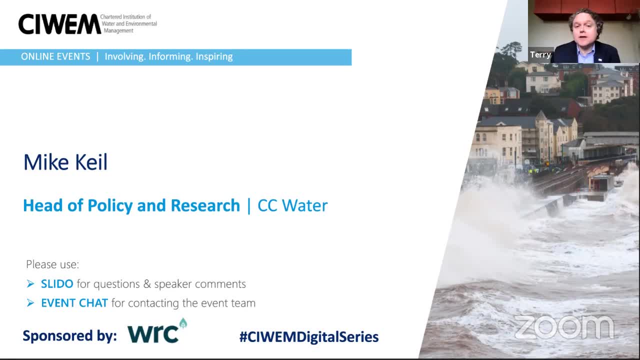 his career at the met office and led its middle atmosphere research group. in 2007, he joined off what as its first head of climate change policy and he wrote their first policy statement on the topic and their 2010 climate change ARP report. Mike then moved to Severn Trent Water in 2011, where he wrote the business case. 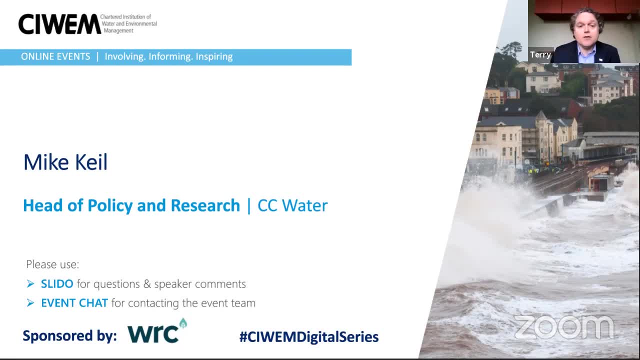 for the Birmingham Resilience Project and was heavily involved in their 2015 climate change ARP report. I'm told that Mike currently has toothache and he might be a bit grumpy, but don't let that stop you asking him some difficult questions, because I'm sure that will take his mind. 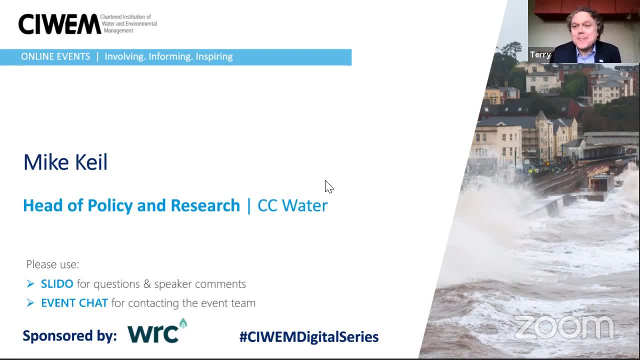 off it. So, Mike, over to you. Thanks, Terry. Yeah, I've got a double root canal. that was supposed to be this morning and I've put off till tomorrow. but that's not what you want to know about the cowboy dentists that exist during the age of Covid. So I'm here to talk about adaptation. 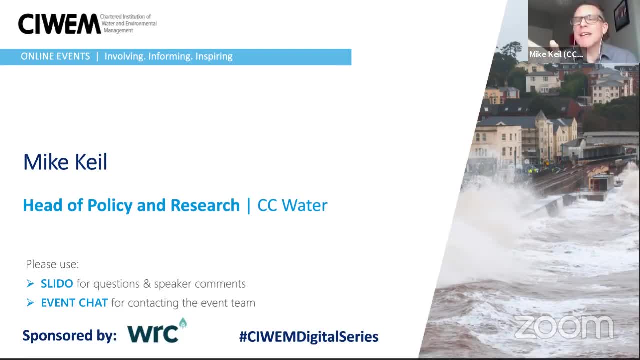 from a consumer perspective. Now I just want to start by saying: imagine playing a game of football without a ball. It'd be totally pointless. and that's how I view the climate change adaptation reports. So I'm going to start with the climate change adaptation report. So I'm going to start with the 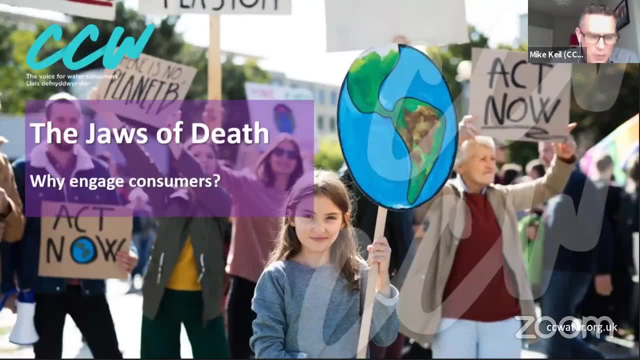 climate change adaptation report. So I'm going to start with the climate change adaptation report Now. you might not share that view, but climate change matters to every single person, as it affects our, it will affect our way of life and, when it comes to utilities, it will affect the. 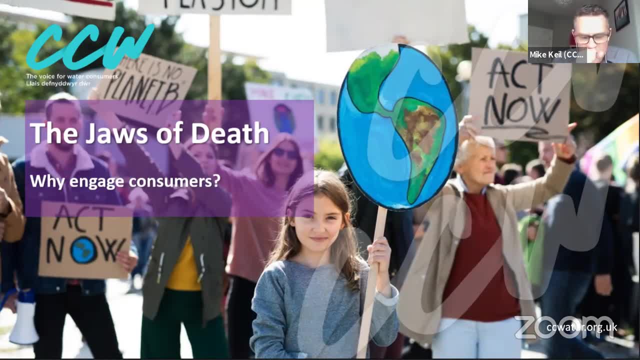 essential services that we rely on and the price we pay for those services. and that's why, as a consumer body for the for the water sector in England is England and Wales- climate change is a priority topic for CCW, So why engage consumers on climate change? 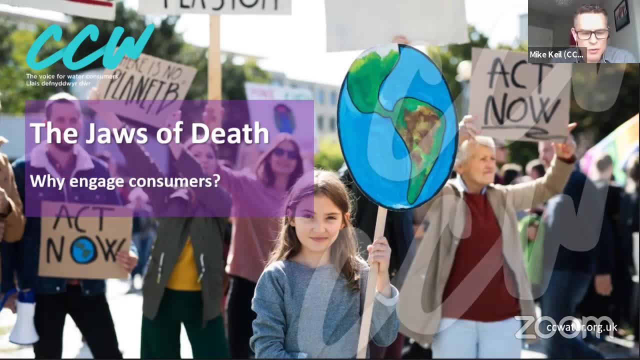 Climate change, adaptation, and what difference will it make? I mean, that's a crucial point. it's got to actually make a difference. It's not engagement for the sake of it or some sort of tick box exercise. This is what I'm going to explore over the next few minutes. The points I'm going to make are: 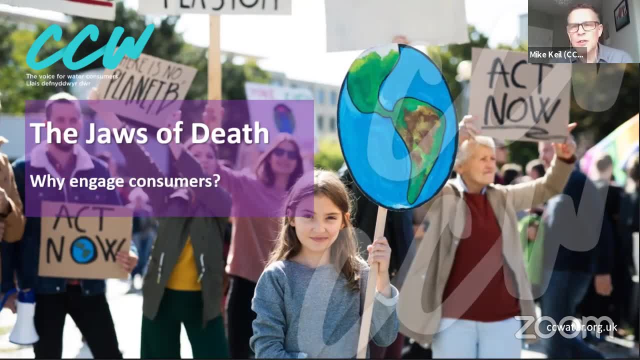 focused on the water sector, but many of them apply to other sectors too, particularly other regulated utilities. So a couple of years ago, Sir James Bevan, the Chief Executive of the Environment Agency, made the famous jaws of death speech, and that speech brought out the fact that climate change is not a 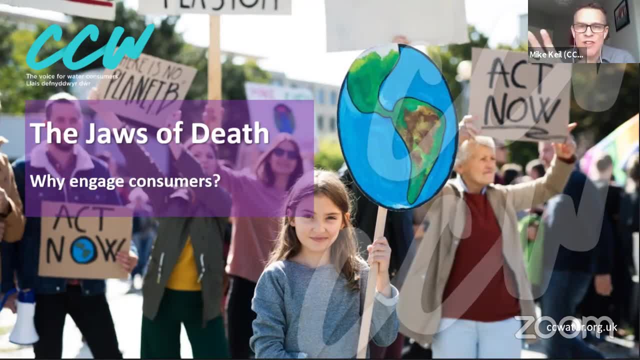 significant, brought significant attention to climate change and water issues, and by some very colourful use of language, which was which I very much welcomed, and that speech. he said that the missing ingredient to the coalition needed to escape the jaws of death was, was, was the public, was consumers, and in fact he said that they were the most important ingredient of all. and I couldn't. 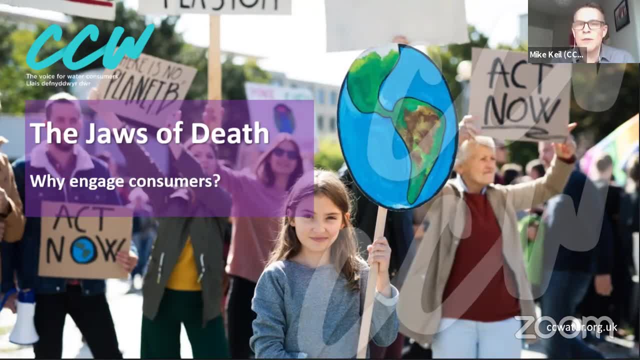 agree more. I don't think we talk enough about the role that people can play in climate change. Now, James Bevan was talking about engaging, empowering the public in terms of water efficiency, and of course, that was in the context of a speech that was talking about water resources. 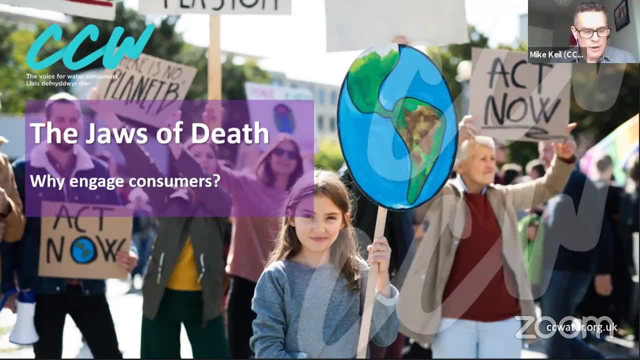 and the impending supply demand gap. that is, that is on the horizon. but when you consider the wider perspective on climate change adaptation- so not just water resources, all the other things that can affect utilities, for example- the need to involve consumers is even greater, and that's why the climate change adaptation reports are so important. The climate change adaptation reports. 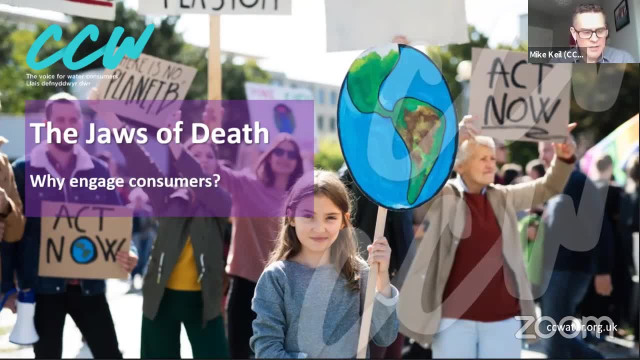 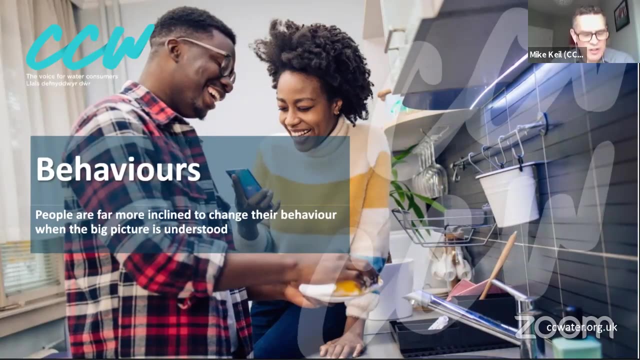 present a massive opportunity to kick start that much needed engagement and empowerment of consumers. So let's explore this in a bit more detail. We've already mentioned behaviour change when it comes to water efficiency, but behaviour change isn't just tied to water efficiency. there's also what 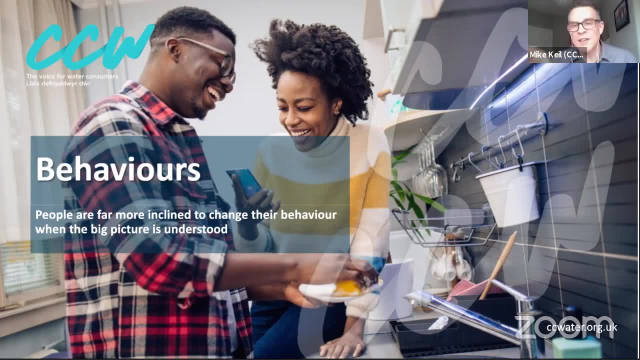 we put down our loos. when it comes to water, sewer misuse, putting the wrong thing down the toilets, or fat soils and greases down our sinks- it's a it's a really big issue, and people's own behaviour can make a big difference here. Now, I'm not saying that sewer blockages are caused by 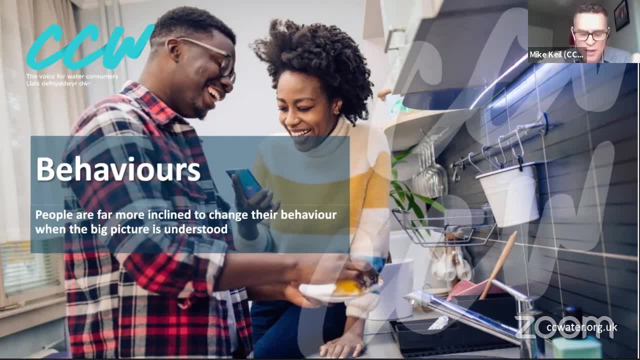 climate change, because they're not. but climate change puts further demands on our sewage networks and then exacerbates the problem, and we've done some work on consumers attitudes in the context of water efficiency back in 2017, and that showed that no matter how a consumer badged themselves, 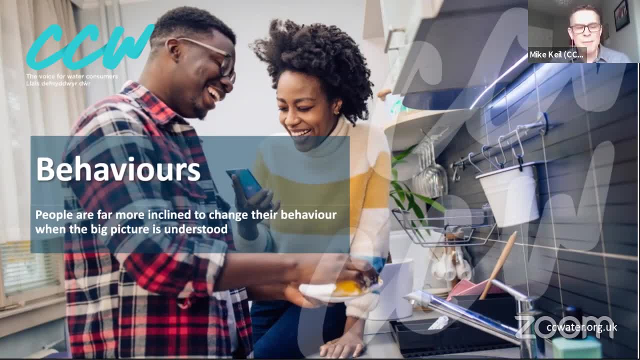 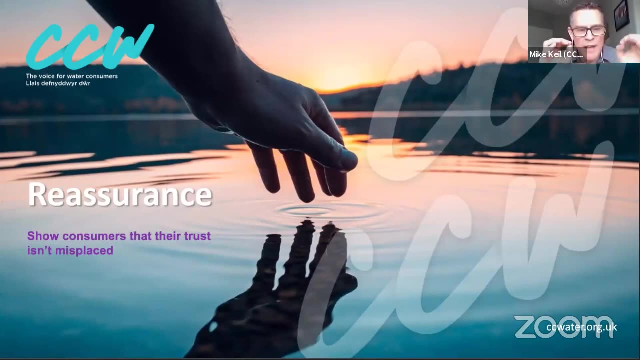 for example, if they buy themselves as an environmentalist or a penny pincher. an explanation for the climate change adaptation report is that the big picture of how climate change is impacting our weather was absolutely critical. People were far more inclined to change their behaviour when the big picture was understood, and the climate change adaptation reports are a really 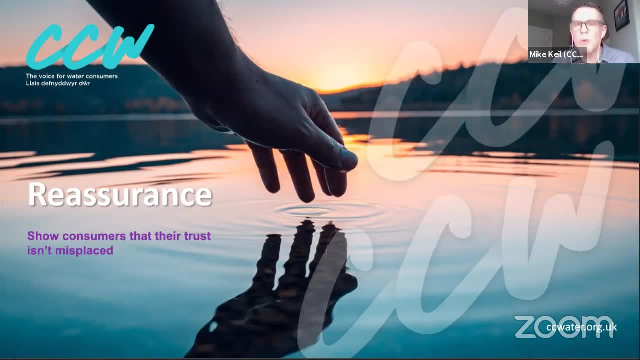 great place to set out that big picture and and the ways in which companies can help empower people to change their behaviours and their habits. Now the next point is reassurance, and I think this is a great thing to think about. We've talked about the issue of trust and adaptation reports. 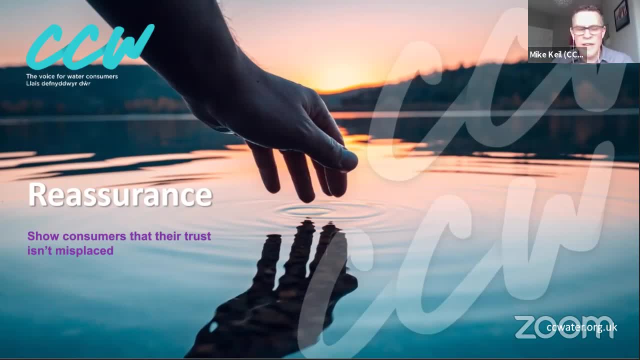 and I think that's a really important point to think about. You can't simply go. when you talk about adaptation reports, it's there to reassure customers, and I think it is absolutely true, but it's not the only game in town here now. currently, there's a very high degree of trust in water. 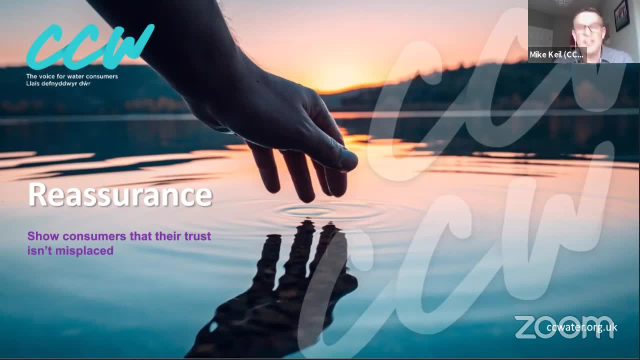 companies, and that's a really, really positive thing. it's something that should be celebrated. Most people trust that the water company is doing the right thing and is dealing with the challenges posed by climate change. Now the adaptation reports are, of course, a great way, a great vehicle for 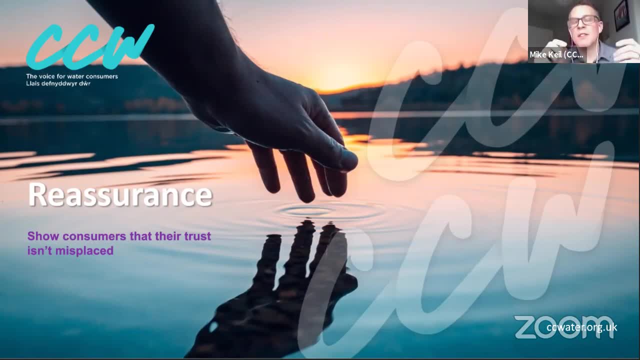 sure people that they are, that their companies are on it. then show companies, customers sorry, that their trust is in this place and you might be surprised to know there is actually a desire for people to have this information. yes, really there is, and we did some more research on this. 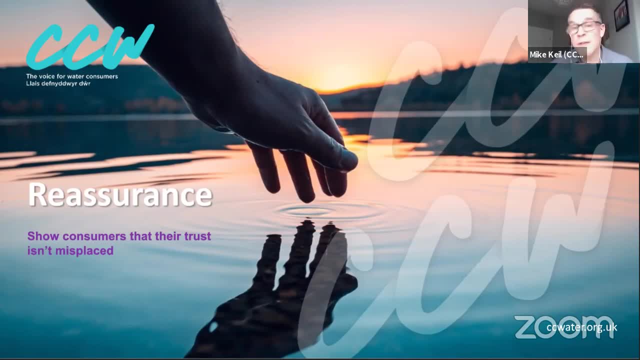 last year we talked to consumers about climate change. they they recognized it was the biggest environmental challenge that we faced by far, and and just under half the people we spoke to also thought that water companies were currently feeling the impact of climate change today. also, around two thirds of the people we spoke to said it was really important that water companies 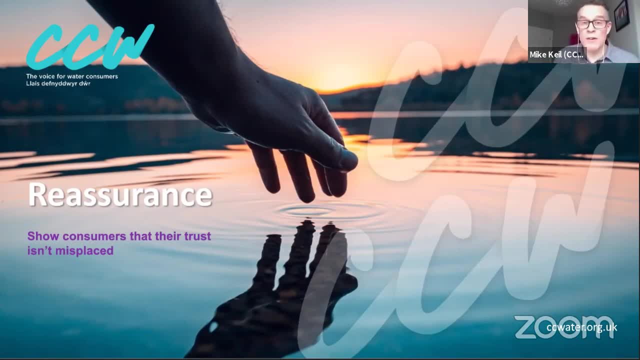 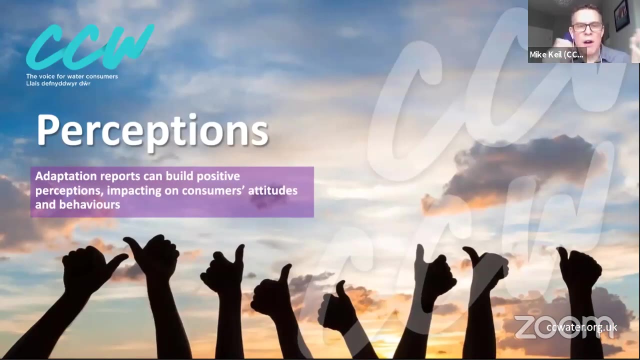 made this information available and this type of thing. so not just climate change, but wider environmental impacts too, and again, the adaptation reports provide us really good platform for doing this. and the third aspect i want to look at is is perceptions consumers use are really important for any business- anybody. 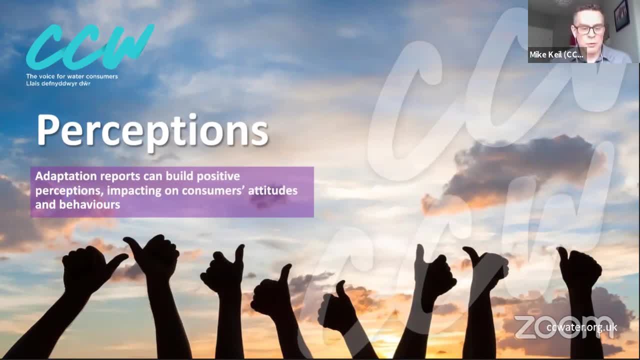 should be concerned with what their customers and consumers more widely think, that this is especially true in the water sector and regulated utilities, where customers can't well, particularly in water. actually, because customers can't choose their supplier and they can't walk away if they don't like what the provider is doing. so it's vital that water companies do all they can to 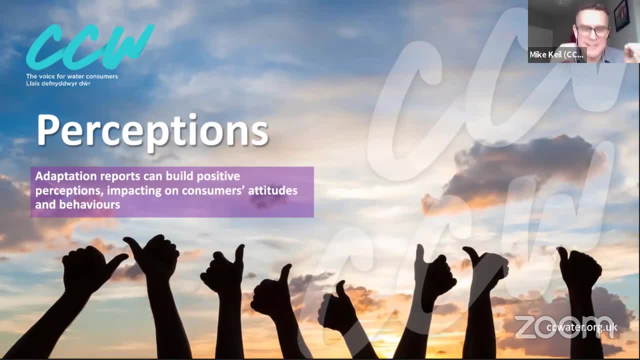 ensure that people view them in a positive light, because it's essential to maintain legitimacy in a regulated monopoly, particularly in the context of a monopoly that may have to be spending money in the future- significant money to build resilience. so consumer perceptions in water industry are really important, are really positive in a number 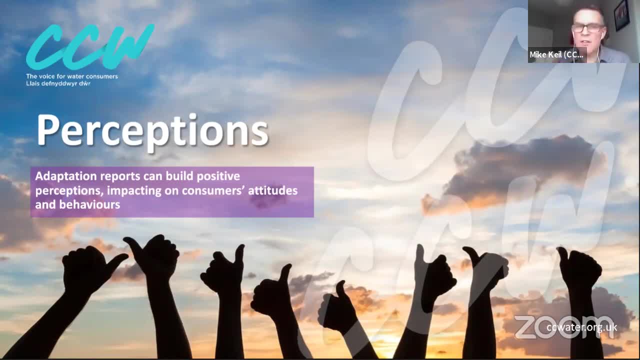 of areas that i've mentioned, for i mentioned trust earlier, but others aren't so high. you know, things like value for money and fairness of bills could be much higher and uh- and that's something that actually does affect people, people's attitudes- and the adaptation reports can really help you. 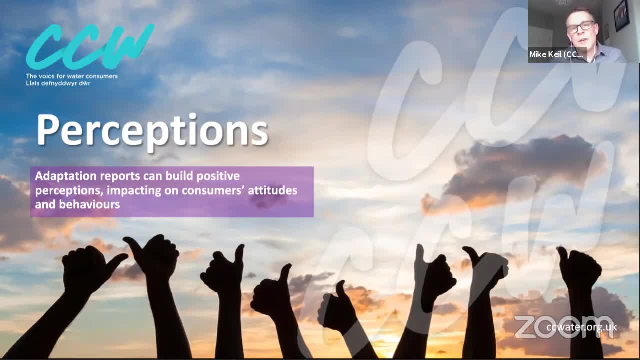 because one of the things customers said to us when we talked about how do you increase value for money scores is they were saying: well, tell, tell me how my money's spent. i have no clue where it goes. and actually using the adaptation reports to explain that the money is invested well. 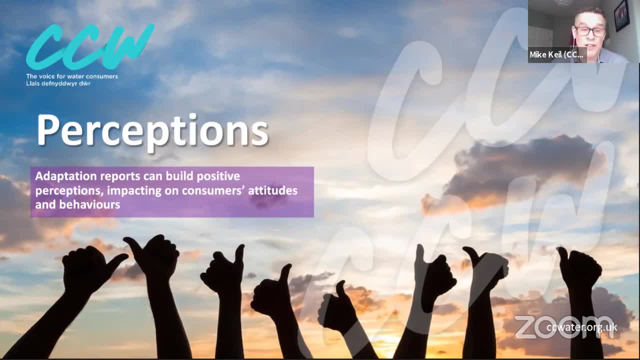 can and invested in areas that customers think are really important, like reducing crime at risk, can really help change perceptions. but perceptions aren't just about bills and bill levels. it's about other things, including views on whether the company cares, uh, whether the company is viewed as profligate in their use of resources, and there's a link back to the behavior point here. 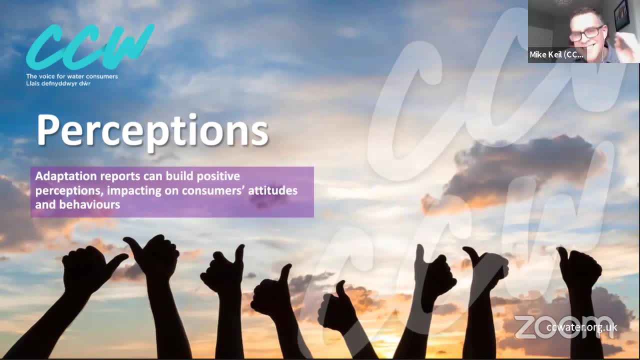 because if if people are much more are less likely to change their own behavior, they're much more likely to change their own behaviors in their homes in terms of being water efficient if they view their water company is profligate in their water use and that's why leakage can be very damaging. 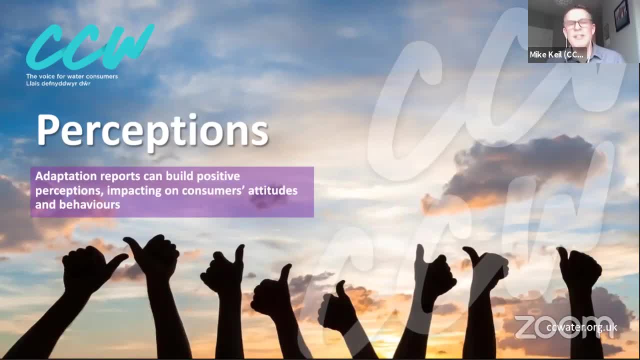 to perceptions, those visible leaks that run and run can have a hugely demotivating factor when it comes to personal behavior change. and again, that's why the adaptation reports can build positive perceptions by clearly articulating how much the sector is doing to be good stewards of our 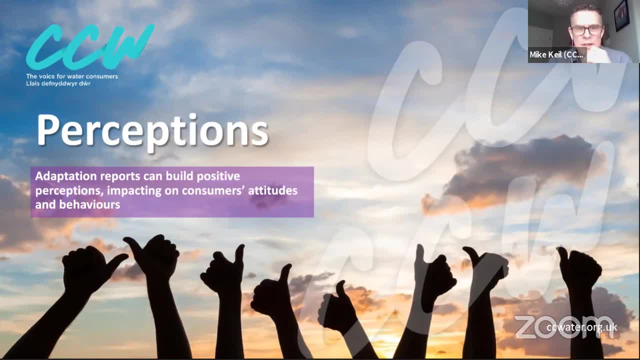 water resources and how they're protecting them for the future. now, perceptions are notoriously hard to shift, and that's why companies need to take all of the time before they're able to change their own behaviour. if they are not able to, then they will continue to change. 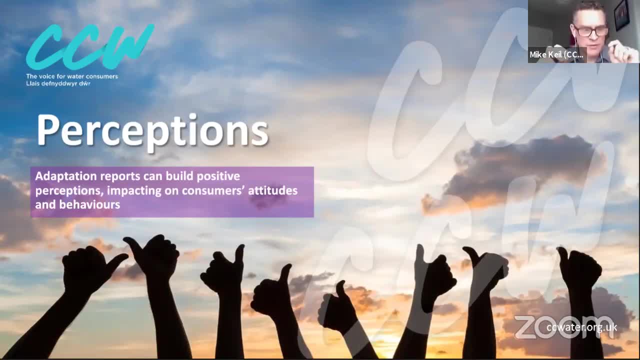 including these adaptation reports to turn that dial in a positive direction. So, in closing, we are very keen that the most is made out of the adaptation reporting And this is one of the reasons why we've written to all the water companies to give them some pointers. 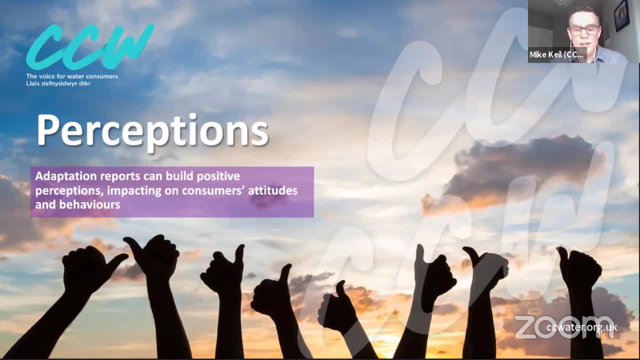 on what the next adaptation reports could look like from a consumer perspective And we intend to keep that dialogue going and helping to bring people together, such as this event, And we want to look to share good practice and share insights more widely, And there's tremendous potential here for companies to use these reports as a communication tool. 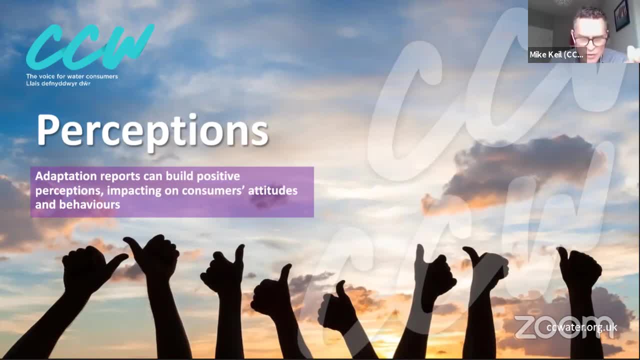 with a clear purpose of communicating with consumers in mind and trying to act as a turbocharge for behaviour change. So it's not just about providing reassurance that climate change risks are being managed. It's also about building positive perceptions and acting as that catalyst for behaviour change. 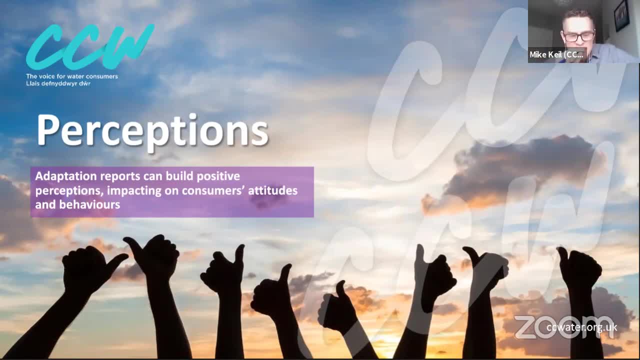 It can make a real impact on our journey to adapting to climate change. So if we're serious about adapting to climate change, then we've got to get serious But understanding the role consumers can play. So that's all I'm going to say for the moment. 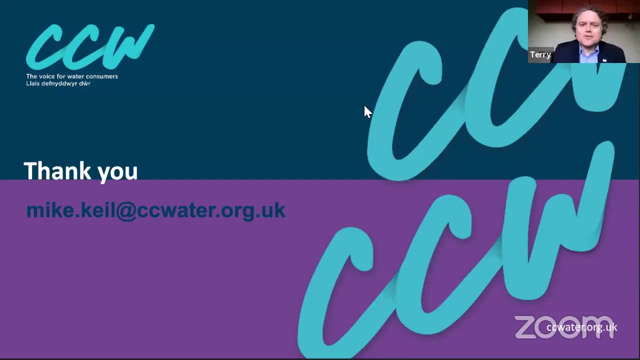 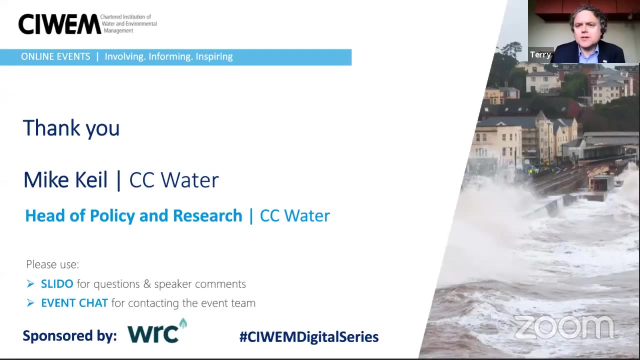 So thank you very much. That's great. Thanks ever so much, Mike, And a really good reminder of how important it is that we we understand people's perceptions and then we get that consumer and public view on on all the things that need to be done. 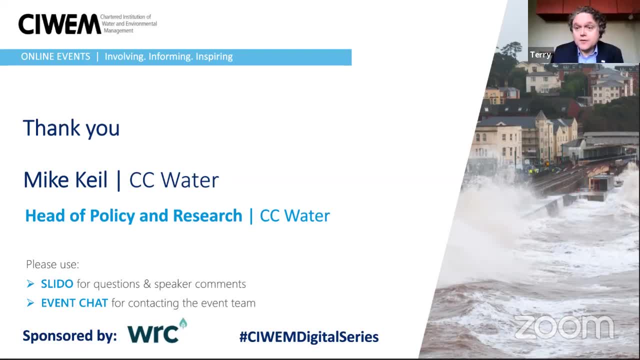 I can see some questions are coming through on Slido- and quite a few in fact- and also some answers being generated as well, So that's great. Please keep that coming. We're now going to move to our final speaker in this session, who is Francis Pimenta from DEFRA. 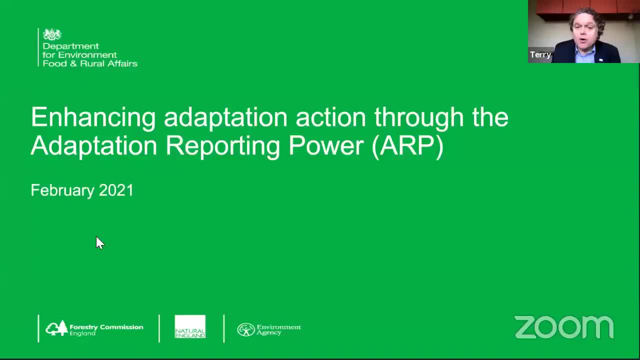 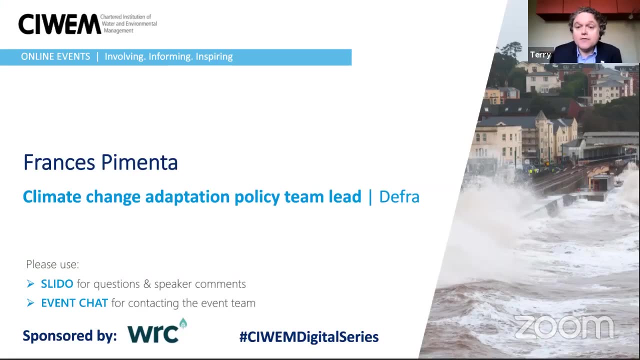 Francis leads DEFRA's climate adaptation policy team, responsible for delivering duties in the Climate Change Act of 2008 on preparing for climate change. This includes implementation of the National Adaptation Programme, working with action owners across government, public agencies and in wider society to ensure actions and objectives are achieved. 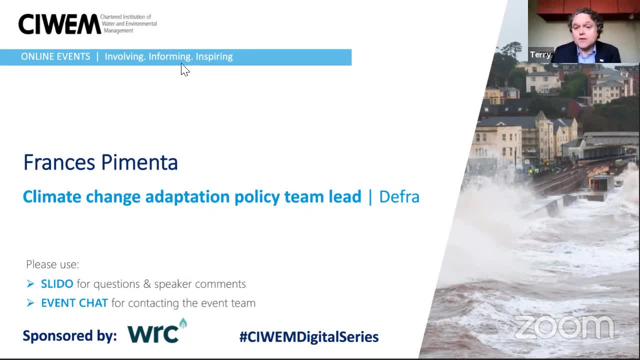 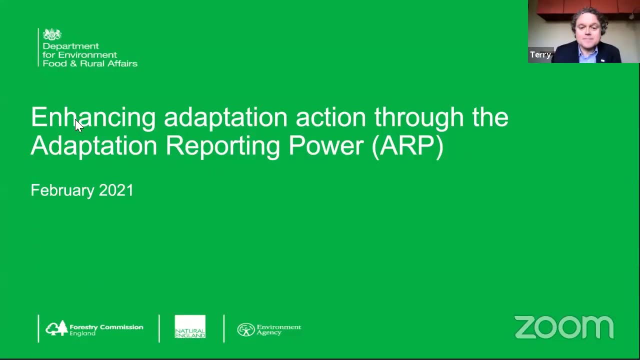 More broadly, the adaptation team is involved in promoting adaptation within government to ensure that consideration of climate risks is embedded in policymaking. Francis, over to you. Thank you very much, Terry. Apologies, I was just struggling with my technology a bit there. 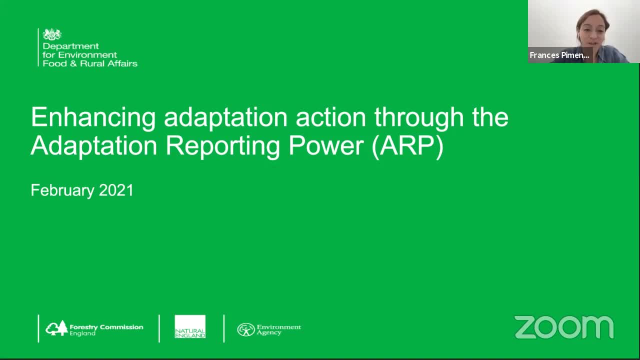 All good. Thank you very much, And I'm Francis Pimenta, as Terry mentioned, and I work in DEFRA's adaptation team. It is a pleasure to be here speaking today about adaptation reporting power and just how important it is for us and our statutory framework overall. 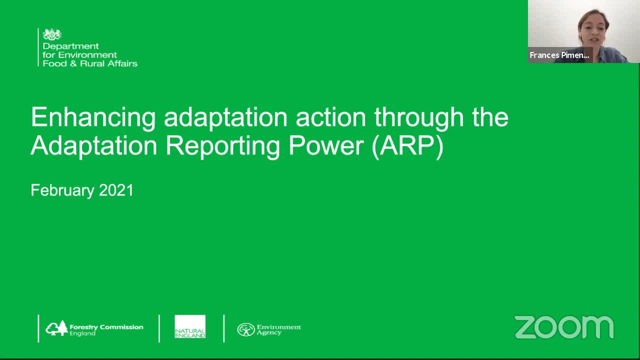 I think this is a really timely opportunity to have this conversation today as we enter that last phase of the adaptation reporting power theory. Thank you. So we're going to start with the adaptation reporting power third cycle which, as has been mentioned, ends at the end of this year. 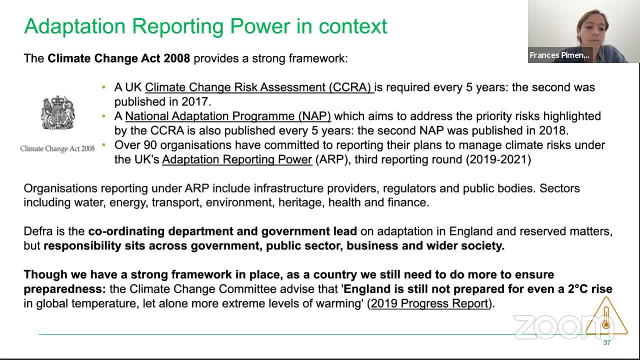 So I just wanted to kick off by framing ARP in terms of our statutory framework, So the Climate Change Act 2008.. And, of course, the first pillar of that framework is our climate change risk assessment, which is required every five years. 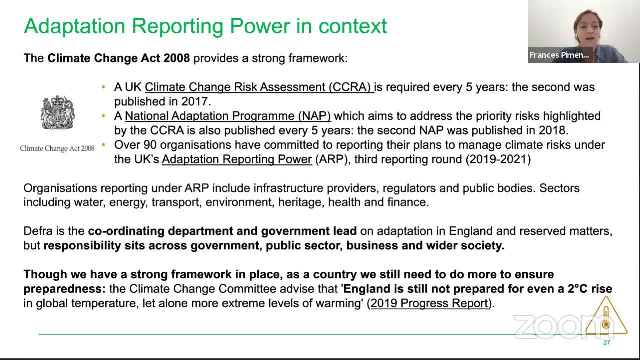 The second pillar of that is the National Adaptation Programme. So that's our programme to address the risks highlighted in this framework. So that's our programme to address the risks highlighted in this framework, highlighted in the CCRA, and we're currently in the second national adaptation program midway. 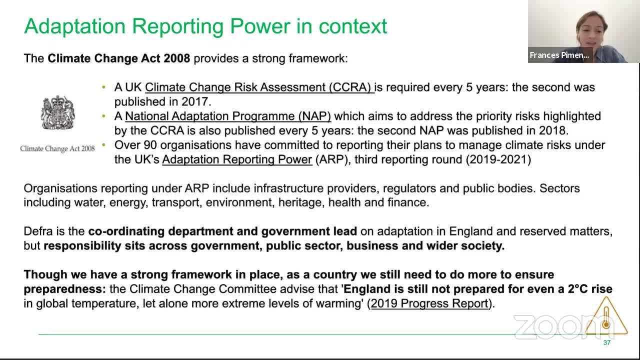 through delivery, and that will complete in 2023.. ARP is our third pillar and it is, of course, the power that our Secretary of State has to invite or direct relevant organizations to report on their plans to manage climate change risk. I don't think I really need to go into this, but ARP covers. 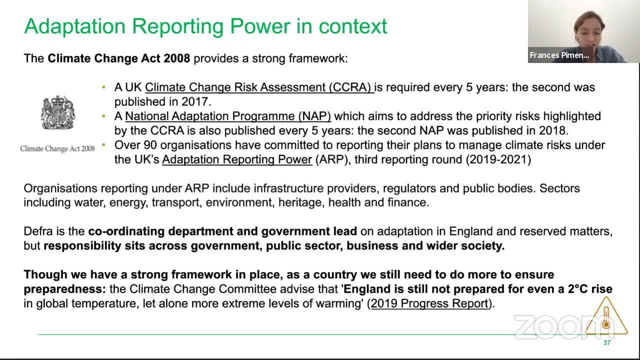 a wide range of organizations, from infrastructure providers, regulators, public bodies and across sectors such as water, energy, transport, the environment, heritage, health and finance, amongst others. So DEFRA, where I work, is the coordinating department, but of course, responsibility for delivering actions, making change and addressing risks sits across government public sector. 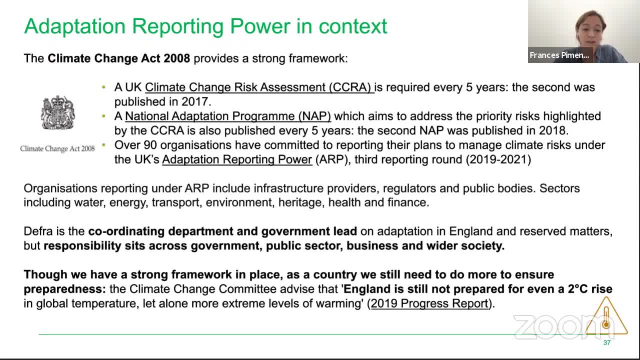 business and wider society. so we all have a very important role to play and, as Chris and others have mentioned, we're a very important part of the government. We're a very important part of the government and we're a very important part of the government. We're a very important part of the 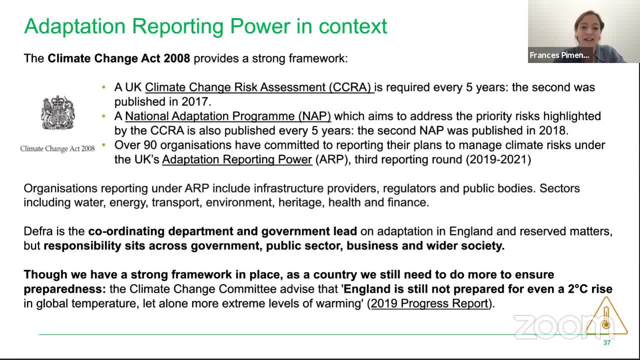 mentioned today. we have a strong decade of have a strong decade of this statutory framework in place, but there's a lot more to do and clearly we need to get real about those risks posed by the two and even four degree levels of warming that we may have to confront. so to put ARP back, 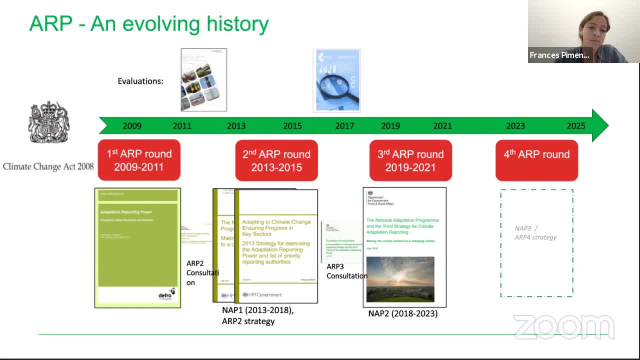 into that context. ARP was the first step of our statutory cycle that actually was enacted back in 2009. it kicked everything off and since then we've had two rounds. now in our third, we've had a mixture of different mandatory and voluntary rounds. in the past, these have been 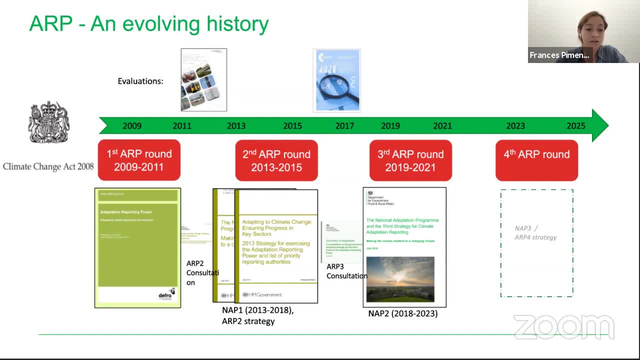 informed by, by consultations and obviously our ministerial steer, and we've had some good evaluations, something that is quite interesting from our perspective as we enter this third round, we enter the end of the third round. it's just, I think, what something I felt is just how much climate has risen up the agenda and just the level of interest that we're 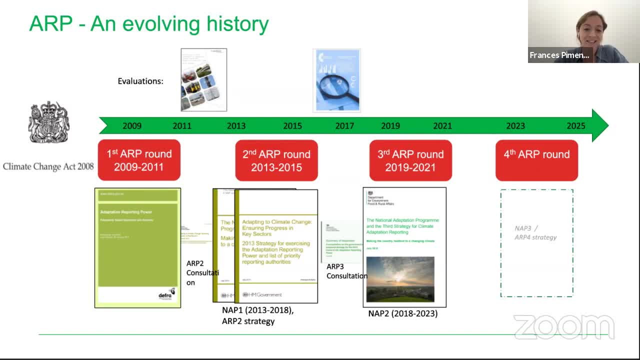 getting and inquiries we get about ARP and indeed it's the part of our statutory framework that I get the most questions about from counterparts and governments across the world. so I think it is definitely a hugely important part of our armory and and actually a very innovative and interesting 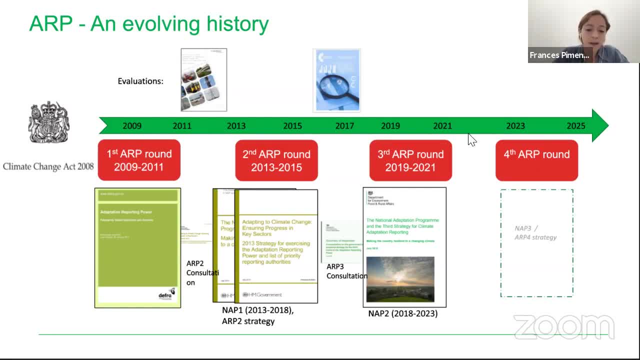 part of our approach, I think, in terms of ARP. so just to warn everybody, the ARP override has been removed from the system. at this point. we're actually close to inkling the next stage of the scale, and so I can't really say anything about which I found was better. 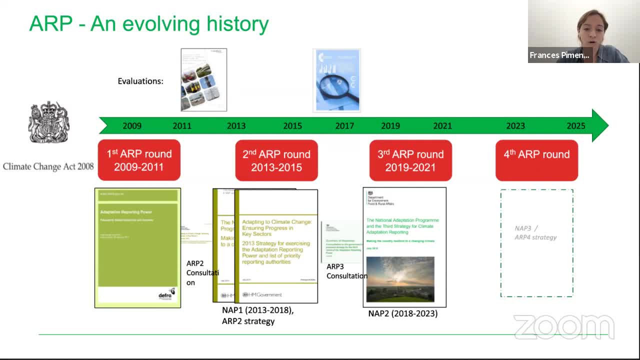 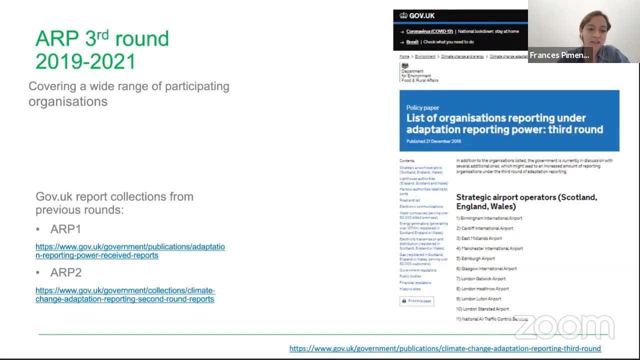 but we're re-en Holly. Mr Stewart, yes, we have that, that kind of stronger role compared to the second round, and we're very excited by the large number of organizations reporting. so it's feeling been a positive experience so far. if you'd like to find out a bit more about previous reports, they are all available on. 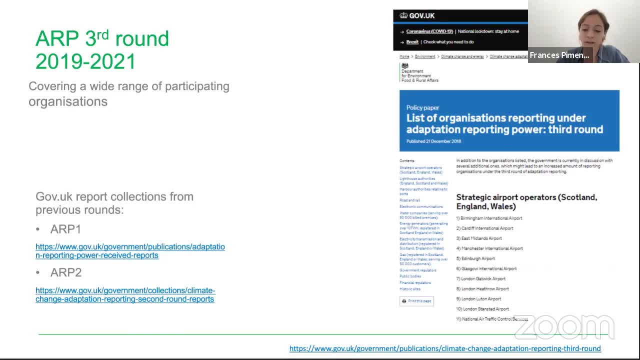 govuk. so we've got that transparent portal to to read more about it. we also publish a list of reporting organizations in the third round there on govuk as well. in terms of the principles for erp, i've gone into this a little bit, but it is very much framed. 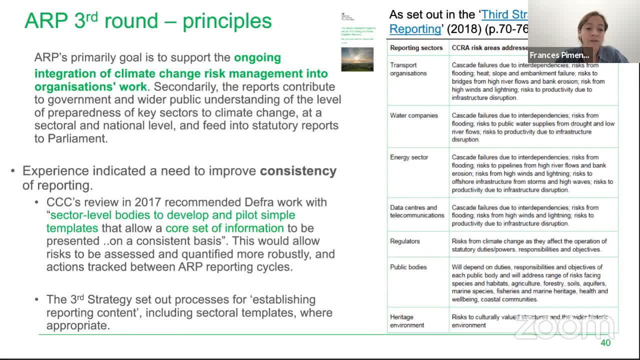 around primarily supporting the ongoing integration of climate change risk management into organizations work. so it's there to benefit the organization's reporting, as has been mentioned, but has a secondary role as well as informing government, the ccc's and the wider public understanding on the level of preparedness across key sectors. so it has this really important. 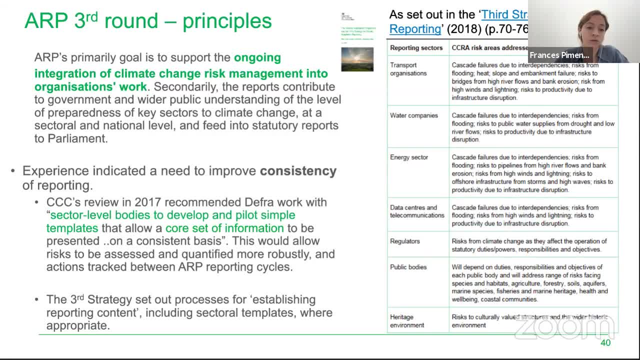 role of supporting the ongoing integration of climate change risk management into organizations. so it's there to benefit the ongoing integration of climate change risk management into organizations. um, and as, as i've mentioned, this for this third round, we've really looked at the question of consistency and quality and support for those sectoral approaches, those common sectoral. 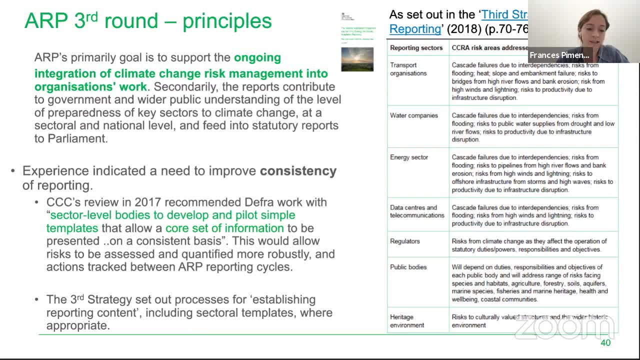 approaches to reporting to ensure high quality, content and consistency and approach. um, i think with this third round, where we've really been looking to see that maturity of approach and building on the good foundations of previous reports, there's a lot organizations will have learned in the in the period in between and was. there's also been a lot of developments in terms of the. 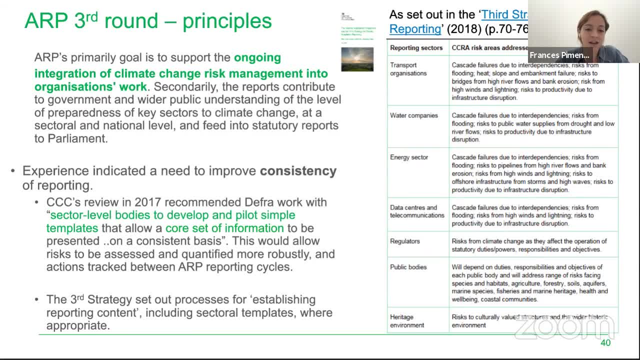 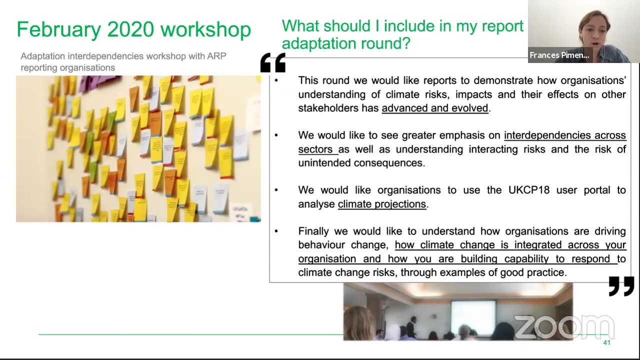 science. we've heard about uk cpat and projections. i think since the last report ended in 2015, we've broken just about every weather record, so there's a lot to take stock of, i think, as organizations think about this for their third round of reporting. so, in terms of defra's offer, 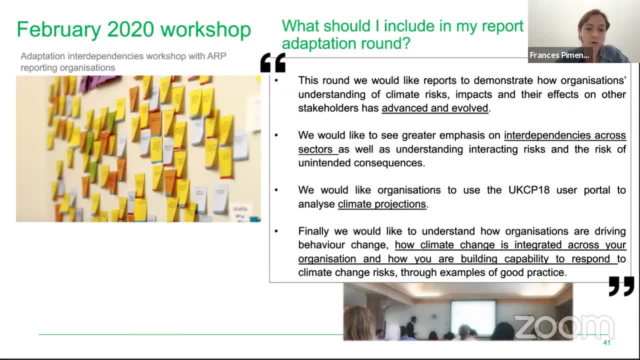 with uh. we've been convening sectoral conversations and working with reporting organizations and just about this time last year we hosted a workshop uh with the all the range of reporting organizations in defra and and had a deeper discussion on what some of the the key issues. 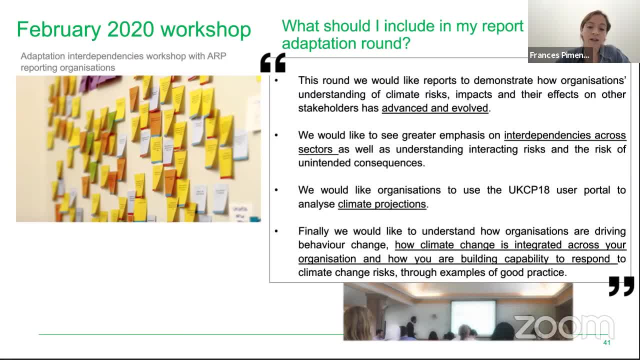 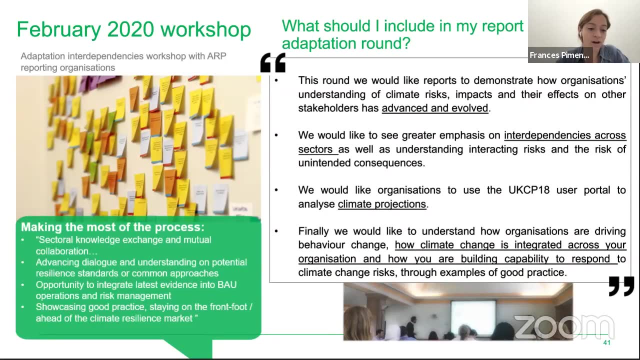 to think about in the third reporting round should be so that covered the the topic of interdependencies in particular. we also spoke about climate projections and the role of promoting and sharing best practice. so organizations shared some of their takeaways on on how to make the most of the process as well. i've summarized them on the slides there, um, but there's, i think, a lot. 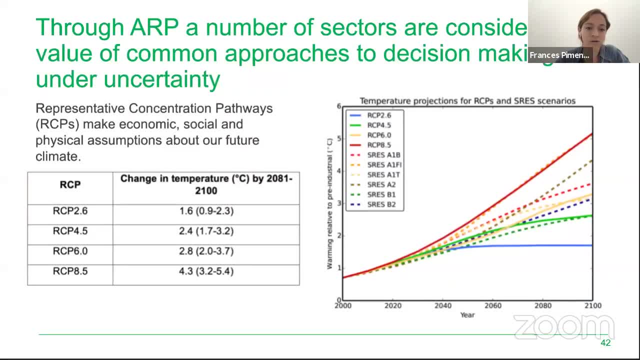 a lot around this concept of of common approaches and sectoral conversations. arp has also helped foster a number of conversations around common approaches to decision making and, just reflecting that, defra's been part of conversations with the water sector and transport sector bodies around how to how to grapple with the question of 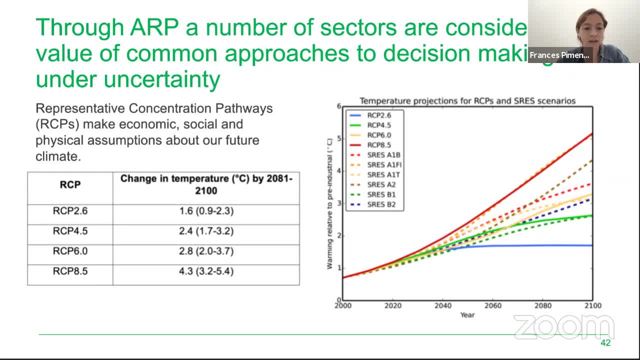 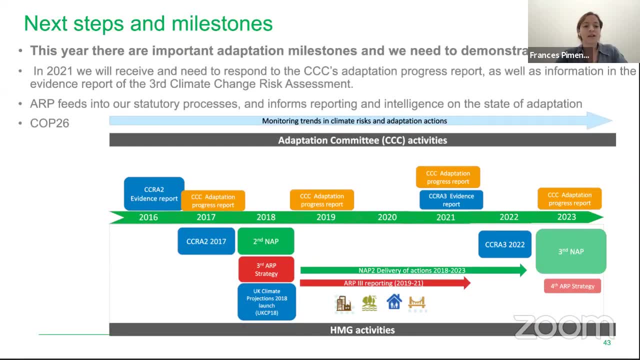 of scenarios and which scenarios to use, and whether we can converge around those in our planning approaches. coming towards the end in terms of next steps and milestones, this is a hugely important year for adaptation, not just, obviously, because the uk is hosting cop26 and adaptation and resilience. 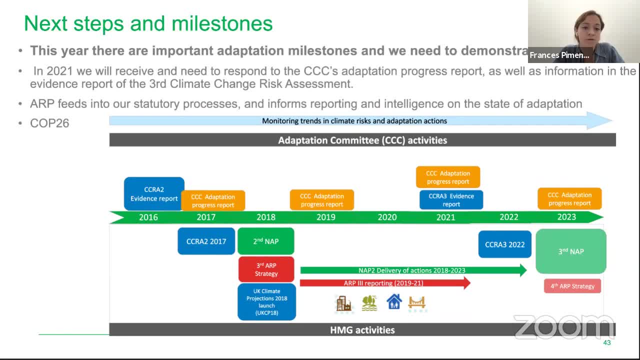 are one of our top themes for that, but for in terms of our domestic framework, we've got some big milestones coming up. so on this timeline, you'll see that we've got a progress report in june. so the ccc's two yearly progress report comes out then, and we've also got an evidence report that will inform our third. 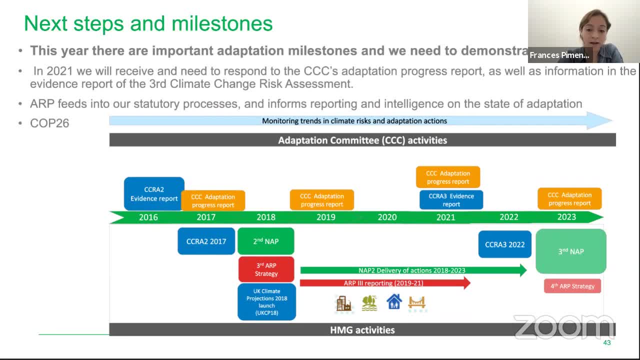 climate change risk evidence report as well, and so that government response will come out in january next year. so there's everything to play for. our arp. three reports, i think, will provide that excellent benchmark for just how far we've come in that decade since, uh, the climate change act came. 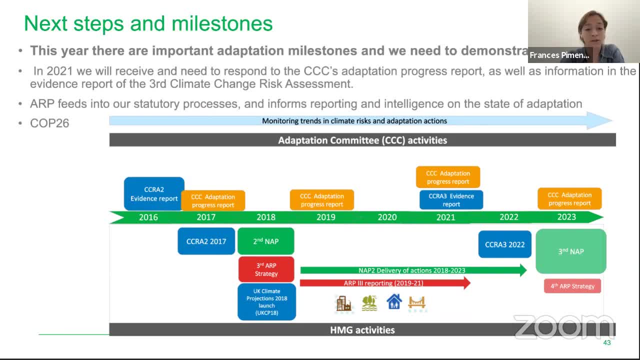 into into the climate change, climate change act and the impact that it has had on the climate change impact and the impact that it has had on the climate change impact into place. um arp very much feeds into those statutory processes and informs our reporting and general overall intelligence on. 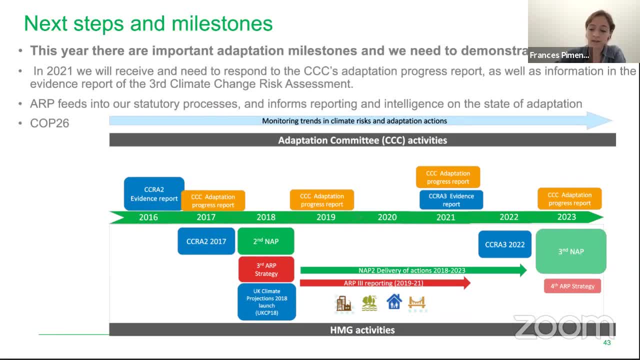 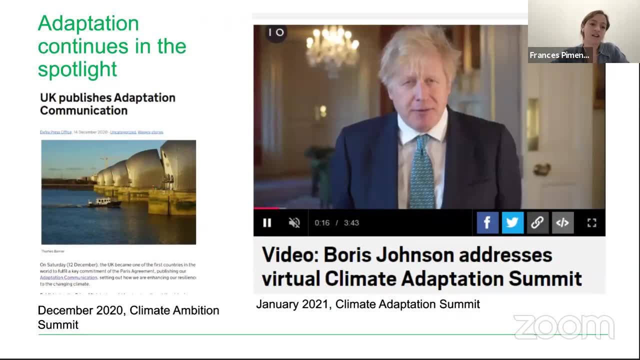 the state of adaptation in the country. so it's cannot be on overstated just how important it is. um, and just to kind of end on on a positive note, we've definitely seen and felt, uh, in depth for just how much adaptation has been rising up the agenda. um, we've recently had some, some big moments. 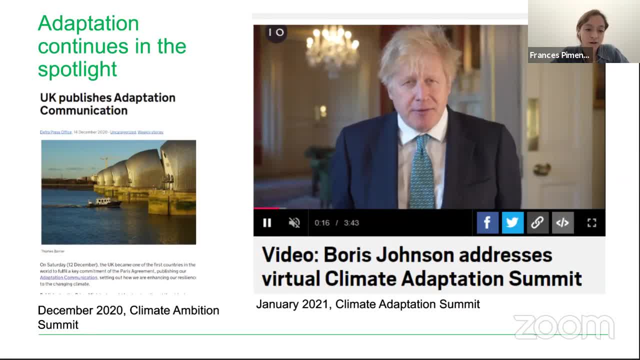 in a couple of weeks the first climate change summit in the uk, publishing its first adaptation communication to the un, the un triple c in december at the climate ambition summit, alongside our ndc commitment on emissions reduction. and we've recently had the prime minister addressing the virtual climate adaptation summit in january and indeed yesterday he addressed the un. 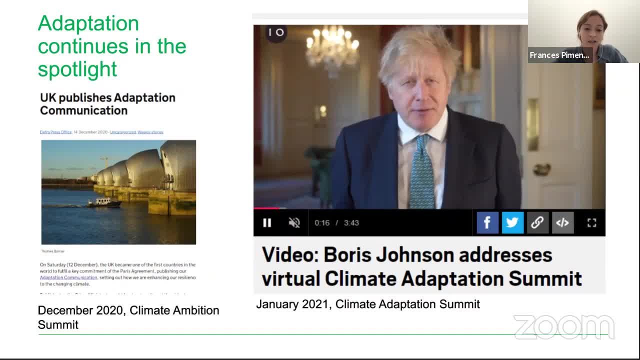 on the topic of climate security and impacts in that sense. so it is a hugely important moment and i just wanted to to end on the note of thanking all the reporting organizations for their work. and- and i just wanted to to end on the note of thanking all the reporting organizations for their work- and 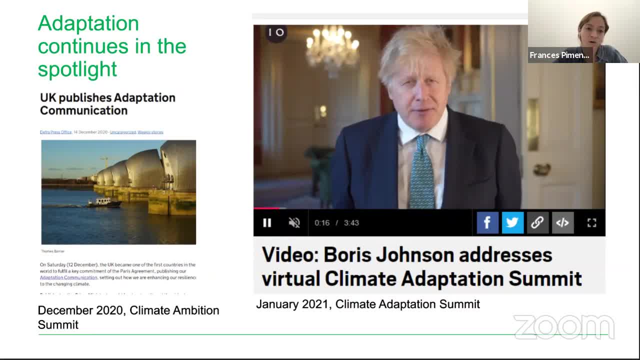 for their continued commitment and leadership in reporting. i hope that this process continues to be as useful for you in galvanizing action within your organizations and in your sectors, in showcasing best practice, as chris said, in really getting real about the huge challenges we face. but i hope it is as useful for you in that sense as it is for us in deferent. so a big thank you. 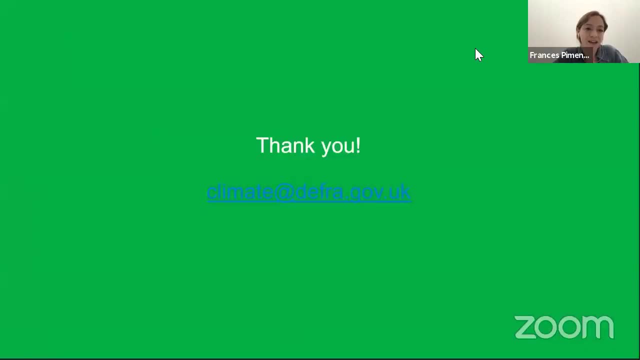 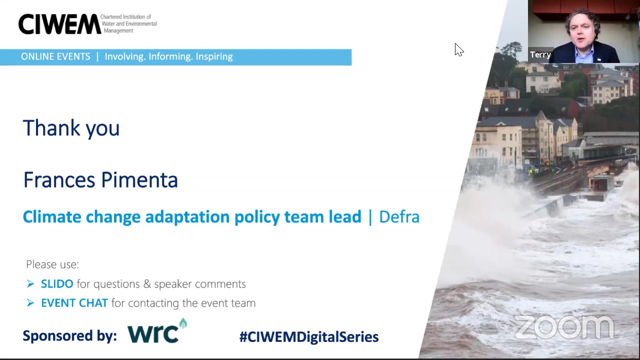 from us. i'm really looking forward to receiving the reports um as they come in throughout the rest of the year and looking for the presentations later today. thank you, that's excellent. thank you very much indeed, francis, and thank you to all of our speakers this morning. um, if you could perhaps. 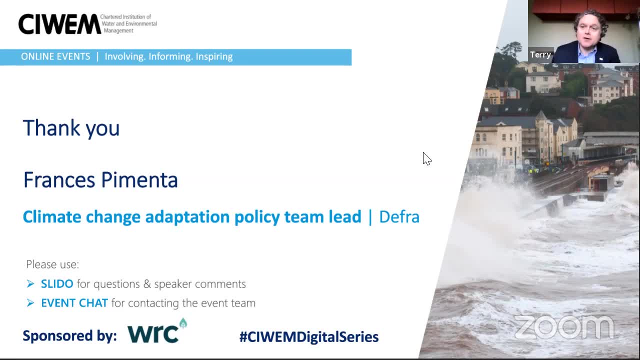 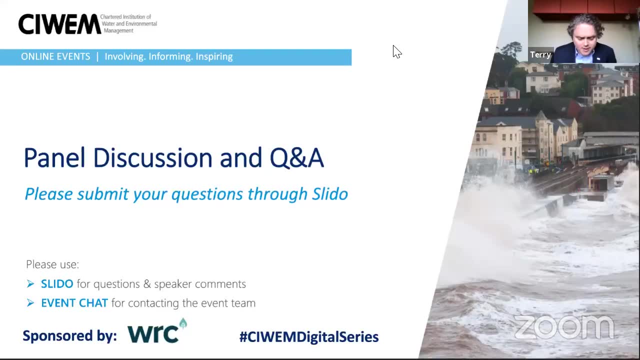 come back on to to camera, please, our panelists. we're going to move straight into some questions. there's some great ones, um. in fact i'm just going to go to um one of one of the top, or couple of the top rated questions here which some of you have touched upon in your presentations around the mandatory or or not. 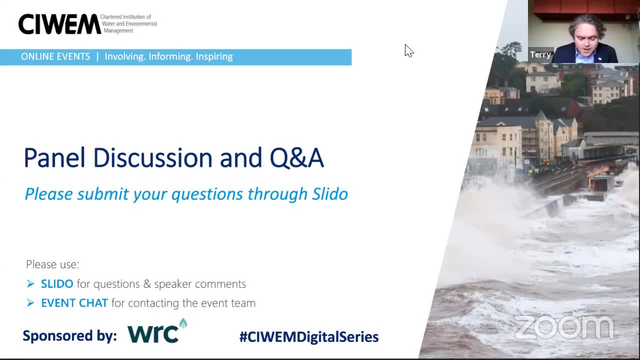 non-mandatory nature of of reporting. so a question we have here is um should reporting be mandatory and, if so, for who and why would it be useful? and i think the related- a related question here also is around the role of the task force for climate related disclosure and whether that's a a useful 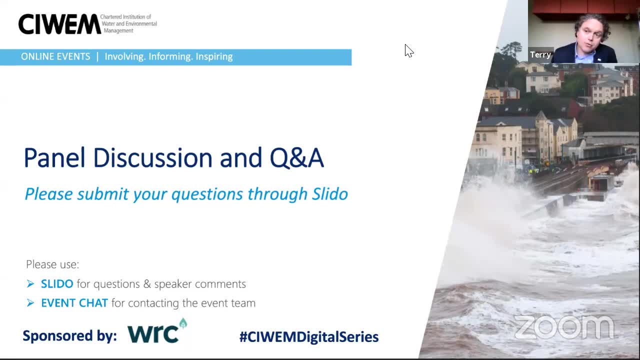 sort of channel and tool at all to um encourage reporting. so, um, i'll open it up to all of the panel, please to to respond. who would like to to go first? i could take that, one, terry. i mentioned it. um, yeah, thank you. um, yes, i think it should be mandatory and that's a long-standing position of the ccc. uh, we've made. 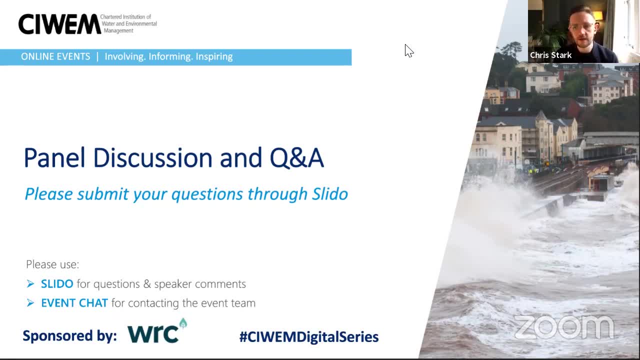 that point several times to uh different ministers, uh, and the importance of that is that i mean we've kind of lost. i'm afraid the momentum that we've had over the last couple of years is that we've got through the first round of reporting into the second and now the- i'm sure- the third reports will. 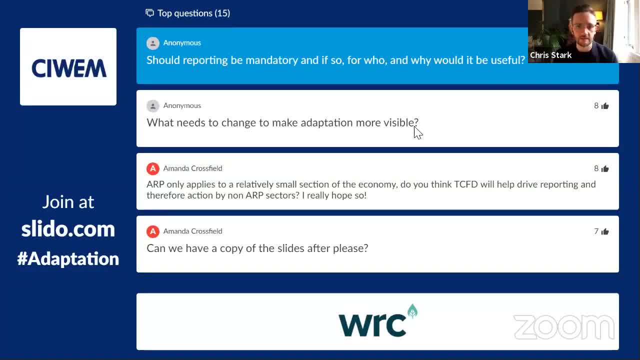 be better, but it would have been better if we'd been consistent in, uh, you know the need to produce these reports throughout the uh, the last, the last 12 years. so that idea of being mandatory- mandatory is not a good word, is it? it sounds very, it sounds negative, but uh, the point about this is that, with 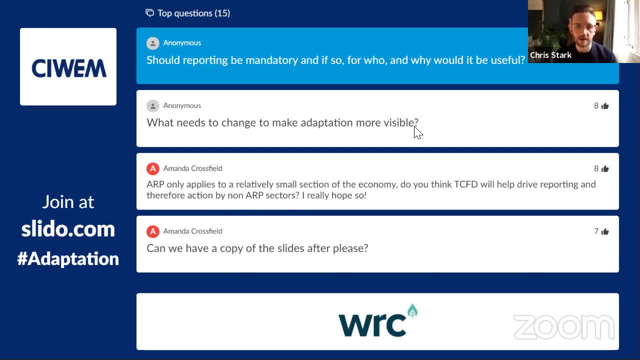 with mandatory reporting comes more consistent reporting and and augmenting and improvements over time come with that too. so that's the that's. the key thing is that we we're going to have to be. we do see these gaps in the reporting now, sadly, that have come uh and some of the organizations. 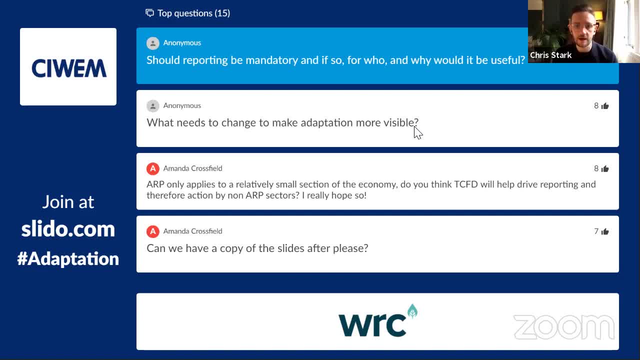 that uh reported in the first round, didn't report in the second round and we're kind of making up for lost ground, i'm afraid, on that and i'm afraid we're not going to get to the outcome that we all seek until we return to um uh, mandatory reporting. sadly, and for me, that the other 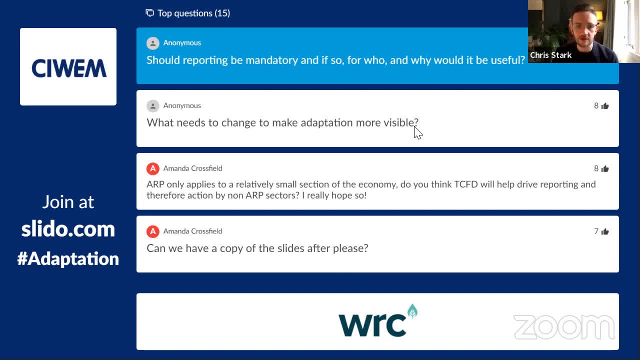 point i would, i would accompany with that- is that it is possible to do this in a strategic way so that it doesn't become a huge burden. uh, i made that point in my um, in my, in my talk, uh, and in any case, that the, the reporting has benefits not just to the, to the state, to the, 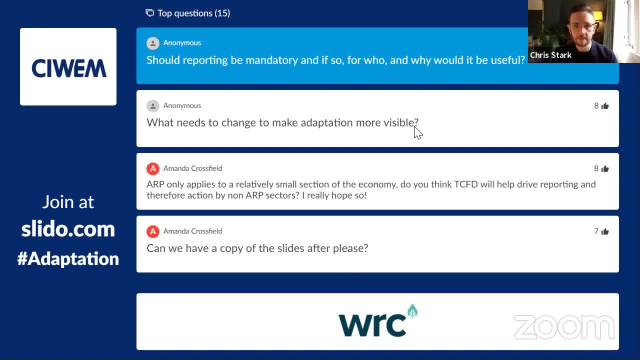 government and to citizens here, but also to the reporting organization. so it needn't be as this burden that it's sometimes framed up, as if um, if it reveals those kind of benefits to the organization as well. so yeah, i do think we need mandatory reporting. we'll be in a better place. 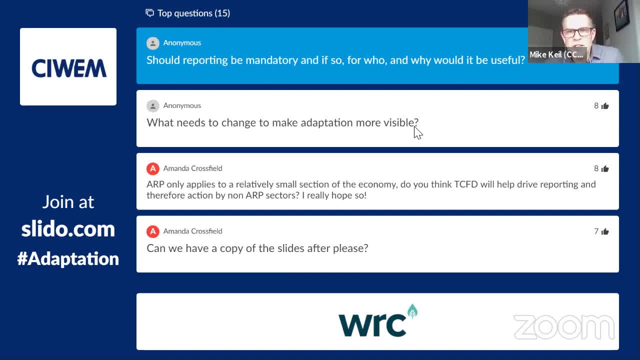 at the end of it. yes, thank you, harry. can i just chip in there? is that? is that okay? um, okay, sorry, yeah, just on the mandatory reporting: we've we've long been supporters of making it mandatory. um, it's bizarre in the water sector that you have, well, some water companies. this is true, this isn't. 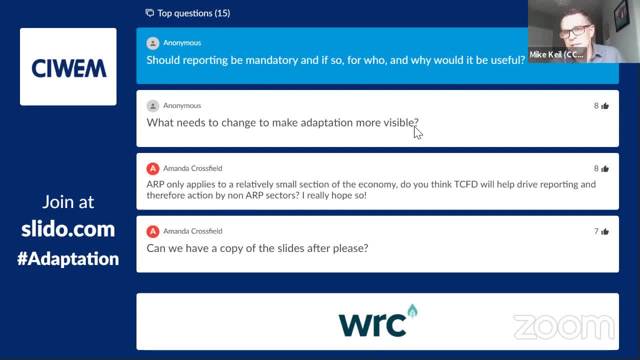 just made up. some water companies will have all of their business plans. they submit to all thought that climate change is our number one thing. they've got to spend all this money on adapting and then they'll go. now we can't be bothered reporting because you know, uh, it's not seen as 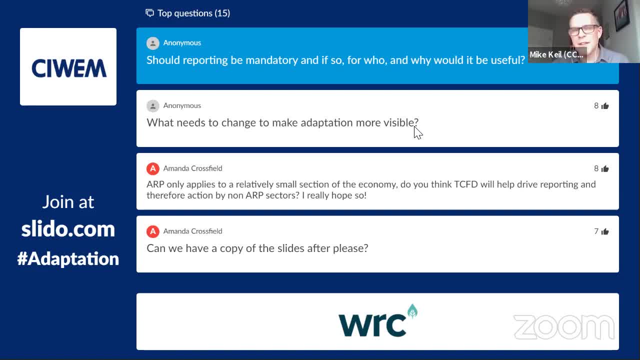 important enough, you go: oh, it can't be both, you know. so i think we just need to. i mean, the phrase that chris used earlier in different countries was: get real. i mean companies need to get real. it's either important or it's not. and if it's important, then make the difference between the. 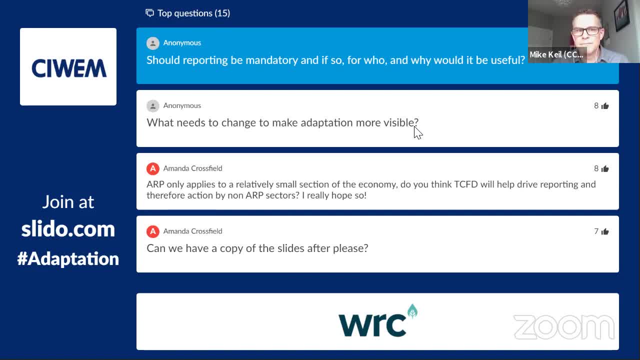 most of the reporting. absolutely the enlightened businesses that i talk to um see the benefit of of the reporting um directly to their business, the sustainability of it and and things like shareholder value as well. you know, it's um, it's uh, it's pretty clear examples out there, i think. 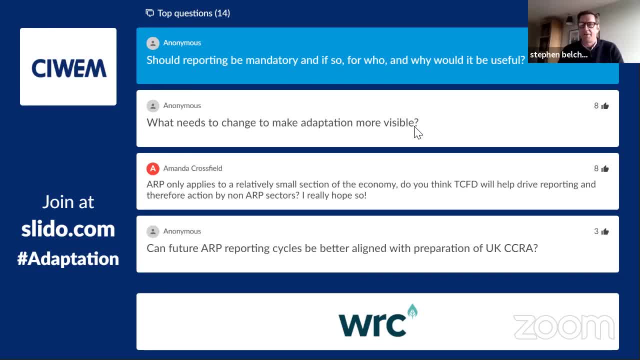 um, stephen, you wanted to come in as well, please. yeah, thanks, terry i i don't have a view on whether it should be mandatory or not, but, um, chris and mike have both mentioned the co-benefits of doing this and it just seems like a basic stress test of a business, particularly utilities business. 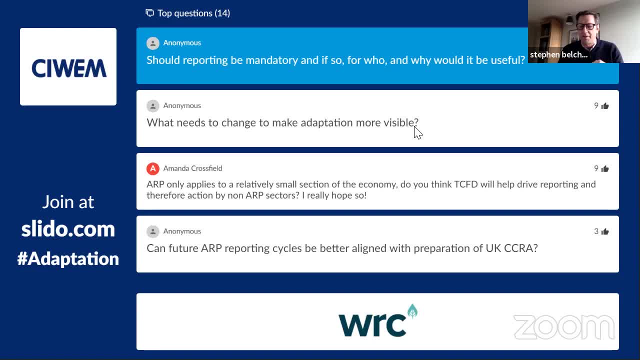 that has such broad exposure to to weather and climate hazards, it feels like good practice. the tools, as i think all the presentations this morning have demonstrated, are there for an analytical approach. um so it it feels like this is the right time for folk to be having a having a good go at this. to me, yes, thank you, stephen. 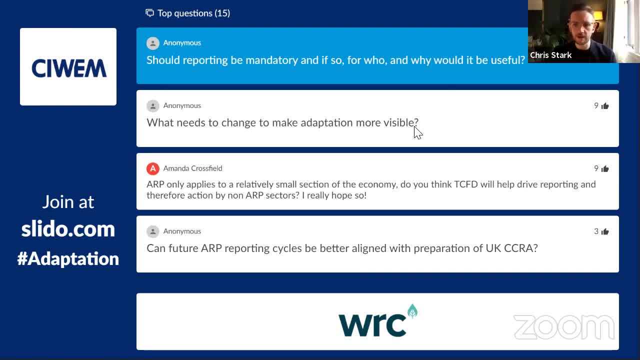 okay, it might be worth talking about tcfd as well. at this moment i don't know whether that's something. yes, yes, i. yes. there was a related question around the um, the task force for um, climate related disclosure, and whether that um is a, um, a driving, you know, factor for for us um. 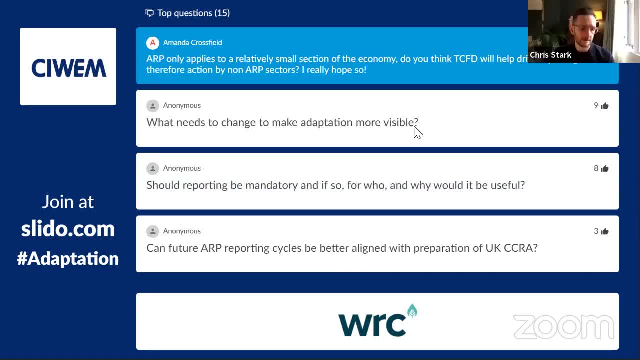 can i just go to francis? perhaps on the previous question, then we'll come to you. sorry on that. no, thank you, francis, would you? that's i? i think, um, you're just kind of echoing what stephen said. there's, there's definitely that benefit to reporting, and i think that's really. 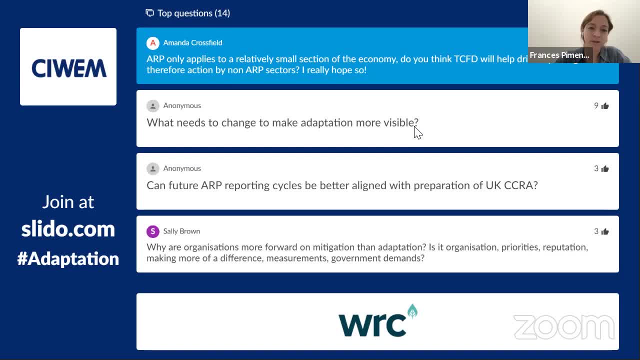 come through strongly in this round, even though um technically, organizations were reported, invited to report, and the numbers in terms of those who've committed in fact are not that much lower to um than that kind of initial um mandatory round. so i think that's the real kind of takeaway, positive. 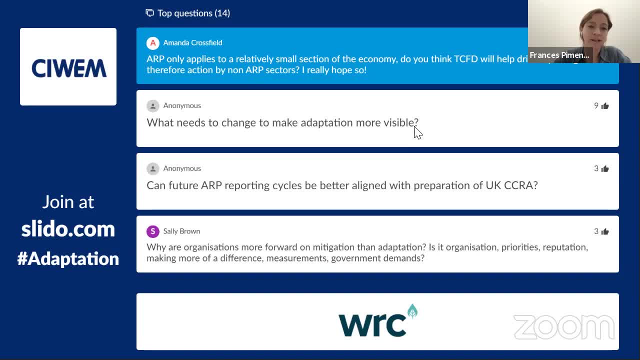 for me, we're heading in that direction. organizations are recognizing the need to take this really seriously. so i think that's kind of where where things are and, as chris mentioned, we've got other things looming now with tcfd and i think it organizations one way or another will recognize that this is something that 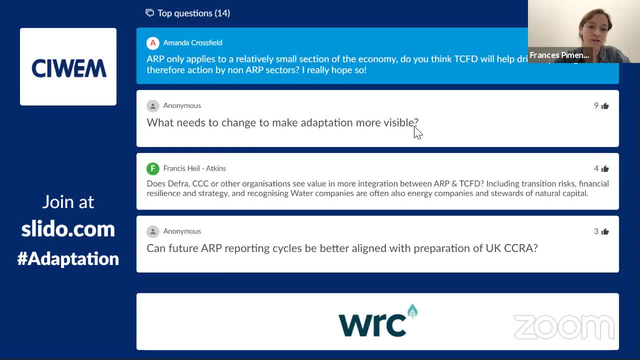 needs to be um, captured and reported on and the key part of business as usual operations in in our big organizations and indeed every all organizations. thank you, yeah, uh, so we. yes, tcfd has been mentioned. the question is: will it help to drive reporting and therefore action by? 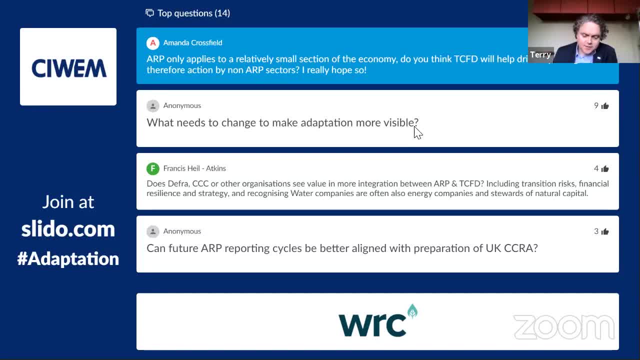 non-arp members, and tcfd is the task force for climate related disclosures. um, would you like to comment on that, chris? yeah, i was going to make the point that uh, francis, from uh francis health matkins, has just made in the in the, uh in the in slido questions, that there is uh a lot to be. 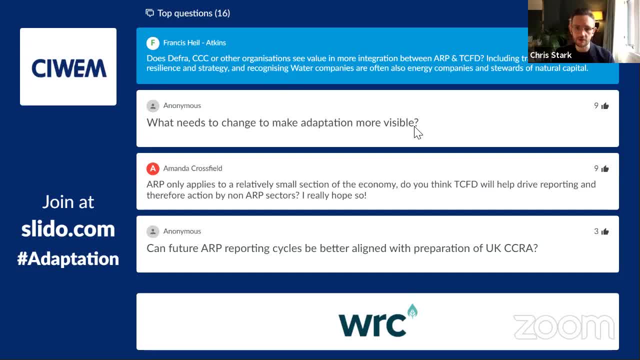 gained from trying to integrate the um, the financial disclosure uh requirements of tcfd with um, with the, with the adaptation reporting requirements. now, they're not quite the same thing but the, the hope has to be surely that through a combination of uh, the adaptation reporting and and the, the soon-to-be mandatory tcfd rules that we're going to raise the issue of, of looking at 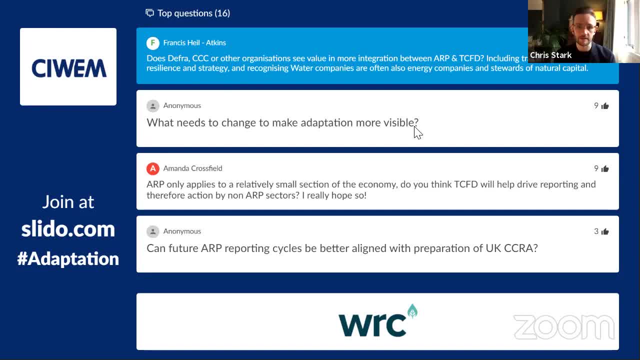 climate change in the round to the level of the boardroom, which is where it really needs to be. um and tcfd is a. it's a. it's a very complicated thing. it trips off the tongue, doesn't it? task force for climate related financial disclosure. but in reality, if you peer through that, 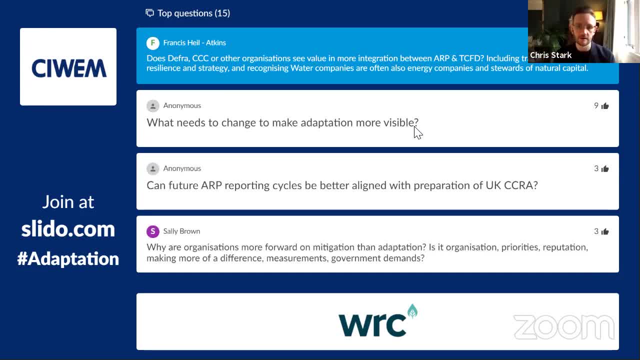 what we're looking at is the exposure of a, of a of a business, to the two risks for climate change. one is the physical risk of climate change- is what we're dealing with today, and the other one which is worth dwelling on is the, the exposure to. 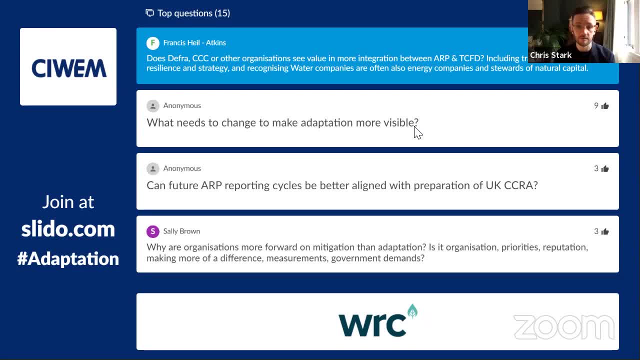 um, you know the the transition to net zero, which um many corporates are not ready for to now. both of those issues need to be tackled. they are real climate issues and i have to say that raising it in in that way, through these disclosure rules, is, i think, probably more important that many of the 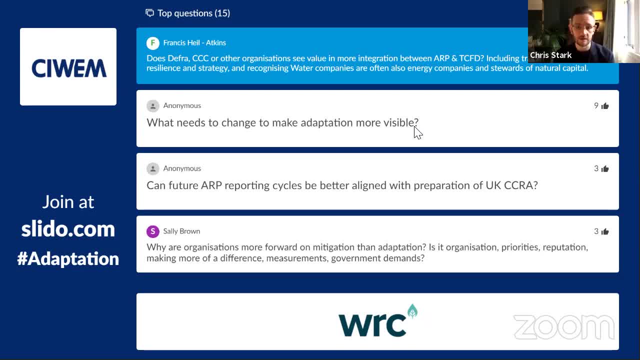 climate policies that ministers will be able to put in place over the course of the next 10 years, and so i think it's a really, really deep implication for um the progress that we'll need to make over the course of of the next few decades. so i'm very excited about it and i'd 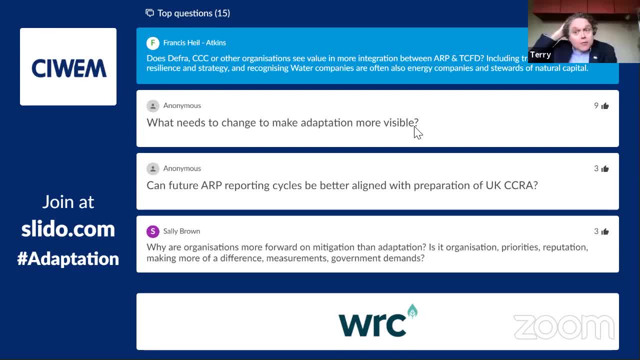 really wanted just to make the point that we should be bringing these things together as much as possible. yeah, thank you. okay, look, we're very rich on questions and very poor on time at the moment, so i'm going to um, move on um to, uh, actually the top rated question that we've had. 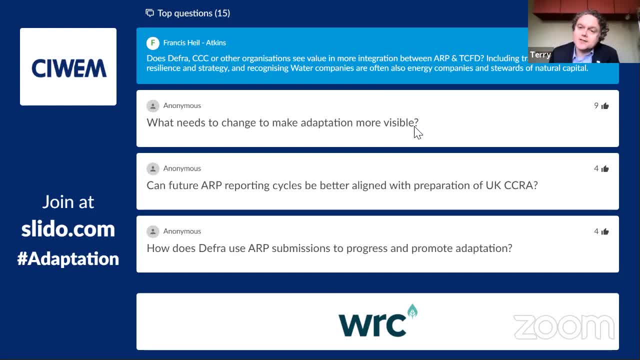 so far this morning, and, uh, this is one that will chime with cyweb's director of policy, who is the poor relation of, of mitigation in terms of climate. uh, addressing climate change, um, and so the question is: what needs to change to make adaptation more visible? who would like to? 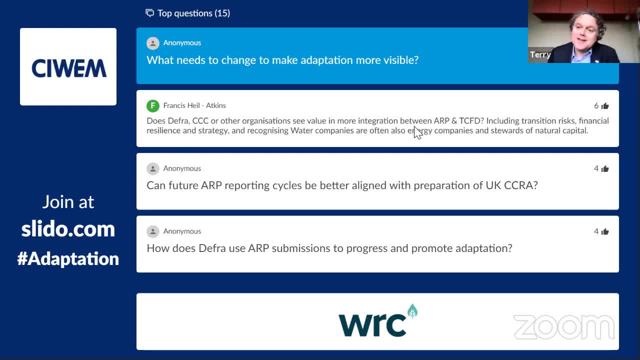 address that first. yes, yes, please, steven. yeah, i mean i'm sure others will have a view on this- the the mitigation target is very straightforward: right, net zero. it's very easy to state, probably rather hard to get to, and charting a path to that is difficult. um, what good adaptation looks like. 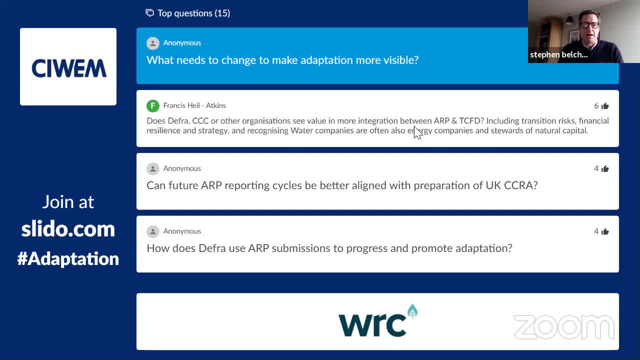 is much harder to define, maybe, um, but, as as we discussed this morning, it's really the richness of this that makes it so compelling and so important to really embrace properly, because it it's part of how we, in any of our operations- and i would include the met office in this- 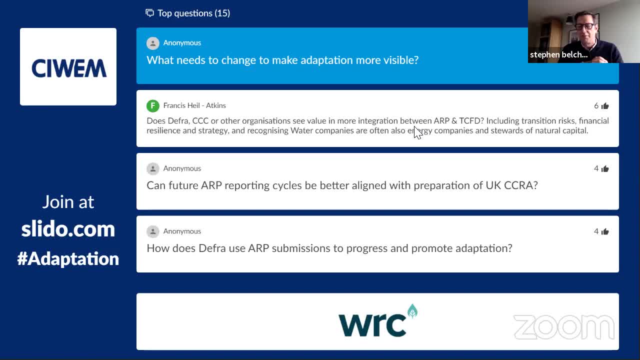 are going to perform both now and a resilient way, but also in the future in a resilient way. so it's part of that resilience building um thing that any any business um would want to go to through. i would think um how to make it more visible specifically um. i think the climate change commission do a great job. 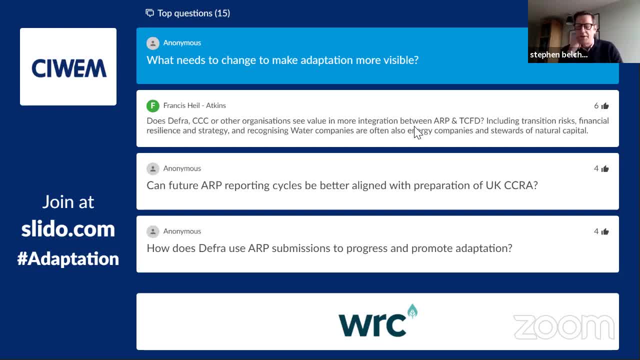 in in driving this draw track and- and i think there's more that, uh, the rest of the community can do- to just make sure these things remain part of the same sentence. so the catchphrase i would advocate is: we talk about a pathway to net zero. how about a pathway to a resilient net zero? and 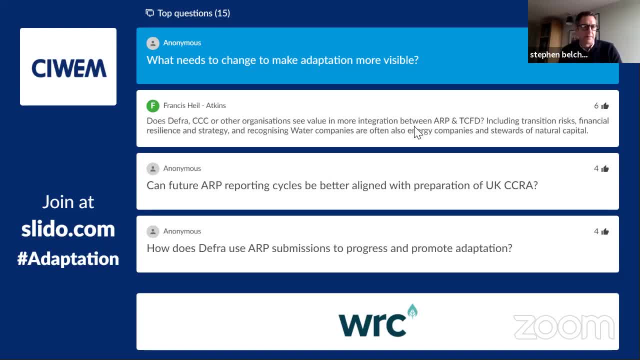 let's talk about the word resilient a little bit more. yeah, thank you, steven and mike, please. yeah, i mean i think we can also work harder to capture the attention of the public when it comes to adaptation. so, for example, people love seeing infrastructure and like seeing images of big. 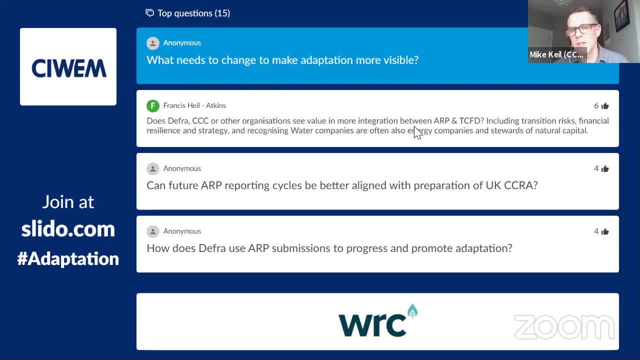 things, impressive things. you know, temps have done a really good job recently on showing images of the fatberg that they clear up and they're not going to be able to see the images of the fatberg- um, whilst that isn't climate change adaptation, but people do like seeing, you know, pictures of. 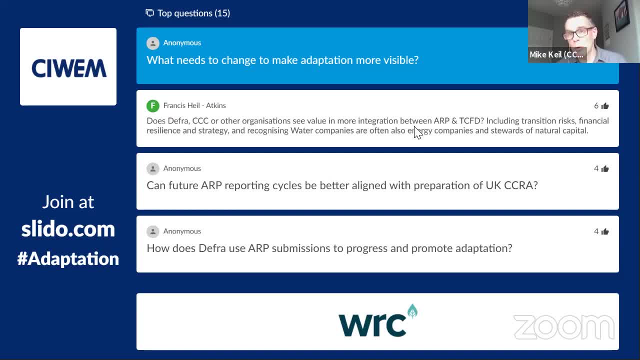 infrastructure, and actually it's not just about showing what they are doing, although what that actually can help capture the imagination. it's also getting people involved in the projects themselves because, look, it's a kind of like um consumer body Tourette's to say, oh, you should. 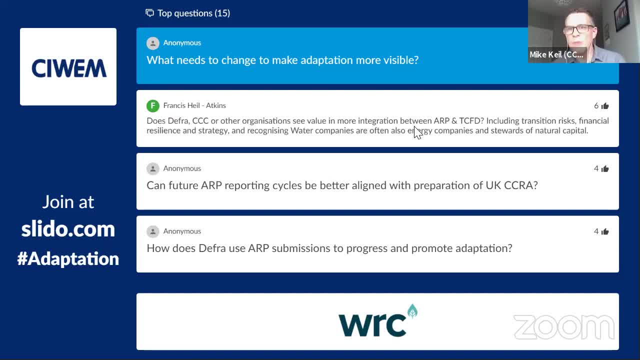 consumers should be engaged in everything. yeah, absolutely shouldn't be involved in everything. they should be involved in things they can have a meaningful saying. but do you know what? there's loads of big infrastructure where there's still meaningful choices, where communities can get involved to actually influence, and that way you can really connect to. 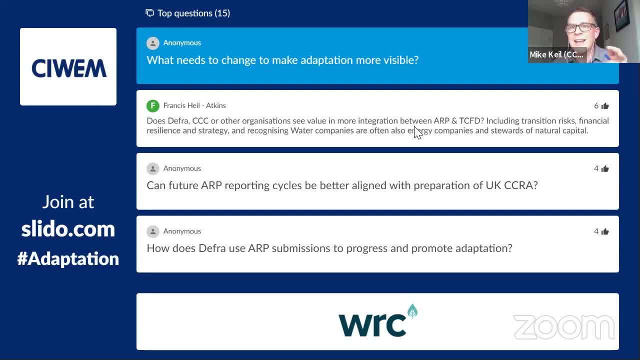 people and you know what that presents huge opportunities to then say, actually, have you thought about doing this water efficient stuff in your home? have you thought about what you chucked in your toilet in terms of sewer misuse? so actually that wider community engagement um is really important. there's been some really good work done in the water sector, but there's 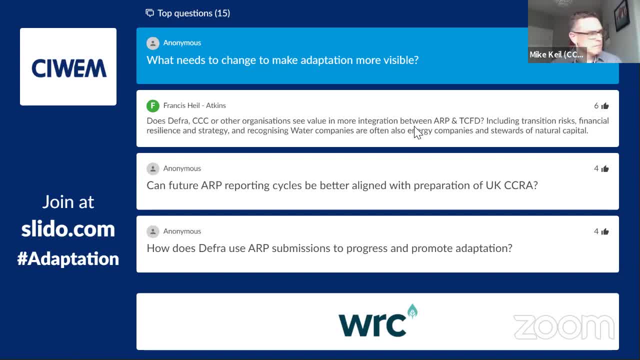 tons of untapped potential here. yeah, thank you, mike. okay, we could talk on on about that, but i'm going to try and squeeze in one last question very quickly and just ask for a round by answer from from each of you, if that's at all possible. and the question is: has anything? 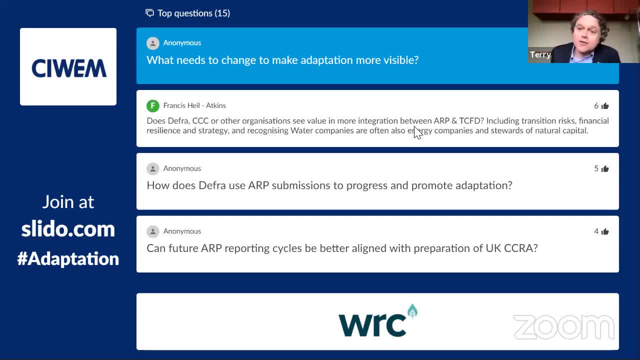 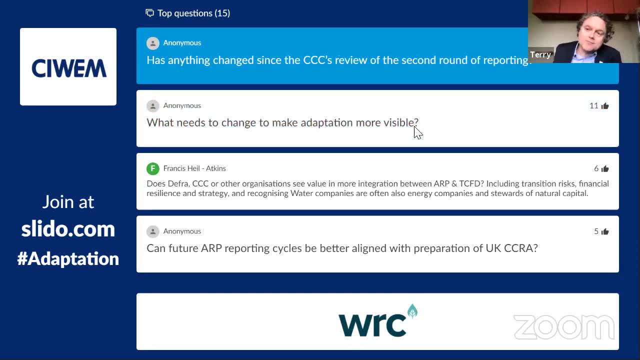 changed since the ccc's review of the second round of reporting, or rather what has changed? perhaps you could answer it that way as well. so just quick sort of one word, one sentence answers, please, from each of you. if i can, um, mike, go for you first, i'll come to you, chris then, not enough. 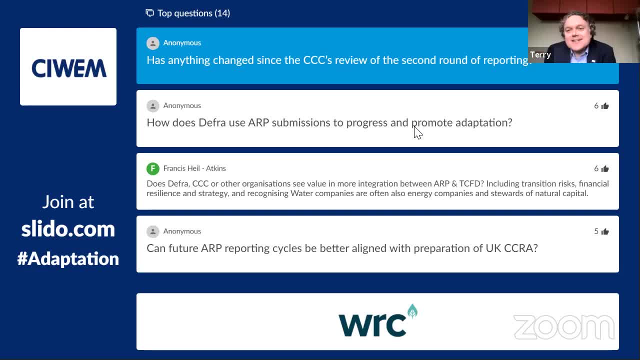 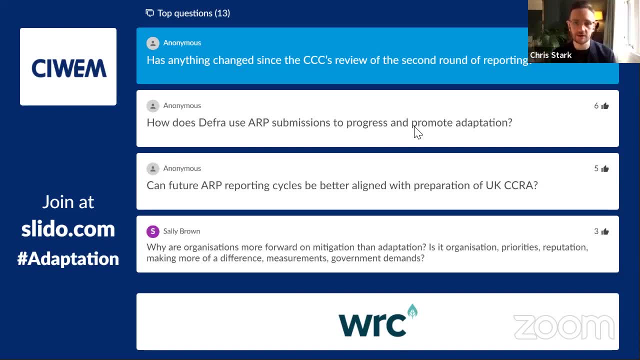 chris, yeah, we've got better at assessing, so that's one thing, that's got, that's uh, that's improved and um, and i think there is a general much, much higher awareness of the issues, which i think is helped by the net. zero stuff, uh, but of 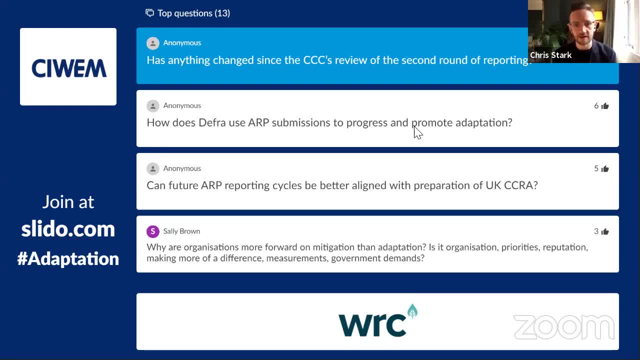 course we've got to move on from that into. i firmly agree with what what steven and mike said in their in their last replies. so so not enough is a very good answer to that question, but we're in a better place to improve things than we were at ccra2. that's a really good and hopeful thought. 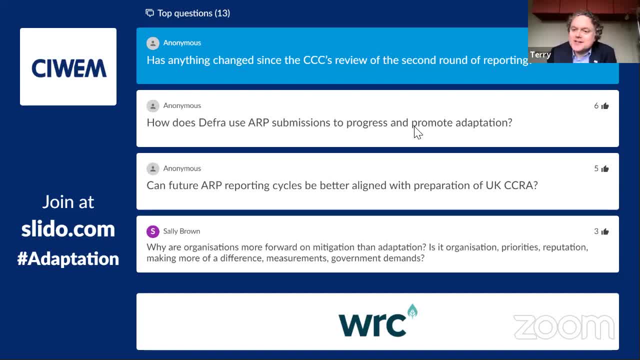 uh, anything else to add at all from you, steven, or francis? no pressure, the ccc's review provided some really helpful steers for the third adaptation strategy in terms of big questions of interdependencies on use of evidence, as well as a sectoral led. 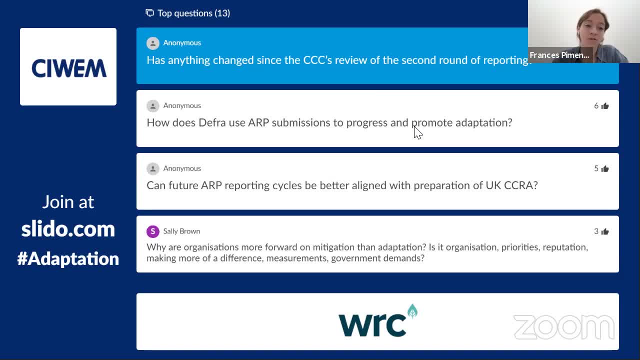 conversation. so i think all of those things have been really crucial areas of progress from what i've seen so far of this round. so so good and more to go. yeah, well said. thank you very much, steven. you get the last word if you want it. i'm not sure i have anything very profound to say other than that this event, as as really i hope- 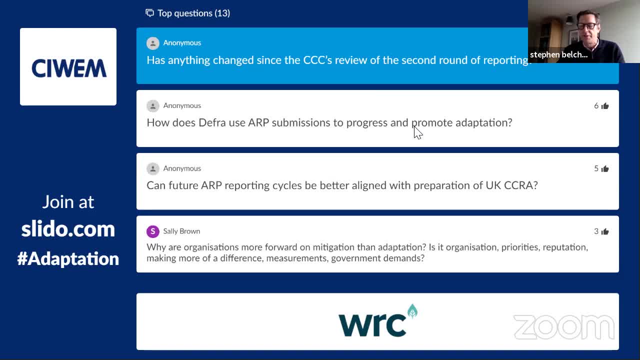 going to galvanize some thinking around this, and it's been great to be on a panel with such a rounded range of views. yeah, thank you, and that's what i would say. actually, it's great to be on such a well-attended event and we are at least having this discourse. that surely is is progress. 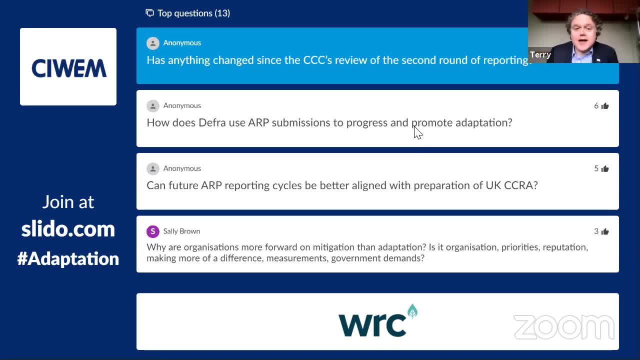 okay, right, let's move on to the next question. so, steven, you've got a question from steven. thank you ever so much to all of our speakers this morning. um for that, um and the quick five questions. um, we will be capturing these questions, they won't get lost and we're going to help to. 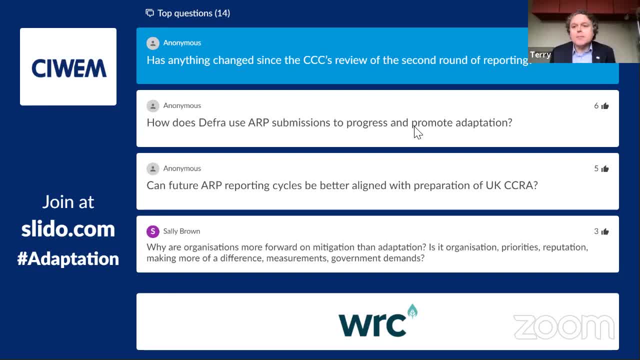 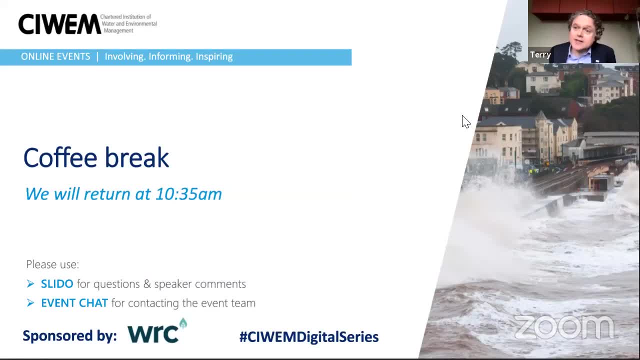 sort of use them in the um, the output from today's event, but that's all we've got time for at the moment. we're going to have a five minute break now, so i'll make that 10, 36, please, just to kind of stretch your legs and and we'll get started with them with part two. okay, see you then. thank you. 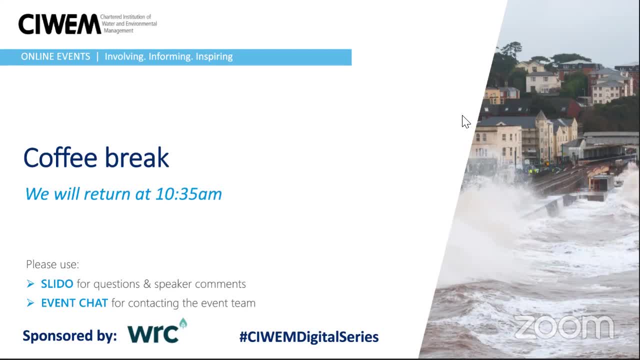 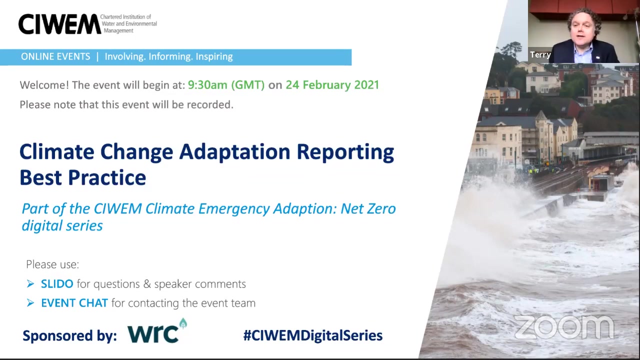 you, you, you, hello and uh, welcome back everybody. i hope you had an opportunity there to stretch your legs and maybe even boil a kettle, if you were lucky. um, we're now going to move on with the, the second part of our webinar, and this session will be a bit different from the previous one. we're going to 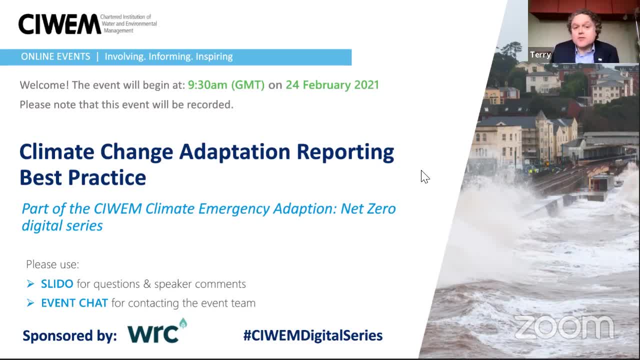 start from the first um. we've got six experienced reporters from different sectors, from regulators, finance, water and infrastructure, and we're going to give them each three minutes to impart their wisdom on how to get the most out of the arp process, how submissions can be used to prioritize. 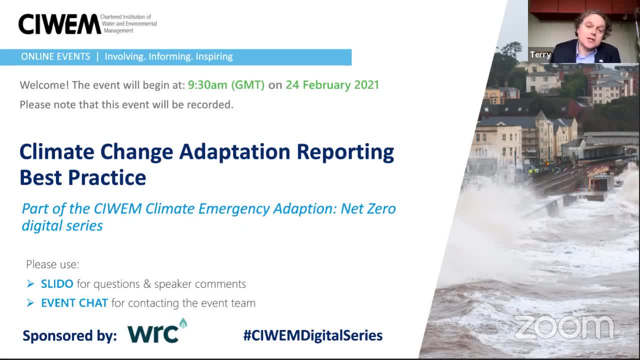 adaptation and how it's been used to mobilize change within organizations. and, after all have spoken, we will go to your questions to them, so please do get slidoing during these three minute slots. it should be quite frantic, but let's get lots of questions coming in, please, um, and we'll put them to the panel at the end of the 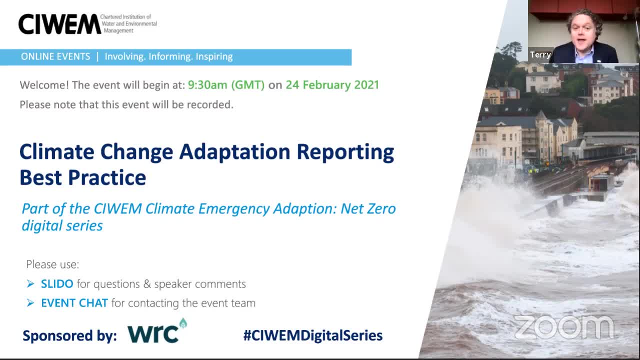 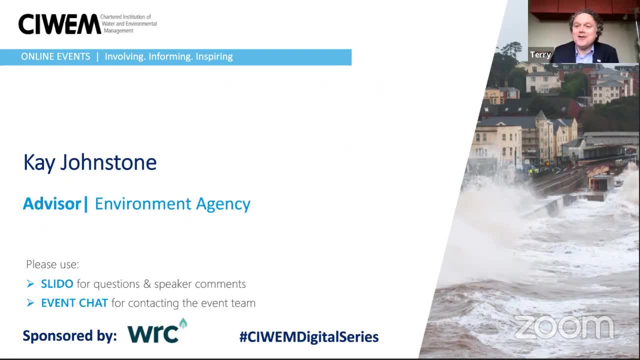 session. so first up we have k johnston from the environment agency. i'm really hoping that you're there, claire, somewhere. yes, you are okay over to you, thank you. hello everyone. thanks, terry. um, yeah, so so much has changed since we first did our first report back in 2011, both in terms of the public and political discourse on climate change. 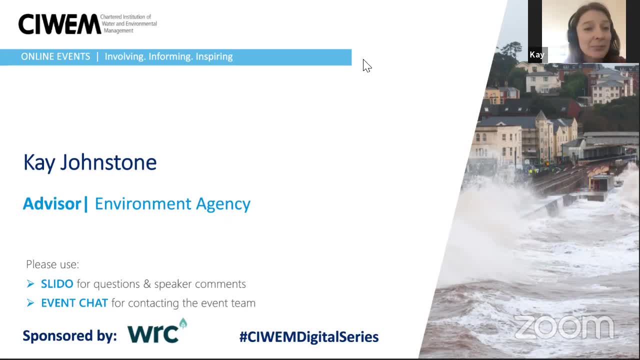 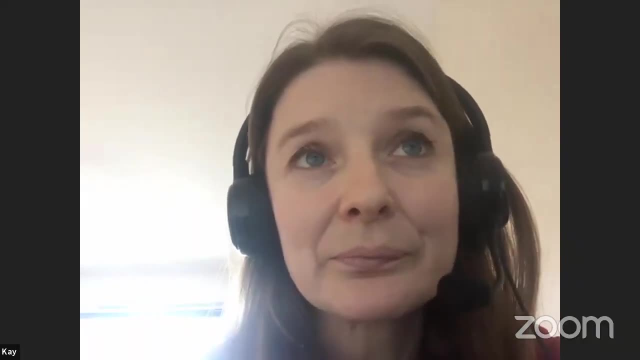 in general and also developments in evidence and practitioner experience on adaptation. and the preparation of our third report now comes at a time when the global response to the coronavirus crisis has demonstrated a really pressing need to work together on um to share solutions to overcome global uncertainty. cop 26 hosted the 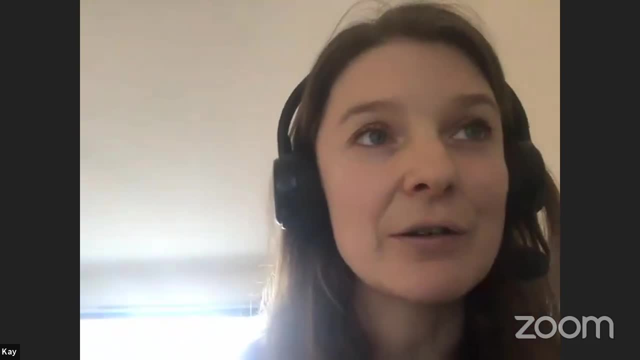 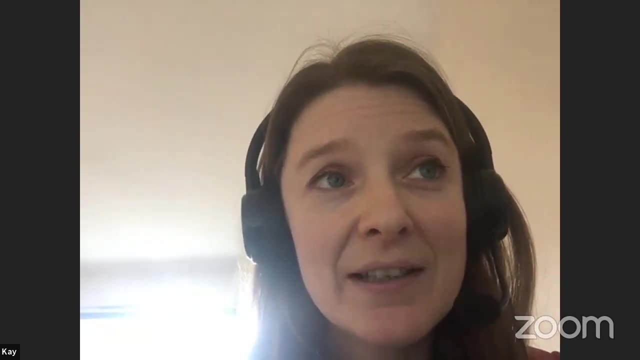 climate change crisis in the last year, of course, is certain to shine a light on progress that we're making in this country on climate change, and the environment agency manages risks on behalf of the country through our roles as regulator, advisor, operator, flood and other assets and, as such, we 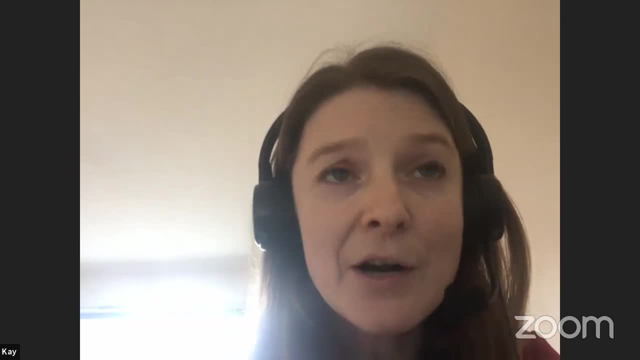 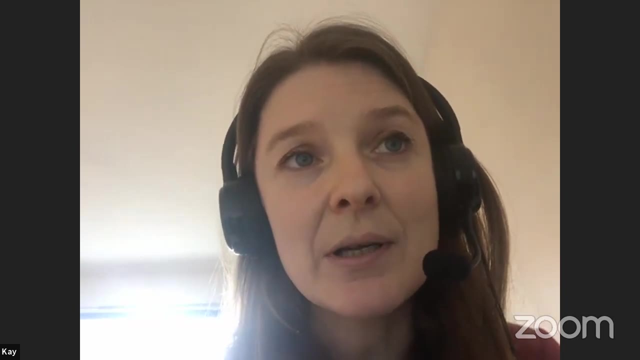 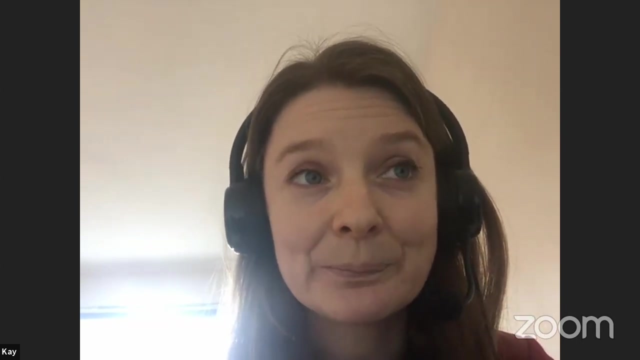 operate within quite specific policy and legal frameworks and our report can't be abstracted from these. these have also matured in recent years with respect to their um treatment of climate change adaptation and experiences. what are the possible implications of them? So thank you very much for joining. 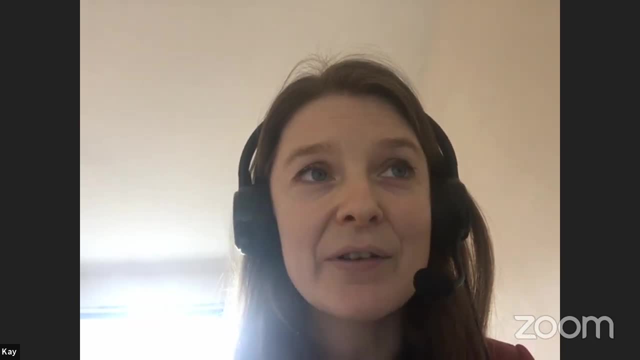 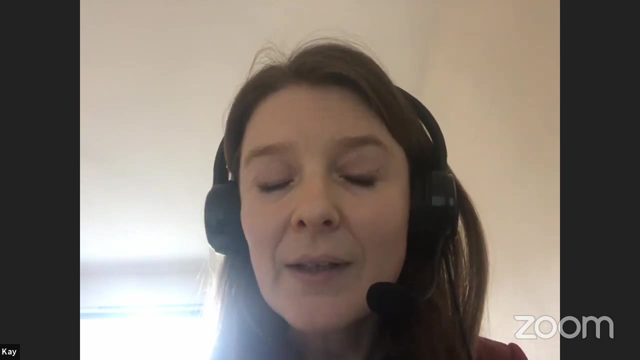 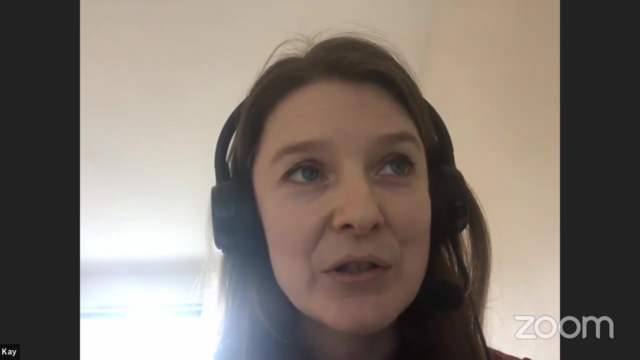 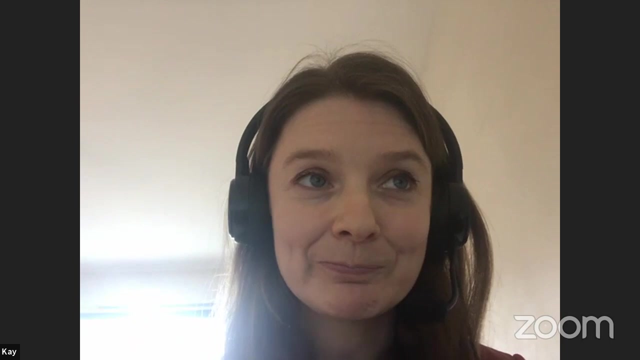 me today, mel at the University for climate change has water options, our inclusion on your back environmental plan and the flood strategy, which has climate change both as a top priority and also as a visible thread throughout. So our third report will put more emphasis on long-term adaptation. 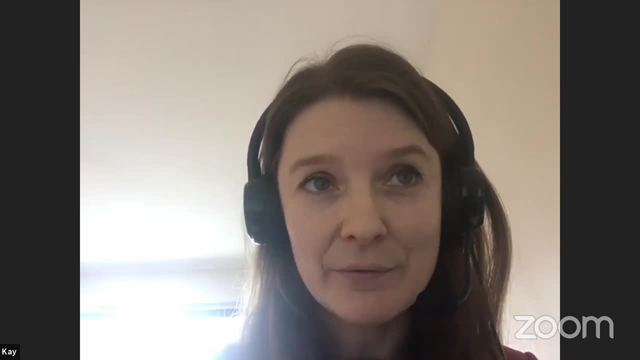 strategy. It will set out how we are preparing for the full range of climate futures, including some high-end scenario, how we are embedding actions across the organisation and how we are planning ahead for areas where a step change or more transformational adaptation is required. 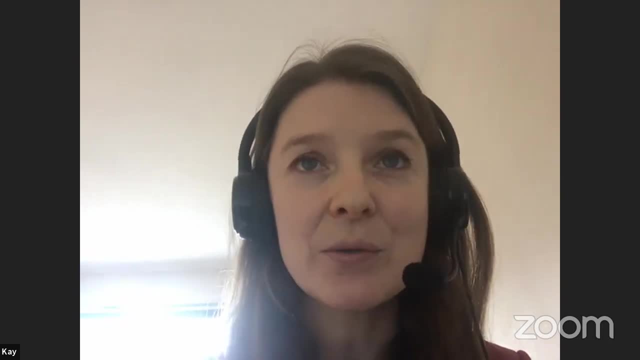 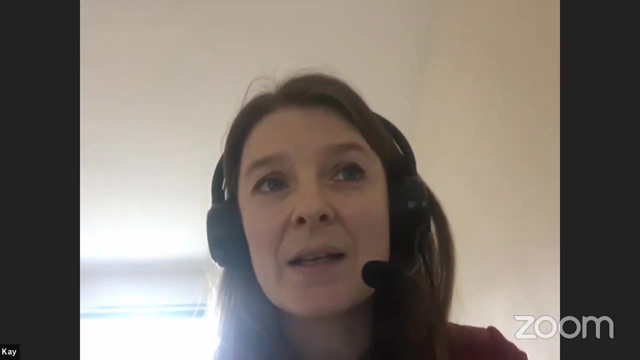 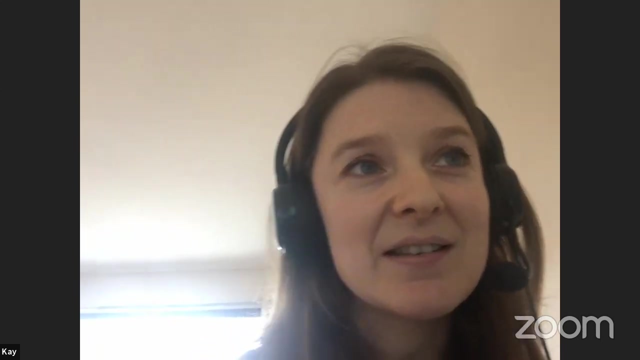 In our third report we are building on the risk-based approach that we took previously, but we've also introduced the concept of urgency to our scoring methodology, alongside the familiar severity and magnitude assessment. So this is looking at the time needed to respond versus the time that we have to respond in order that longer-term risks that are still urgent are. 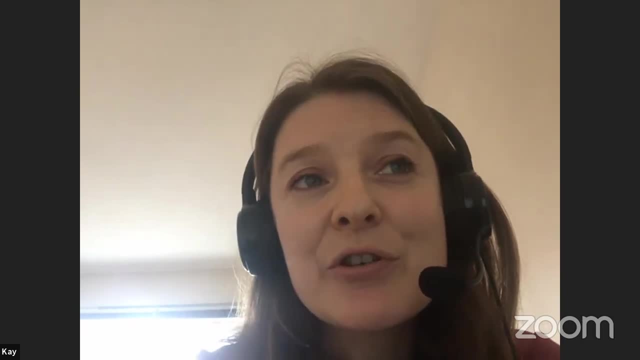 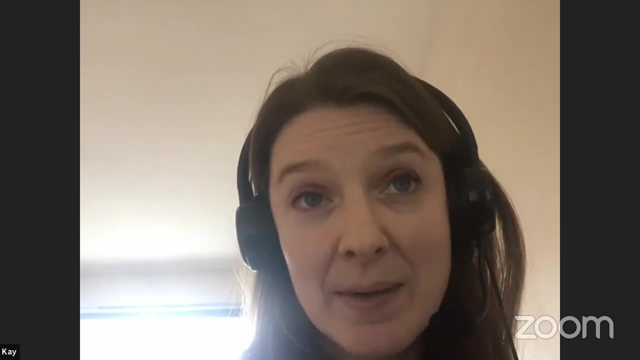 not deprioritised. So we're hoping to produce a report that will resonate across the organisation and externally, showcasing our ambitions for tackling some of the country's biggest climate risks and setting out our strategic direction on adaptation. We're planning to be quite open. 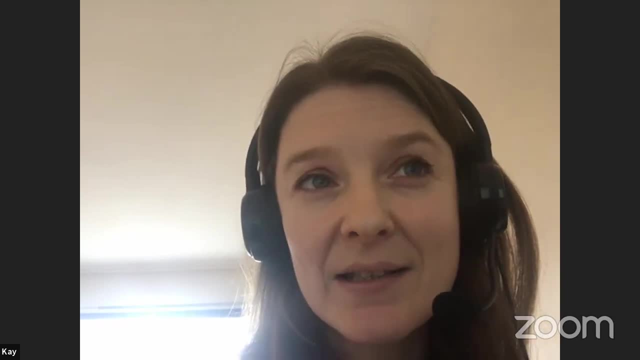 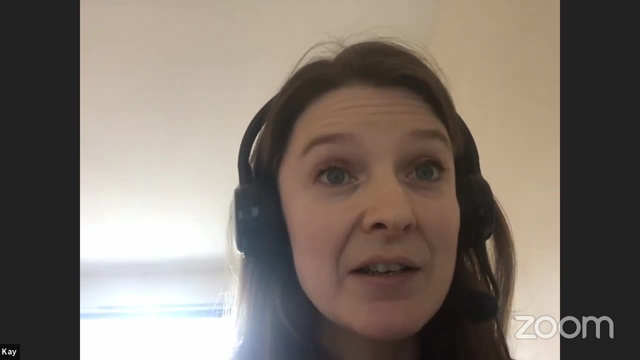 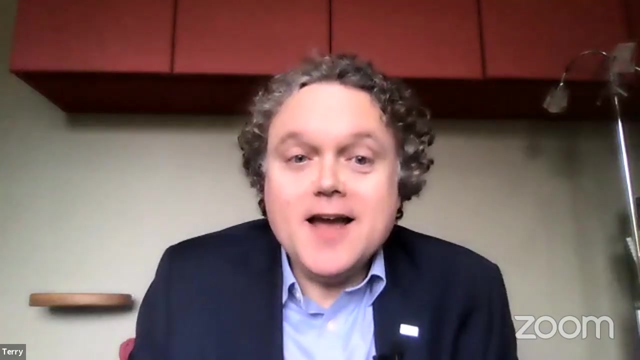 and honest about where the future might hold, limits to current approaches and limits to what we can do alone, so that we can use the report as a means of challenging both ourselves and others in support of bold action. Great, Thank you very much, Kay. Moving straight on now to David Quincy from Network Rail. 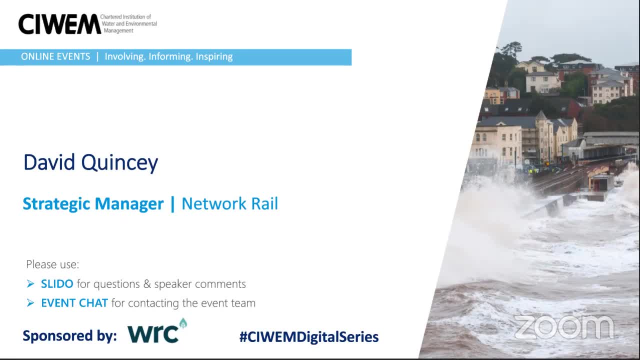 David from Network Rail, Are you there, Right? I think we may have lost – no, David's back. David, can you hear us and can we hear you? Yeah, I'm in a truly resilient fashion. My phone is ringing out. there There's people. 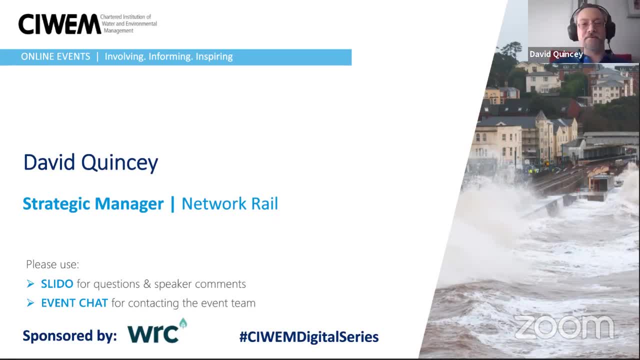 shredding a tree outside my window that I don't know if you can hear, and I've just got kicked out. so let's just go with this show. Timing is everything, isn't it? Yeah, Off you go, Okay, Right. So I have been involved in adaptation reporting twice before, but not with Network Rail. 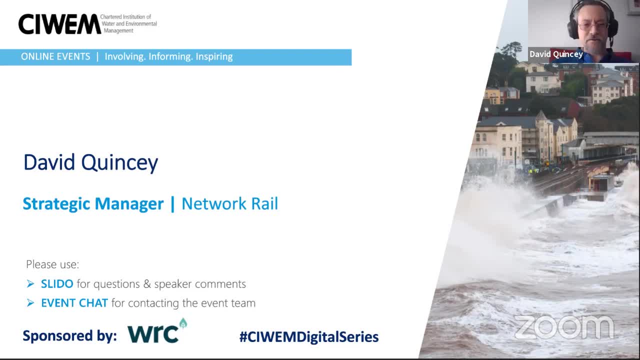 and so this will be my first time with them. So I've got some thoughts looking back at what they did last time and where we're going to go this time around. So adaptation reporting is seen as important to Network Rail. as key, It's seen as: 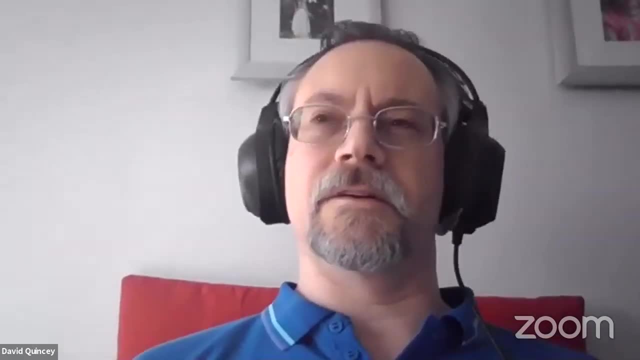 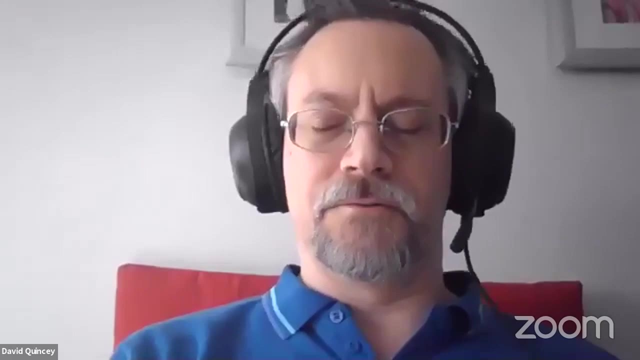 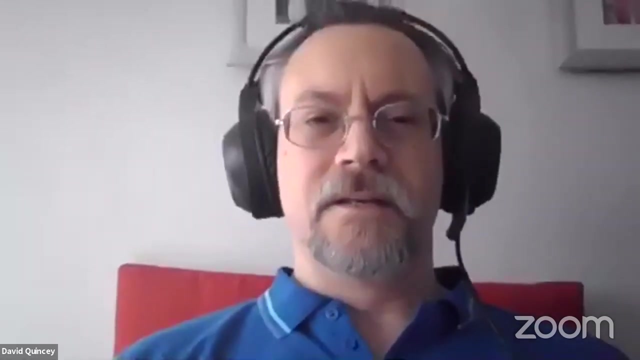 a way, as a sort of basic minimum, of an opportunity to refresh our view of our risks, look back on what we thought we'd got as risk before, see what's changed in the way of science and the and our understanding, and how and when the business has changed it. Again, as a basic, 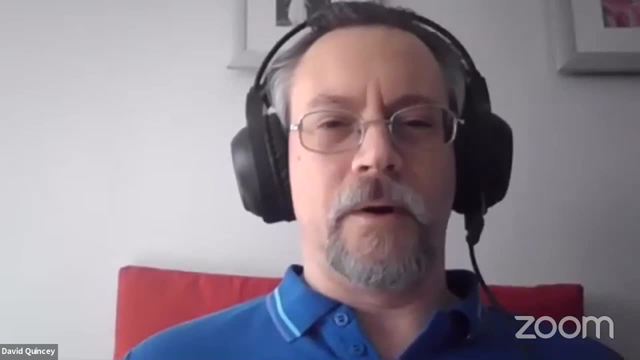 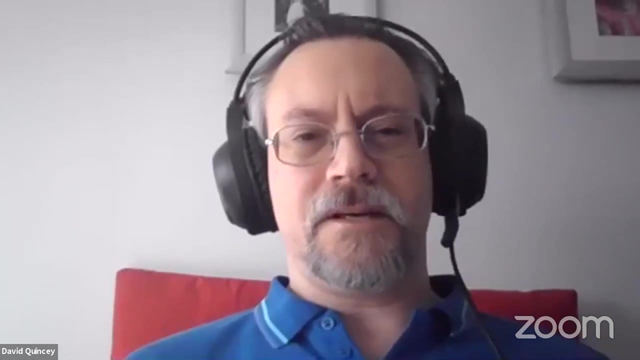 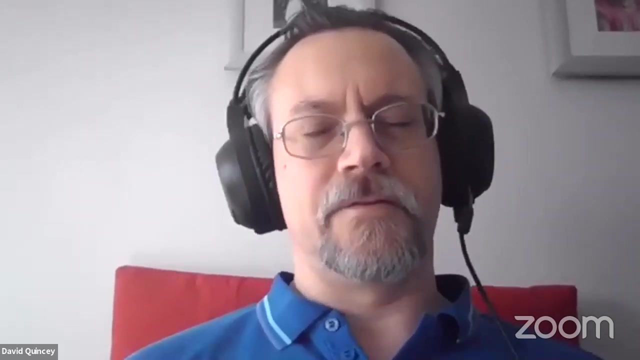 it's an ability to summarise our position: where we are, where we've been, where we're going. Historically, looking back at the previous two iterations, they had a lot of detailed weather stuff in them and an understanding of climate risk, but they were very much done from a centre. 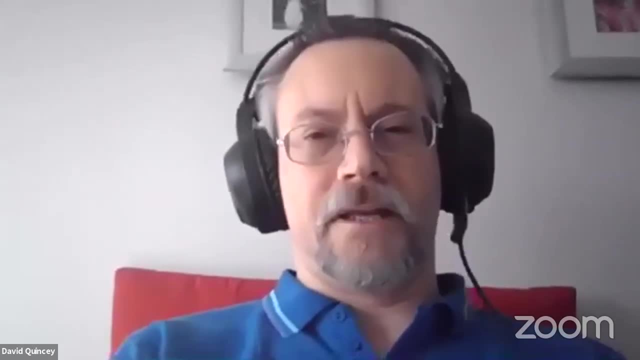 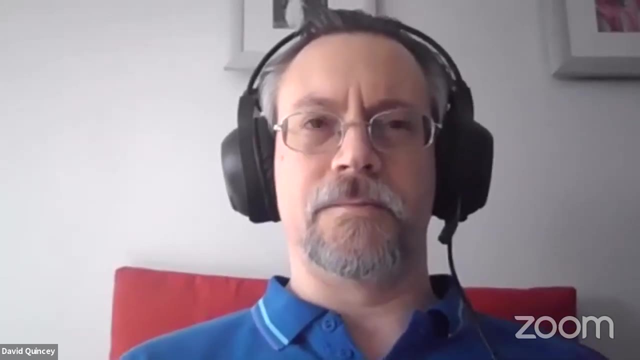 of Network Rail approach and didn't really have a lot of connection to what's happening out at the coalface. So that's a big change that we're going to see this time around, but we're going to have a much more holistic approach. We've done a lot of work on understanding our level of risk and a lot of 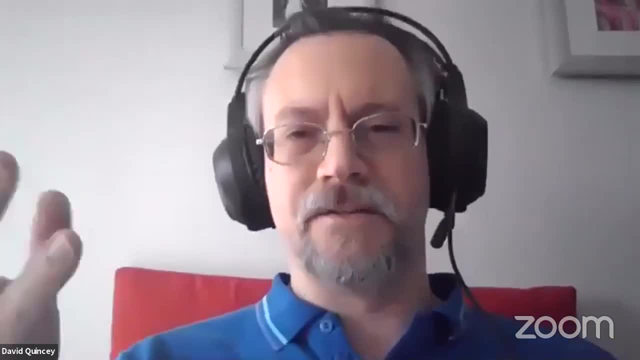 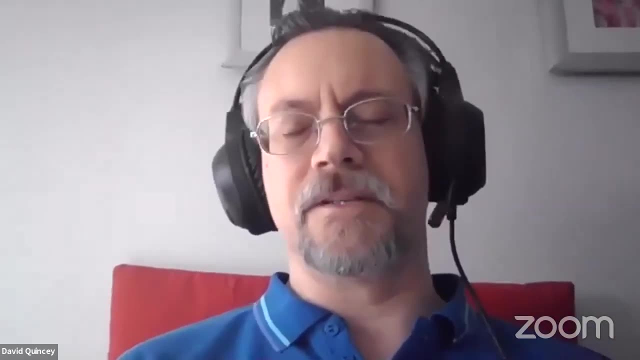 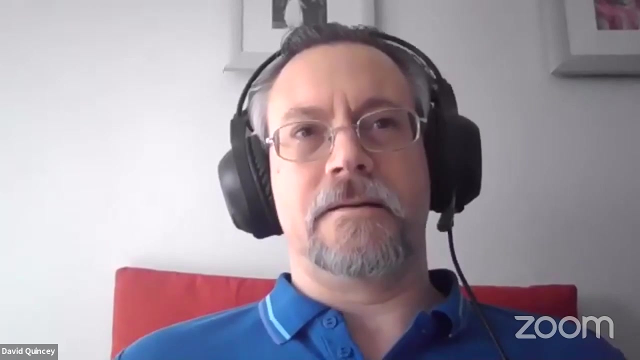 work on understanding both the weather and climate linkages in that risk. We've republished our route rack of plans, as we call them, weather resilience and climate change adaptation plans, so they will form a key backbone to the inputs of this. We have just completed an asset function. 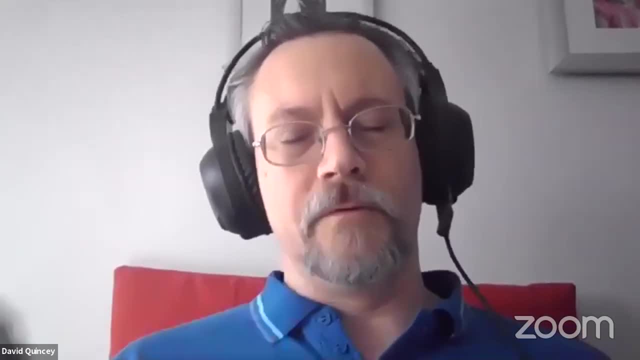 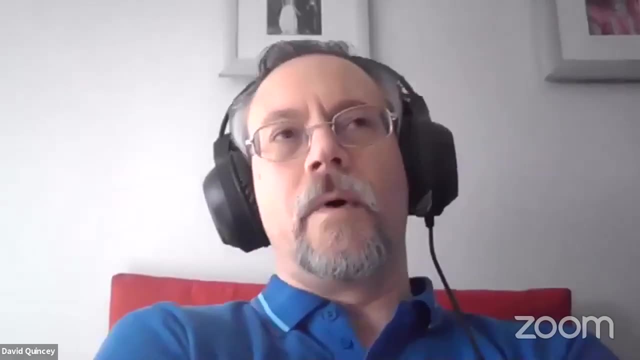 risk assessment for the first time, looking at all of our internal central asset functions and how they relate to the routes and those route rack of plans, and understanding where those risks lie and where we need to take them and enter an action plan. So again, that will form a backbone. There's 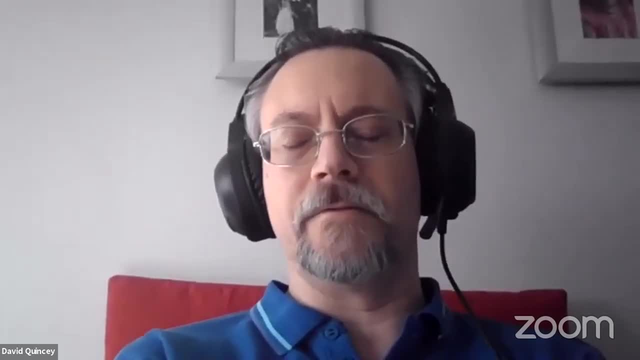 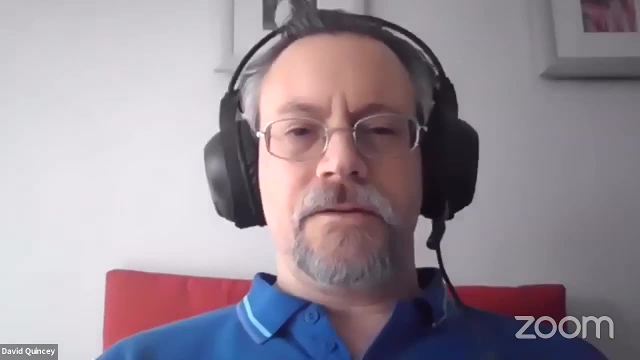 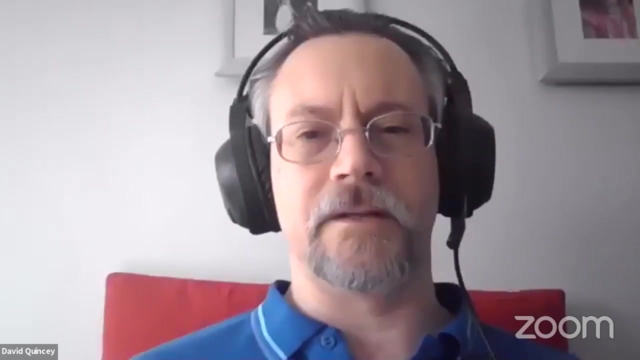 a lot of extra work to go in on this and hopefully it'll be a lot more in the way of action plan this time, rather than just risk and weather action. It's also being used as part of developing our overarching strategy and plan, which will align with our new environmental sustainability strategy. 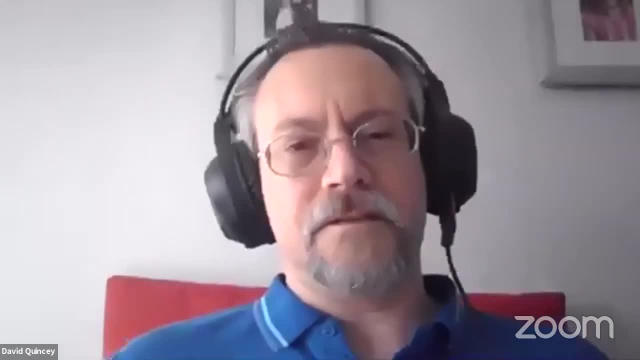 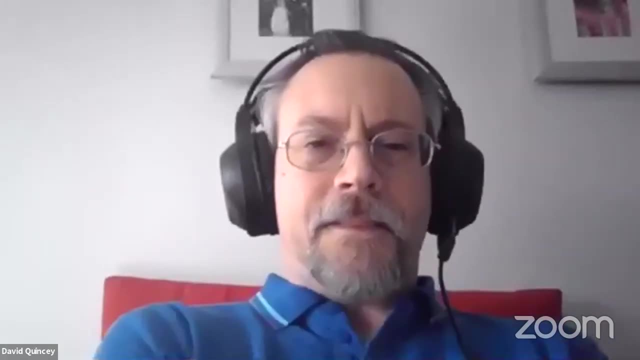 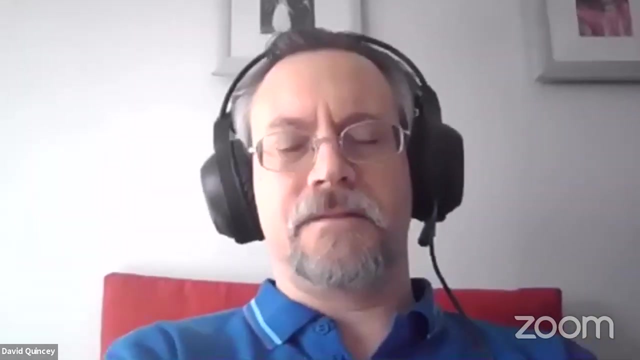 So again, that's a key alignment with our key business targets. So again, there will be a much more tie-in to the end-to-end delivery of those. And its biggest benefit to us has been engagement. It's allowed us to engage with the individual parts of the business And when we're a big 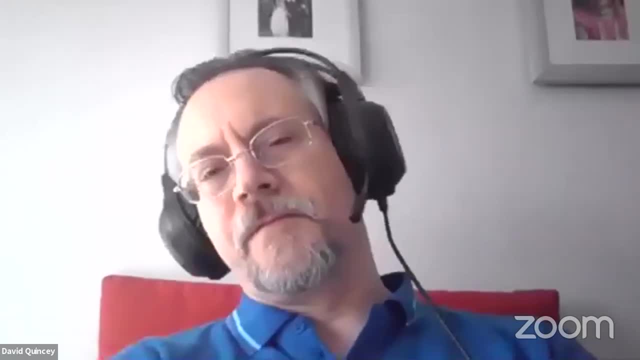 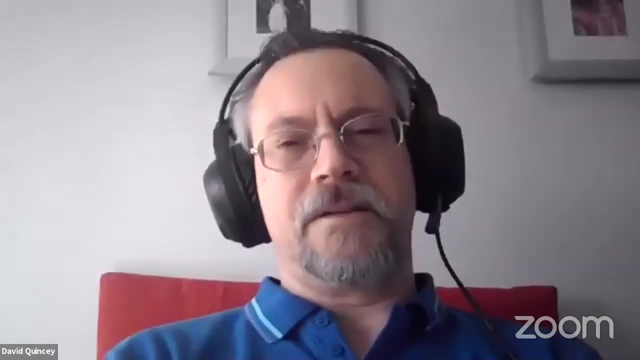 organisation like this, it can feel quite remote for us And from the top of the centre to someone on the coalface on the track. So involving the routes and developing their own plans and making those plans a central part of this process is involved, by its very nature, a lot of talking, a lot of interaction, a lot of understanding. 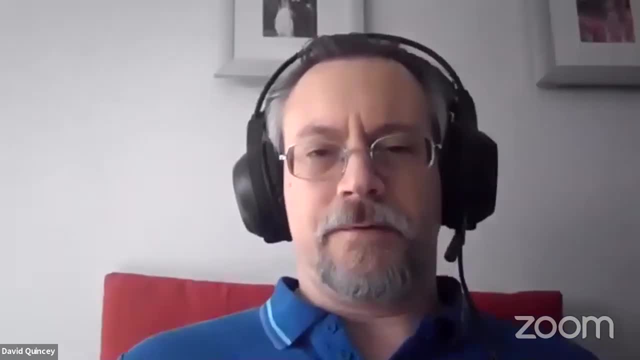 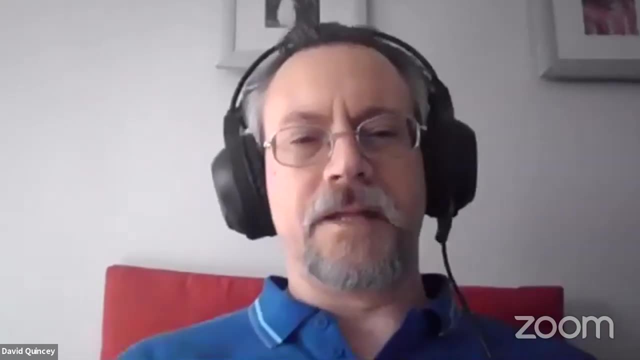 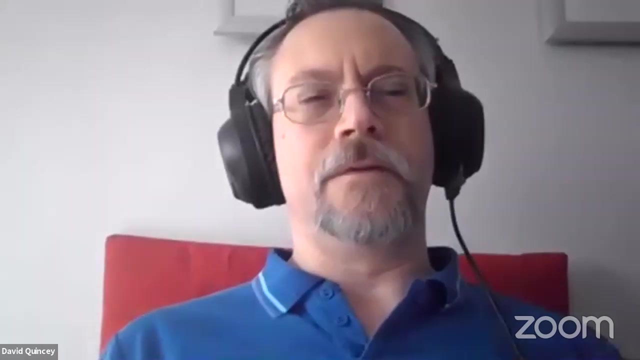 It's happened in the light of the tragic events that happened in Scotland, So it's an ill wind, but it is a timely reminder of the need for the importance of resilience, and it's put a lot of focus onto the review of where we are and where we're going. 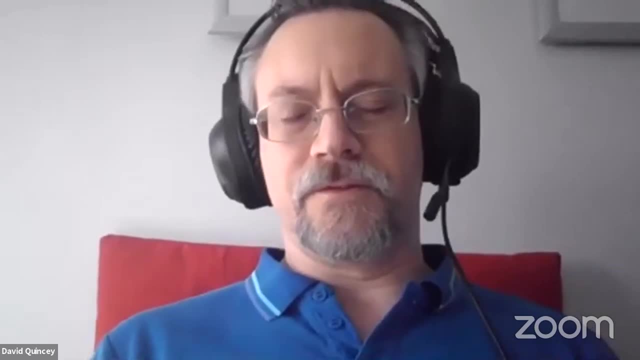 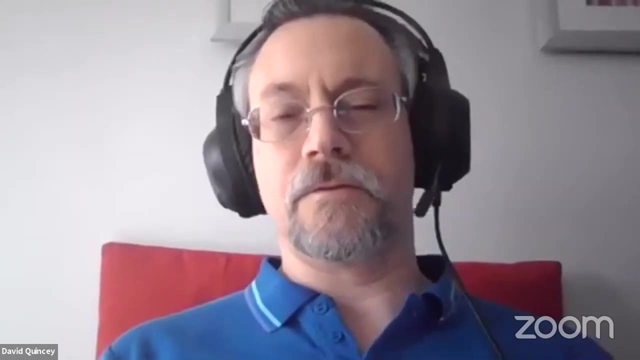 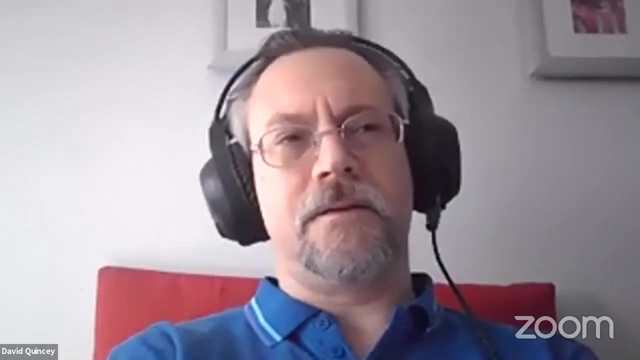 It's opened doors. There have been two big task forces created as a result of it to look at how we respond to weather and how particularly, earthworks respond to that and future weather. It will allow us to develop greater integration into our CP7, our next control planning. 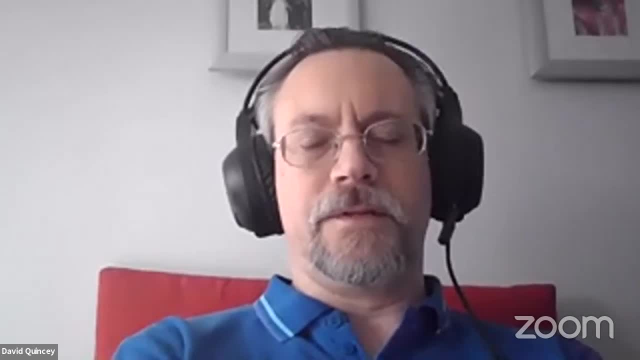 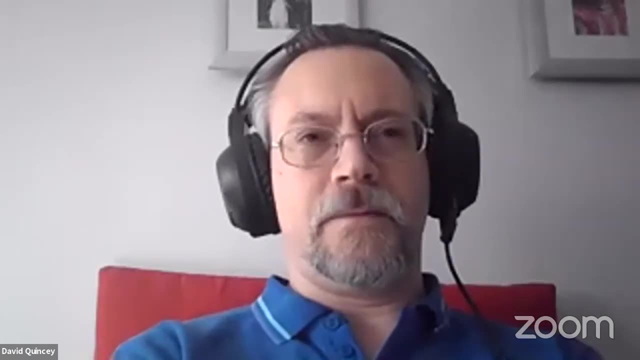 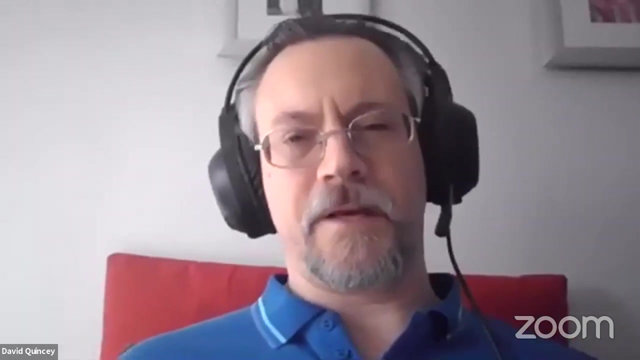 which is being driven through And again that will be reported in this report. It's focusing our attention on investment plans this time around. We're obviously aware in COVID we're in an interesting funding situation where a railway is being funded more by the taxpayers than the passengers on it at the moment. 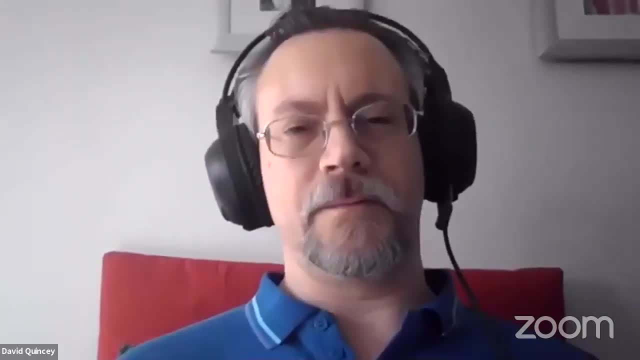 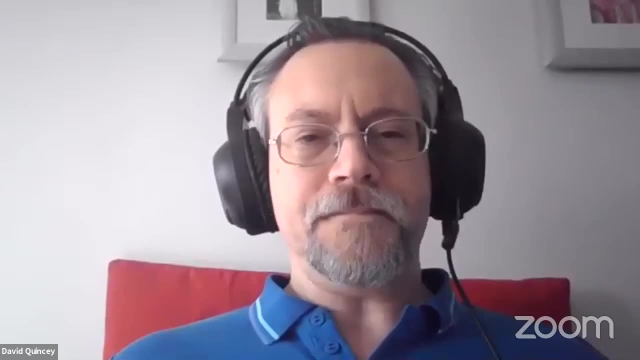 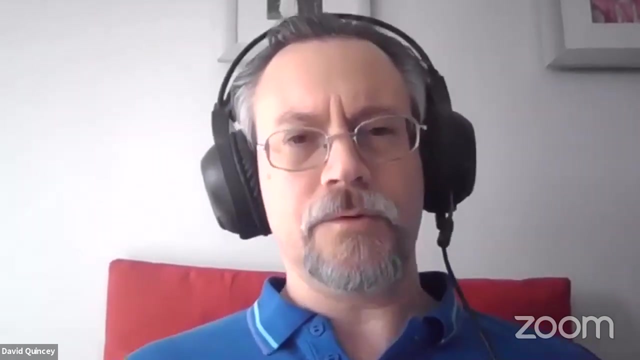 And we need to think about how to build back better. So resilience is a key part to play in that, not just to the weather and climate, to the economy. So it's all becoming a very holistic viewpoint. I think it's good to note that it's much more on the radar of our executive board. 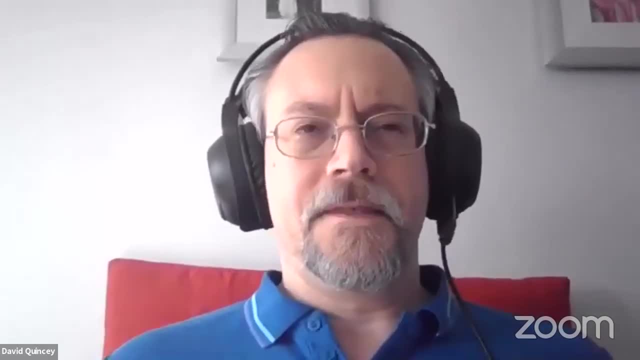 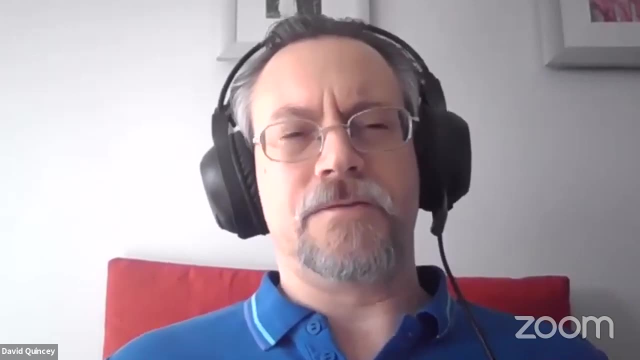 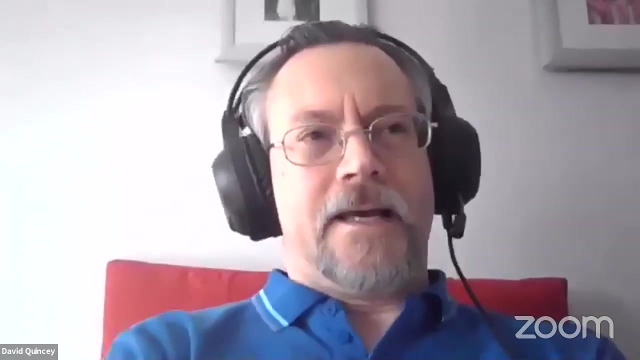 and they'll be more involved in the sign-off this time, And I think it really gives us a platform to identify the gaps we need to address over the next five years, before the next one- assuming it is five years, as briefly mentioned, and whether it's mandatory or not. And we're now into the position where we're into that long game because 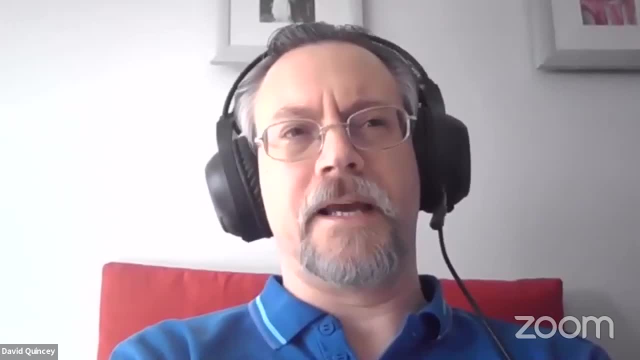 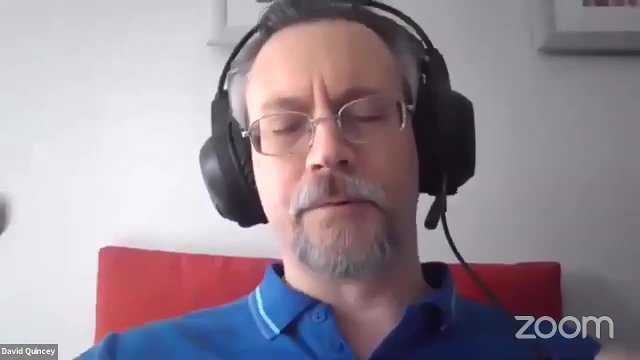 we've spent a lot of time understanding the challenges in the system, the challenges for the, our risks. we're now moving into the delivery and our plan is to is to see a resilient railway over the next 20, 30, 40 years, to allow for appropriate staged investment and as part of 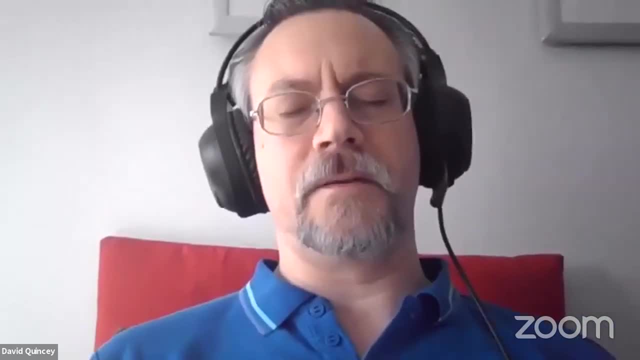 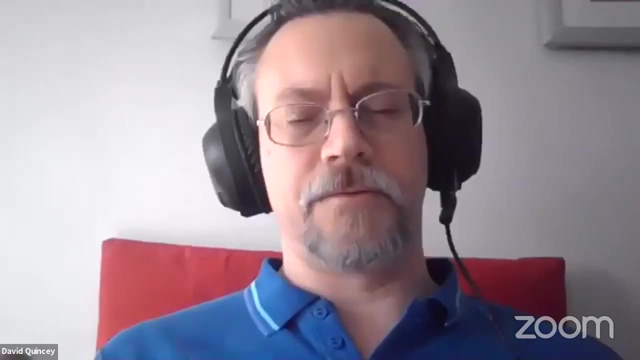 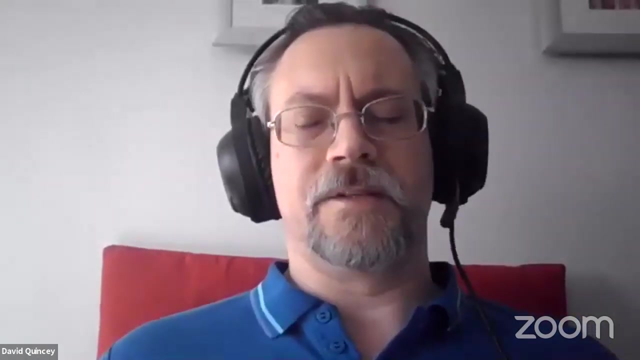 that and as part of this ARP we will actually be attempting to develop with the routes and regions um the climate adaptation pathways approach. so again, this should all come through in in this ARP. we haven't in the past done a lot of work in interdependencies um, so this opportunity will 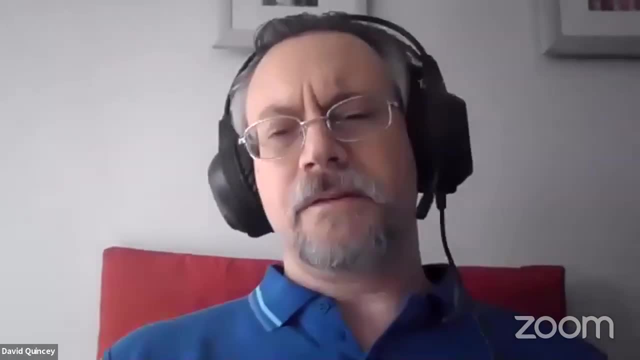 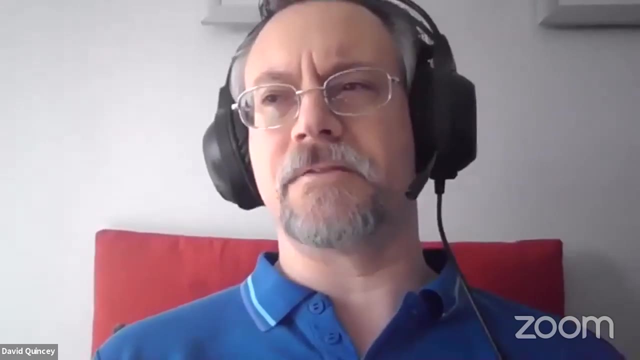 be taken as part of writing this as well. so my hope is that, basically, all the good stuff that ARP gives you, which is the collaboration, it's the, it's the reminding people of the importance, it's the gathering information, it's the summary, it's the understanding and the ability to identify gaps- 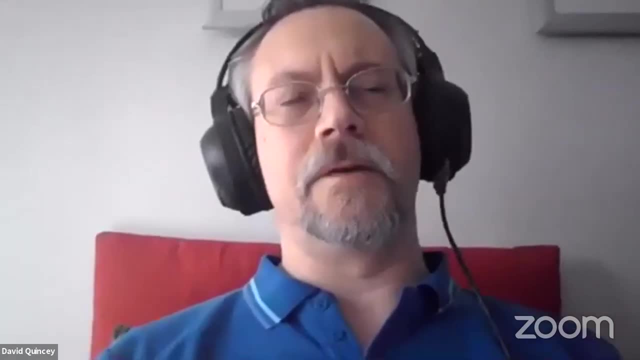 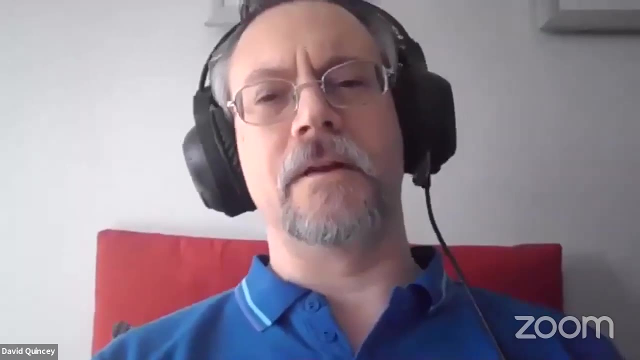 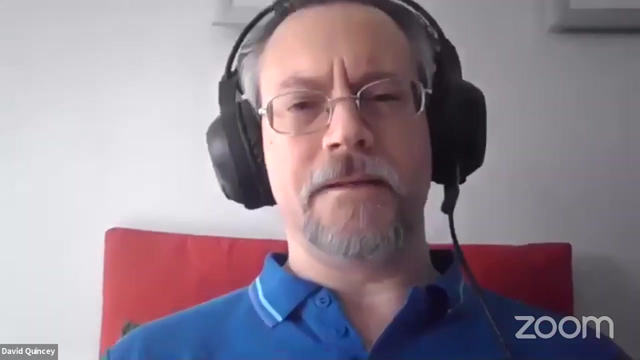 and address them all. that will follow through into this one. but hopefully we will learn with a um, an actual action plan, and we'll end up with it tying much more to the frontline parts of the business than it did in the past. um, I think really that's probably a bit of a ramble, but it's sort of um, it's our stream of consciousness. 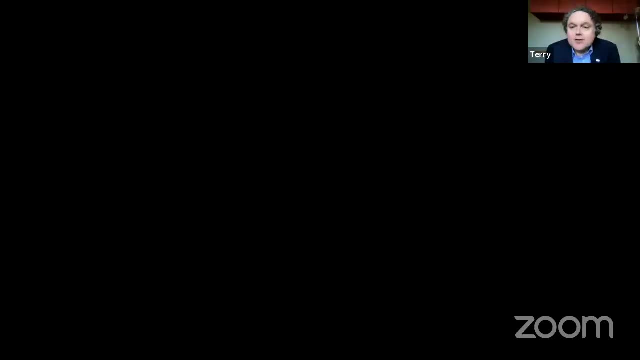 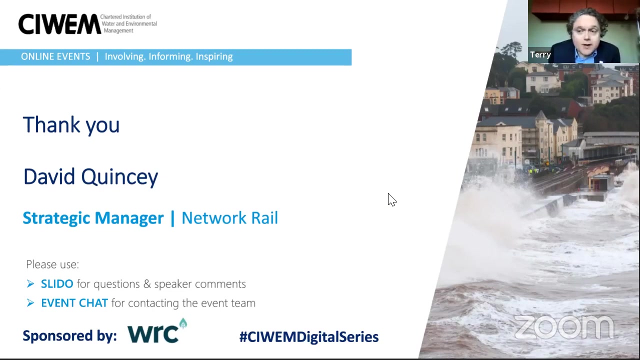 on the reporting, I think, David. uh, not a ramble at all. that was um very clear and very, very interesting. thank you very much. um okay, um, I can see some really cracking questions coming in on on Slido. please keep them uh coming. um. we're going to move on now to our next speaker, who is James. 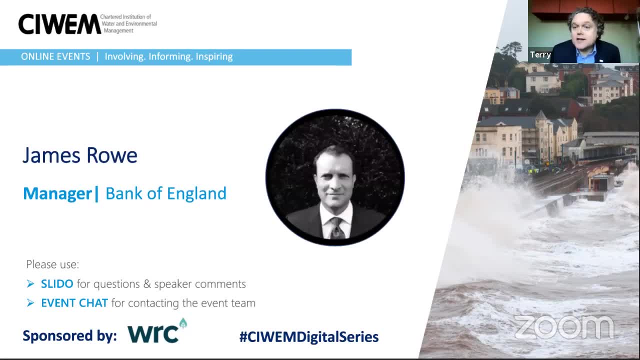 Rowe from the Bank of England. uh, James, I am saying you don't have a camera, but I'm hoping you have a microphone, so over to you I do. can you hear me okay? yes, loud and clear, thank you, perfect, um, so a quick couple of minutes then on on PRA. uh, in April 2014, the PRA accepts an invitation from: 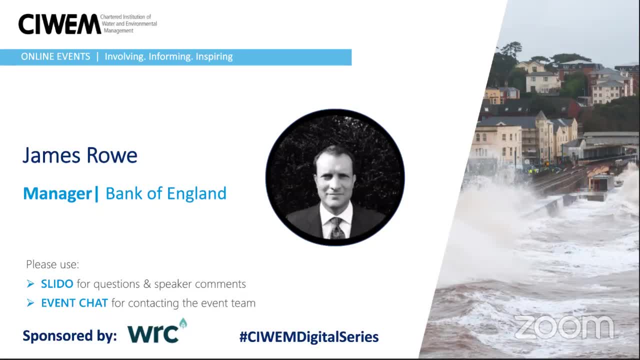 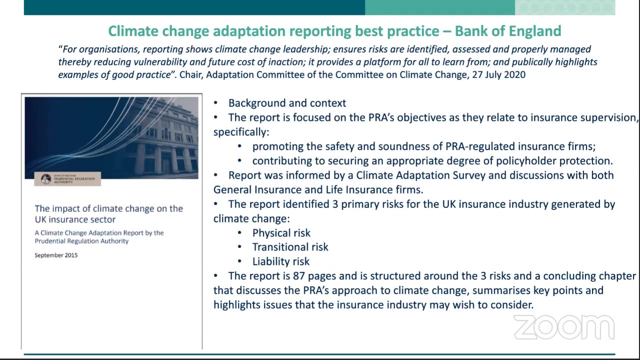 DEFRA to complete a climate change adaptation report focused on the UK insurance sector. the result of an 87 page report was the PRA's response and also the PRA's first report on climate change. the report's objective was to provide a framework to identify the risks arising from climate change through the lens of the PRA's statutory objectives. 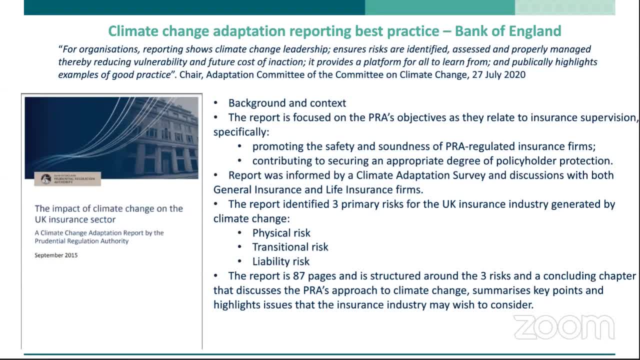 in relation to insurers, ie the safety and soundness of firms and the appropriate policy protection for policyholders. the report took the form of initial risk assessment. it explored possible responses to the risks identified, but was not intended to provide a policy prescription. the report also discussed opportunities for the UK insurance industry as a result of climate change. 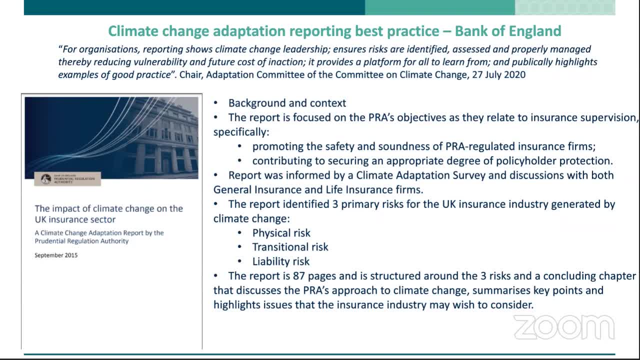 regarding inclusion of climate change science, the report sought to reflect evidence provided by respected authorities, particularly the IPCC. the PRA's areas of judgment in the report were focused on the relevance of scientific evidence to regulated firms and to the PRA's objectives, as you're probably aware. 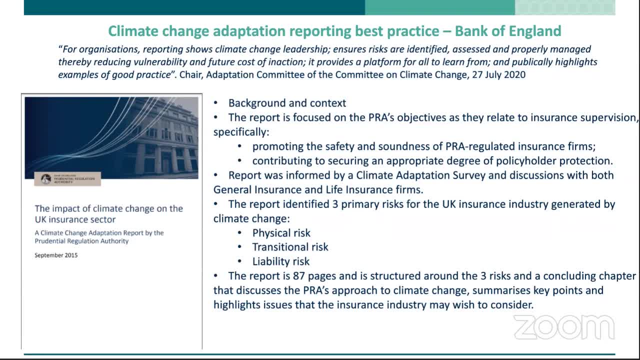 insurance is a market-based mechanism for the transfer of risk. PRA's role, through its objectives, is to contribute to ensuring that the risk transfer can occur in a reliable and effective way throughout the UK insurance sector. as you're probably aware, the report identified three primary channels or risk factors through which impacts from climate change might be expected to. 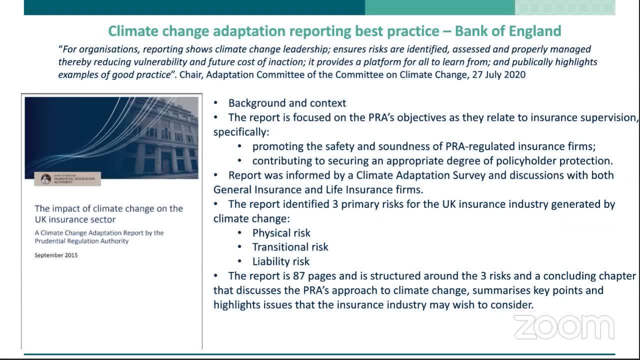 arise. first of those was physical risks, ie the first order of risks that arise from weather related events such as floods, hurricanes and storms, and these effects the report determined could be direct or indirect. secondly, transition risks. these relate to the financial risks which could arise for insurance firms in transition to a lower carbon economy for insurance firms. 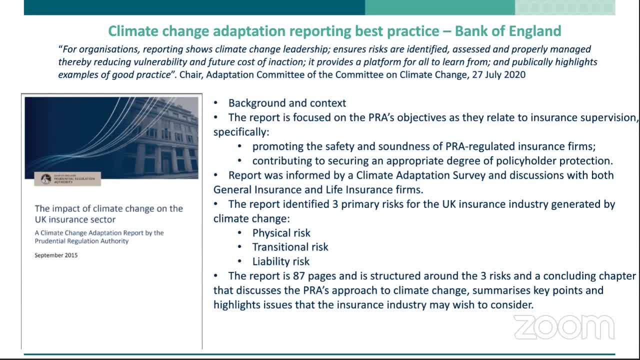 the risk factor is mainly about the potential repricing of carbon-intensive financial assets and the speed at which any such repricing might occur. the risk factor is the risk that could arise for insurance firms from parties who have suffered loss and damage from climate change and seek to recover losses from others who they believe may. 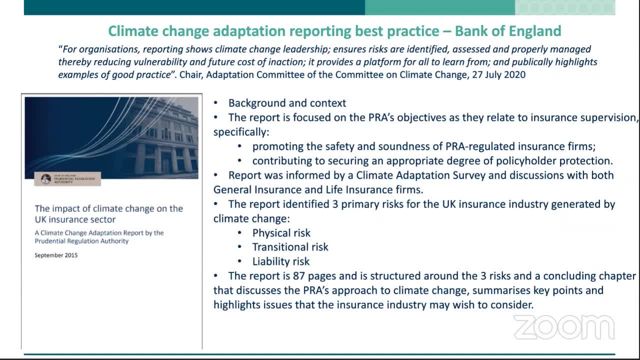 have been responsible for these factors. the report explored the nature of the risk, possible impacts on insurance firms balance sheet and the action firms could take to mitigate them. clearest risk identified in the report was from physical risk only. most of the report is focused on that aspect. 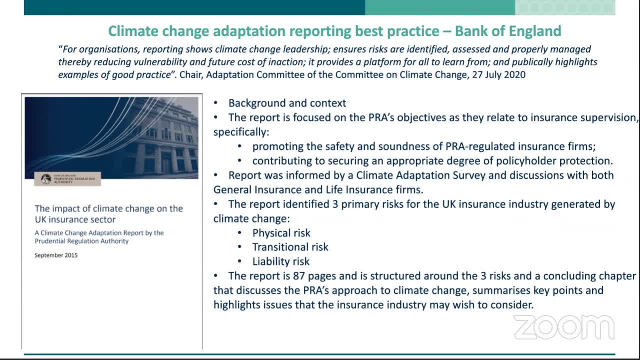 at the time of writing, understanding of the other two risk categories was less well developed and more uncertain. nonetheless, the report anticipated that it could have a meaningful impact on the pras objectives over time across these risk factors: the pras analysis, potential climate change to present a substantial challenge to the business model of insurance in particular. the report 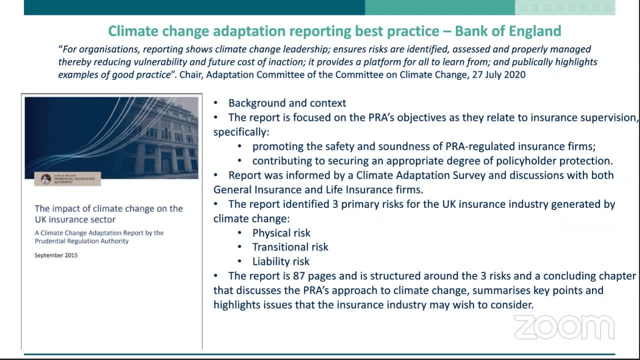 highlighted, it was possible that climate change will reduce or eliminate the sector's appetite to provide insurance cover specific sets of activities, assets for customers, and this is relevant to the pra's objectives. it was highlighted in an area of interest for other policy makers. in terms of preparing the report, the pra participated in four roundtable discussions. 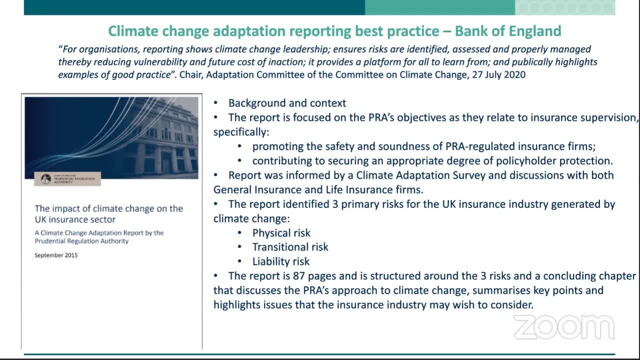 which were fundamental in helping to determine the content of the report. these were each attended by up to 30 participants, including at least 10 different insurance funds. the report provided a number of conclusions in relation to the risks identified, which i'll highlight just one here now. climate change quote. sorry, climate change is becoming increasingly. 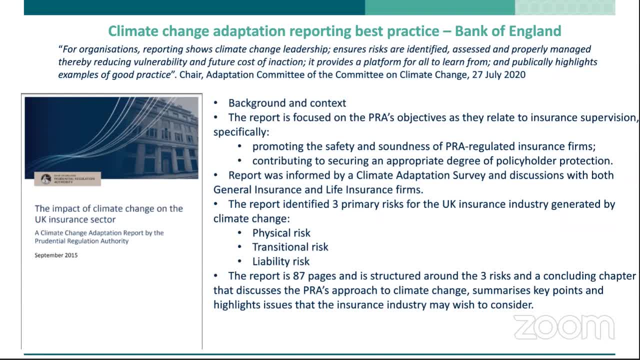 relevant to financial regulation. the pra's approach will focus on promoting resilience to climate change and supporting an orderly financial sector transition to lower carbon economy. the pra will do this through a combination of international collaboration, research, dialogue and supervision. on that last sentence, in the intervening five years, our approach continues to focus on these priorities. the report helps to. 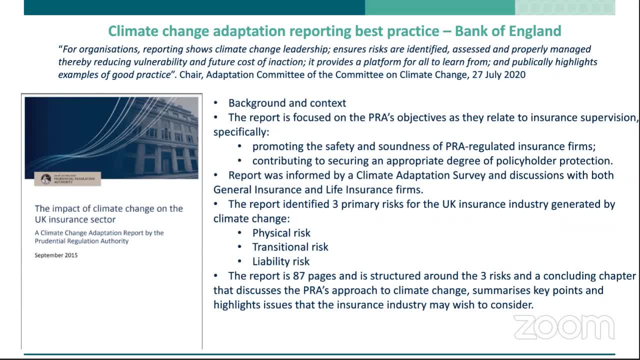 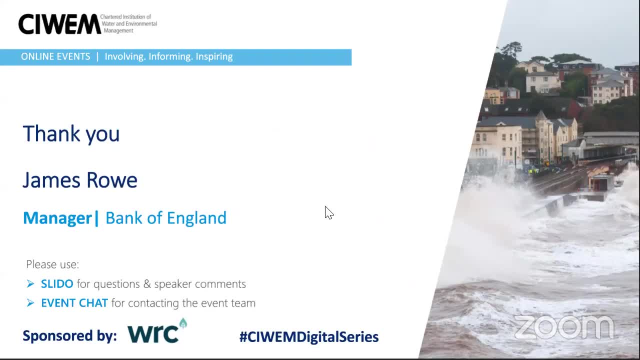 drive forward these priorities and our focus is a central bank and regulator which will be fully reflected in our next report. thank you, james. thank you very much indeed for that. i understand sad you can't join us for the questions, uh, later, but um i, um, i trust that we'll be able to kind of reach out to you as we put together the. 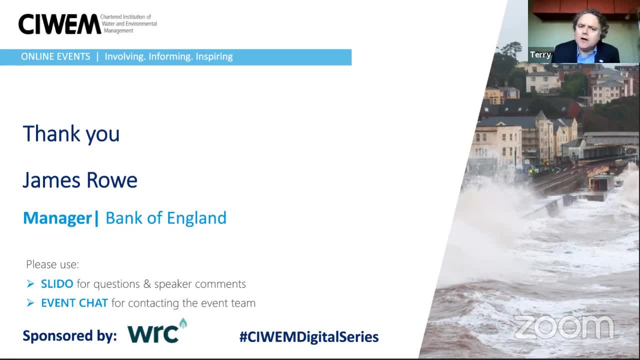 um the output from today's uh web webinar. um, if any specific questions do come, absolutely apologies for that. and yeah, absolutely, we'll speak again in the future. that's lovely. i really appreciate it. thank you very much. okay, we're now moving on to um hannah armitage from the 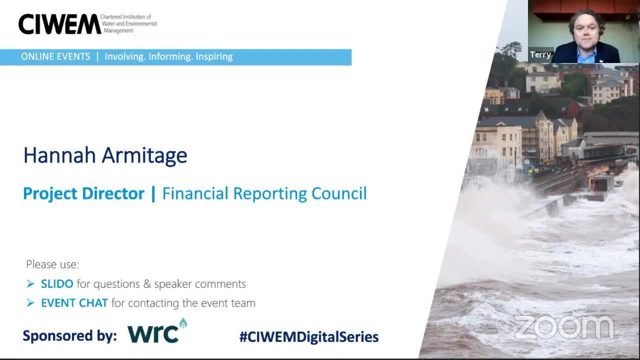 financial reporting council. hannah over to you. hi everyone, thank you very much for having me today. i'm coming, as terry said, from the financial reporting council. now, we're an organization that many of you may not have heard of. we're regulators of accountants, auditors and actuaries within the 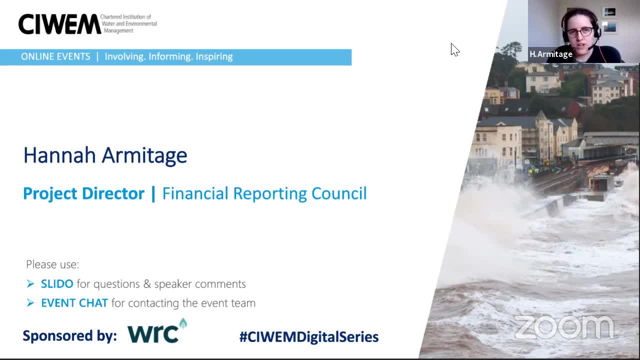 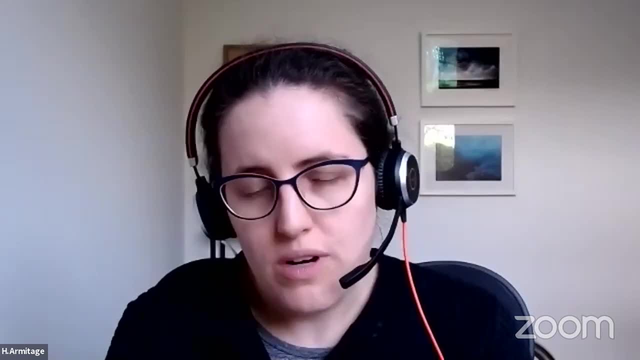 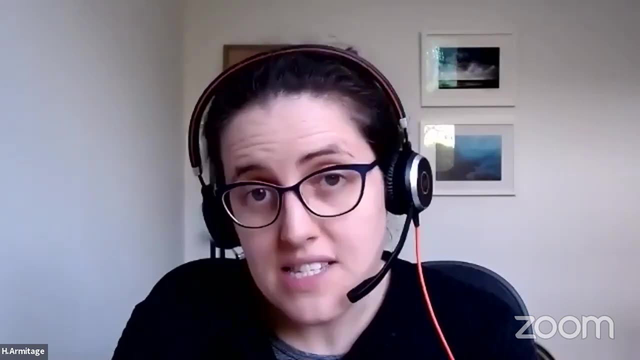 united kingdom. so last year we did a project looking at a range of a range of entities within the reporting and investment chain. so we looked at how the governance of companies, company annual reports, audit activity, professional associations and investors are taking account of the financial account of climate related considerations. as part of that report we found that there was some 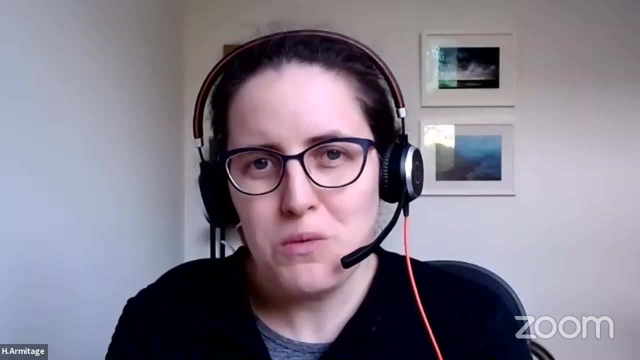 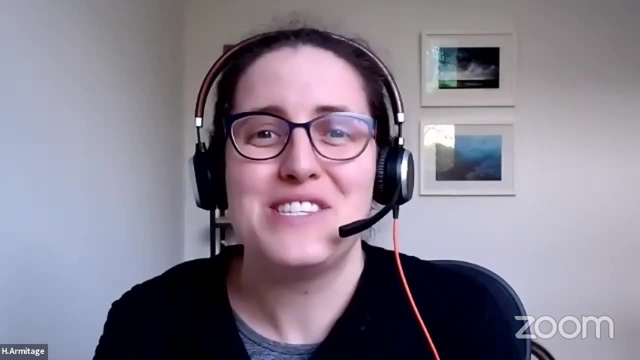 interesting practice but that more needs to be done. so we'll be coming up later this year to do our first climate adaptation report. so i apologize that i don't have the um, the history that some people have about what they've done in the past, but what we learned from our report last year. 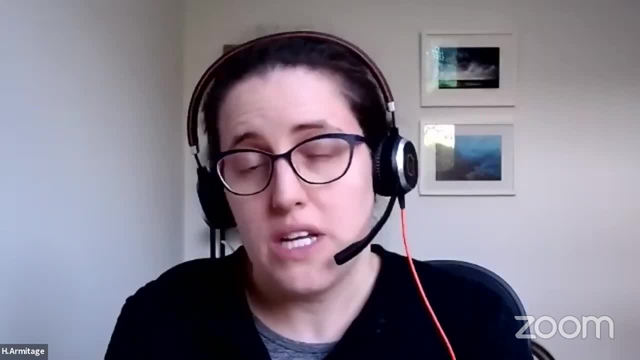 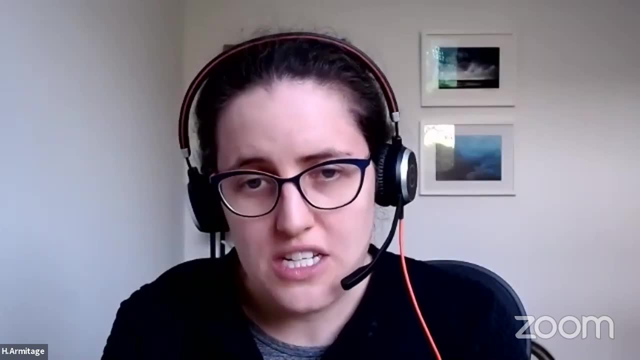 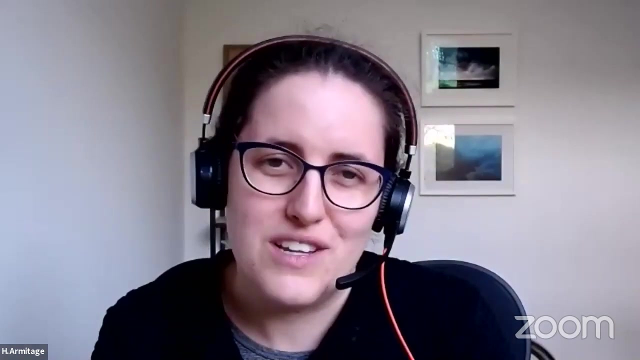 is going to enable us to put forward some thoughts across a range of real economy, businesses and also the investment, the investment chain, as we make some um, some reflections on adaptation issues. as i said, we're in the first round of climate adaptation reporting, so very much at the start of the process, and our regulatory remit is a bit different to some of 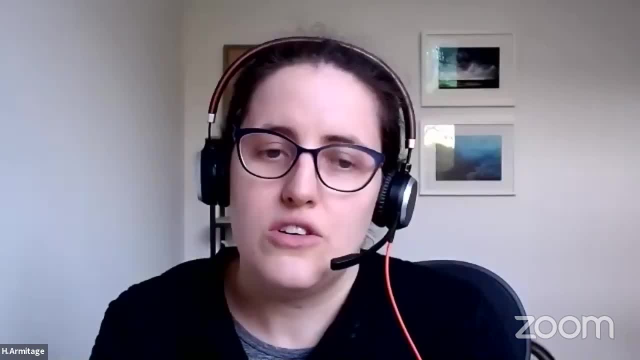 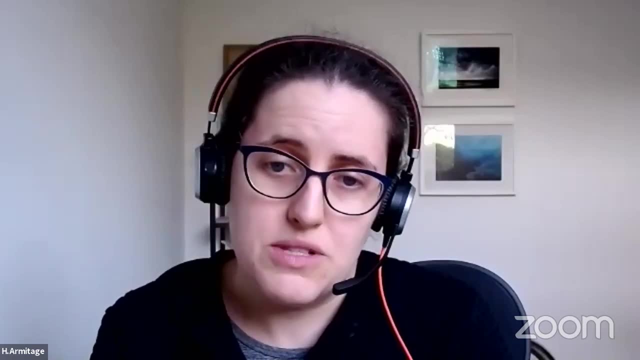 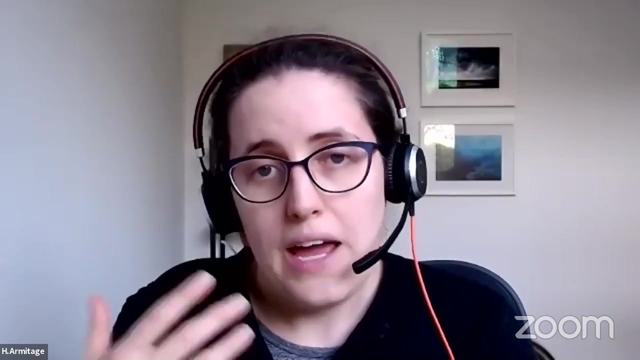 those other regulators on this call, but we are going to be looking to consider, as part of our climate adaptation report, how, through their reporting, companies are demonstrating that they're taking account of climate related considerations, including adaptation, how auditors are doing so and what we can expect of investors. 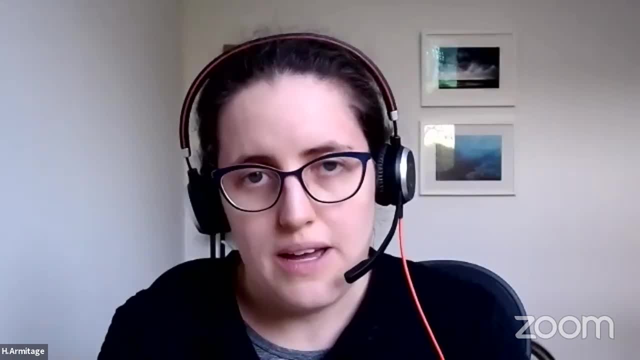 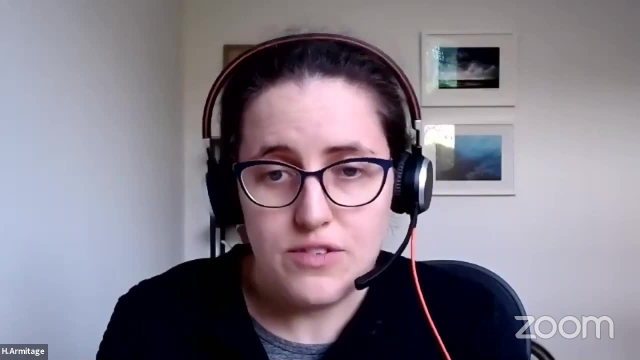 and others throughout the investment chain. as we aim for um a consideration, a better consideration- of adaptation, we're going to be focusing on our ability to influence and encourage the direction of change. as we talk about what that reporting might look like, and we're also hoping that 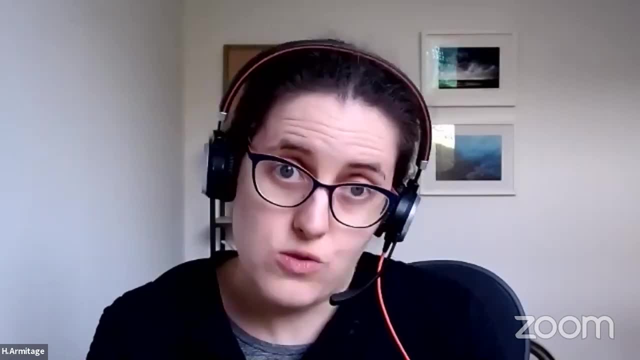 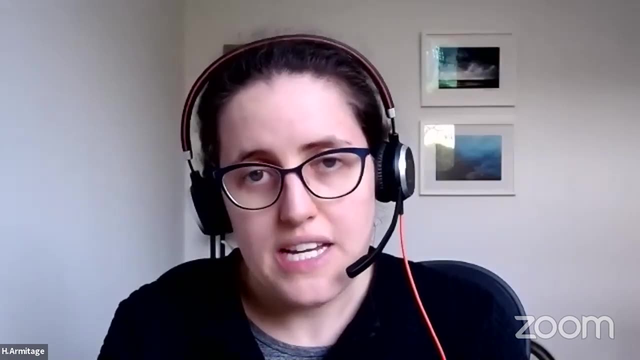 alongside some of the other regulators who work more in the financial space- so bank of england and pra, the pensions regulator, and the fca- that we might be able to coordinate to come out with some quite key messages about climate adaptation and how we're going to be focusing on that as well. 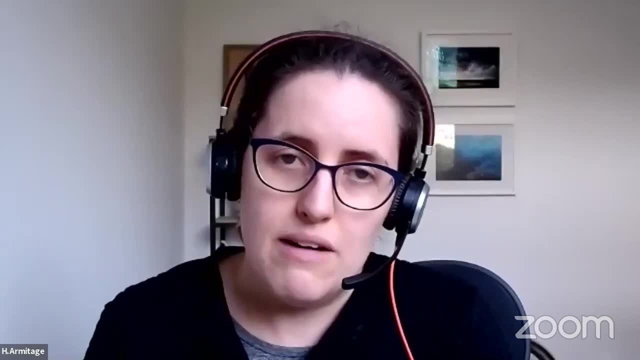 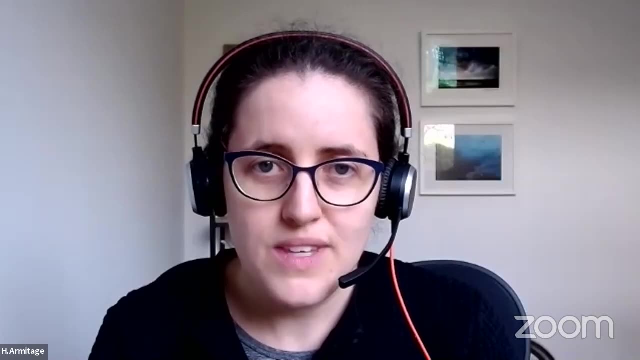 so we're going to be focusing on what the risks are, what the risks are that we face in the financial arena and how we're all viewing those and what that means for our individual remits. it's very happy to take any questions on that in the q a session. 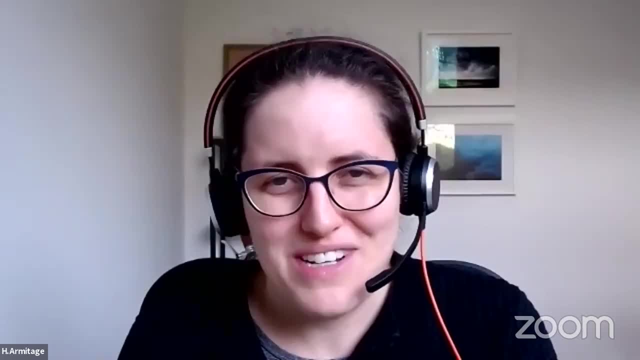 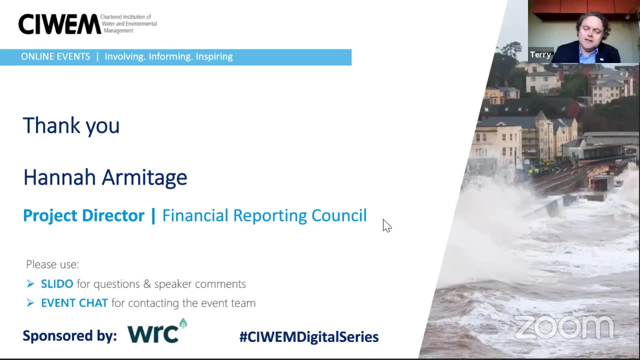 and i look forward to hearing others tips of how they've done climate adaptation reporting excellent. thanks very much, uh, hannah. it's really good to get the financial perspective into into this debate. thanks very much. okay, we're going to move on now to uh daniel. 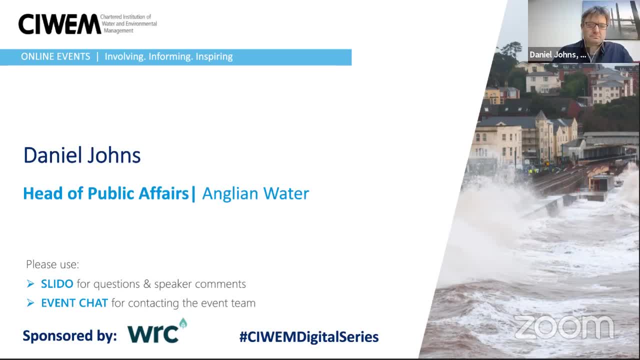 johns, who is a cywem fellow and works for angling water, who are a cywem business partner. so we're doing lots of good things together at the moment. uh, daniel, it's really good to hear what you have to say on this particular topic over to you. thanks very much, terry, and i've got uh. 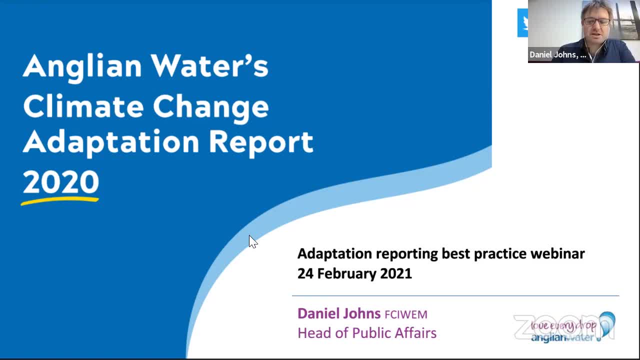 the pleasure of presenting at angling water's third adaptation report, which we published in december 2020, having consulted on an early draft last march. obviously we wanted to- you know, given what chris stark was saying earlier on this morning- we wanted to bring our adaptation report to the 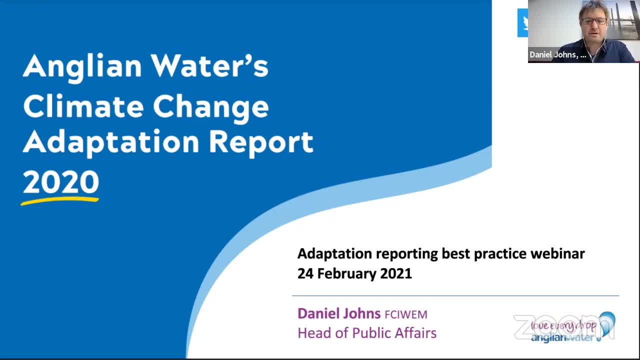 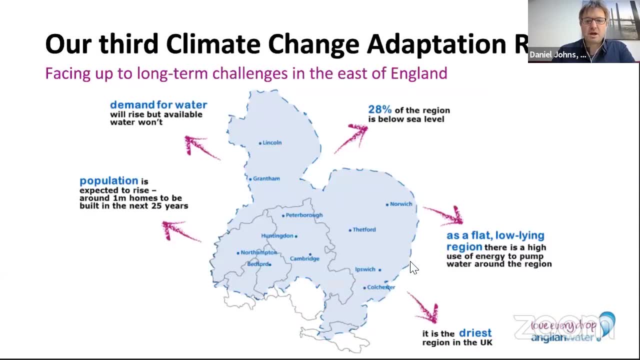 out and get it published, get it consulted on. uh, we're in advance of the third climate change risk assessment so that our our results and the progress that we've made we fully factored into that assessment and, as a as a water company serving the east of england, climate change. 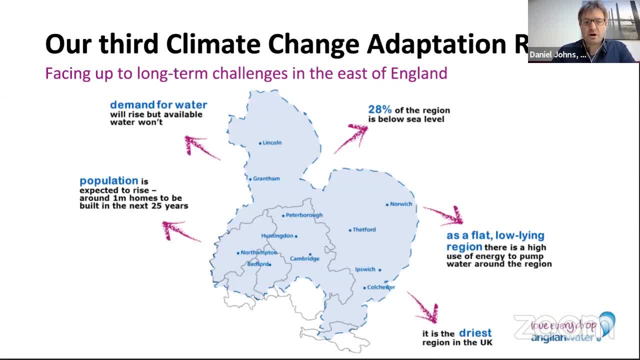 climate change adaptation, of course, is incredibly important to us. what carbon is to net zero, i would argue, water is to climate change adaptation. uh, this is the driest part of the country. it's the flattest parts of the country, so we are managing the risks of water supply shortages on a daily. 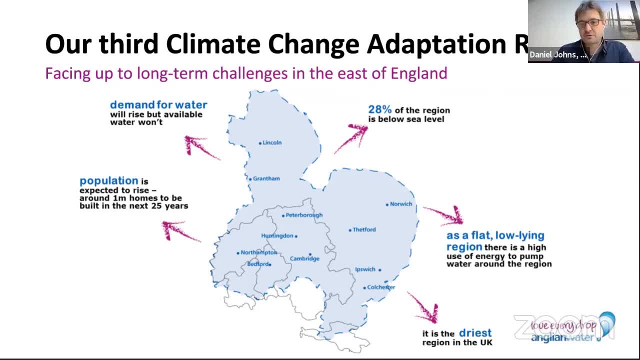 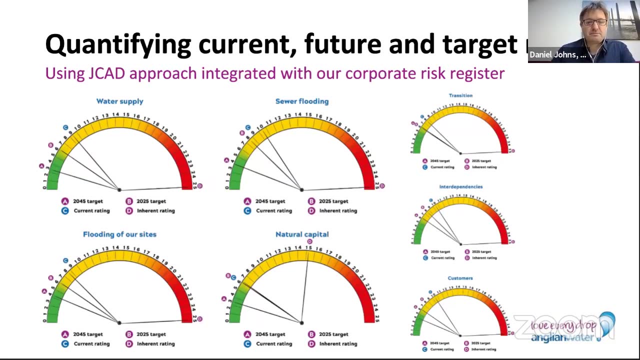 basis. managing risks of flooding- absolutely the amendments seal rise with a long eroding coastline. so all these risks, given the population growth and environmental uh degradation, are very much front and center of our climate change adaptation uh report. and just obviously i can't do it justice in the three minutes that i've got, but just to kind of encourage you to go to our website uh to. 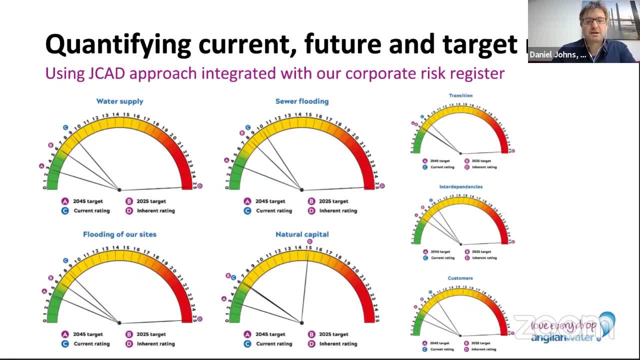 take a look at the report and together with the summary that we published alongside it in december. so we've got a nice, neat summary for customers. anybody else who wants to dip in for five minutes to take a look? uh, having reviewed, uh, from from the kind of ground up, uh, 40 plus risks that we 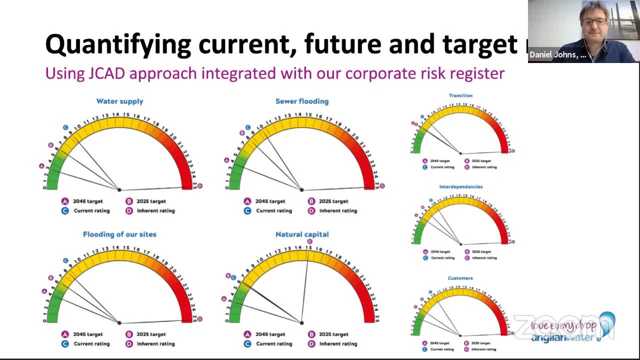 manage measure as part of the corporate risk register. we highlighted these four headline risks on the left-hand side, these kind of physical risks to the business, from water supply, if two relates to flooding and one relates to the natural capital, the kind of the quality of the ecology within our triple size in particular. so looking at the physical risks on the left-hand, 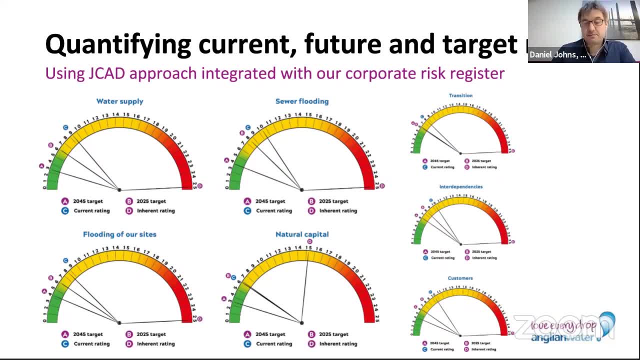 side. we also took it took a look at the transition risk business, so those financial risks, the business that we face in uh, moving to a net zero economy and, in particular, to becoming a net zero business by 2030, as we have committed to do. but we also looked at independencies and 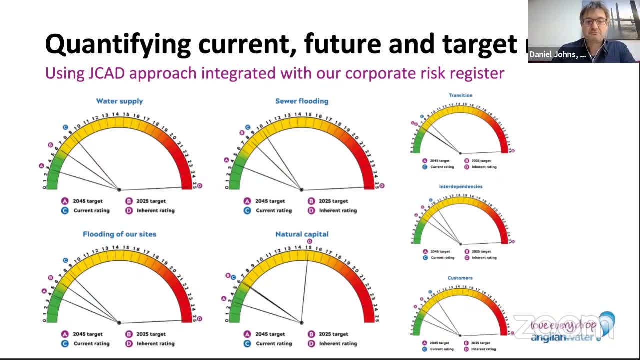 also on in a cross-cutting way, looking at our customers and the risks of extreme weather events. so our customers, looking at each of these cases, at the existing risk, uh, what the risk would be if we took no action and, of course, what we want to get to both in 2025 and in the longer term to 2045. 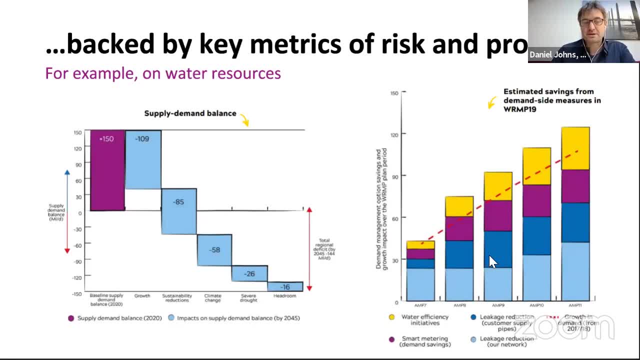 uh again. i'll just skip through the next slide. but essentially we try to make the report as as visual, as kind of uh engaging as possible and packing, packing it as far as possible with with all manner of evidence, thinking about the scale of the risk of business, plus also the impact of 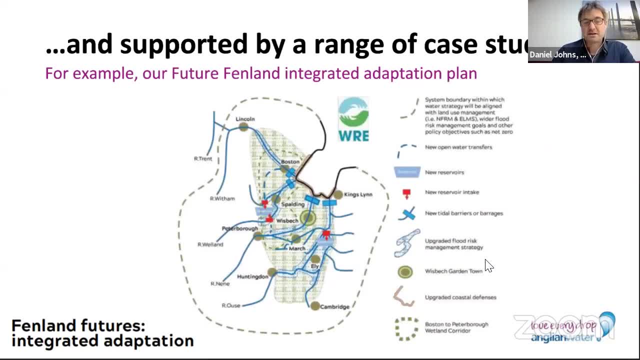 actions that we are taking, uh, together with a whole range of case studies, just taking examples of how we are managing adaptation risk on the ground, including taking this place-based approach to the fens, which is a risk of a range of different impacts from climate change, and trying to come up with a kind of place-based integrated adaptation plan. 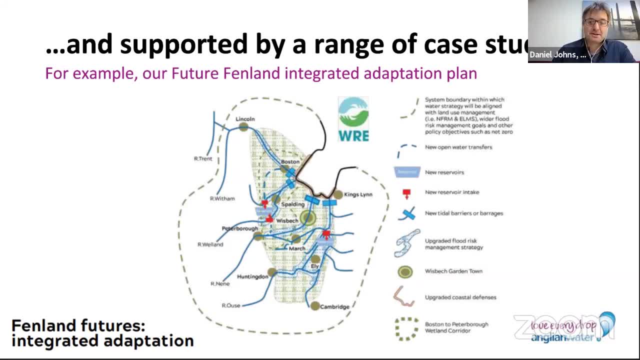 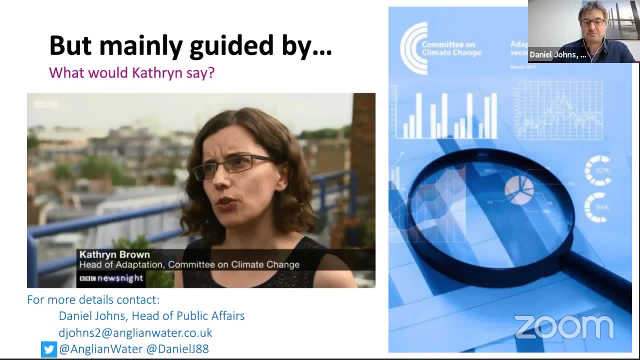 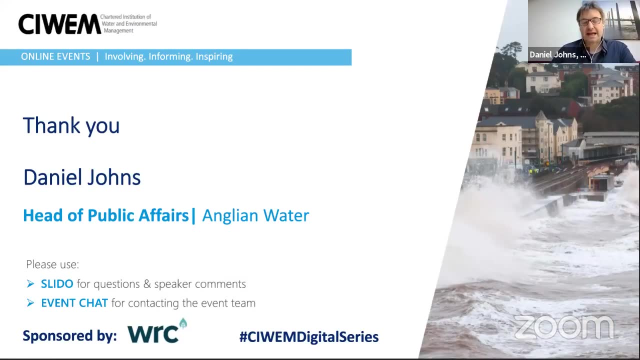 which also thinks about the long-term economic development opportunities that there are within that region. but first and foremost, as you know, given my previous role was at the committee on climate change, where my team literally wrote the book on what a good adaptation report should look like. uh, what was really driving both me personally and the team was trying to make sure. 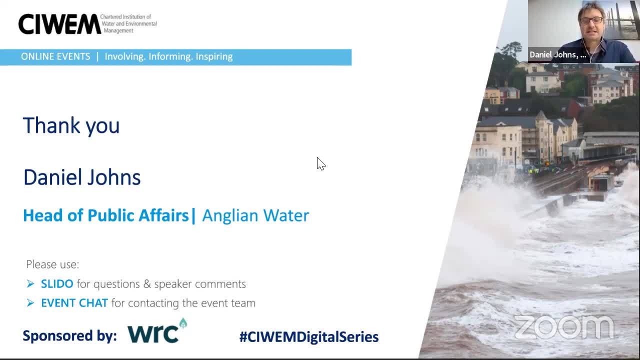 that we got some good feedback from ccc and that, uh, we got out earlier, say, with our report, to make sure that we got some good feedback from ccc into ccr3, but also we tried to set a bar very high in terms of what a good report should look like. so, thanks very much. great, thank you very much uh. 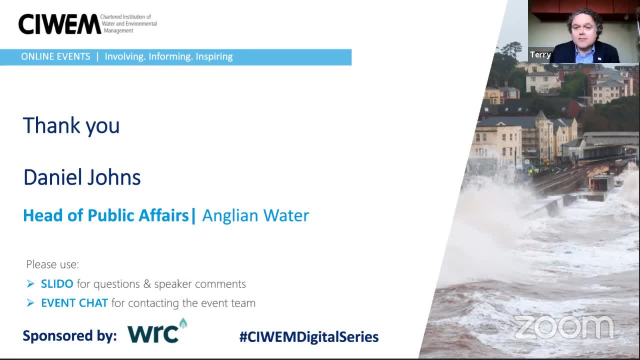 daniel, i think within your um boundary, you have a fascinating um range of of issues and uh and to uh to consider, and i'm sure there are days where you might find a different adjective to describe it, but i think it's a really interesting mix of things that you're looking to address. 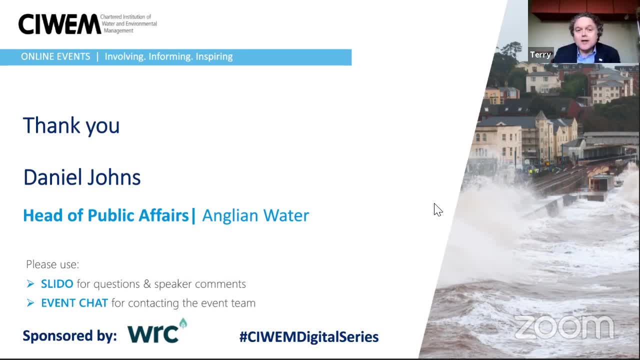 and we're now going to move on to our final speaker, who is, uh, howard perry from seven trent water. good morning, hopefully you can see me and thank you very much. so my name is howard perry. i am the energy manager at seven trent water, so we cover the midlands and into wales and very similar to. 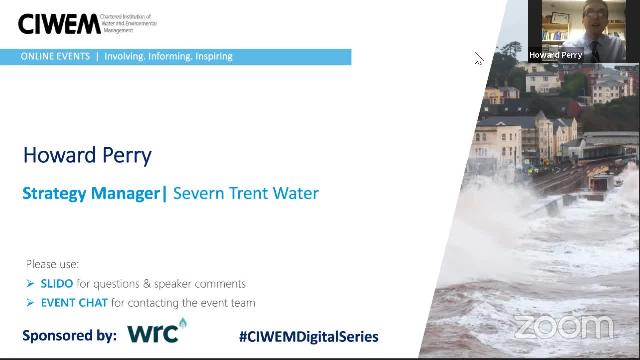 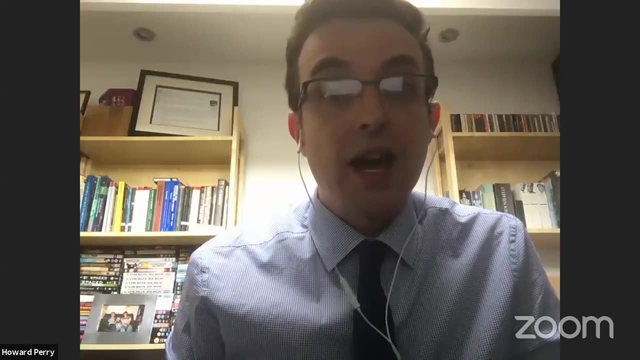 remit to anglian for our own region and i particularly lead our carbon reduction strategy to meet our net zero operational greenhouse gas by 2030 goal and i also lead our- And it's worth remembering that every year we report to the CDP and elsewhere on climate change, on carbon and on climate change risks as well. 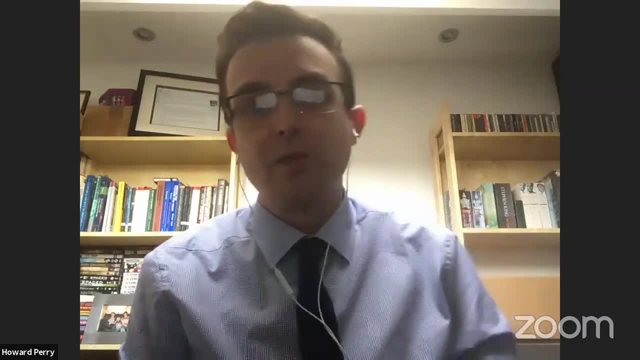 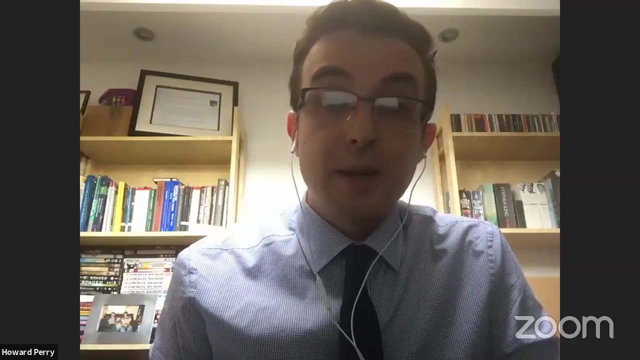 So there is potentially more out there in the public domain than people realise sometimes. I also did a lot of work with Mike, as he's mentioned, back in 2015 on our previous adaptation reports. That was published September 2015 and still well worth a read. 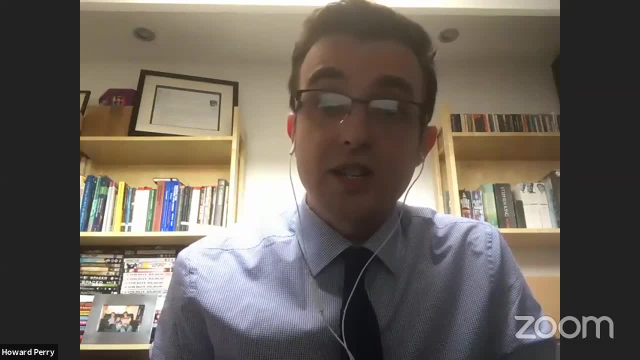 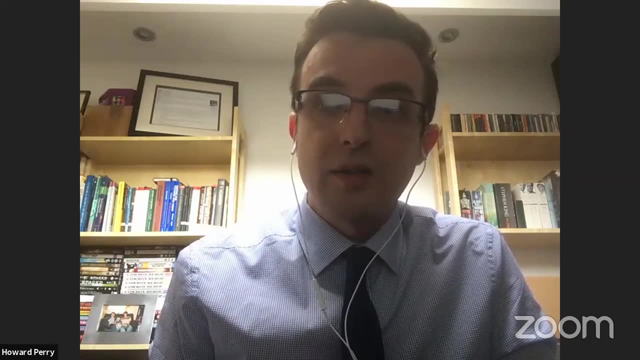 If you Google 7T adaptation, you will find that the risks and the actions that we've laid out there are still remarkably current and up to date. It's not been proven problematic in any respect so far, So it's well worth a read and a reflect. 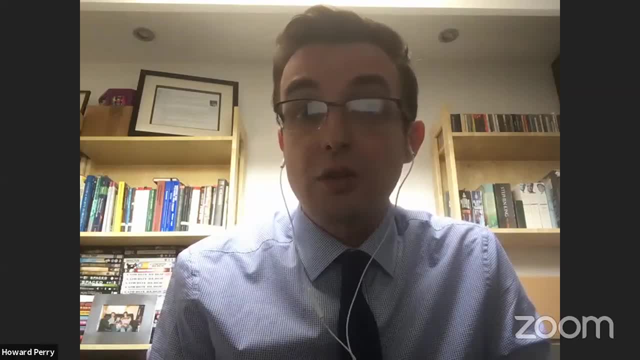 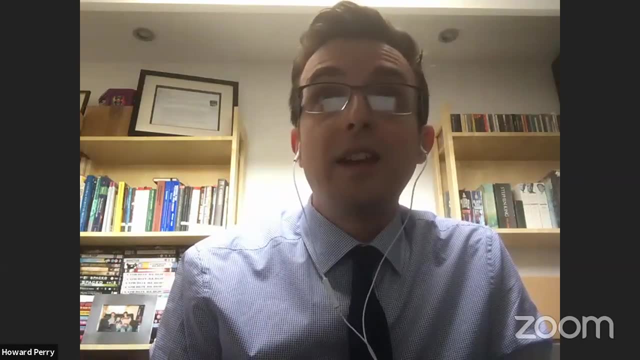 It is worth, though, I think, reflecting on the way in which COVID has given us some lessons to learn on adaptation, And it's interesting that's not been mentioned so far. It's a good example, I think, if you look at the government's pre-pandemic planning documents. 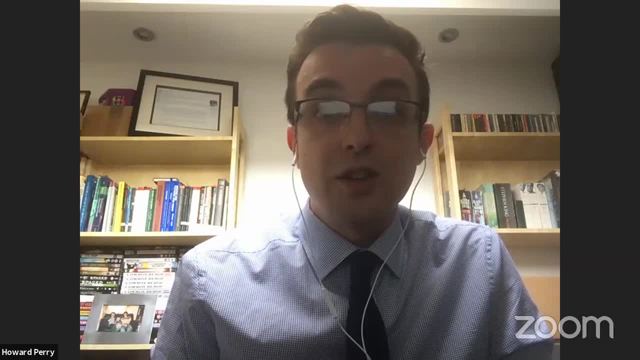 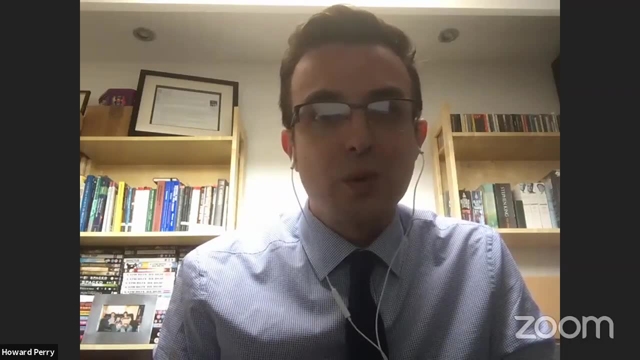 there were some very well thought out risk assessments there that showed that the risk was foreseen, and it was pretty well sketched out as well. But But the policies that were recommended were the absolute opposite, in some cases, of what actually came to pass. 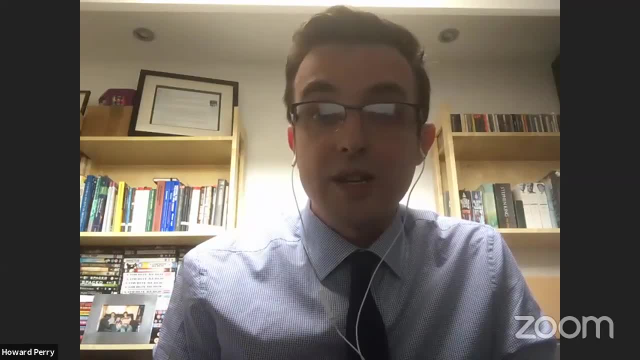 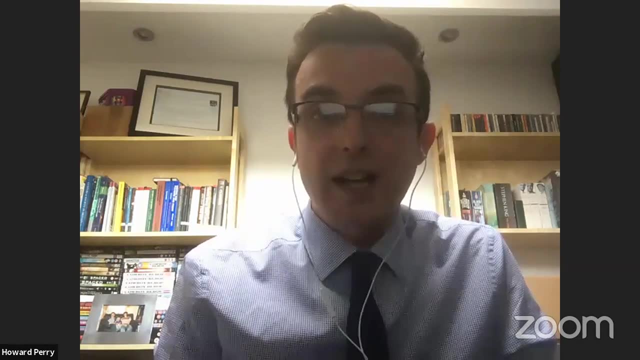 There's a real lesson there in adaptation planning, I think of. you can understand the risks centrally, you can plan for what you think is a sensible response, But in the event of when these things materialise, you may very well see something radically different. 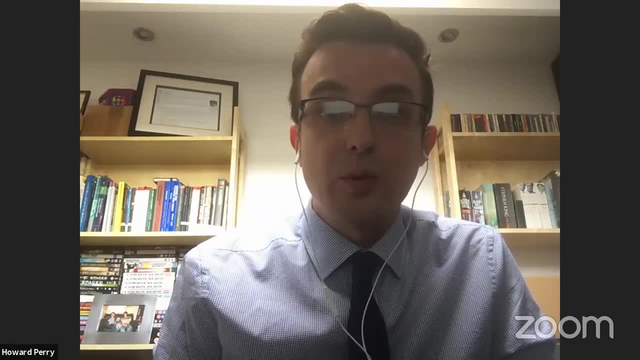 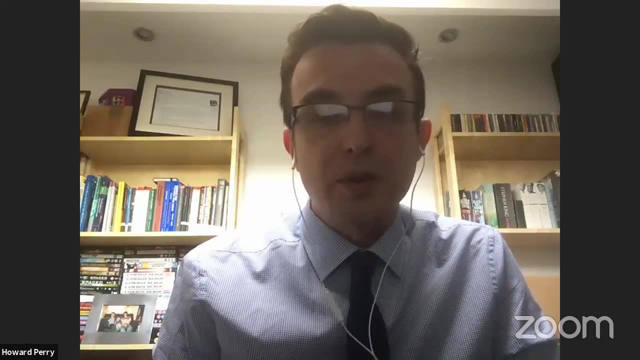 So the point from the Met Office speaker earlier on was very important. We need to think about some of those fringe risks that might not necessarily be on our existing radar and really stress test and think through what would responses be if certain risks came to pass. 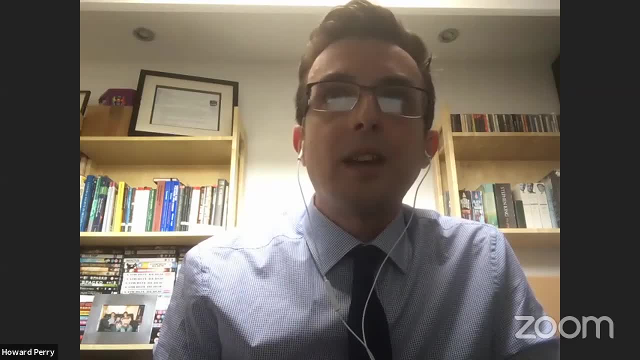 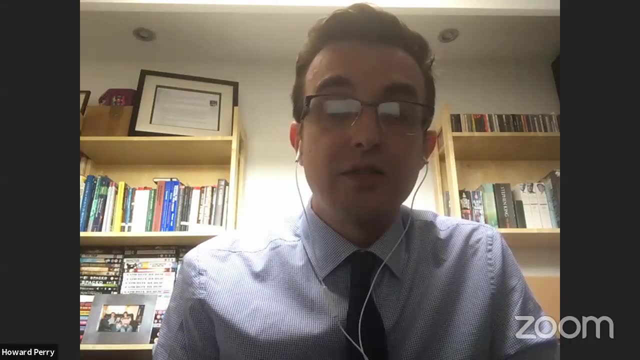 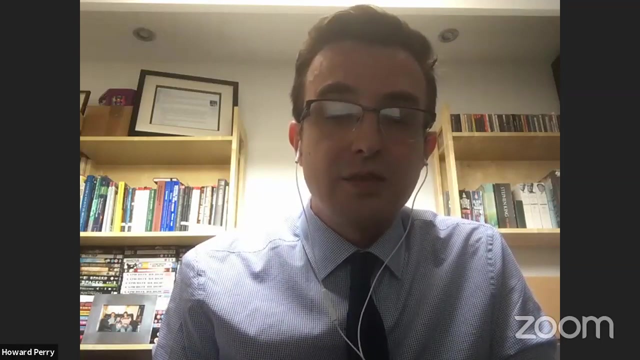 So really useful lesson for us there. In the last report, we outlined some of the major risks, and there's three key things that I just wanted to highlight that have changed really since, since 2015.. The first one is we've had a number of experiences of really severe weather events, and many of those were exactly of the sort that we highlighted in that report. So, for example, rising customer demand due to hot weather was our number one risk and is a risk that we've seen in practice. So, particularly the hot summer of 2018,, we saw record high water demand. In the summer that we've just had, 2020, we saw record high water demand as well. 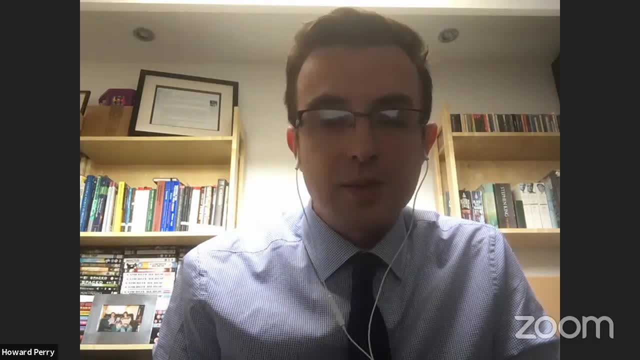 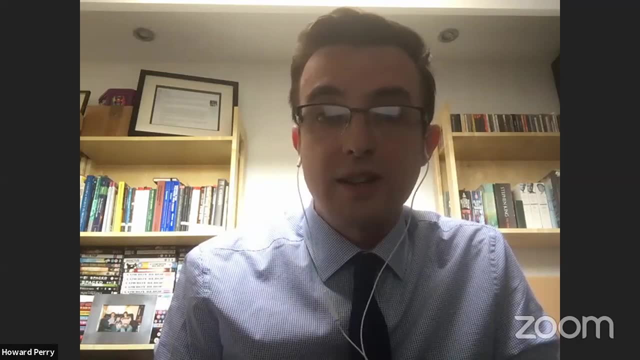 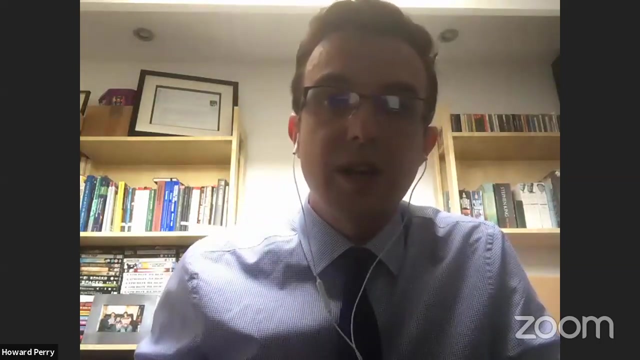 And what's been really encouraging, I think, is there's been some organic adaptation to those events that really help us to respond. So, as an example, off the back of the 2018 events, we really strengthened our network response team and we also targeted our customer communications in a much more specific way to some of the regions that we know suffer when there is a hot summer. 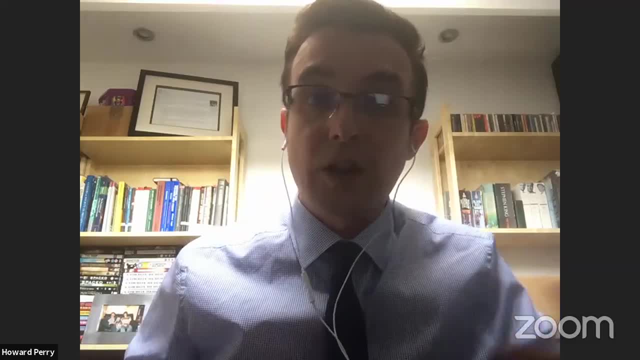 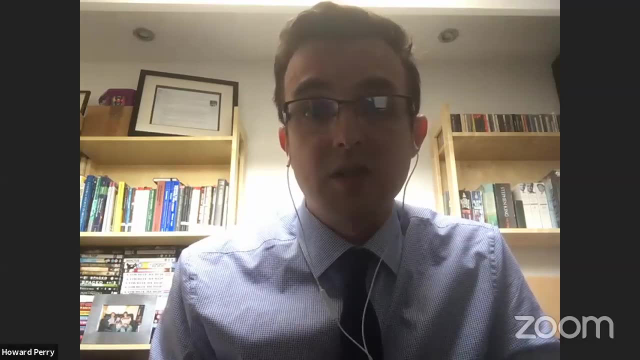 So I will give you a good example of that. Thank you, Thanks so much for that. Thank you, Thank you. hot weather. so there's some real organic adaptation and learning that's gone on from real weather events that we've had. I think the second thing to point out is that we've had some 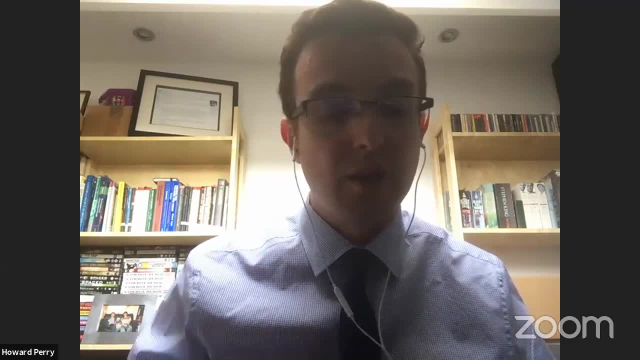 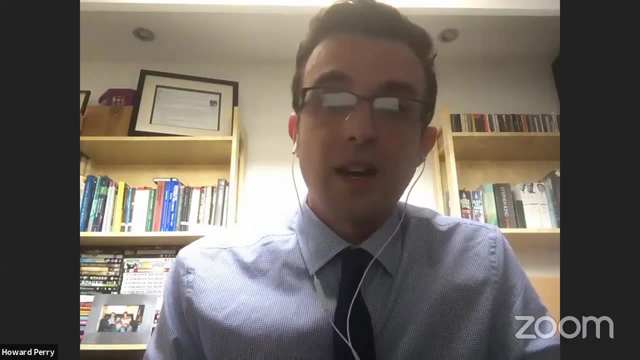 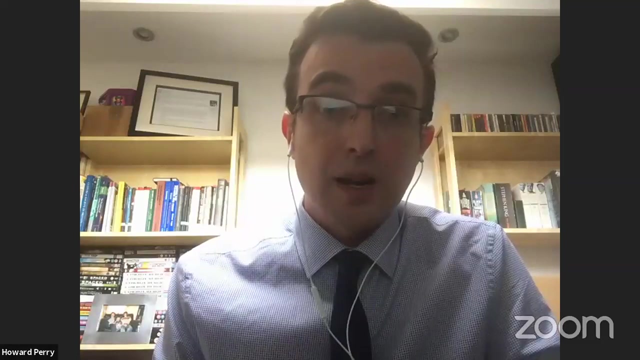 real context change, and a number of speakers have mentioned this already. so, for example, the investor community is certainly asking us much more about climate change risks and how we cope with them, and we've seen more pressure from our internal executive team as well to understand climate risks and make sure that we're declaring those, and also from our regulator and Ofwa in 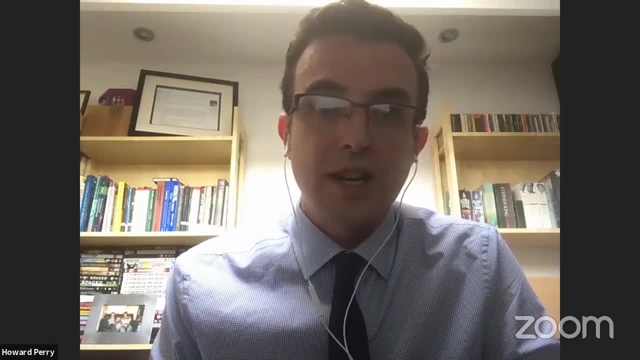 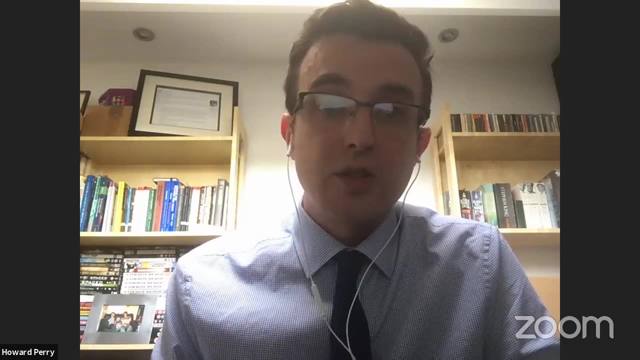 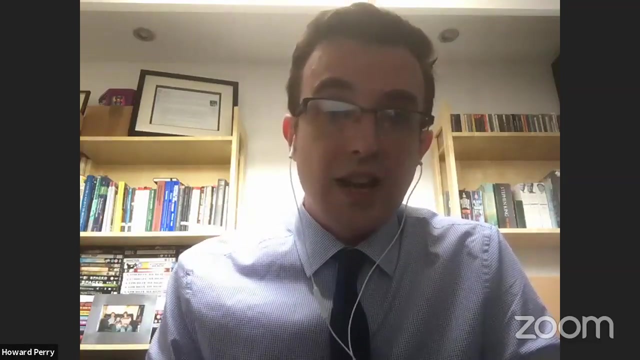 particular, you've mentioned resilience and climate change being key components of the next price review cycle, so that gives us a real golden opportunity to build something better in the next adaptation report and also make sure that it's properly reflected in the investment plans that we put forward. The final point I'll make is that we've also completed a lot of the actions that we 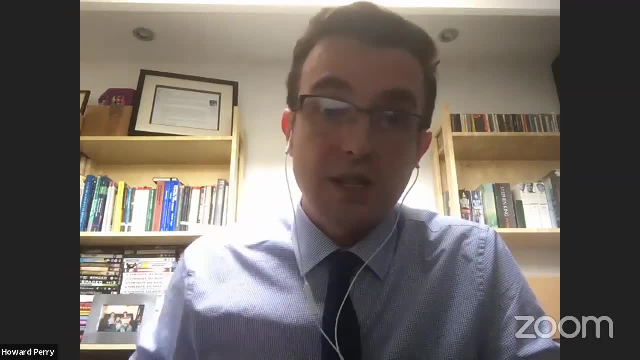 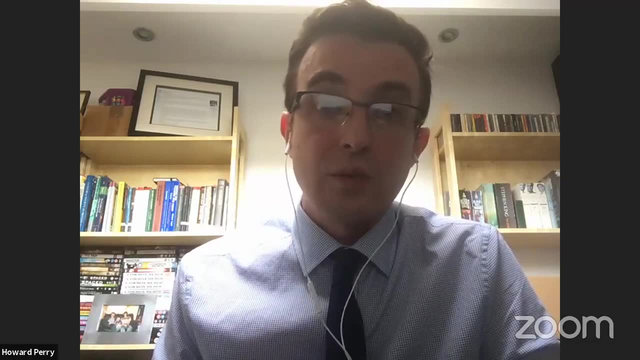 set out in that 2015 report. so the Birmingham resilience scheme is a good example of a major investment that was set out there and we have completed it. so we've done a lot of the actions that we said we would do and, I think, really important in adaptation. 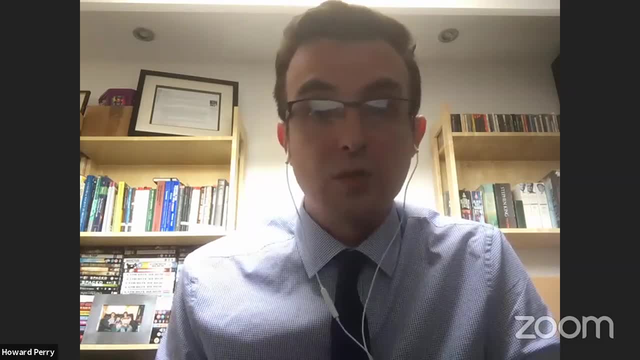 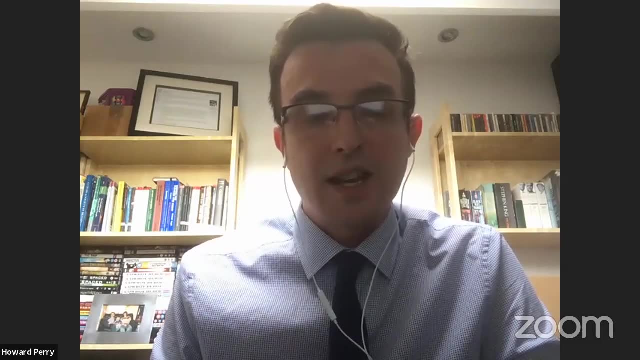 cycles is that plan and do and then check. have you done what you said you would do and has the risk materially changed? and getting into that continual plan- do, check, act cycle will be the way to best practice adaptation reporting in the future, I think. Thanks. 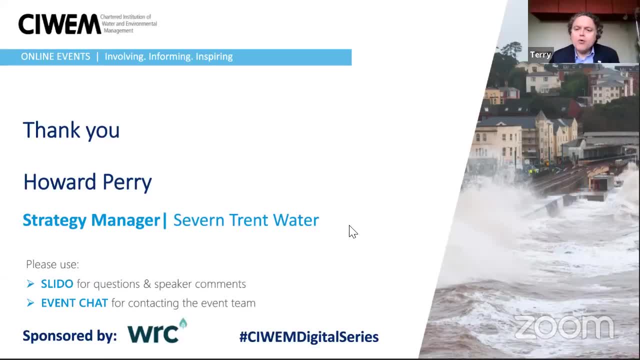 That's smashing Howard. thank you very much. Okay, if all of our speakers please come back on on camera. but we're going to move now into. we've got about 25 minutes available for some questions and I'm glad we've got that amount of time because there's some really great questions. 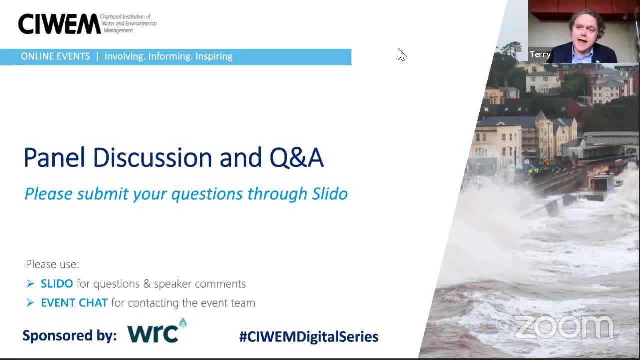 coming through, many of which I think are going to allow you to expand a little bit on some of the things you've already told us. Having said that, please don't feel obliged to answer every single question. it'd be good to try and get through as many of these as we can, so if you don't, 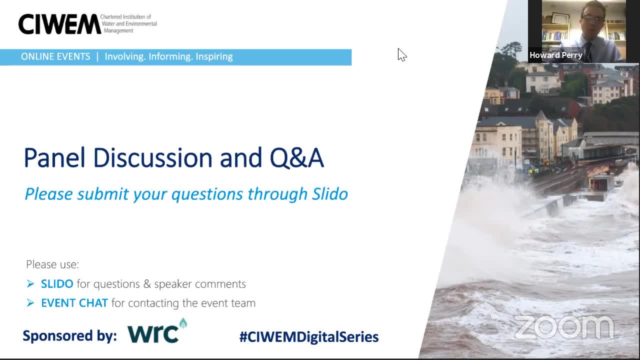 don't feel obliged to try and be additive to things if it's not necessary. Okay, all right, I'm going to go straight to the top question, actually, because I think it's really going to sort of tease out some aspects of how we can accelerate progress. and the question comes from: 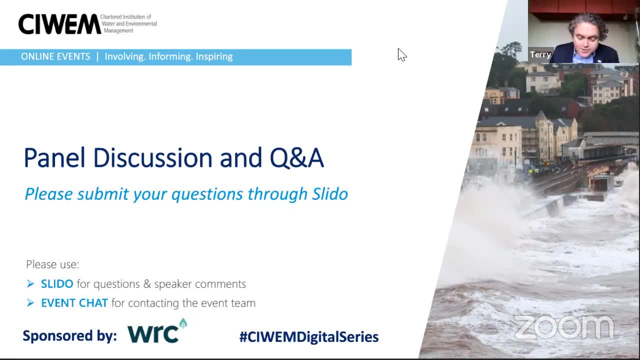 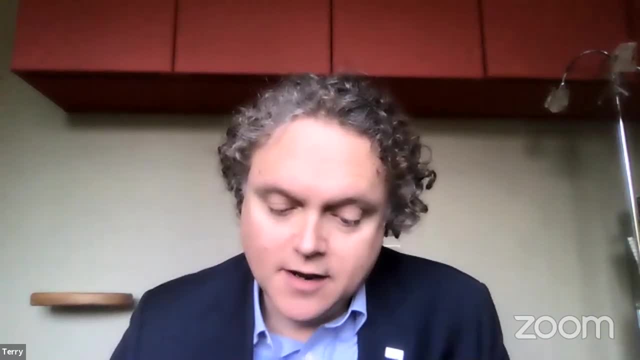 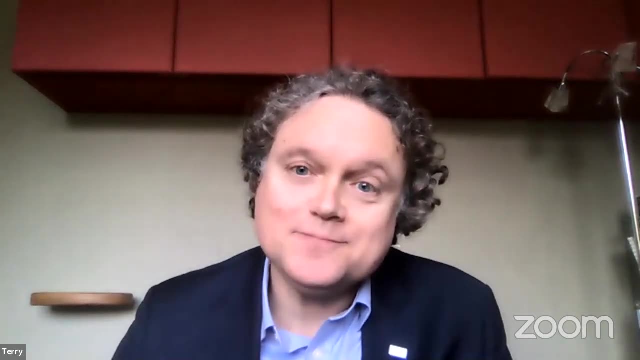 Peter Von Laney from Jacobs and he asks: what have you found to be the biggest barriers that you face in effective adaptation planning? So the blockers and barriers. who'd like to lead off with that? Yeah, I'll have to go first. yeah, so obviously we've just been through one price review process and, in fact, Anglin Water and three other companies. we are still in the midst of it and one of the reasons why we rejected our final determination from Ofwat was because it cut back our business plan by almost three quarters of a billion pounds. 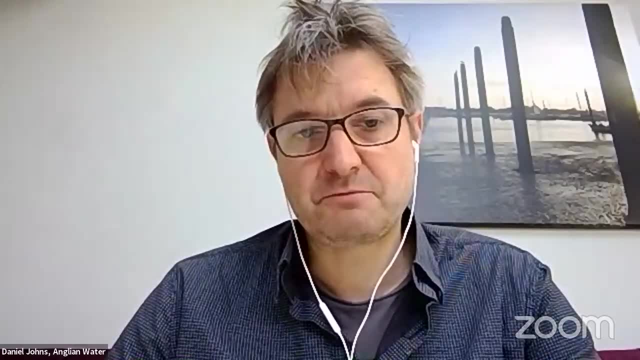 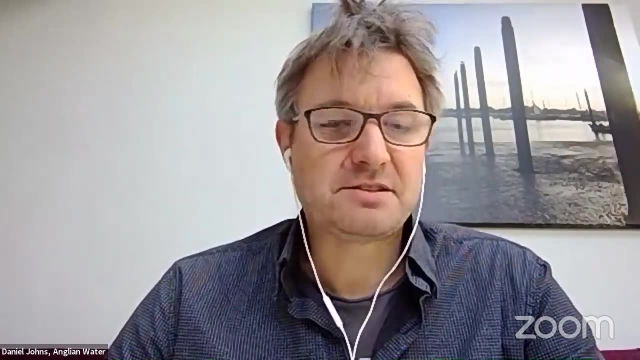 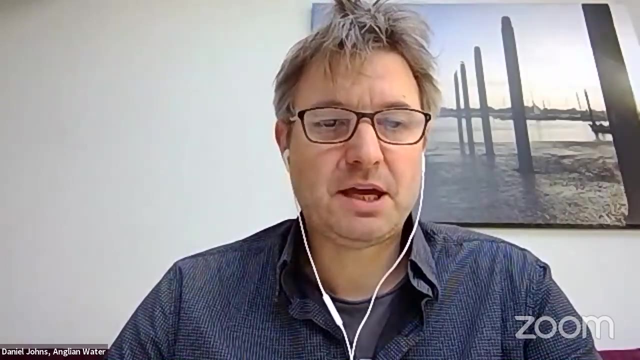 on projects that we see as absolutely vital to secure the long-term resilience of our water and water resource, water recycling services to customers, and so climate change adaptation is, say, the grounds upon which we rejected our determination and, as one of the one of the four companies, to appeal to the CMA. so funding is absolutely a problem and one of the 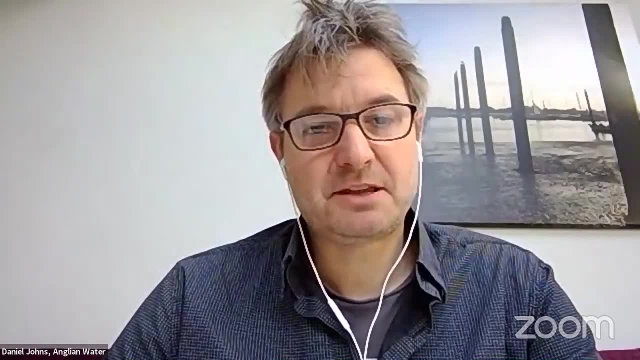 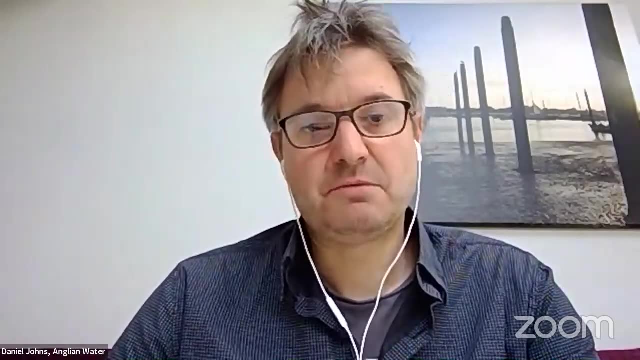 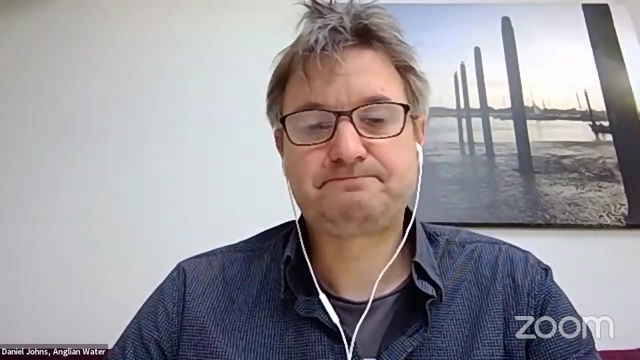 constant challenges we have is trying to counter the arguments that say the best answer for customers is to reduce bills in the short term, not think about what's the best long-term value adding investments that, as a company, we need to put forward to secure supplies into the long term. 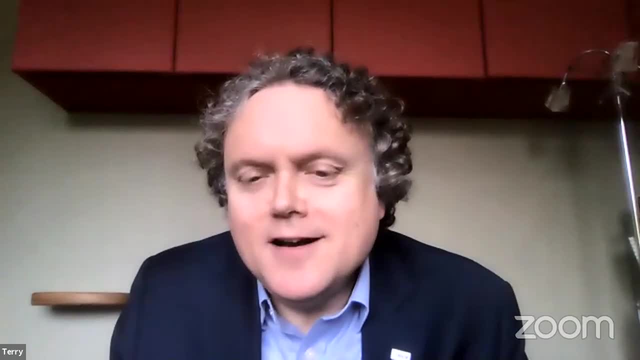 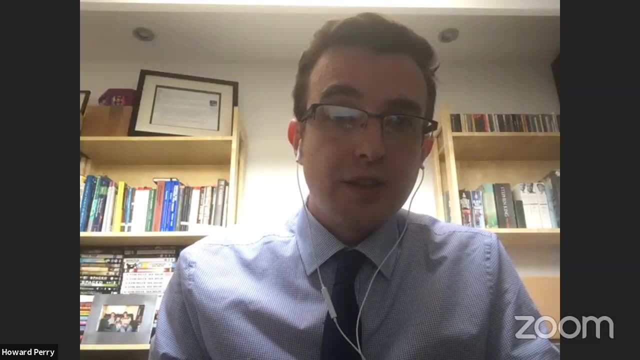 Thank you, Daniel Howard. would you like to add to that, or maybe you can just agree with that? Yeah, I would support that, and I think an additional thing to say is: often the best way to adapt is to make sure that your core services are robust, and it's not a very glamorous topic, but ensuring that. 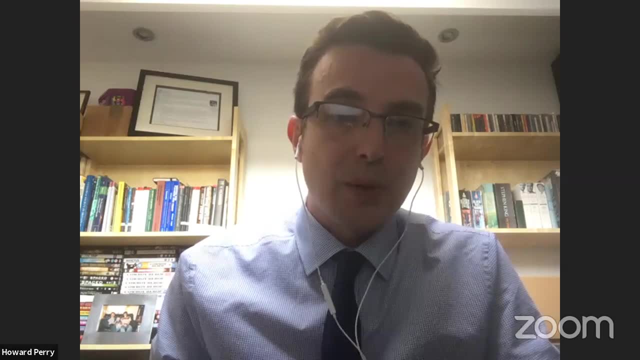 for example, we've got maintenance in our core assets and that they continue to operate and are fit for the future is the bedrock, really, of being well adapted. That's not always the case. sometimes you need to do transformational things, but that is really important and I think the point on 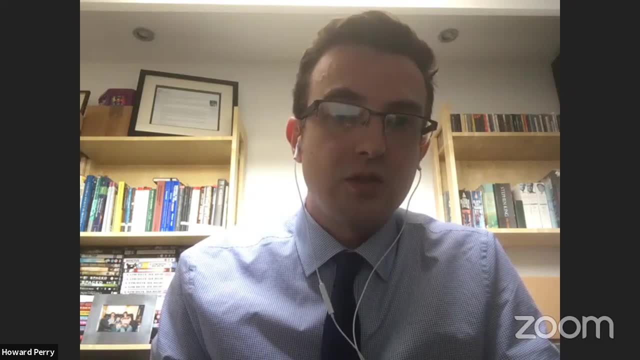 lowest bills now is not the best answer for the future is certainly true, but at the same time, I think Mike's point is that we need to do transformational things and we need to do transformational things and I think the point on there being untapped potential in the customer. 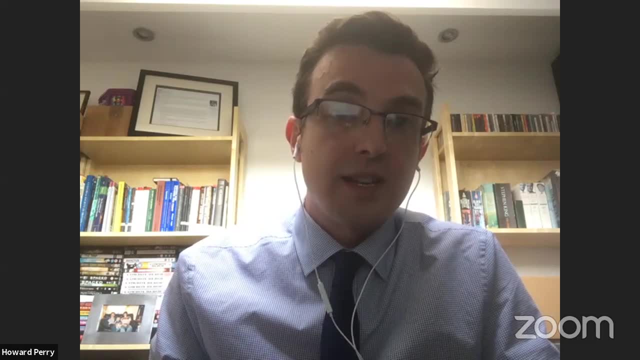 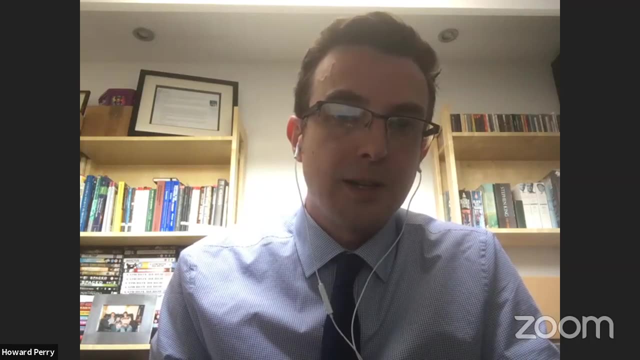 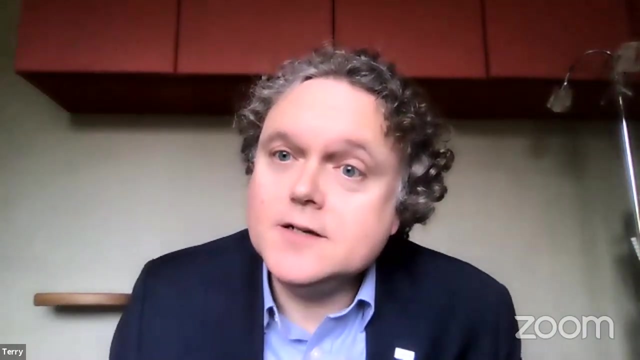 community and in behavioural change and particularly water demand, is true, There is much more that could be done there, but that's not for water companies alone. that's a cross-sectoral and including government thing. really Okay, thank you. Other blockers or similar ones who would like to make a? 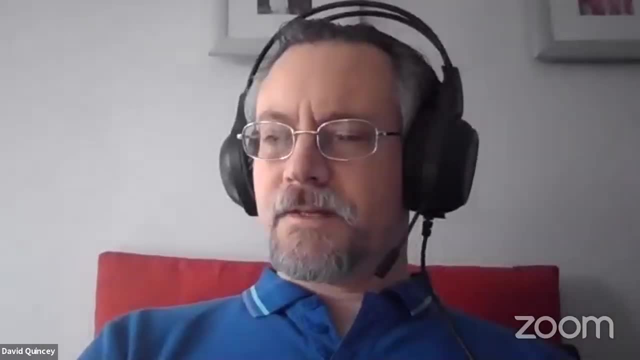 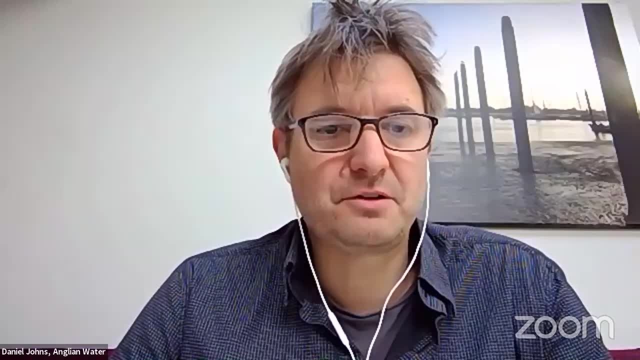 I think I'd say just slightly harking to what they just said there, with those we have a bit of a specific, odd one: been thinking about adaptation for 30 or more years. being thinking about adaptation for 30 or more years was to engage other organisations. 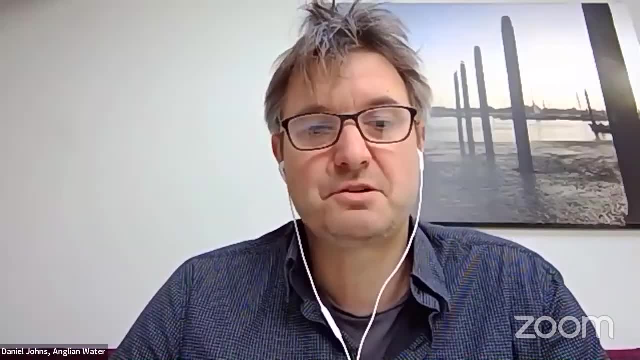 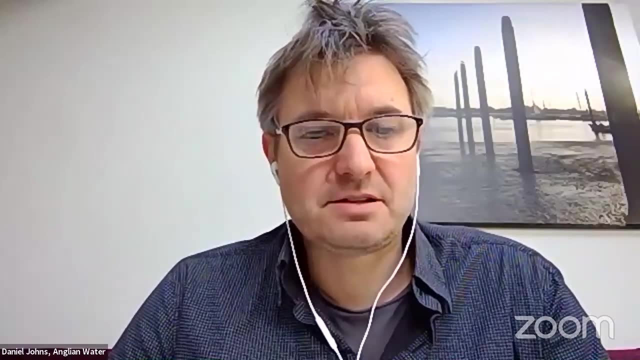 was to engage other organisations in what we are planning to do to get that feedback for even better. I guess that's how to say this. The Water UK team has produced a kind of a standardised template for the sector to make sure we were providing information on a consistent basis. 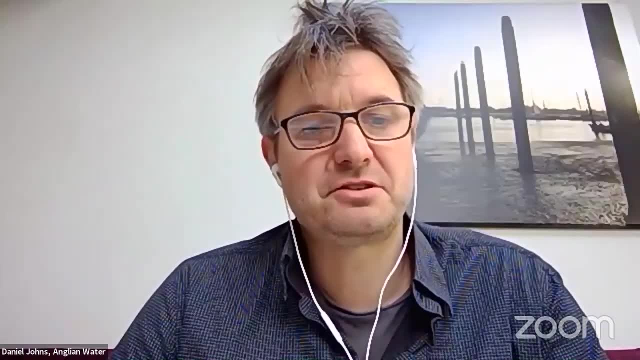 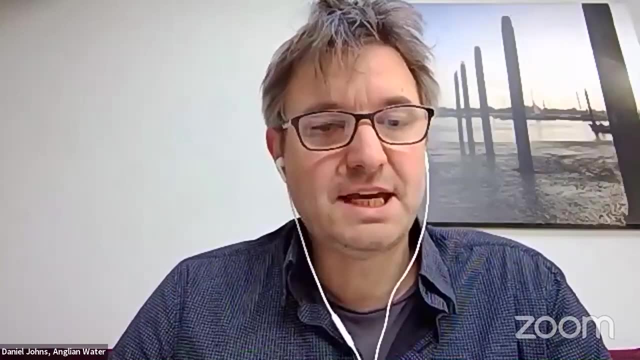 for the sector to make sure we were providing information on consistent basis And I think within the water sector, partly because we've been thinking about adaptation for 30 or more years- we injured some- treatmentNever that was too material in the course, So we were sort of at risk in terms of testing. 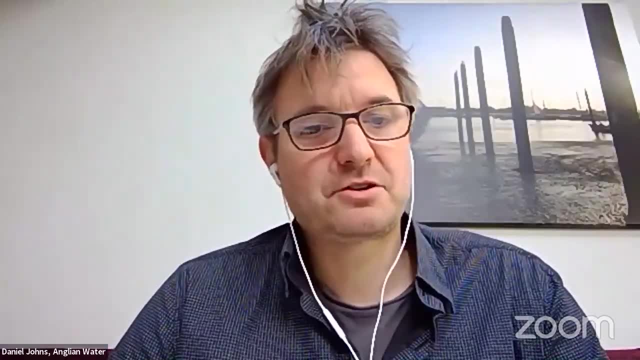 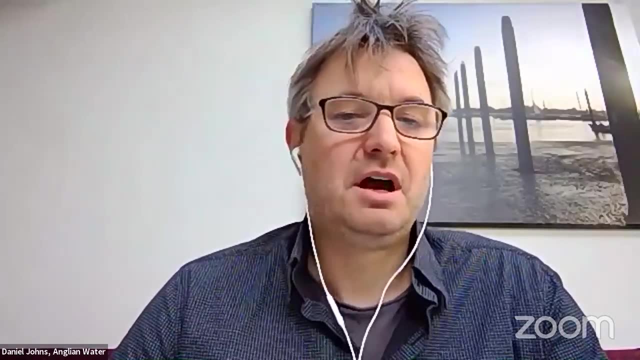 years and because as a regulated sector we've got common metrics that we are reporting on all the time to to off what the environment agency about pollution incidents, about leakage levels, about metering penetration and so forth, which i guess kind of picks up k's point about monitoring and 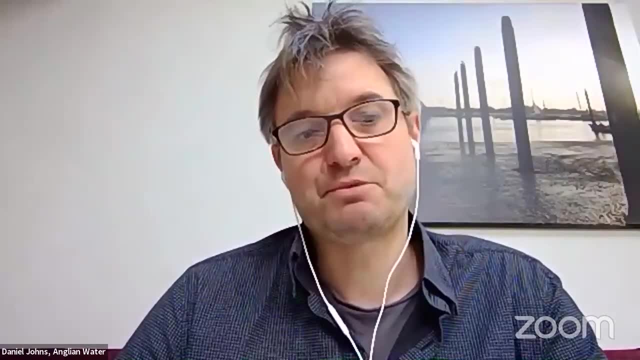 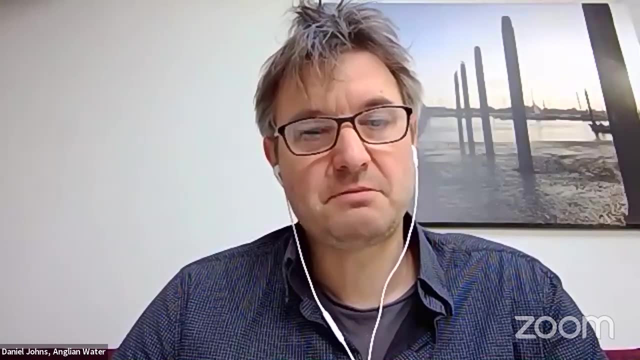 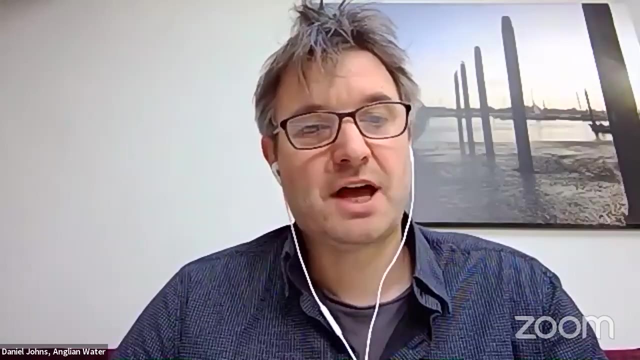 evaluation, certainly within the water sector, is relatively straightforward because we can monitor those things on a regularly, regular basis. and lastly, just say that we spent quite a bit of time thinking about our interdependencies within the report. there's a whole section on it which i encourage people to take a look at so that we are working very closely with those people. we 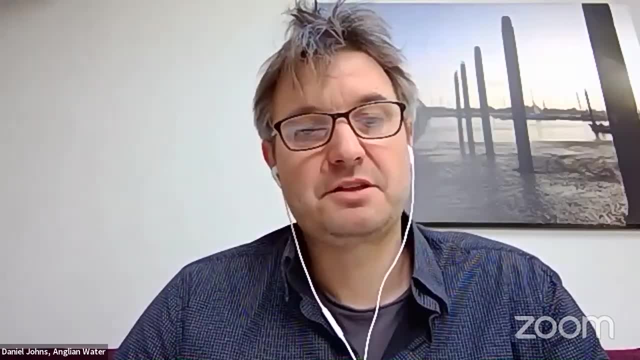 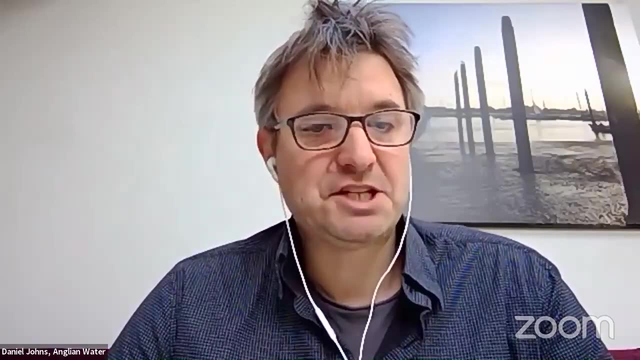 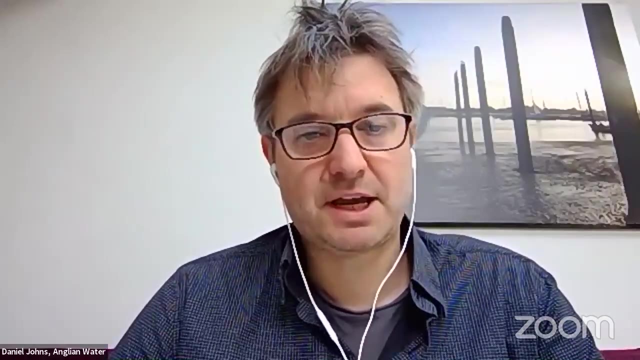 identify, for example, of course, energy suppliers, thinking about where our electricity comes from, but also, as part of our commitment to becoming net zero, we are deliberately becoming our own energy supplier where we can, through solar pv, thinking about storage, thinking about how we use our biogas resources and so forth. so, addressing 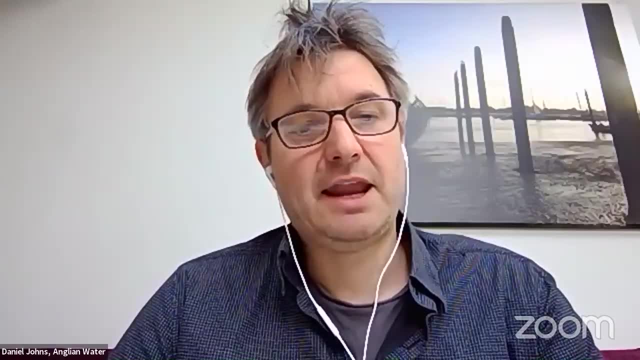 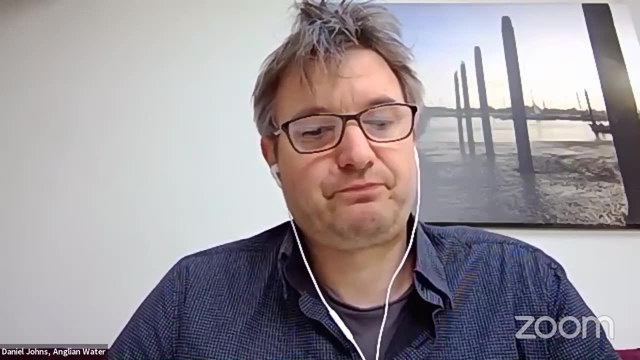 both those kind of transition risks, the business- and then also, where possible, addressing those independency risks at the same time. yeah and hannah, yes, i'd be really interested in your perspective. yeah, sure, so, um, as i mentioned, this is our first climate adaptation report, so we're 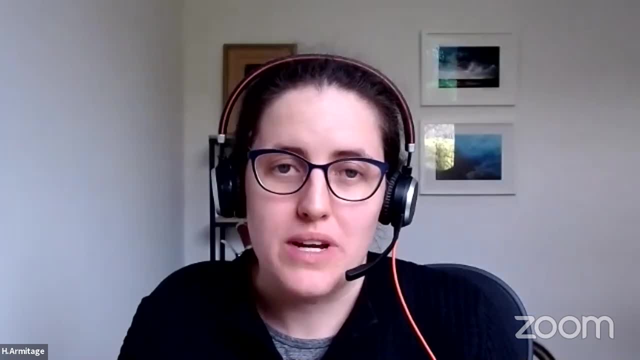 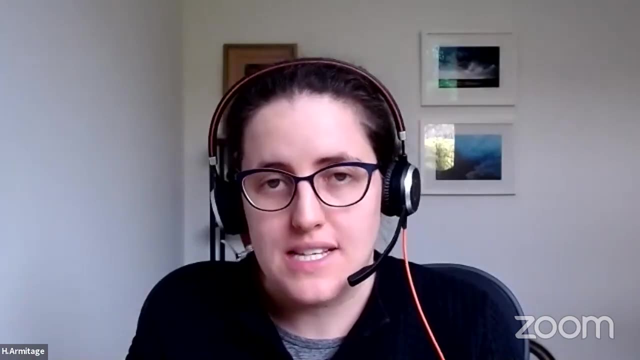 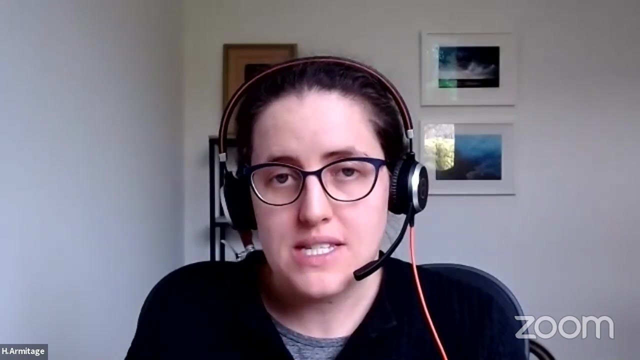 speaking to a number of people to get their perspectives. other financial regulators, like the financial conduct authority and the pensions regulator, are also going to be doing their first round of reporting in this um in this round. so we're speaking to them quite actively to ensure that, as much as possible, our consideration of the risks and our messaging 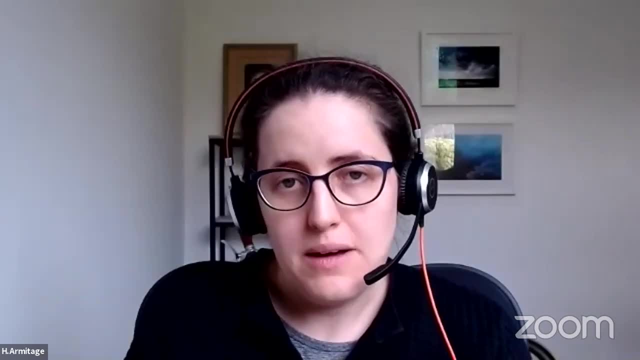 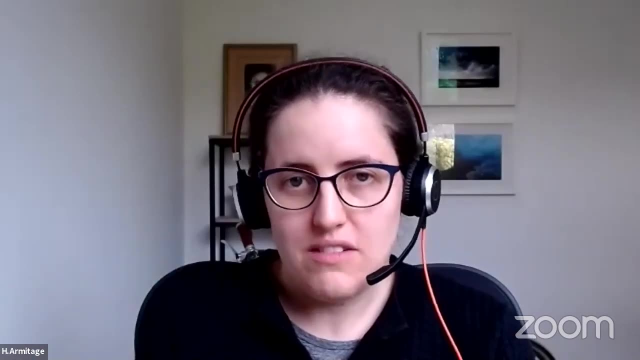 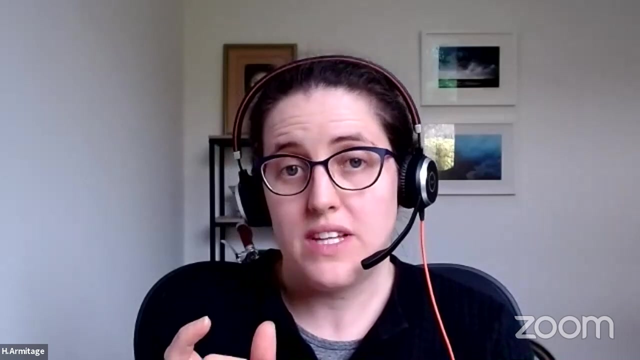 around, what we expect of people in the investment chain and from companies and lenders is actually coordinated and that we can get that, that message, out as actively as possible. as james mentioned, the bank has done a previous round of reporting where they looked specifically at the insurance sector. 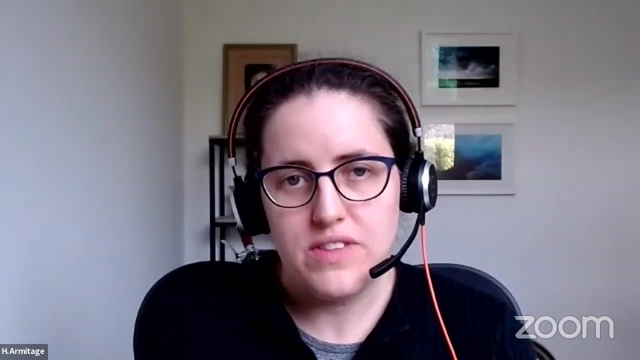 but in this round of the reporting they're going to be covering a wider range of their activities. so it's been quite active and we're going to be covering a wider range of their activities. so it's been quite active and we're going to be covering a wider range of their activities. so it's. 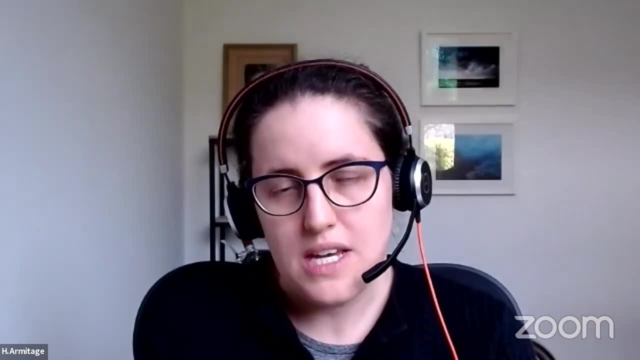 been quite active and we're going to be covering a wider range of their activities. so it's been quite helpful to speak to the bank about how they went to, about that, um, that process, and for us to coordinate across the four organizations to make sure that, as i say, as much as possible when we're 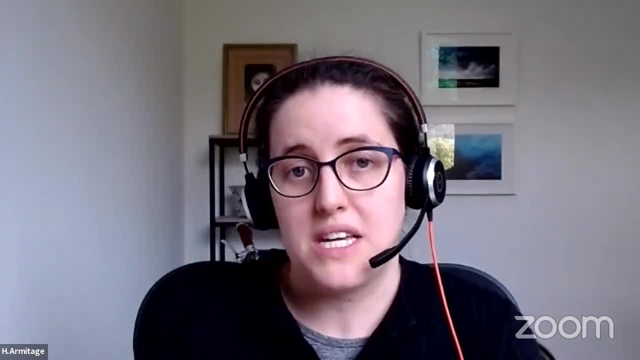 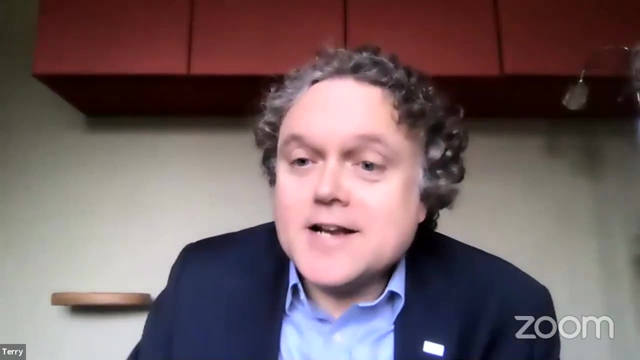 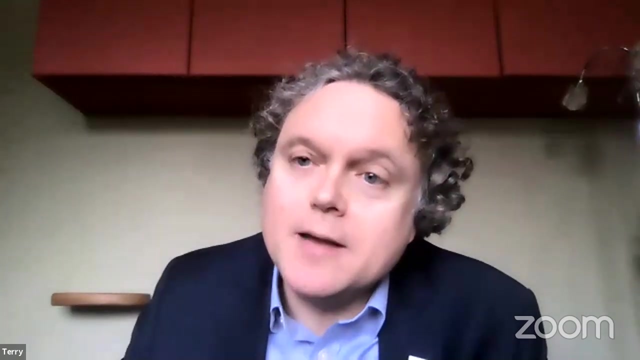 talking about adaptation. we're talking about the same things, we're talking about the same expectations and we're all pushing in the same direction. great, thank you, and k. of course, the environment agency has a strategic overview role, lots of partnership working within the agency and in various respects. have you been able to translate any of that into? 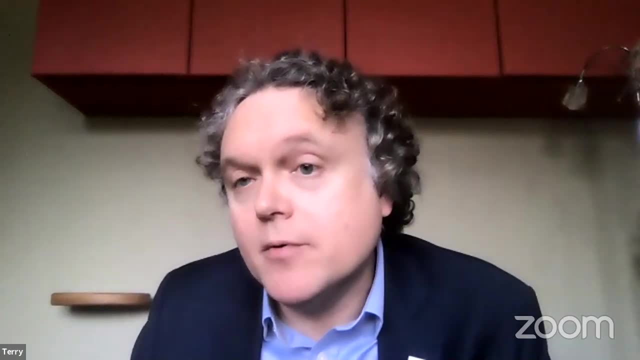 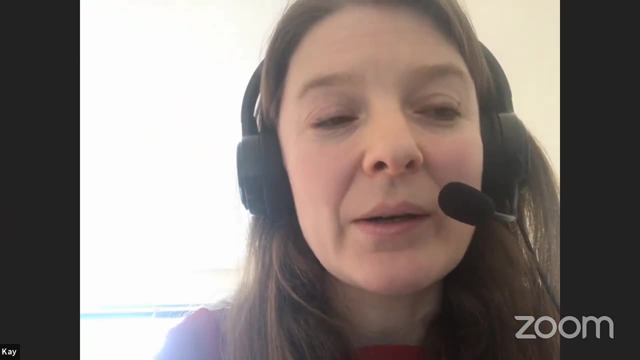 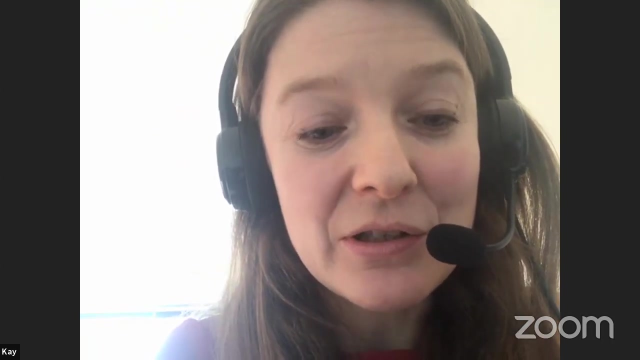 um, you know, cross-working around, uh, adaptation reporting? um, yeah, i think, as you say, a lot of the partnership working we do is embedded within other things. obviously, we did set up the infrastructure operators adaptation forum, um, back in 2012 in recognition of the importance of 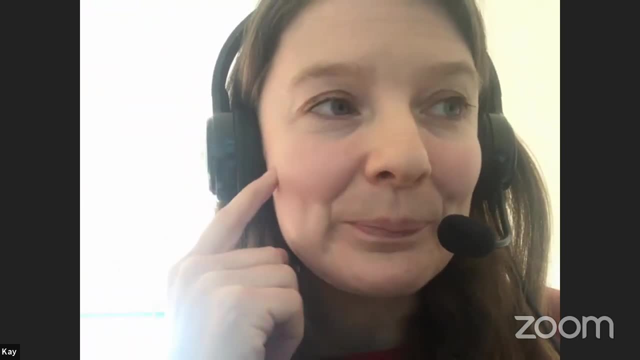 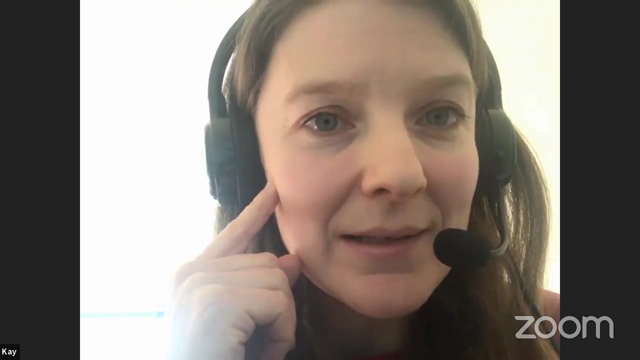 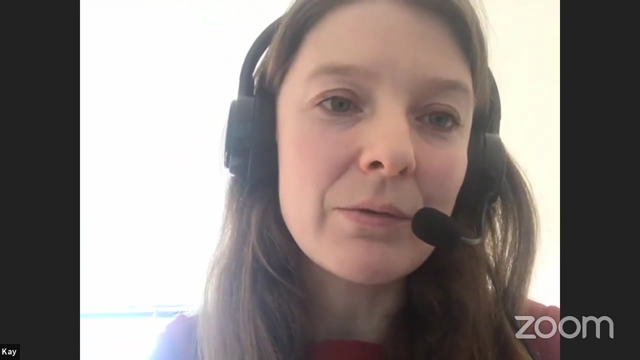 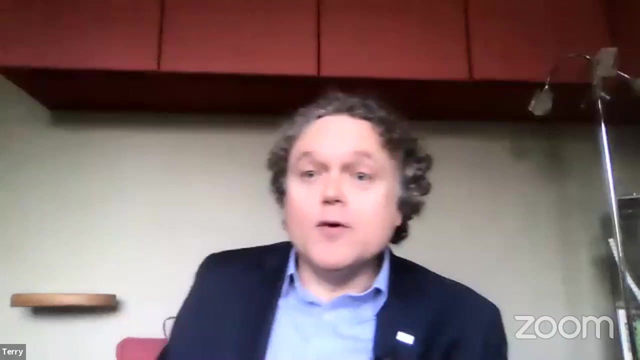 talking cross-sectorally about these issues. um, within our sector- there i mean that would be natural england and forestry commission- are there probably fewer commonalities than perhaps with other sectors. um, but but yeah, i think the cross-sector stuff is mostly embedded and then through the, the operators forum. so, yeah, great, okay, thank, thank you very much. okay, we're going. 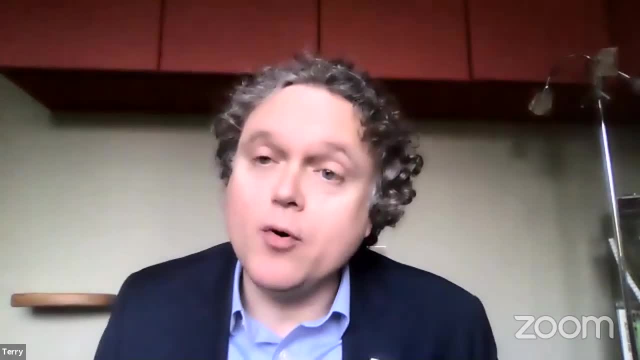 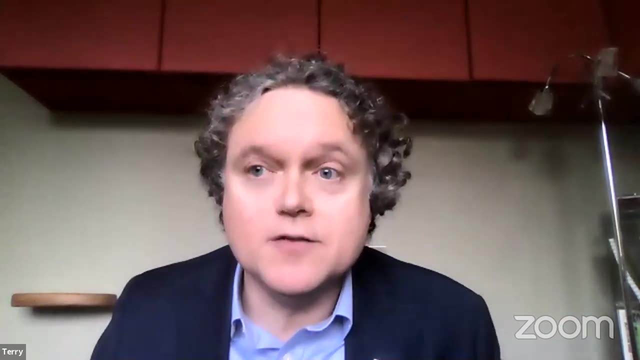 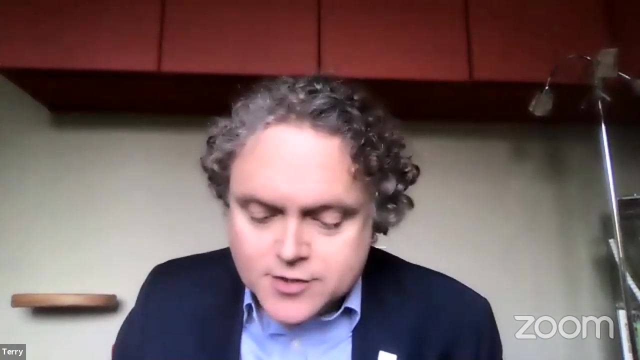 to move to um. another question, and again it's about um reporting and and really i think it's touching upon how the reporting and the effectiveness of that reporting is a real opportunity, if we get it right, to actually make progress, to influence, to change mindsets, behaviors etc. so with um, with a view to um last. 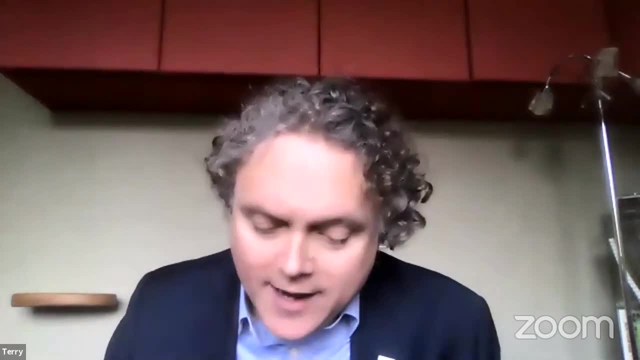 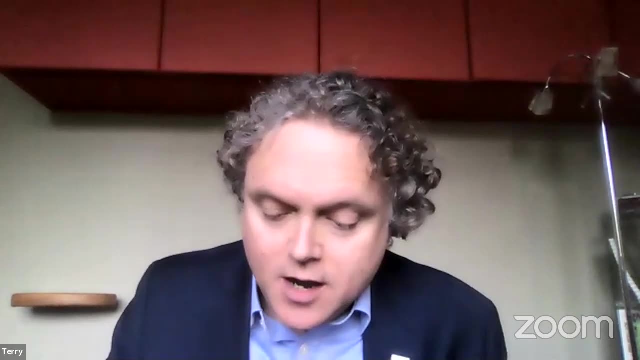 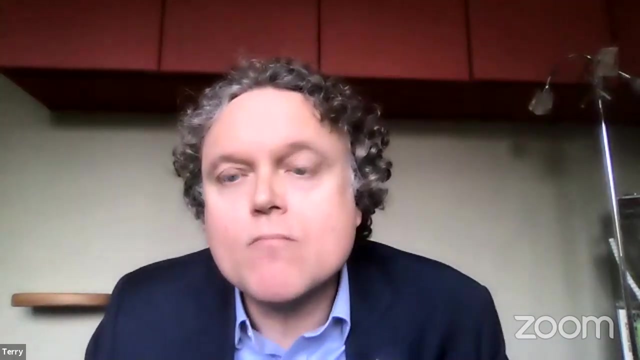 time and looking ahead to this time, what was it in the way that you actually reported last time that made a difference? in other words, was it presentation of risk, um, communication with stakeholders? what were the most effective things about the way you reported? can i come in on that? yes, please, um, yeah, so. 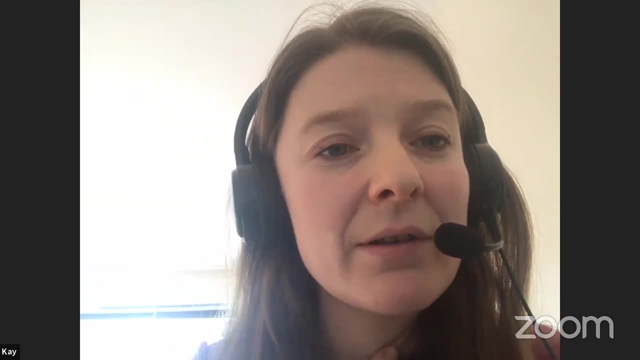 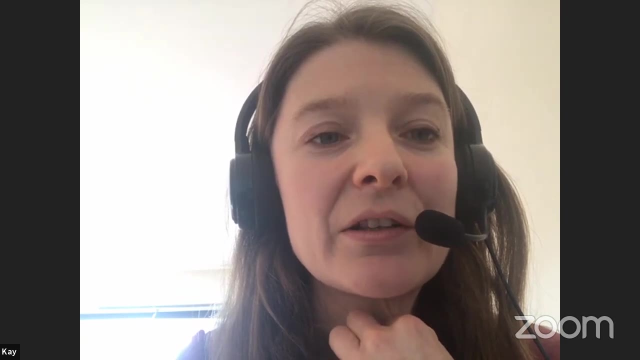 i think the most effective thing that is, uh, framing our risks around our corporate objectives. so, rather than just presenting random impacts, um, looking looking at the sort of aims and goals for our business as a whole and describing the risks around that worked- worked really well as a way of presenting the risks. um, we had a really strong governance structure, so we had senior level. 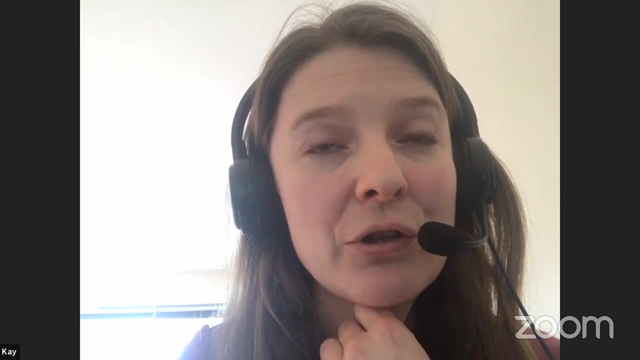 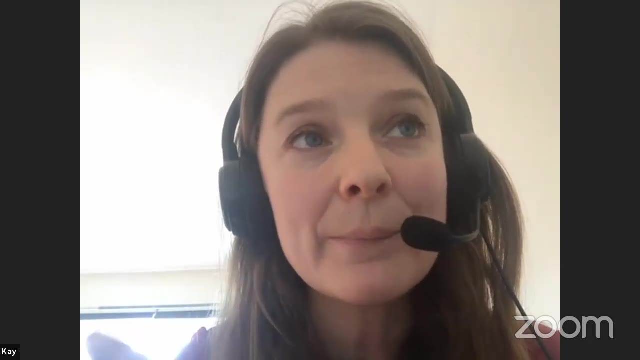 um project board with clear leadership, working level, technical groups to get input from across the business and all the right techniques, and so i think that's a really good point and i think that's a really, really great point and i think that's um, that is definitely important to. 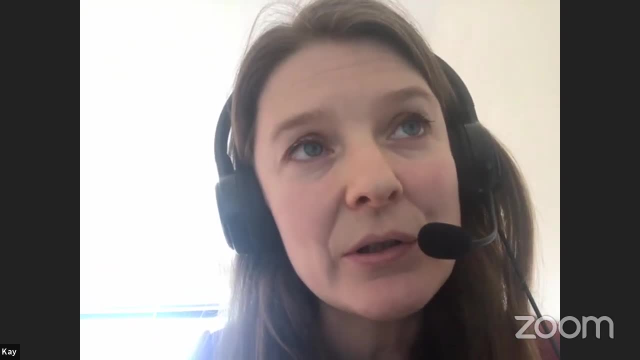 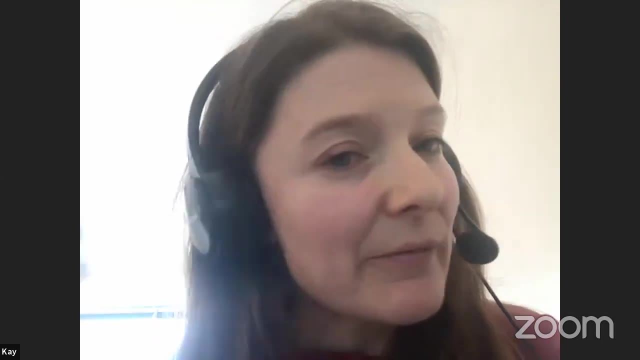 think about. so i think that that's a really good point, um, so i think it's also a really good point from me that, um, we didn't get into the director's office because we could not understand what that made us, because we could not get in and out of that project. it was. 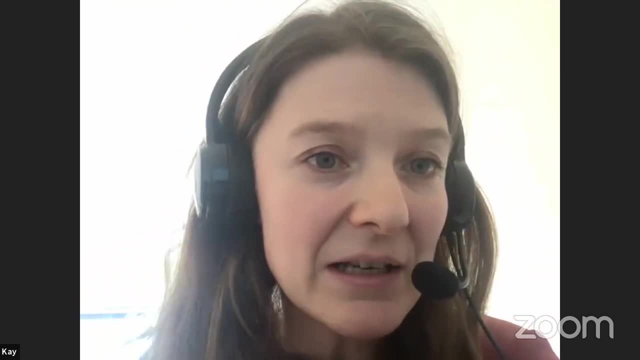 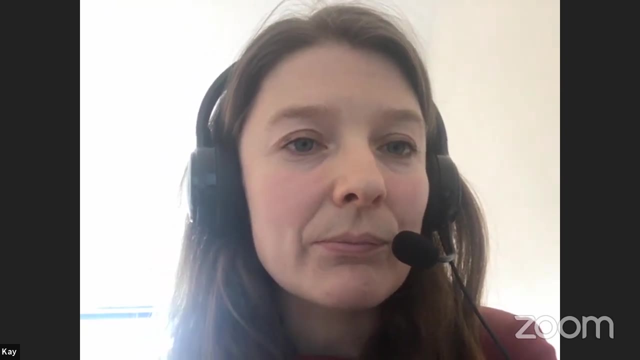 it was a really great um thing. so, um, we did have a lot of talks with our team about some of the staff and deep learning that we were able to get into, but i am still working on that project. so, uh, making sure that the the the technical groups that we had in place. 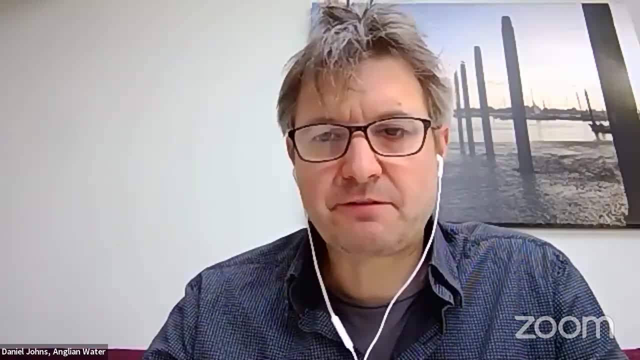 are very consistent and take into account all the things that we've been working on. so I mean so on our third report, I covered it very briefly, but essentially this is the first time where we've tried to actually define in a way that's consistent with our corporate risk register. 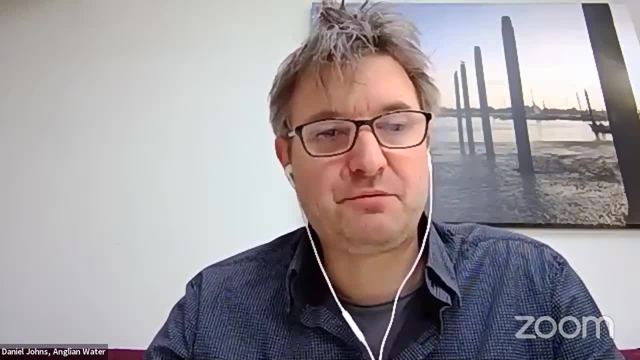 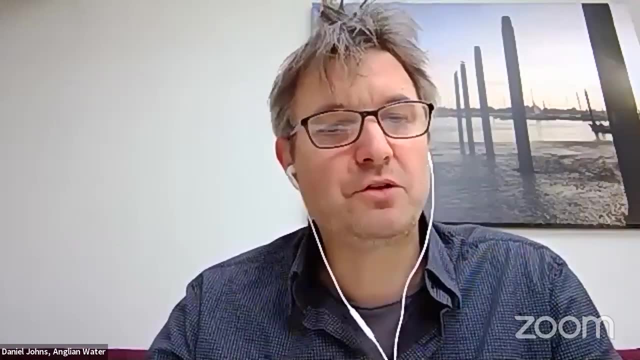 both what the kind of raw level of risk would be if we took no action, where we are currently on that risk management journey and where we'd like to get to both in 2025, and what the kind of long term target level of risk will be. 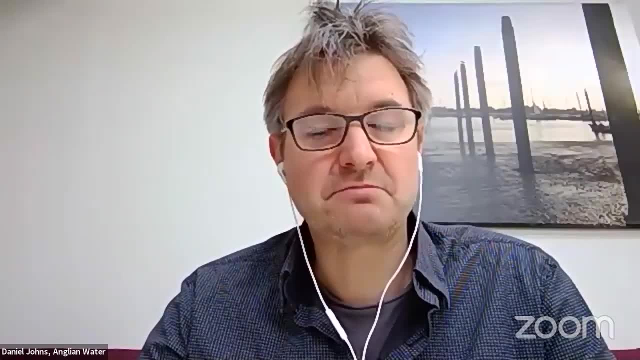 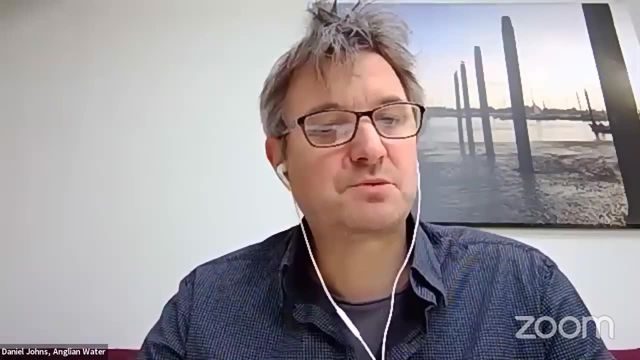 And that recognises that we're not going to be able to reduce risk to zero. There is an acceptable and appropriate and cost effective level of risk that we should achieve, And in some cases we're quite close to that, But in other cases we've clearly got some distance to go. 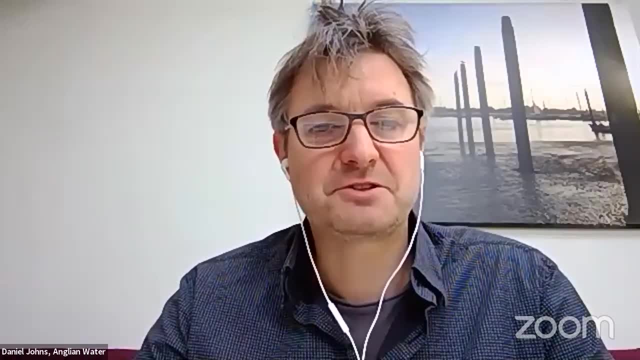 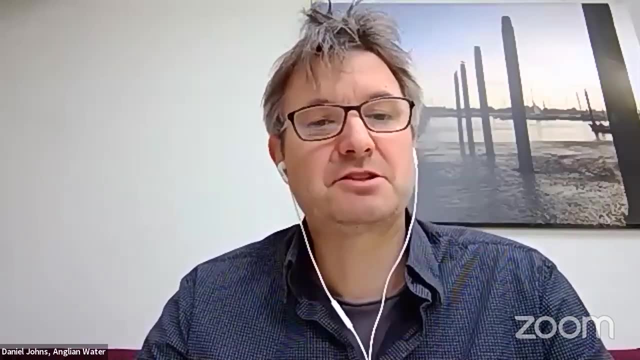 And I think that's really been helpful to both define for ourselves, you know, just realistically where are we on this journey, And to recognise that there will always be a need for that kind of resilience, I suppose, to be able to recover quickly, to be able to respond to events as they occur. 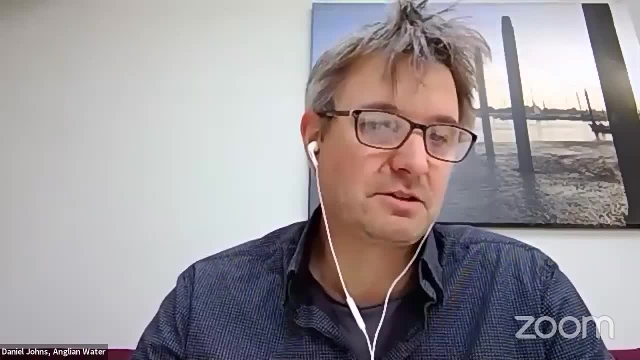 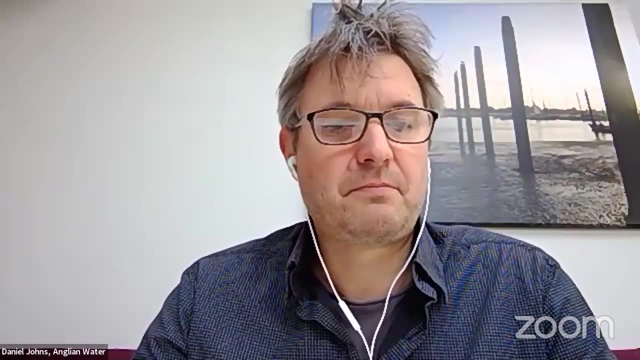 and to make sure that we are ready to go And to kind of protect customers, which, of course, is ultimately the aim of everything that we're trying to do in this space. Thank you, Daniel. Anyone else like to come in on that? 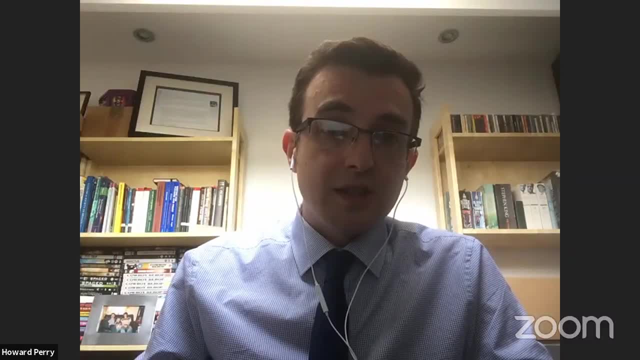 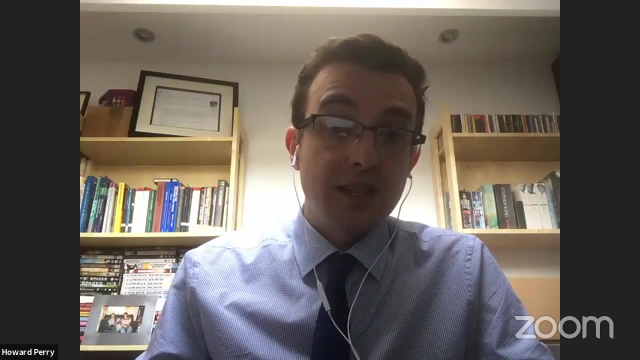 I think one of the most effective things that the ARP gives you is a simple- if you can summarise it- list of what your risks are that you can then take to people who perhaps haven't considered climate change before and say: have you considered these things in your planning? 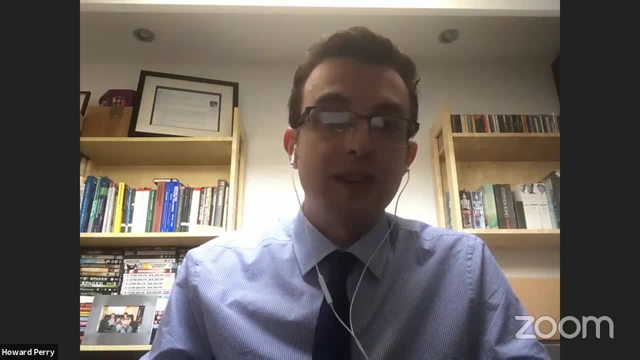 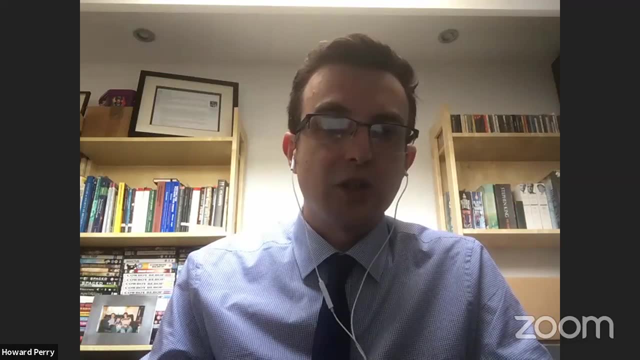 So having that very simple list of this type of future will It will mean this type of impact for us. Is that considered? That goes a long way in getting it considered and worked into planning. If you haven't got that- and it's all a bit amorphous and people just look at the very widespread of potential scenarios- it can be very difficult to do anything about. 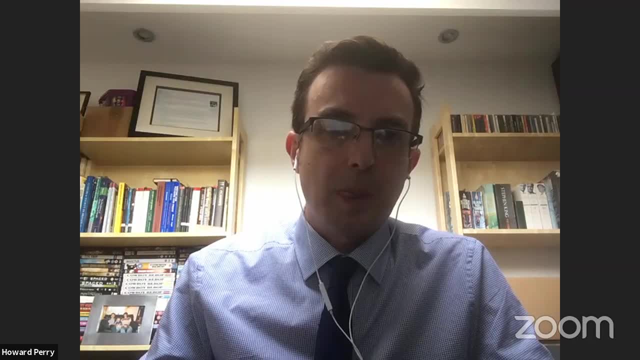 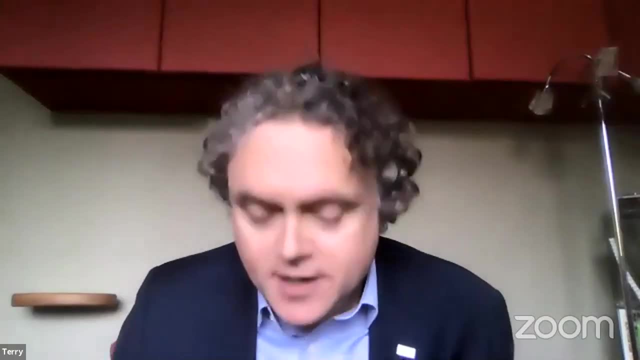 But once you've got that simple list of risks, it's much more usable for people. OK, I mean, I think there's a question here from Nikki Van Dyke that maybe follows on from this a little bit, And it's a question around: how is adaptation reporting? 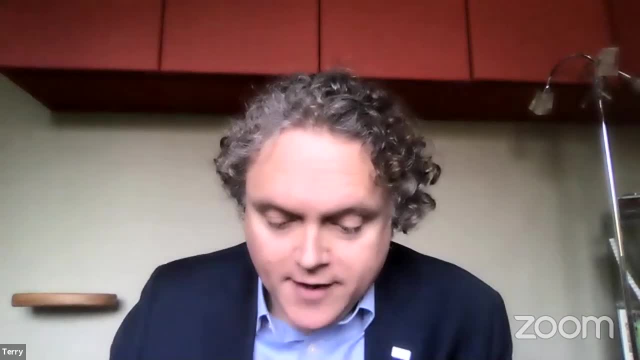 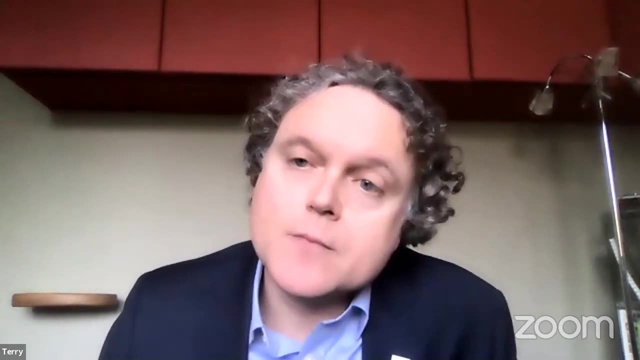 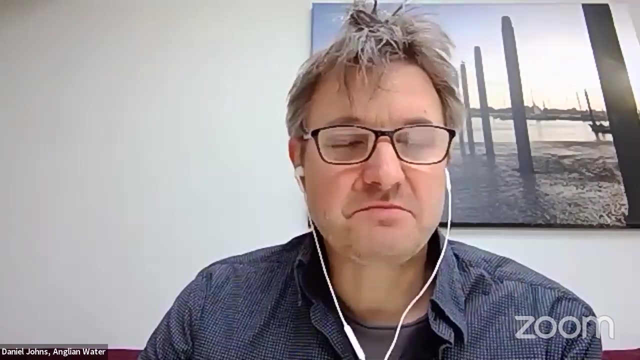 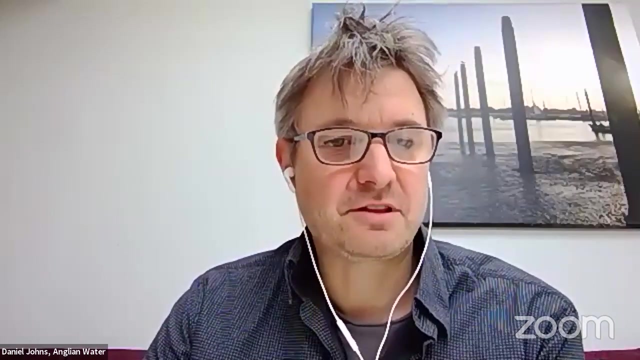 How is it being reported and viewed at different levels within organisations, for example, board level, operational level, et cetera? Again, so the basic ethos is that climate change adaptation is integrated into everything that we do. that it's not. the ARP report was not an exercise that was done to one side and kind of bolted on to the business. 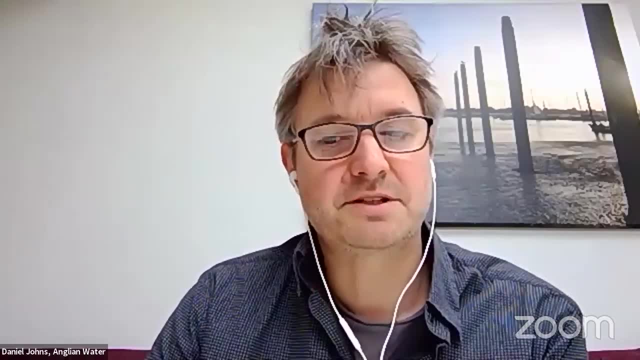 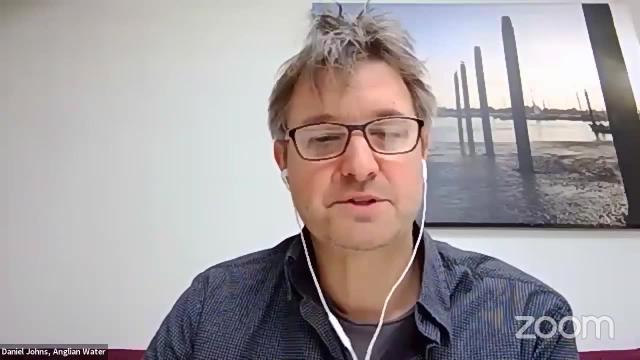 It's kind of retrofitted into the business strategy. It's absolutely core to the business strategy And that's reflected the reason why it's our chief executive that signed off the report. There were board level discussions to make sure that everyone was happy with the assessment that's being made and whether or not. obviously there are certain aspects of the risk that we need to be managing. 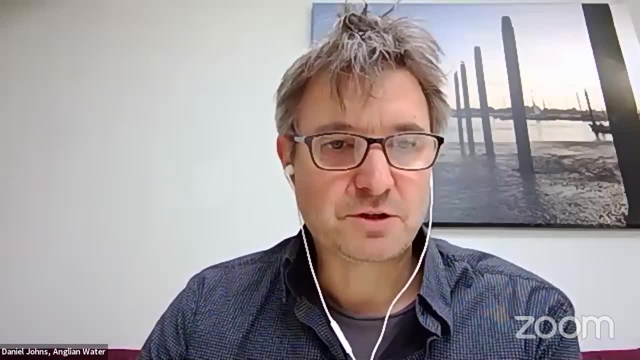 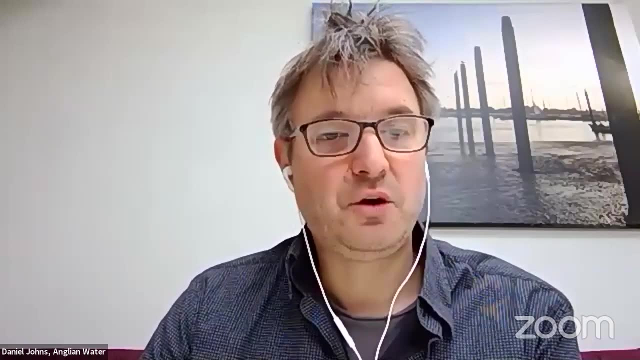 I think it's also to recognise that, as we talked about earlier, it's part of our task force of climate related financial disclosures return, which we've done three times, and also our general approach to climate change, both in becoming an xero business by 2030 and 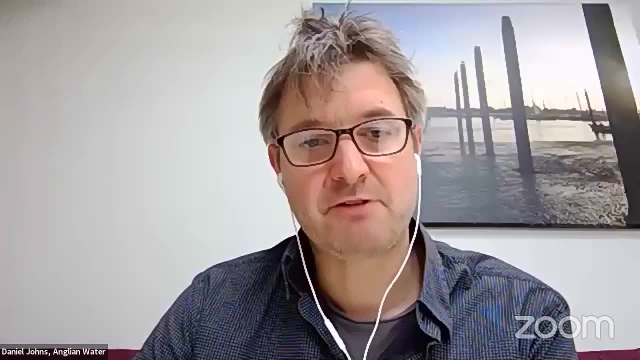 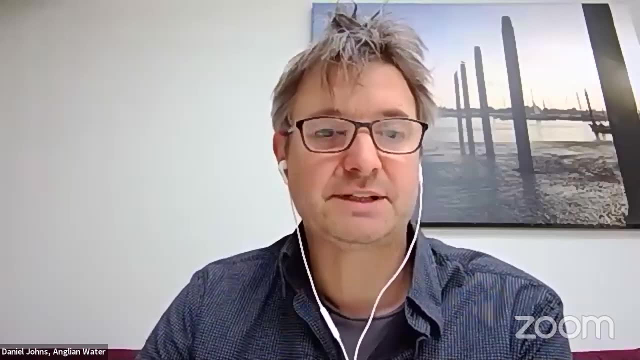 having a strong story to tell on adaptation was core to us being given an a rating by cdp in their latest climate change assessment for christmas. we're the only water company to get that a rating. we're very proud of it, but what that means in practice is that we can then 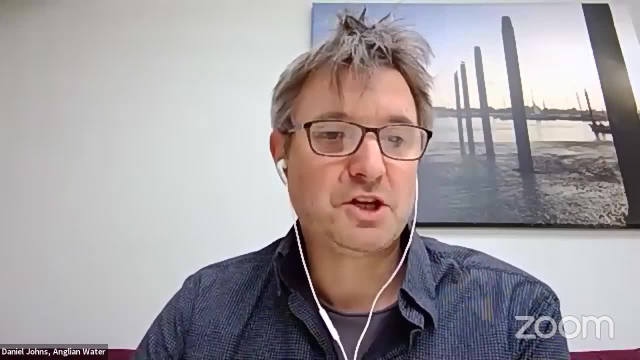 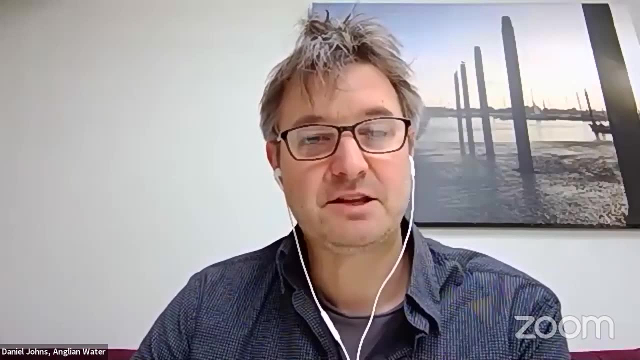 sell our business to investors and we can attract the right kind of investors who have the long-term view in mind- pension funds and other institutional investors who are willing to invest in the business. and also means that we can attract- even if it's by a couple of basis points on the cost. 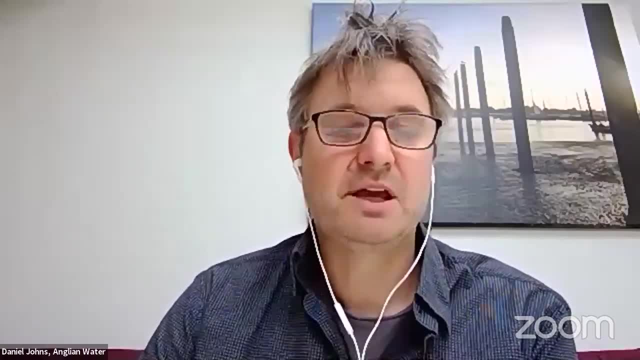 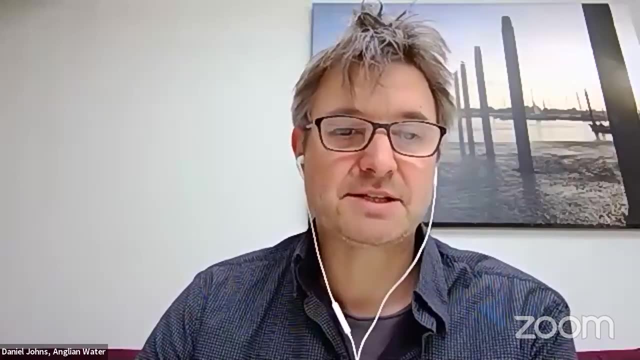 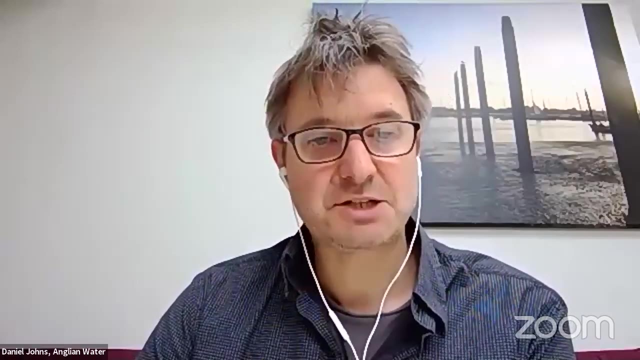 of capital for the billions of pounds of investment they bring in. that makes a real financial difference to our bottom line. so having a good climate change story to tell, being a net zero carbon business is absolutely uh core to our kind of esg credentials and and is having, say, tangible impacts on the cost. 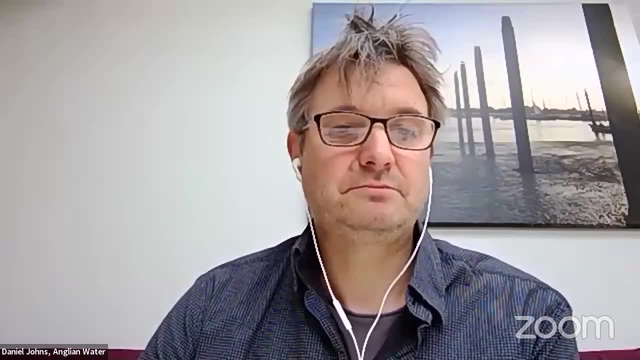 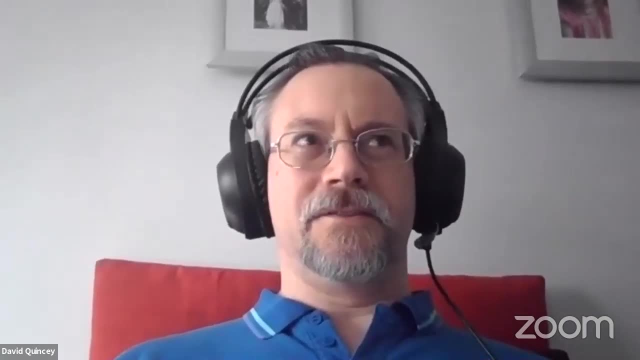 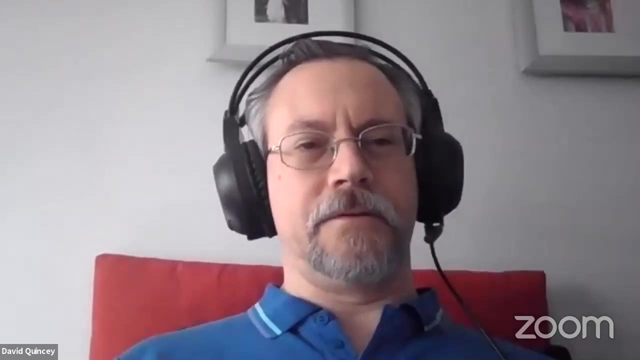 of borrowing and going forward. thank you, i think i've beat me to the punch there. um, i think it the short answer to the question. what does it mean is: it depends on where your company is on the journey. um, you probably mirror it back with sort of environmental reporting many, many years ago. it initially maybe. 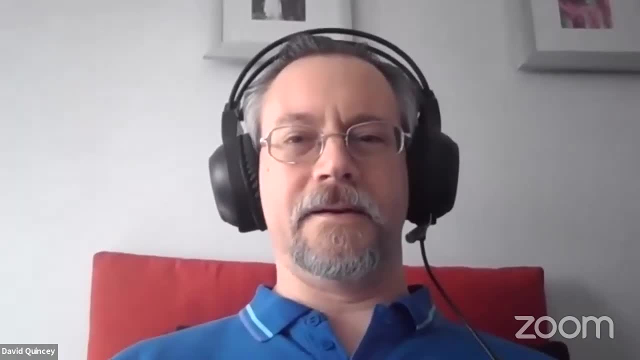 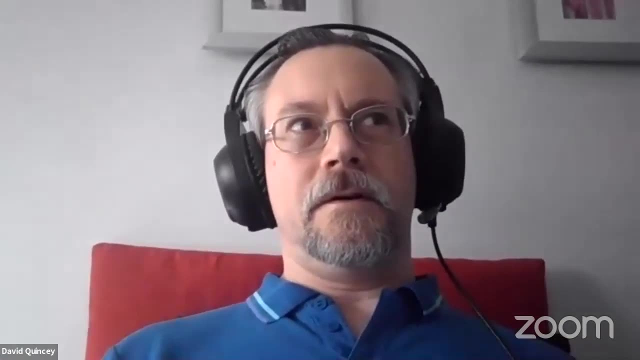 starts out as a you know, a nice to do or a um. it's seen as a um, a reputation seller or something. but once you have done that, you're going to be able to sell your business to investors and you need to have a business plan to ensure that it's done it once or twice and they understand the. 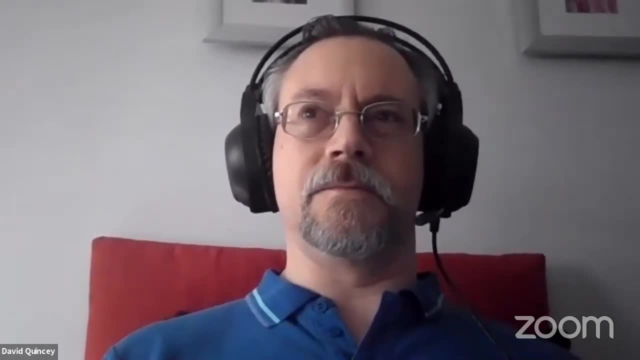 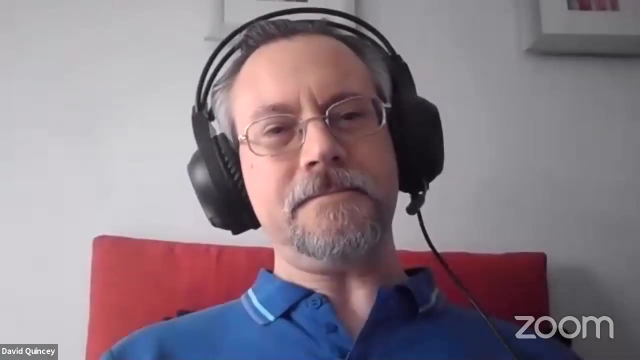 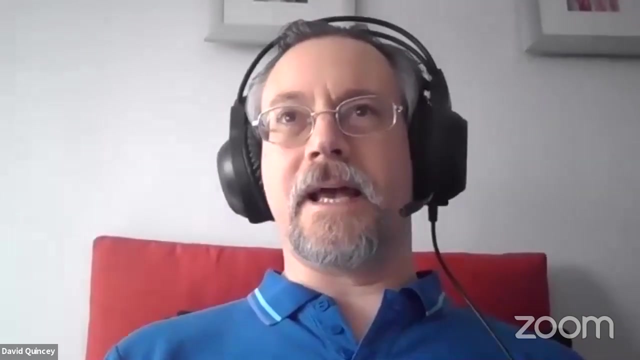 mechanism and once the issue of climate change, climate adaptation, becomes core to your business planning, it becomes recognized as a strategic planning tool, and i think that's where, um, i can remember that journey to angling water and i think that's when it rail are at this, this as of now. 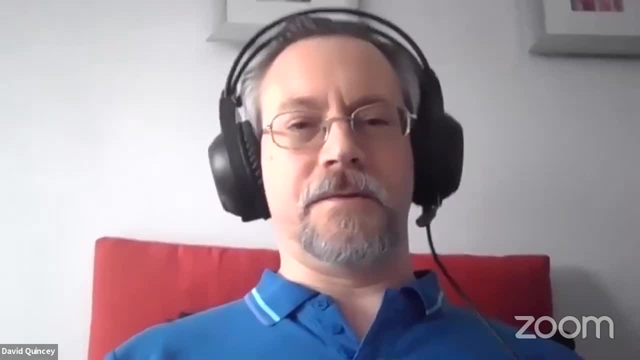 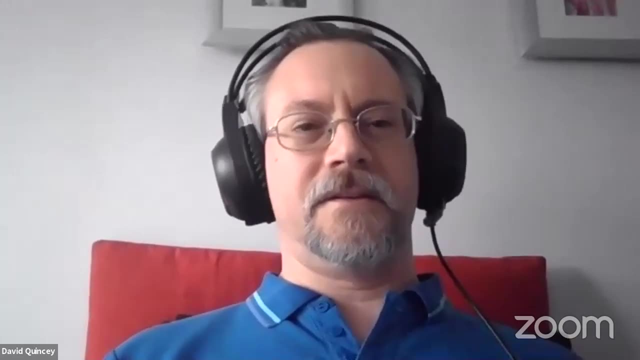 climate change is is now a level zero risk, which may not mean anything to anybody else, but it's our top level of corporate risk. it's been moved from one to zero, and so it's now a board managed. the adaptation report is going to be signed off and reviewed by the board because they see it as: 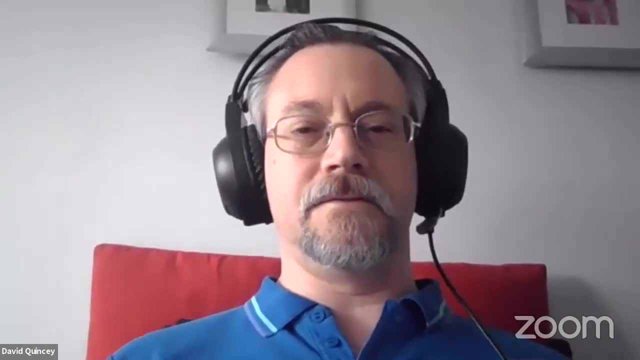 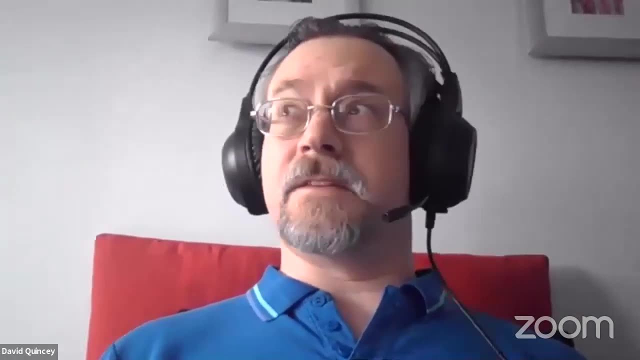 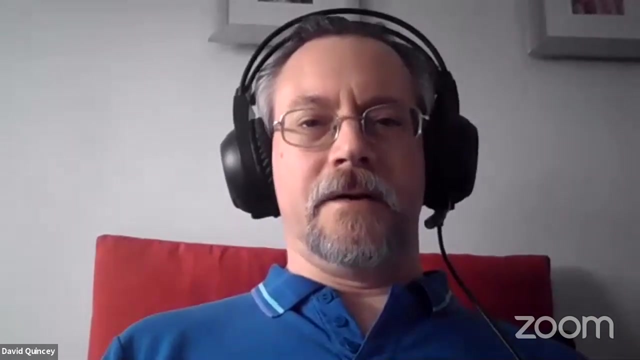 part of the, the journey of integrating and delivering the solution to this risk. um- and, as i said, it's going to be aligned with our recently um published, as september last year, our environmental sustainability strategy, which lays out our strategy for the next 50 years. so it it becomes. 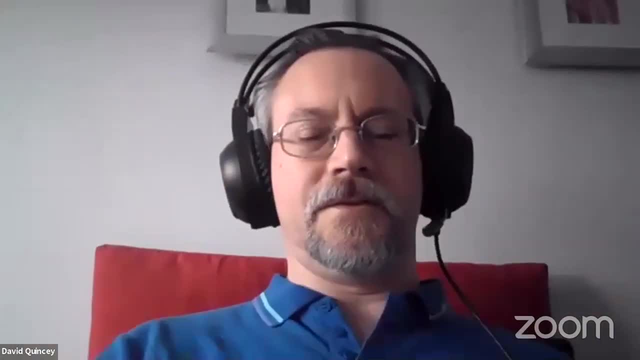 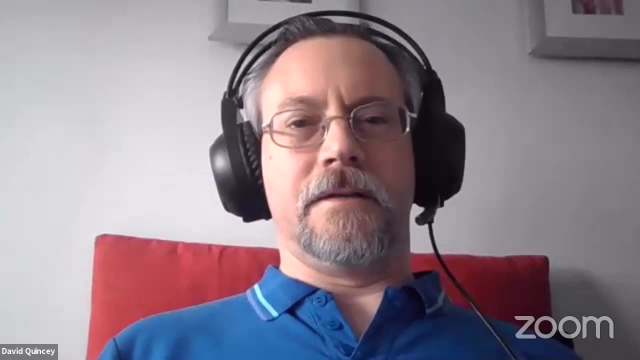 part and parcel of the strategic delivery. how it's then seen within the different parts of the business going down the chain, shall we say it depends on the level of communication and what you're doing and and the degree to which you engage the various teams towards the front line. 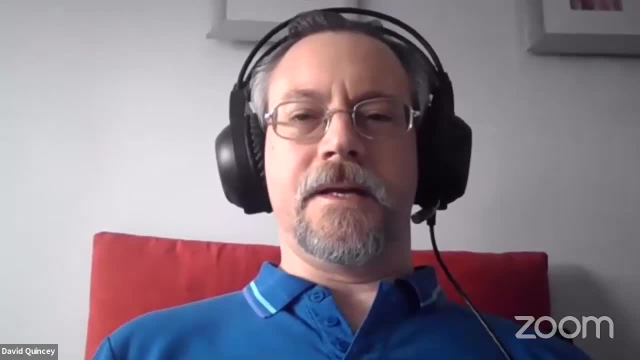 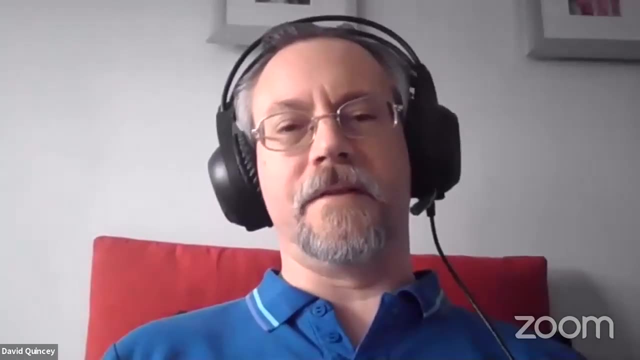 again, that's a journey, um, it's about making it relevant to people's roles and jobs and making them understand what the risk of climate change is, to their ability to deliver their service to the company and the customer. and again, i think we're, we're on that journey, i think we've, we've. 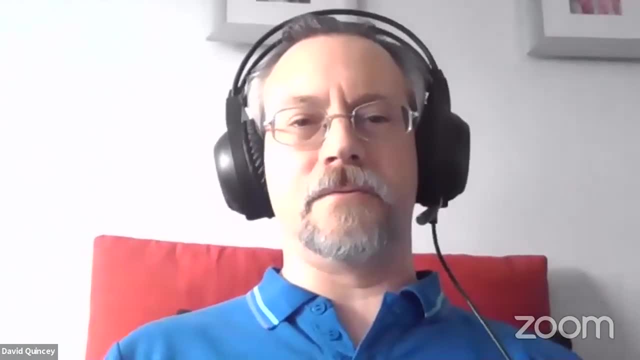 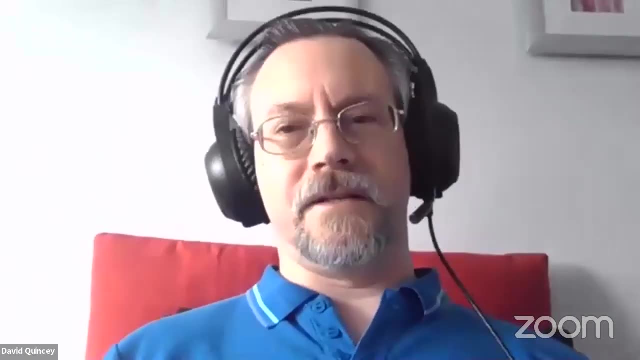 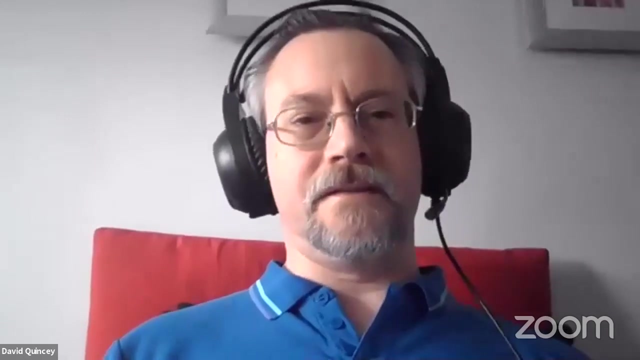 we've improved from last time. um, we're not just doing this as a central strategic thing. it now involves our routes and regions and they're engaged in actually delivering the actions in the plan, generating the actions in the plan. so now it's- it's a much more accepted part of the business day to day than than a report. 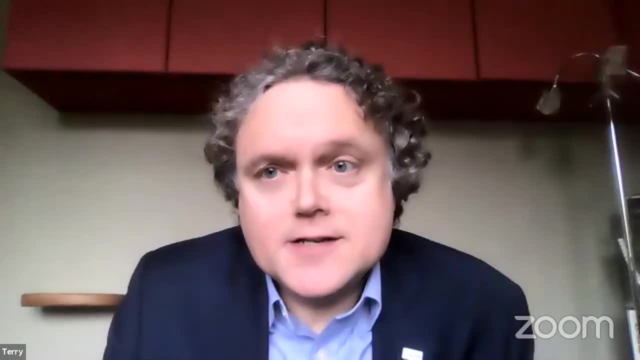 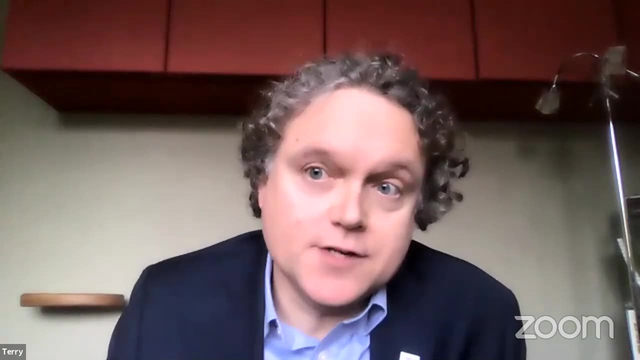 okay, thank you, i mean. what i would add to that is that, yes, the reporting is a is a very um integral part, or needs to be a very integral part, of planning, but it's also about influencing and winning hearts and minds as well, and i think being able to translate that reporting into something that that's. 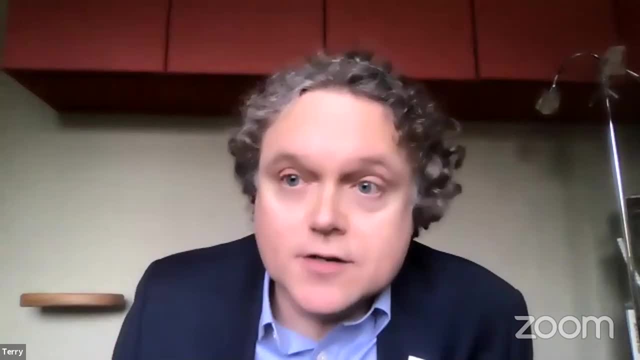 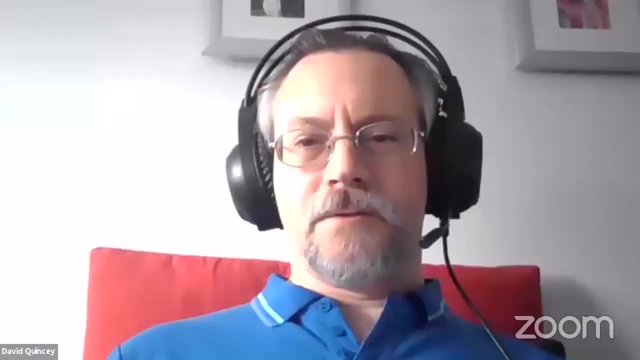 meaningful to the different um operations and and and um aspects of your organizations is is a really important going forward. i would suggest- sorry, howard's point about that. this was really valid and it was sort of what i said in my um piece about what- what the value is to us. 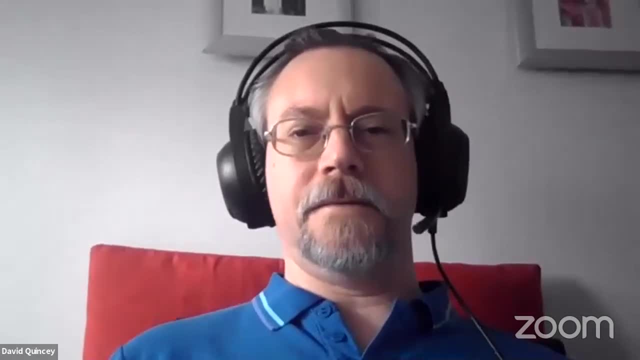 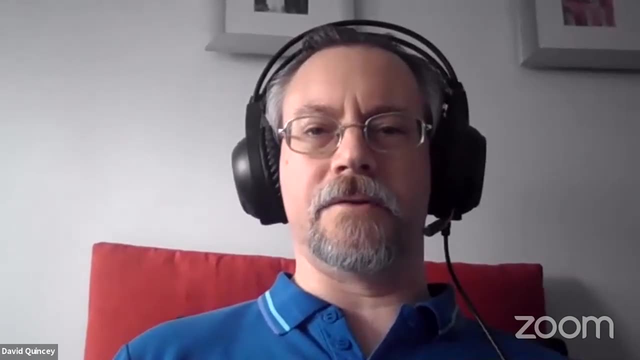 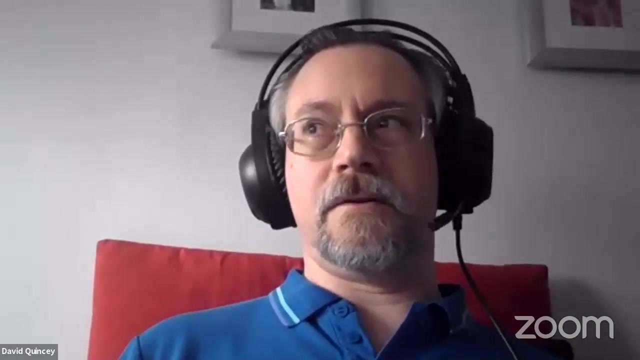 at its most basic level, it provides a punchy set of graphs, tables, messages, bullet points. it lays out for people in a way that they can read it in a few pages. what's the core offering here, what's the point, what the takeaway message is? it summarizes a lot of very complicated work. 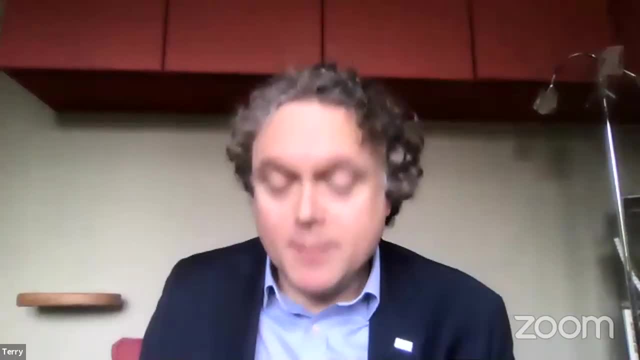 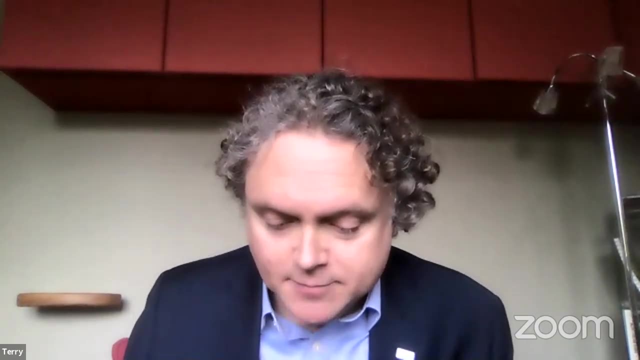 in the background. yeah, indeed, okay, thank you very much. i'm going to move on swiftly now to a final question. we've just got a minute or two to take this um, so again, perhaps some succinct answers please. but it's um, it's a comment or a question from um, from gerard davis, i'm going to ask you a. 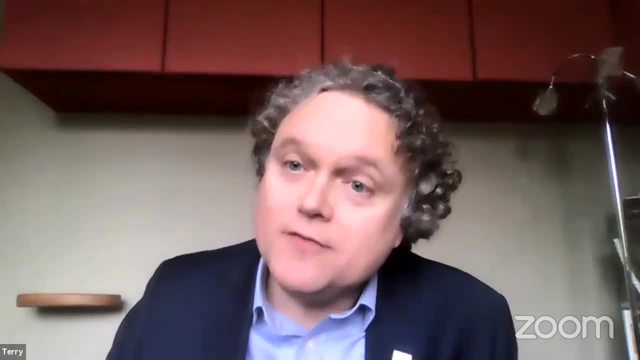 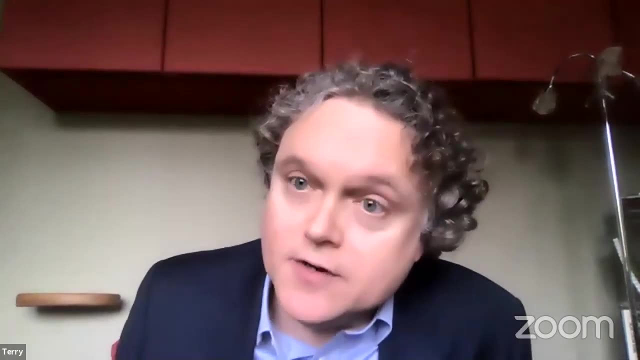 about how um you're collecting data from down the value chain, um supply chain, in in your organizations? um you know, and are you interested, what smes are doing, for example, that are an integral part of your, of your operations. so who would like to give an answer to that please? 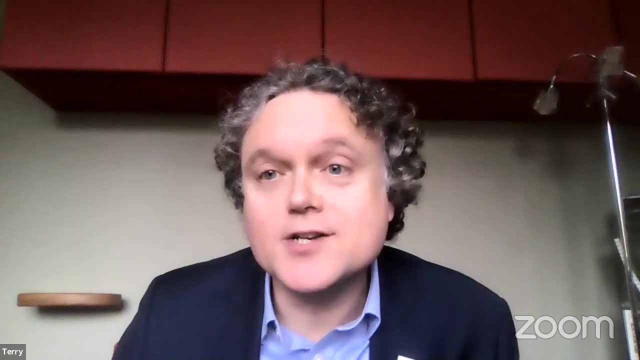 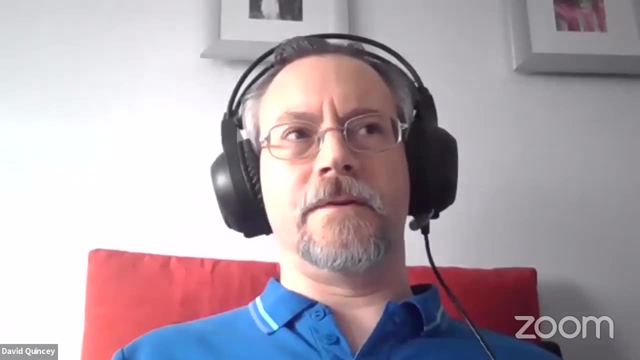 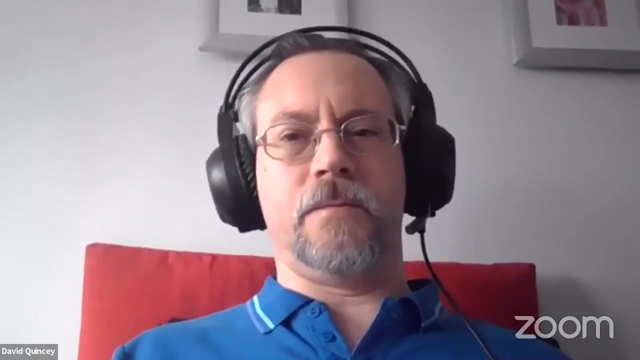 working with supply chain. i'd say that's our next challenge, or our current challenge. um, we've spent a lot of time understanding our risks. we've spent a lot of time developing our, our capabilities internally to think about climate change, where it will hit us and what we need to do. 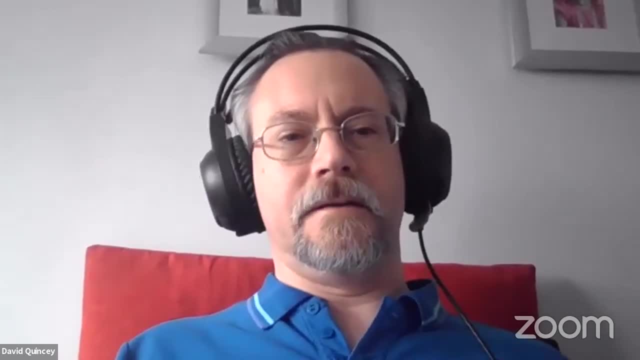 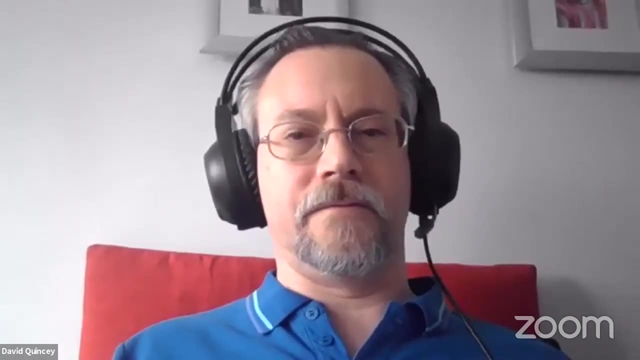 about it and we're now moving into the arena of delivery properly, and there's a big recognition within this, particularly when you're dealing with large infrastructure and, in our case, very old infrastructure- 200 year old embankments and the like- and tunnels that can't just be closed and 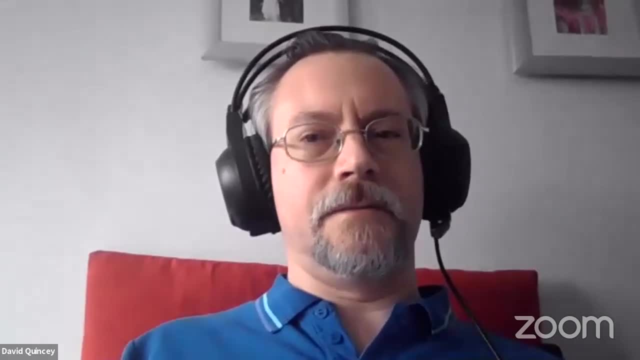 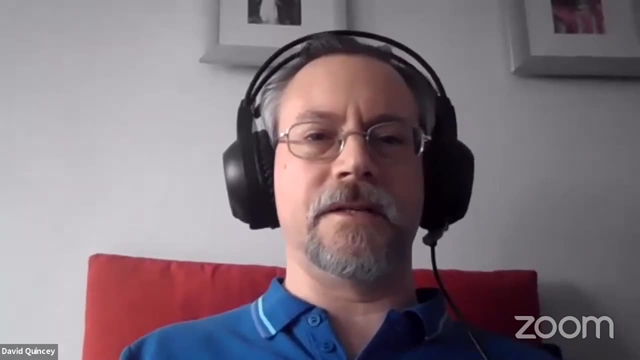 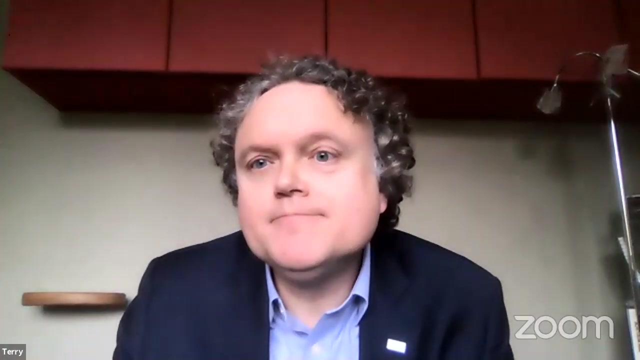 rebuilt um. a lot of innovation in the supply chain is going to be needed and partnership to to deliver adaptation. we cannot do it alone and we cannot do it through solely capital investment in carbon intensive concrete or whatever. thank you, dave. any final thoughts on that? yeah, i just say um. so just on capital carbon, for example, we've set ourselves. 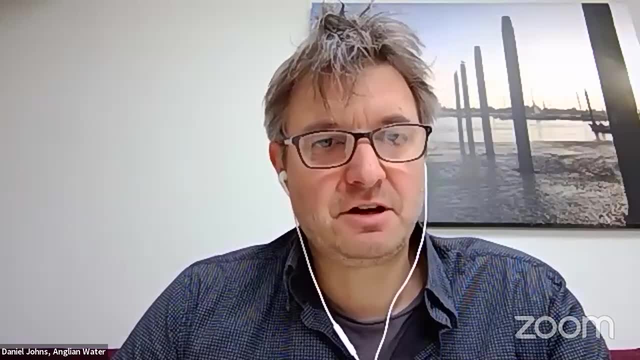 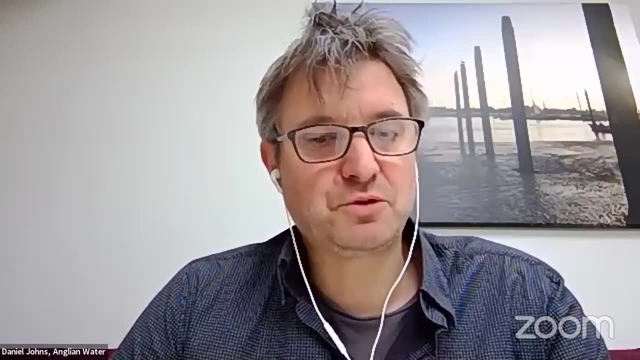 a capital carbon target. i've had that for 10 years and actually focusing on carbon means that you're also thinking differently about the assets that you construct uh and, for example, taking you much more towards nature-based solutions, because they are both uh have low carbon footprints. 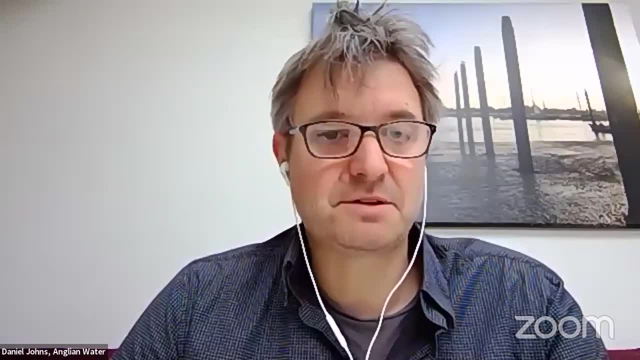 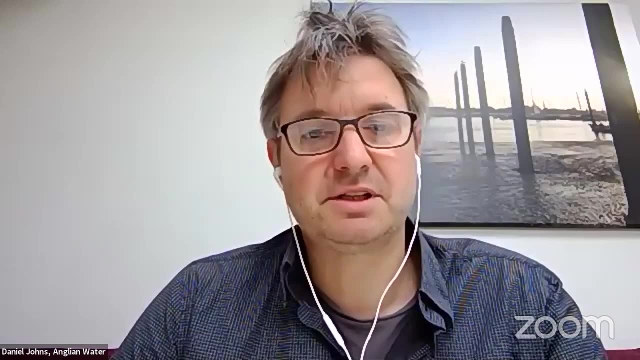 operationally but involve much more of a carbon footprint, and so i think it's a good idea to have much lower carbon footprints in terms of the- uh the capital cost of those. uh, those works much less concrete, much less steel, much more kind of nature-based solutions, uh, and so one of the things 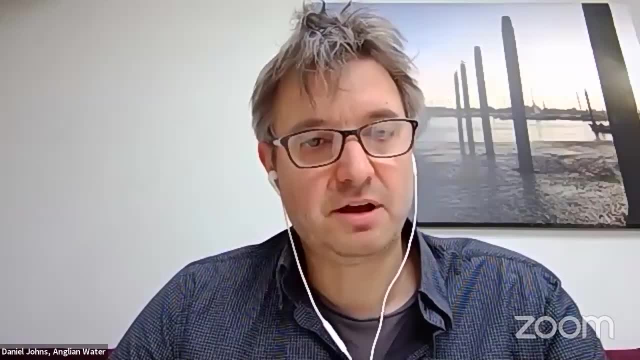 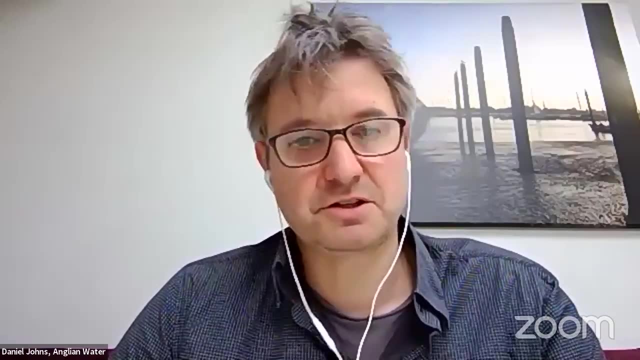 that we are encouraging and, i suppose, incentivizing our suppliers to do is to think differently, more in a kind of six capsules approach, rather than just trying to kind of pitch the lowest cost solutions in response to a particular kind of operational needs. and so yeah, the supply chain. 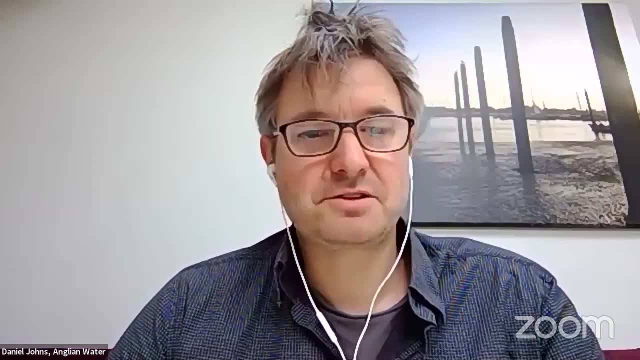 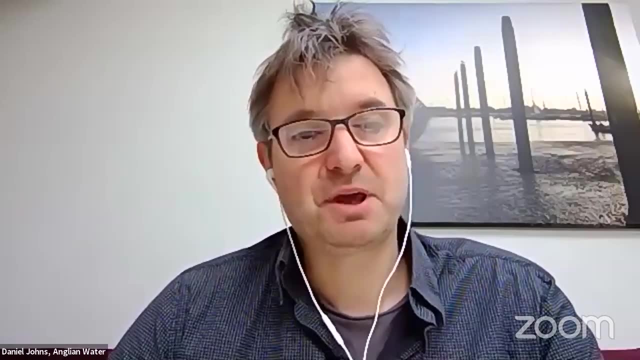 is absolutely kind of key to what we're doing and through those kind of long-term alliance partnerships we've got that last, in some cases 15 years. we we've got the right incentives in place to come to for them to be bringing forward, uh, solutions that both meet the 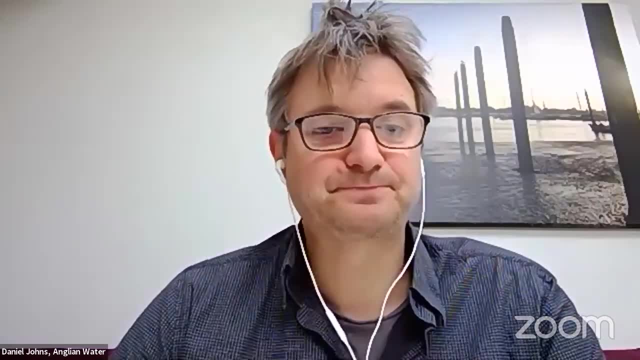 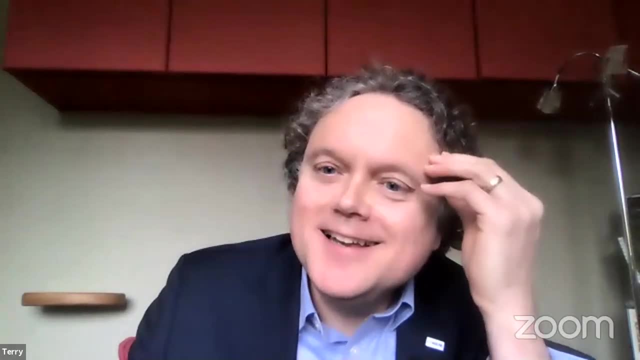 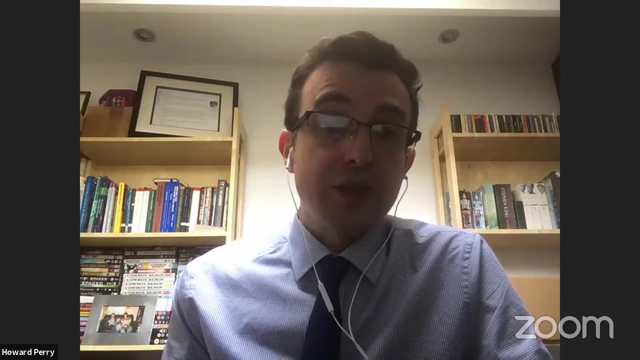 climate change challenge, but also say that the nature emergency too. thank you, and hannah k, would you like the the last word in the final 20 seconds? we've got no, if i can very, very quickly. i think that's another example of where we've we've learned from experiences. so chemicals is a. 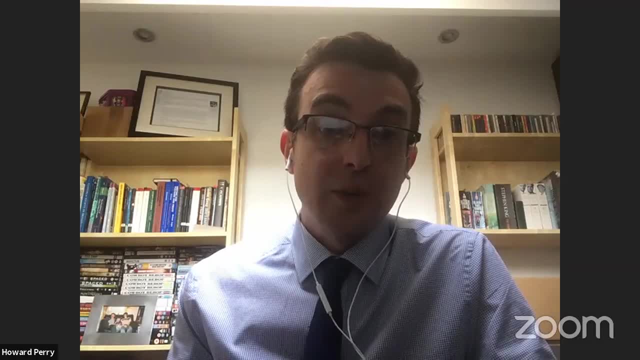 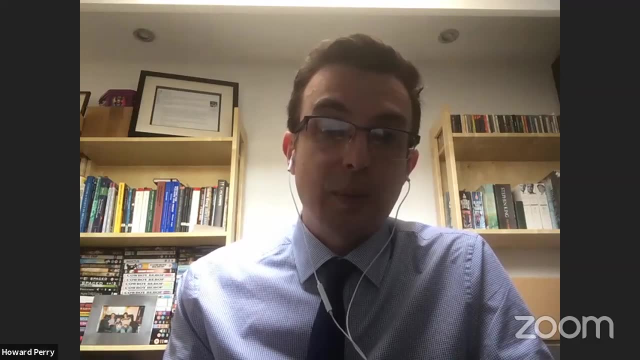 classic example: key supply chain for us. we absolutely rely on those chemicals. we've seen occasions when there's been risks to that supply chain and we've done things about it to strategically try and cope. so some of the adaptation is is happening more to do, i think. and on carbon, 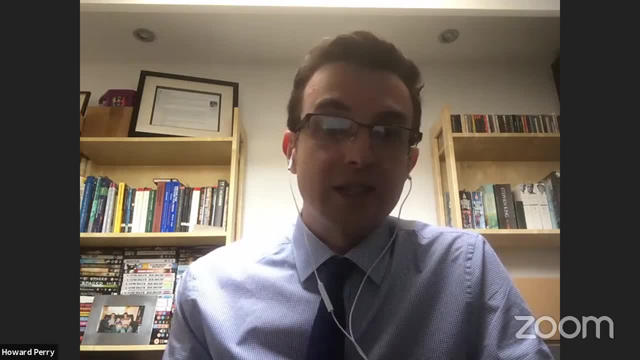 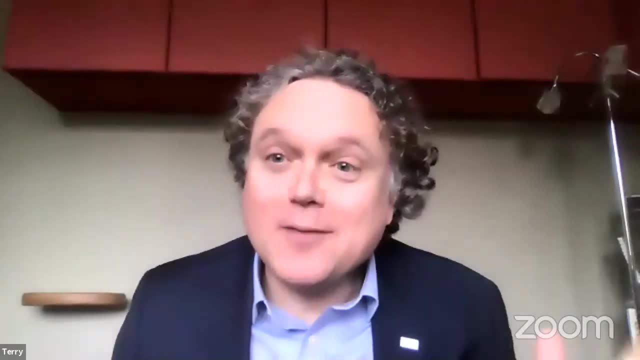 reduction. some of weaning ourselves off fossil fuels in the supply chain, for example, does help as well on the adaptation journey. yeah, thank you. okay, um, i'm afraid i'm going to have to stop the the questions there, otherwise i will be in a lot of trouble with the team for running over time. 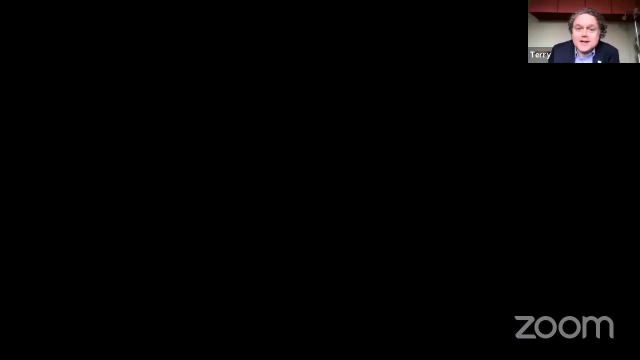 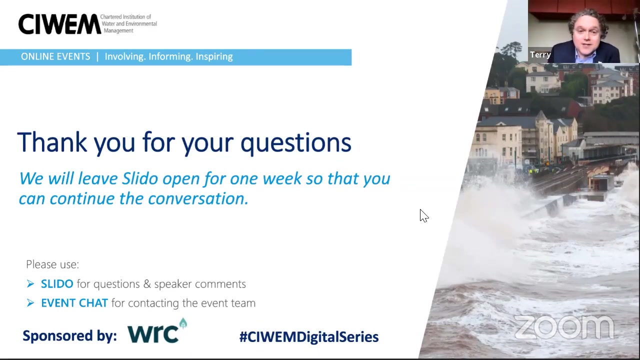 but i'd just like to say a massive thank you to, uh, all of you and our speakers this morning for what's been a really fascinating two hours. it could easily have been eight hours, i think. um, and let's hope the conversations do continue. um, i'd like to um thank wrc as for sponsoring this. 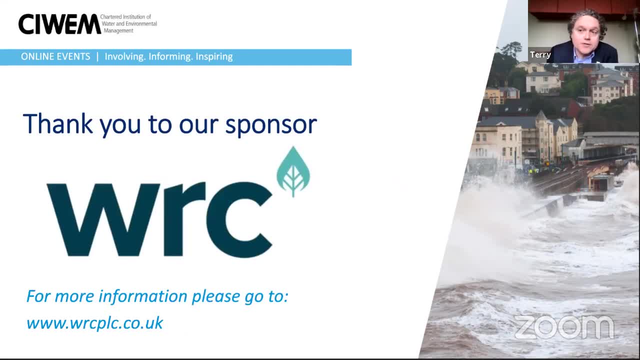 event. uh, we, we cannot put these events on without that kind of support. um, there's a lot of um work and and time and money that goes into producing these and um. that support is very much appreciated. thank you to, to wrc, um, and also to ccw as well, for your support, um also um. so that's, i'm afraid. 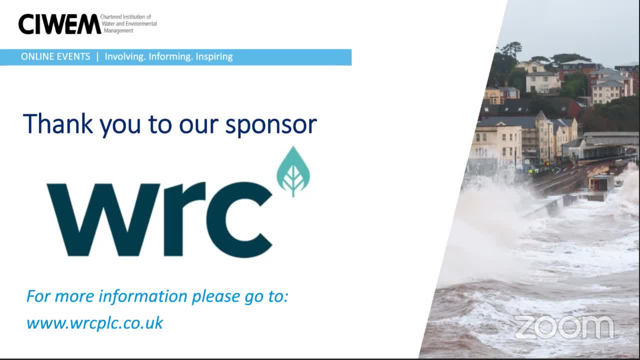 the the end of our session, but please do not go anywhere because, uh, this is our first venture into this new digital platform that you're viewing through today, and it's got loads of functionality in it and lots of opportunity in it to network and find out more. so please don't go away, please. 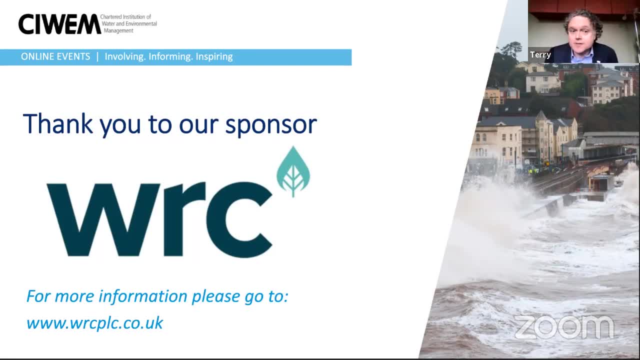 take time to visit the exhibitor booth and to hear from ccw and wrc and also cywem. membership and learning teams are also available for a chat there. um, there's also a networking space as well where you can chat with your fellow attendees. so if you had a particular question and or you want some sort of discussion, 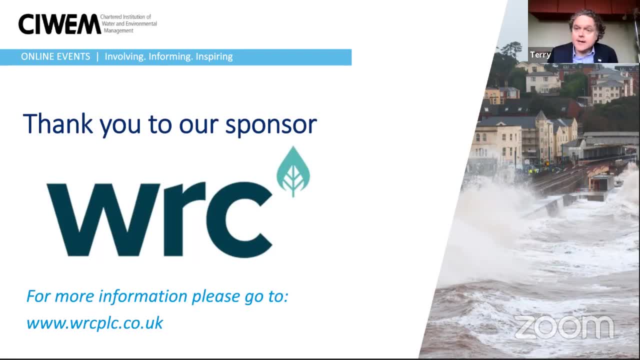 to go on. there's your opportunity to do that. um, now, we will be producing a post-event report which we will send to all of you in the next few weeks, and also we have recorded this session as well. so if you have any questions, please feel free to email us at ccw and wrc and we'll be. 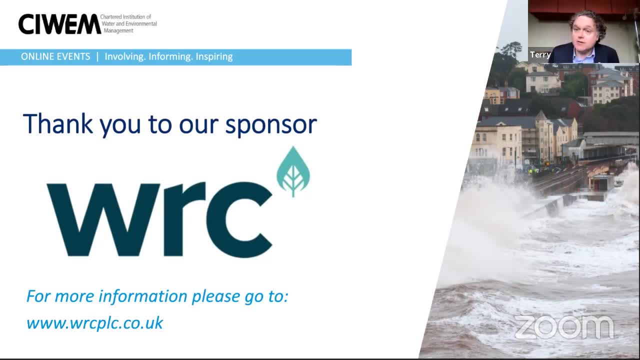 as well. so it will be available uh to you in about 72 hours time, um, through our youtube channel. okay, and uh. finally, we do really want to hear your feedback. we are constantly looking at how we can refine and improve our webinars and make them more engaging for you. um. so please do, um, give us your 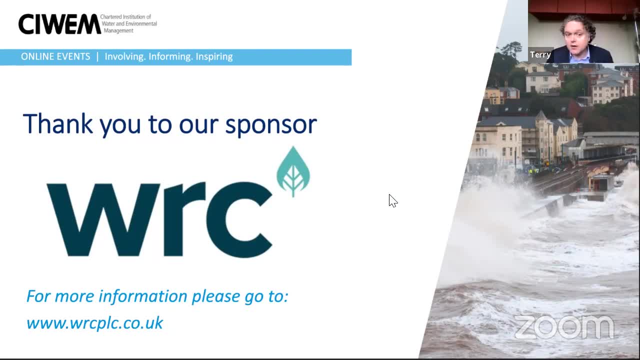 feedback. uh, you can do so in the poll area on slido um, and if you have two minutes um to uh to do that, that'd be um, that'd be really great. thank you, um, and, as i said right at the start, please do get in touch. uh, siwem is a fantastically.